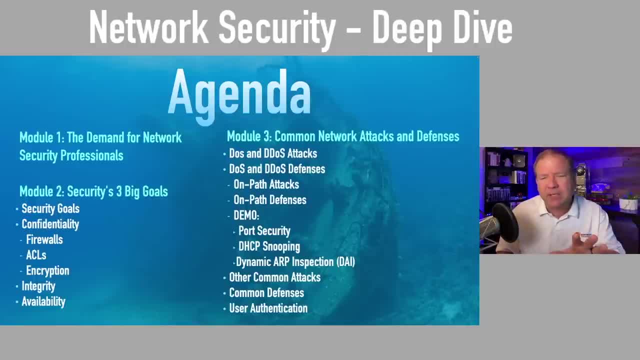 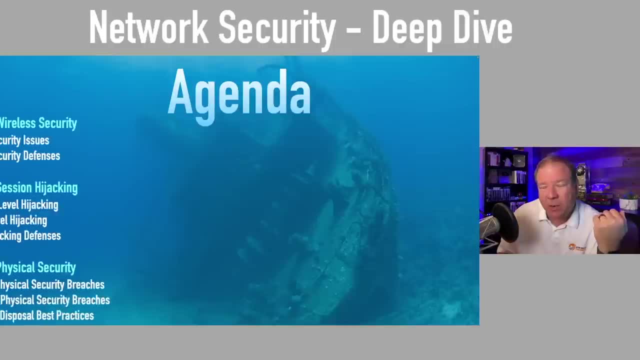 throughout. We'll probably have a couple of major breaks during today's session. Just guessing, and this could vary a little bit. this is just a guess. I'm guessing today's session is going to run about five hours, So you might want to think about that and what you have coming up over the next few hours. 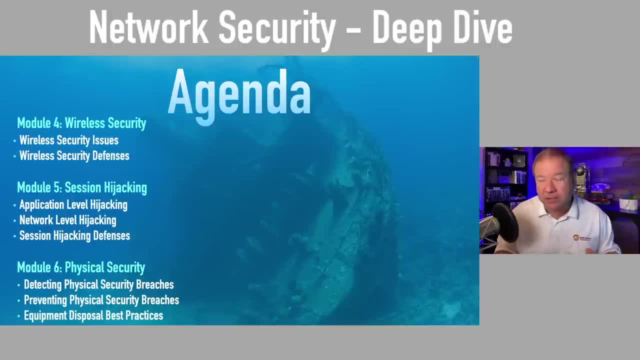 But coming up in module four, we'll get into wireless security. There are all sorts of wireless security standards, and not just wireless in terms of Wi-Fi. but here's a Bluetooth- It's called an Ubertooth One. Here's a Bluetooth adapter We can actually do some hacking with. 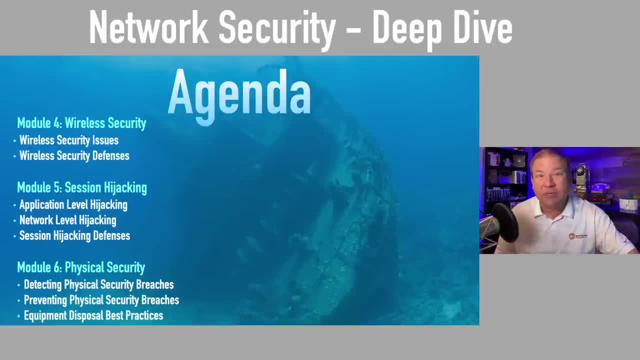 Bluetooth. We'll get into that as well. talk about how we can protect ourselves against that. Then we'll spend quite a bit of time talking about session hacking. So we're going to be talking about how we can protect ourselves against that. You see, here's the deal, Instead of trying to guess or figure out somebody's password to get. 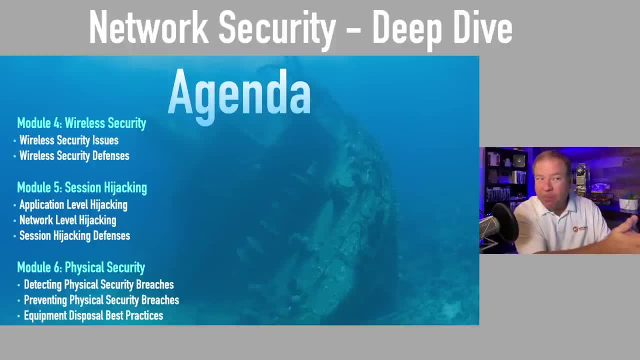 logged into something that they have access to. what if we wait for them to gain access on their own? They log in, they give their credentials, they're talking back and forth, They've got that session established And then we- well, not we, but a malicious user hijacks that session. That 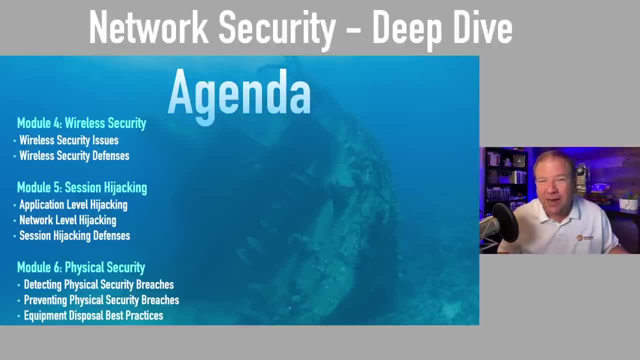 lets them bypass the whole process of being authenticated. We'll talk about how session hijacking can happen and how we can protect against session hijacking. We'll talk about physical security, because we can have all these great protocols and systems in place, But if somebody can just walk up and get to the console, well, 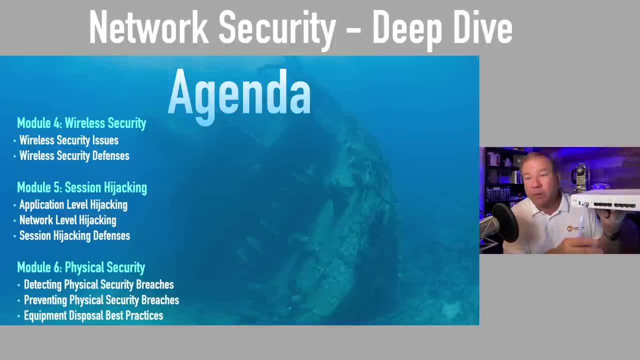 here's. I've got a got a Cisco Catalyst switch right here that we're going to be using for a demo later on. If somebody can get access to the console, they can own your device pretty much. They can do password recovery, So we want to have physical security as well. 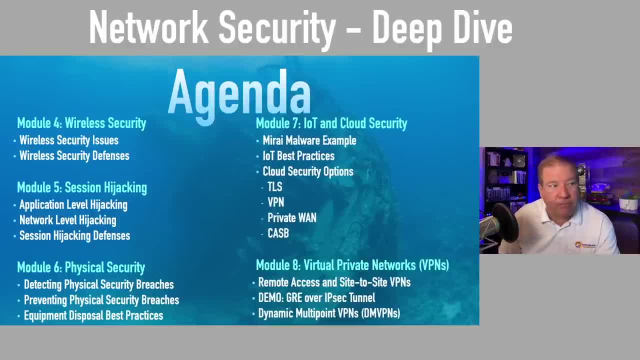 And we'll talk about some of the emerging security threats that we haven't traditionally thought a lot about- or at least I haven't- And that's with internet of things, devices and for cloud: How do we protect as we're moving our resources and our data from centralized data? 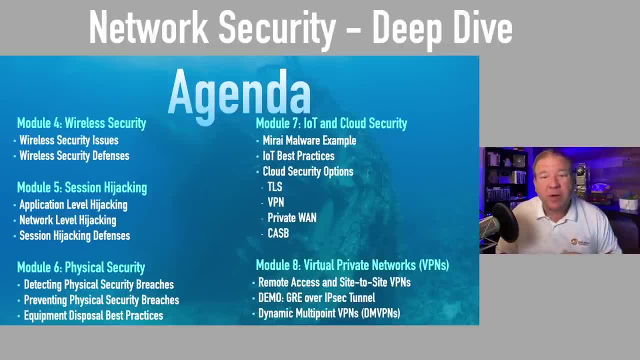 centers on premise at our site out to a cloud service provider And we're going to see. one way of getting that security to the cloud- And we're using it more and more- is VPN technology, virtual private network, Virtual private networks. We'll talk about different types of protocols that can be used. 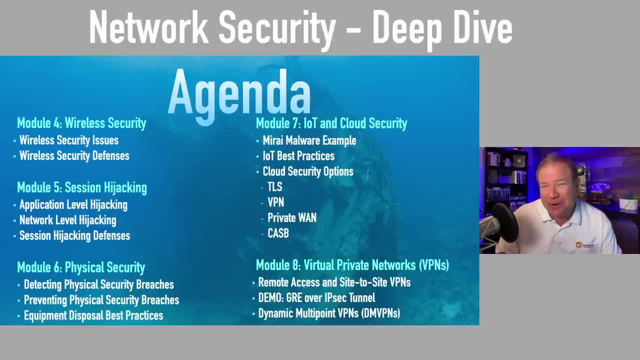 how we might use some of them together And I think you'll really enjoy that VPN discussion And we're going to wrap it up with a discussion of dynamic multi-point VPNs. So lots of great security content coming up today. Hope you're excited. Hope you're going to take a lot of notes. 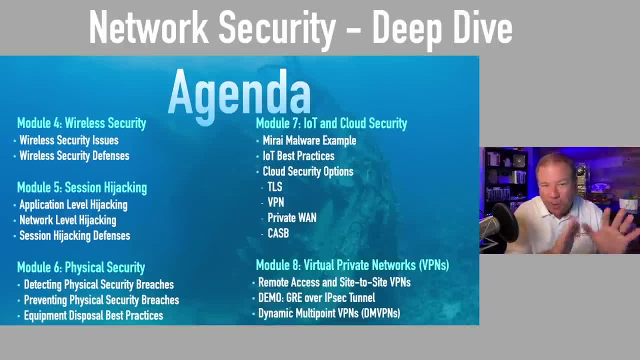 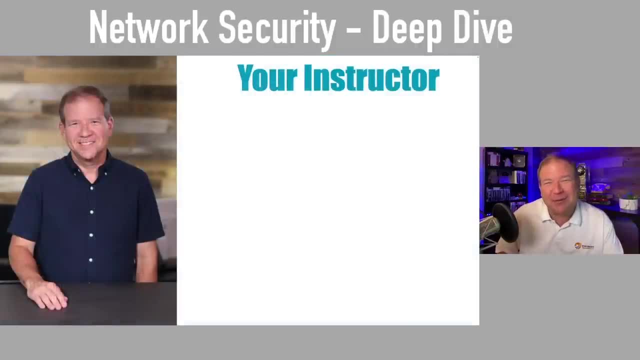 And again, I realized this is going to be a marathon session, So we will give you a couple of breaks throughout. And my brief bio. I'm spending a lot of time together. Here's where I'm coming from As I approach this topic. 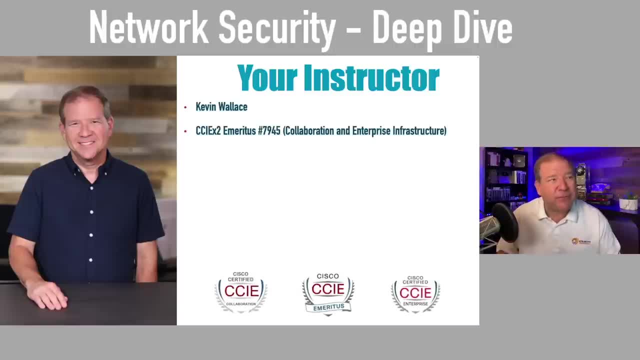 my name is Kevin Wallace. I've got a couple of CCIEs. I got my first CCIE way back in 2001.. It was the route switch CCIE And I've since then upgraded it or updated it to the CCIE. 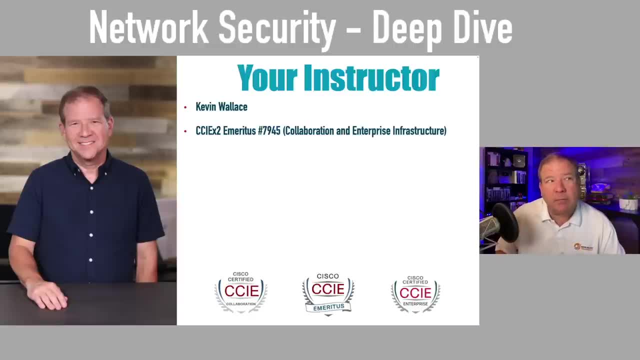 enterprise infrastructure I've also got. in 2012, I got a CCIE in voice and I've since upgraded that to a CCIE in collaboration And now, being a CCIE for 21, plus years, I've reached lifetime emeritus status, So I don't have to retake anything. 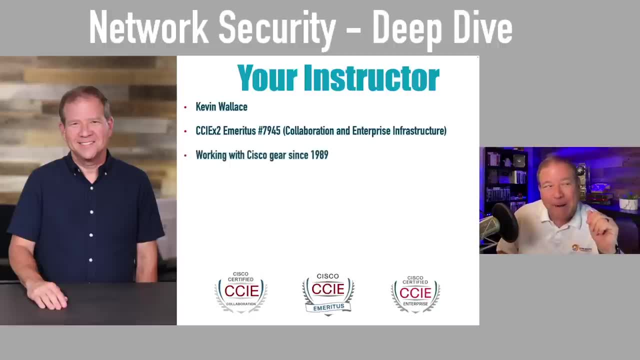 I get to just keep my CCIE for life And that really makes me happy. But I've been working with Cisco gear really since the very first Cisco router back in the late eighties, the Cisco AGS plus router. That was the first router I worked on And I've been working with Cisco gear ever. 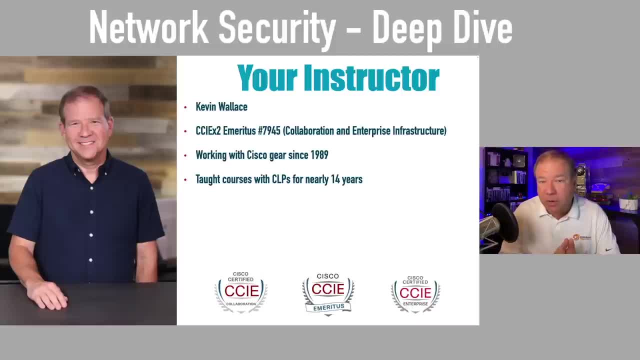 since I've taught courses for Cisco learning partners for about 14 years before I went into business for myself About eight years ago and started teaching these courses online in the real world- One of my favorite jobs ever- Okay, It was my favorite job ever in the real world because my family and I 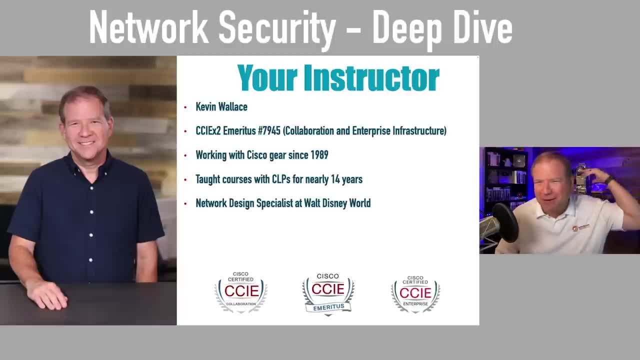 were huge Disney fans. You can probably see some little Disney artifacts on the bookshelf behind me. but I got to be one of five network designers down at Walt Disney world in Florida. That was just an amazing experience. I got to design the network that tied together the magic. 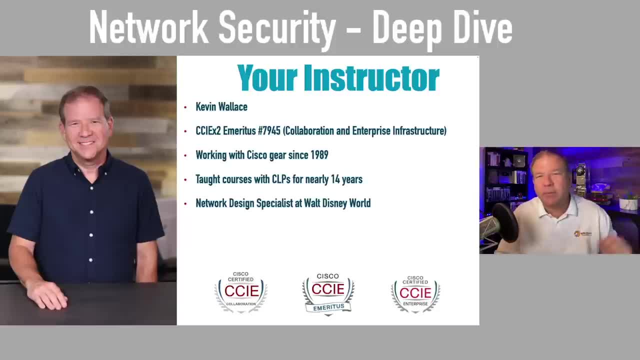 kingdom and Epcot and the studios and animal kingdom and a bunch of the resorts just had a great time And I've written a bunch of books, done a lot of video courses for the folks over at Cisco press And I've been privileged to speak at a couple of Cisco lives and each time got the distinguished. 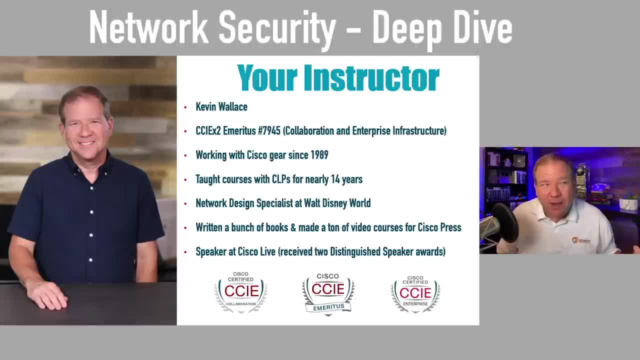 speaker award. Bottom line is: I've been doing this for a while and I am passionate about it. I love this stuff and I cannot wait to add some value to you today, because we're going to be touching on security concepts that show up in a bunch of different Cisco and non-Cisco exams. 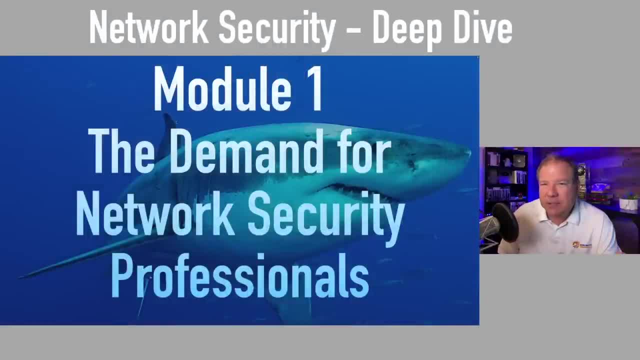 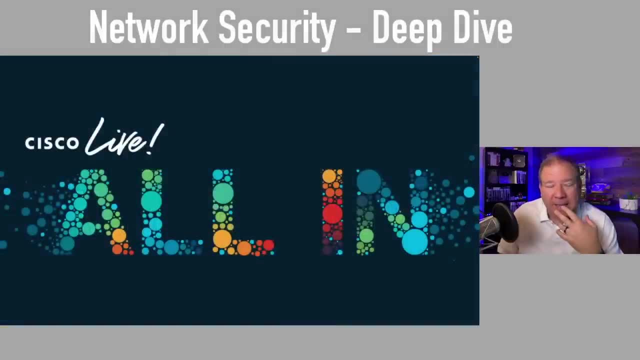 Let's get started here in module one by just getting a sense the incredible demand we have in the industry for network security skills. I attended Cisco live earlier this summer out in Las Vegas- Yeah, let's see, It was in June, actually June of 2022- and got to meet a lot of people. after being 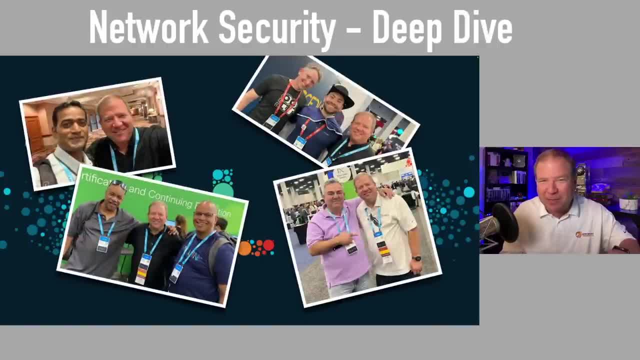 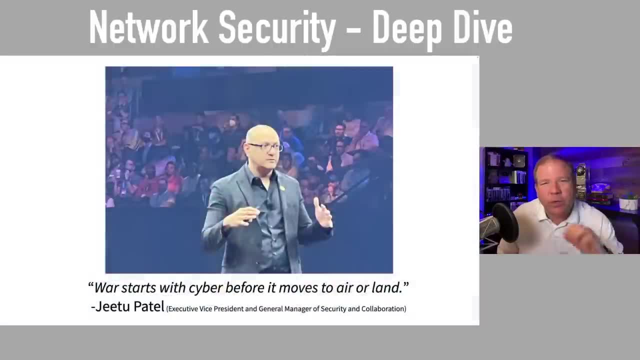 sort of shut down and doing it virtually for a couple of years. It was great to see people face-to-face. I got to meet a lot of people and I attended the keynotes, and one of the keynote statements that really stood out to me was this: It was from a G 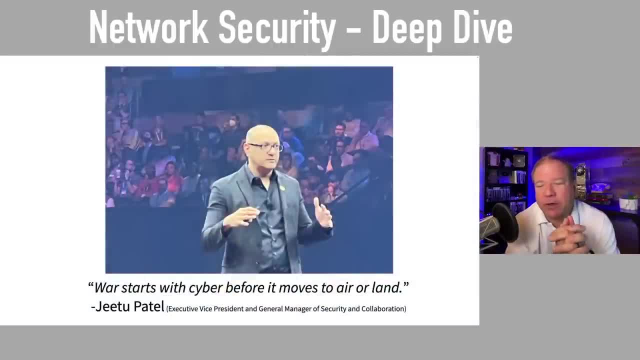 Patel. He's the executive vice president and general manager of security collaboration with Cisco, And when he said this it just jolted me. I thought, wow, that is so true. He said war starts with cyber before it moves to air and land. Think about that When there is war. 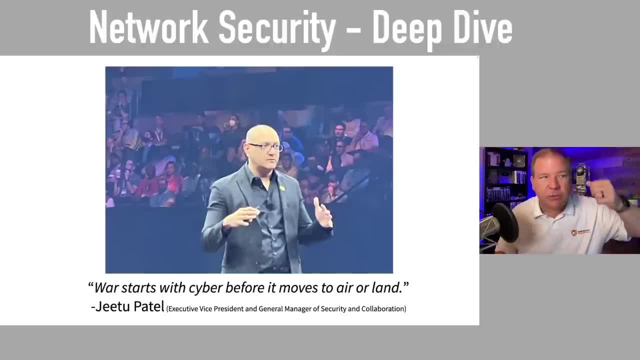 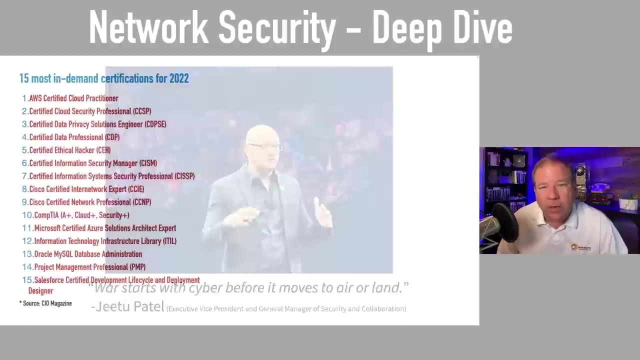 between countries, instead of launching some sort of offensive strike with missiles or something. the first attack is probably going to be cyber, a cyber attack, So we want to protect ourselves against those kinds of attacks. It is so, so critical. In fact, we see that reflected in this year's list of the 15 most in-demand. 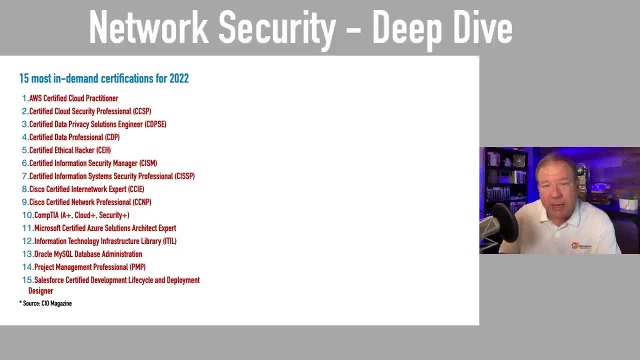 certifications. This is from CIO Magazine And one of the big security certifications out there is CEH, the Certified Ethical Hacker Certification. I'd like you to notice that it shows up as number five on this list. It actually beats out. 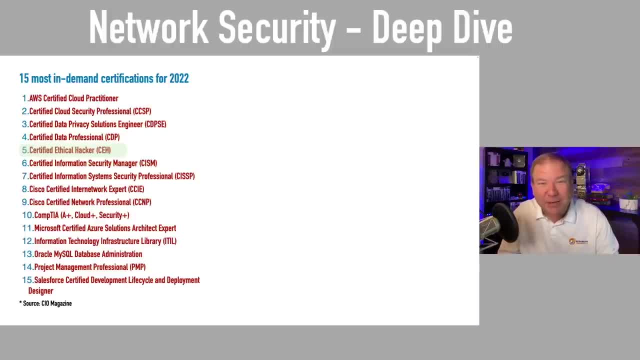 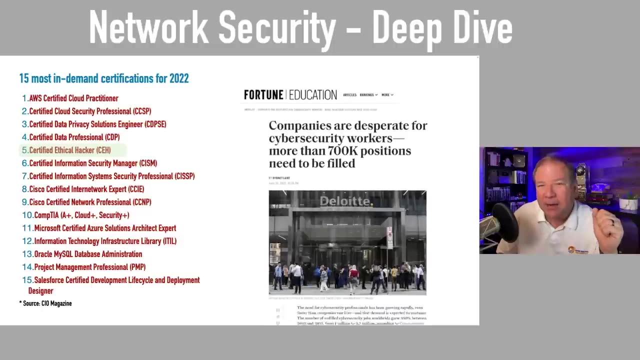 The Cisco CCNP and Cisco CCAE. They're on the list as well, in the top 10.. But Certified Ethical Hacking beats out these top tier Cisco certifications for certs that are in demand in 2022.. And back in: at the end of June this year, Fortune Magazine had this article that I was 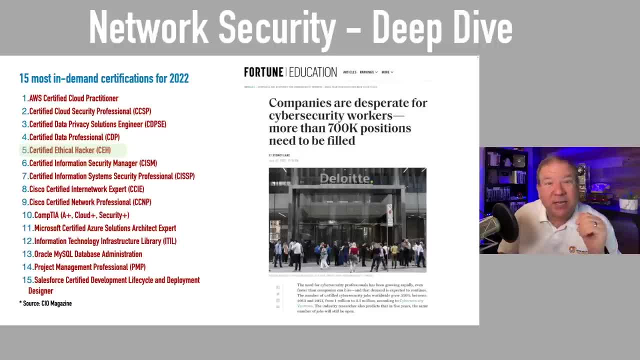 reading And I love the headline. It says: companies are desperate for cybersecurity workers. Currently, there are more than 700, 100,000 jobs right now that need to be filled And if you're watching this in replay, a month or 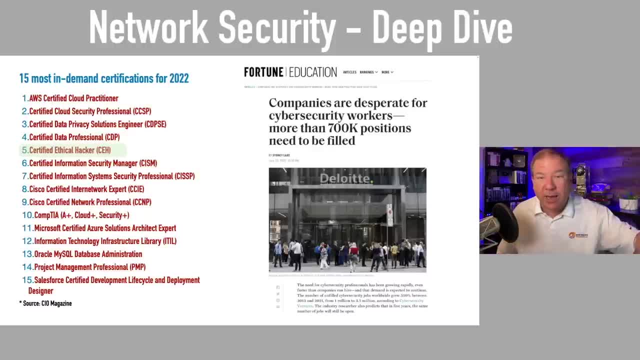 two down the road, it might be even more than that, But the forecast is throughout the rest of this decade, every year. we're not going to make up that shortfall. There's going to continue to be this lack of cybersecurity professionals, So this is something that we need to know. 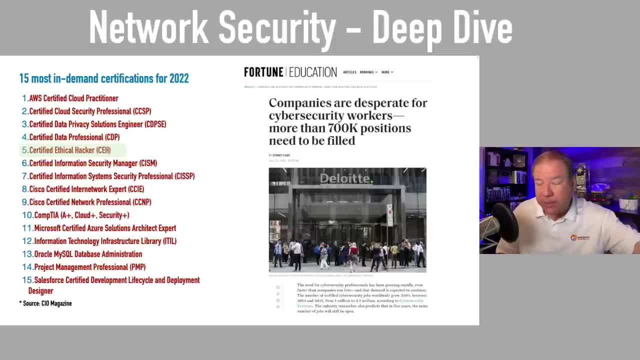 whether we want to go into that as our primary focus in our IT careers or I'm kind of a collaboration. I love collaboration, I love regular enterprise technologies, But in all that there's security. No matter what your focus is, you've got to know about security. I've never I've been doing this. 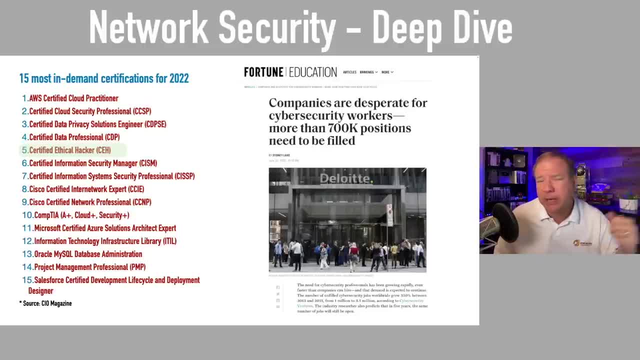 for what? Over 30 years, Yeah, 33 or so years right now, And I've never seen a demand in the industry like we have a demand for security professionals today. So this is going to be critical stuff to know And hopefully I've sold a lot of stuff. I've sold a lot of stuff. I've sold 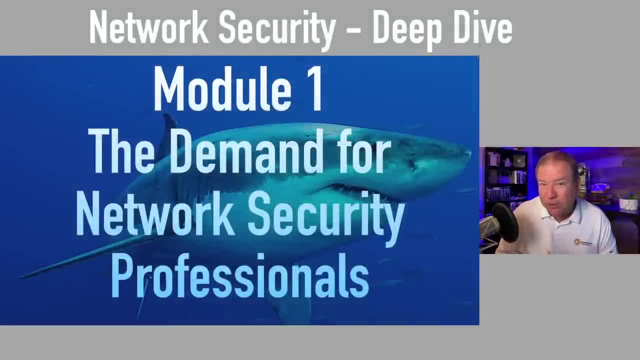 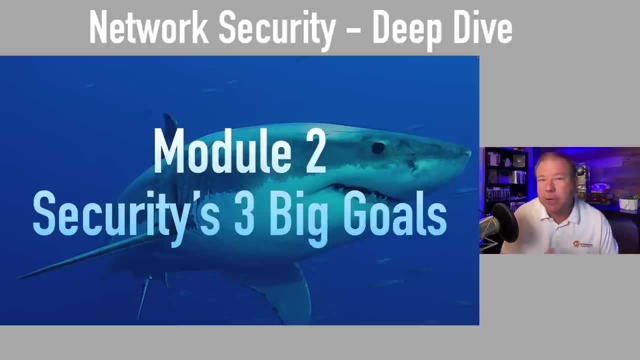 you on the fact that this is super important to your career. whether you're going to focus on security or not, you still need to have a base knowledge of it so you can be conversant with other people in the industry. But let's get in to the three big goals of security. What when I say 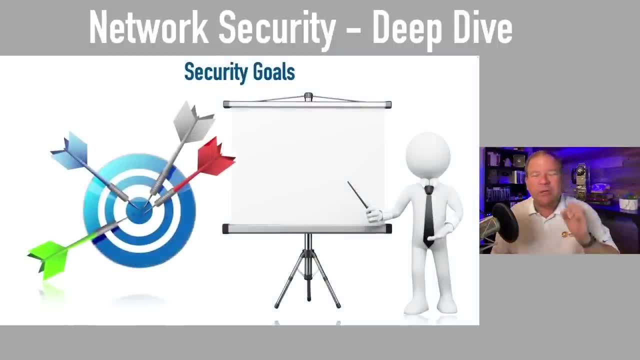 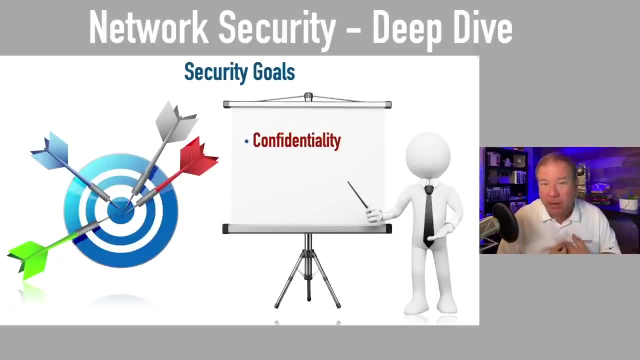 we're securing a network. what exactly does that mean? What targets do we have? Well, first up, I'm talking about confidentiality. I don't want somebody to read my email. I don't want somebody to be able to get on my server and look at my files. I don't want them to print to my 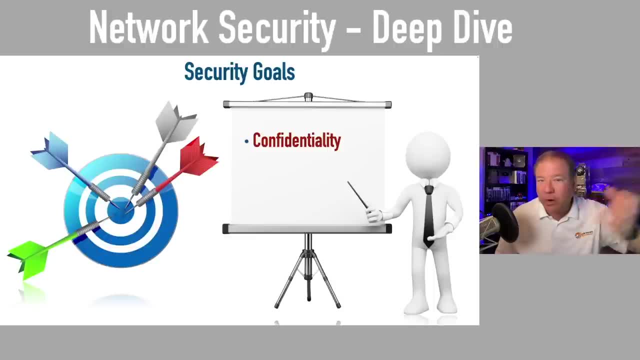 printer If they capture traffic going across the wire or going across the airwaves over an antenna. I don't want them to be able to read it. I want to have confidential communication and confidential storage. We also want to make sure that our data has not been modified. We want to check the 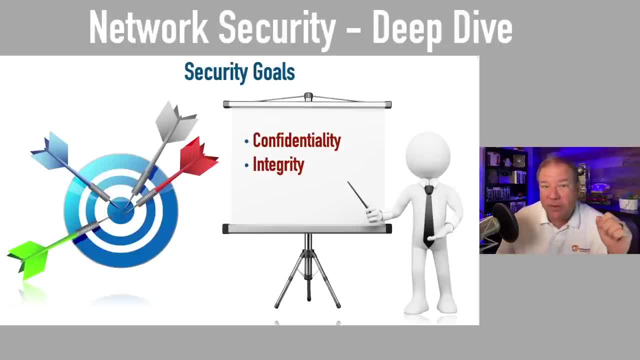 integrity of that data, And one of the things we have to defend against is somebody just bringing our system down. You've noticed that there's a lot of data that's not being modified. There's a lot heard about DDoS- denial of service attacks. That's where an attacker just floods a system. 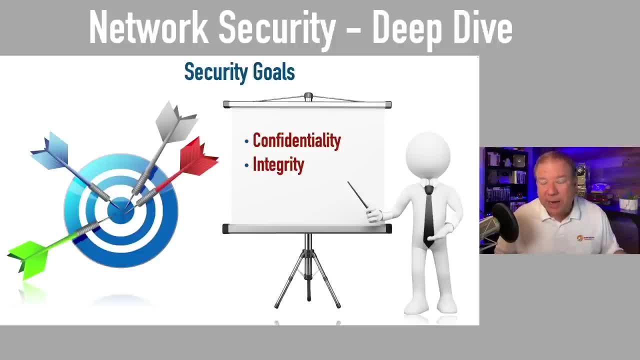 with so much traffic, that system is not able to do its regular job because it's dealing with that onslaught of junk data coming into it And that can bring our system down. We're being denied service to our system. In other words, we want our systems to be available And we're going to 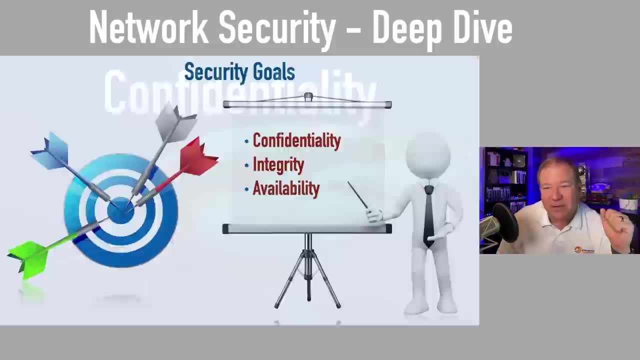 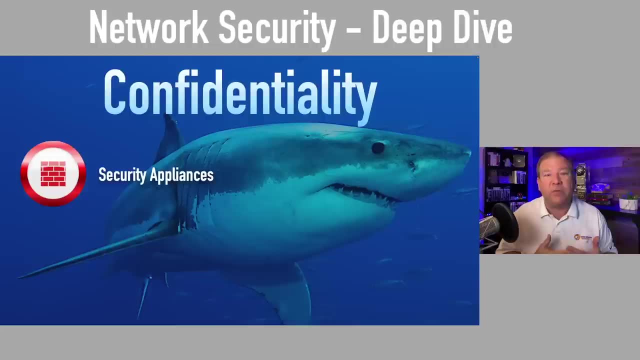 talk about what metric defines high availability. First, though, let's focus on confidentiality. One way we can have confidentiality is through a variety of security appliances that we can use in our network. We'll be talking about those here in just a moment, But in addition to that, on our Cisco routers, as an example, we can use ACLs. 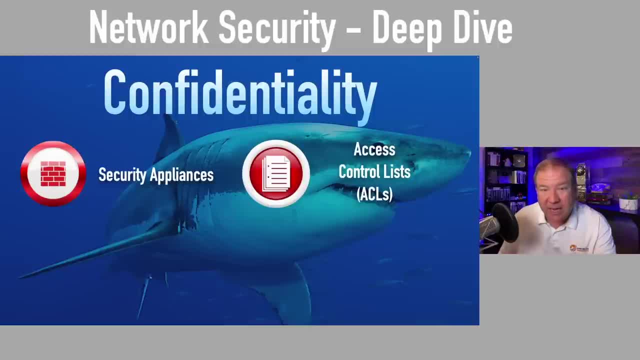 access control lists And I'm going to be showing you the syntax And I'm going to be challenging you with some troubleshooting scenarios, with ACLs coming up here in a moment. And also we're going to encrypt our traffic. When I say encrypt traffic, we're going to take our data string and we're going to scramble it up. 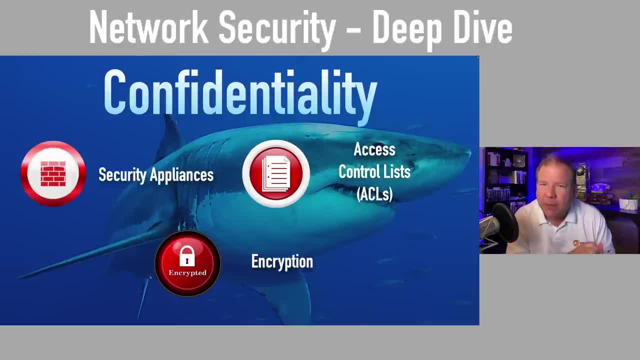 And, as part of that scrambling up, we're using a mathematical algorithm And that algorithm is probably going to use something called a key. Might be 128 bits in length, might be 100.. It can be varying number of bits, But this key is something that's going to be maybe secret. 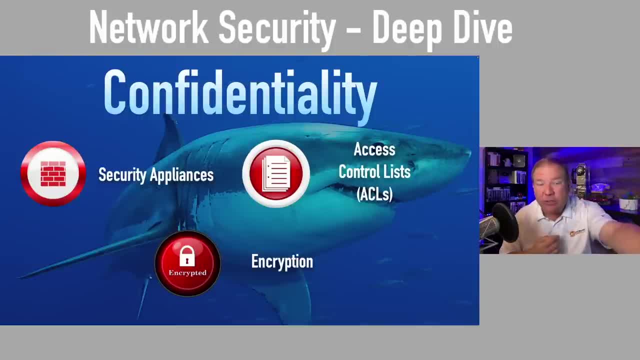 depending on how we do it. And if I use a key and you use a key, and we use the same key to encrypt and to decrypt our data, if somebody can't encrypt our data, we're going to have to use a key. And if somebody captures it in the middle and they don't have that key, they're not going to. 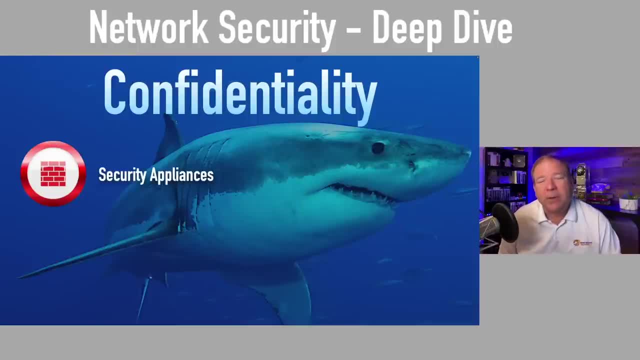 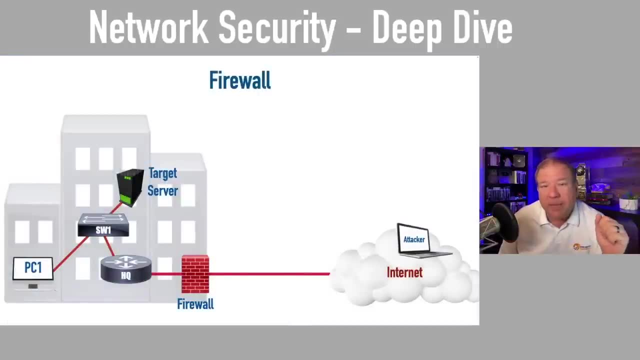 be able to read our data. We'll talk about some different encryption options, But let's get started by taking a look at some different security appliances. One that you've probably heard a lot about is the concept of a firewall. Now, a firewall is generally going to stand guard at the perimeter. 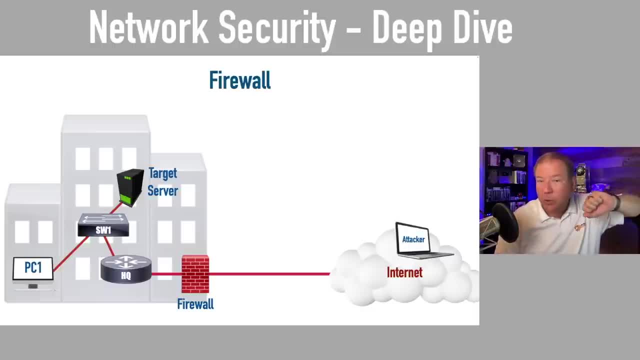 of your network as you go out to the internet or you go out to a wide area network, or maybe you go to just a different area of your network And that's going to be a firewall And that's going to be a network with a different security level. But a firewall is basically a set of rules to say what. 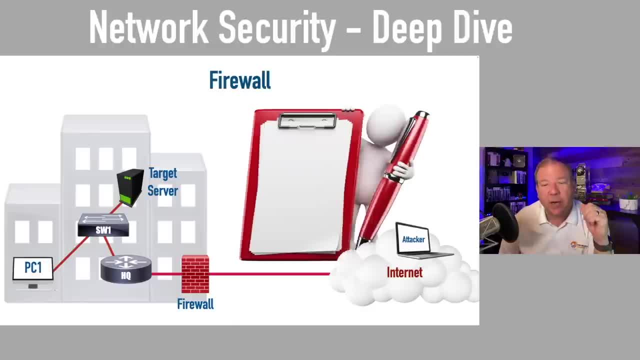 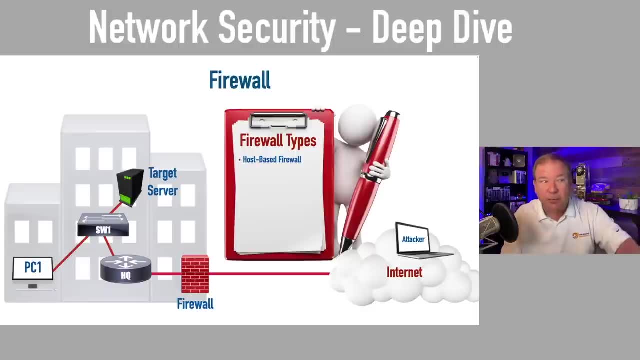 traffic is permitted to come in, what traffic is permitted to go out. And let's talk about some different types of firewalls. One type is maybe running on your operating system on your desktop or laptop computer right now, If you're running Microsoft Windows or macOS or Linux, just about. 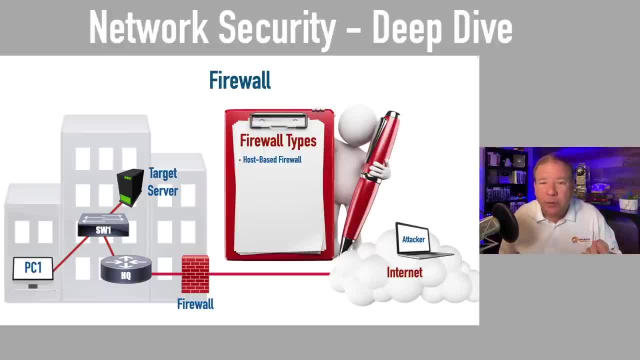 any operating system, there's probably an option for you to use a software-based or a host-based firewall. So if somebody's trying to get to your computer specifically, you can set up some firewall rules to allow or deny that kind of activity. Now that's on sort of the micro level getting down to 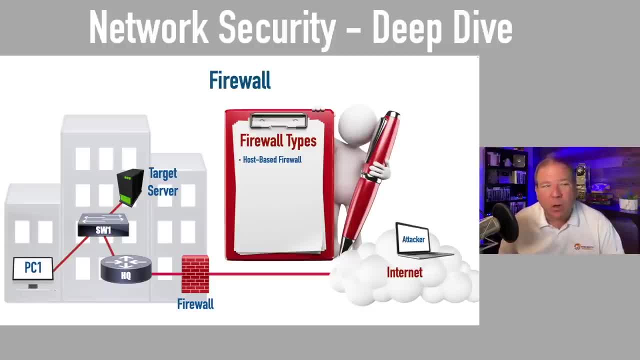 the individual devices, But oftentimes we think of firewalls as being an appliance that's going to sit at the boundary of our network And a very rudimentary type of firewall, and I even hesitate to call this one a firewall, but I want you to know it because it might show up on an exam someday. 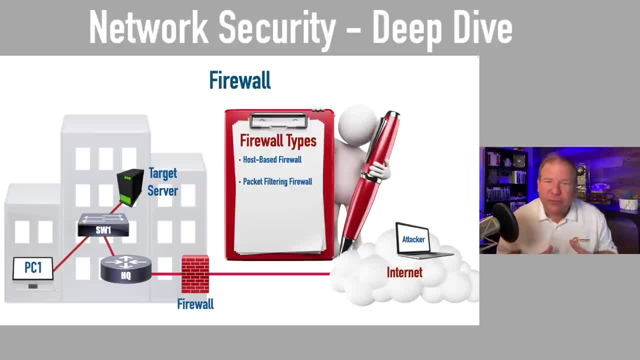 is a packet filtering firewall. When I say packet filtering firewall, I'm talking about an access control list, really A set of rules to say this section of the network or this IP address or these IP addresses they're allowed to go out or they're not allowed to go out or they're not. 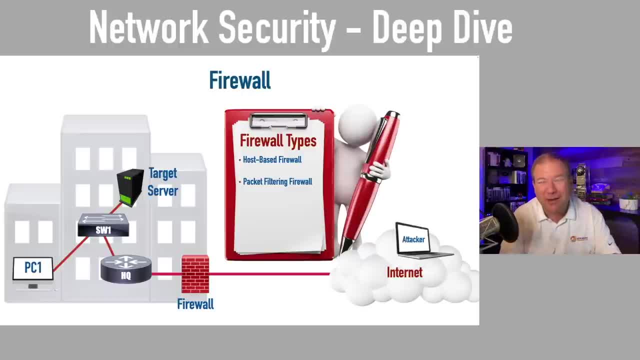 allowed to come in. For example, this would not be a good use of a packet filtering firewall. Let's say that we set up a router at the edge of our network going out to the internet and we thought: inside of my network, I'm going to allow them to come into my router and go out to the internet. 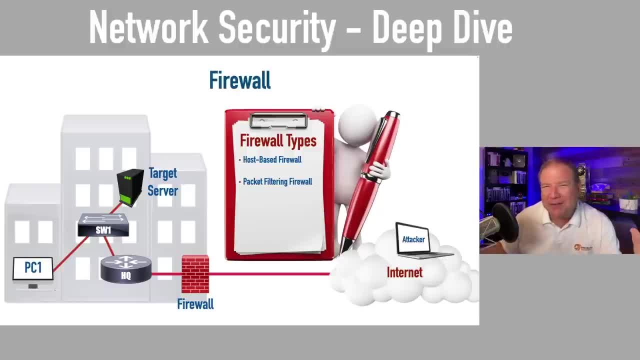 But I don't trust the internet because there's a lot of bad actors out there, So we set up our access control list to block traffic on the internet from coming into us. Think about how that would work, though, or how that would not work. Let's say, you're on the inside, you're a 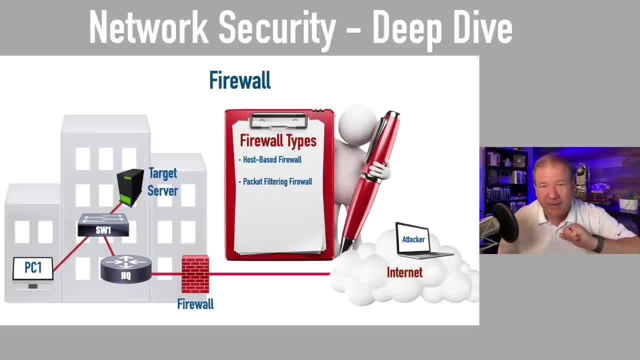 trusted individual and you're trying to go to a website on the internet. Well, as that packet goes into the router, it says: oh, they're good people, they're on the inside of the network, let them go out to the internet. 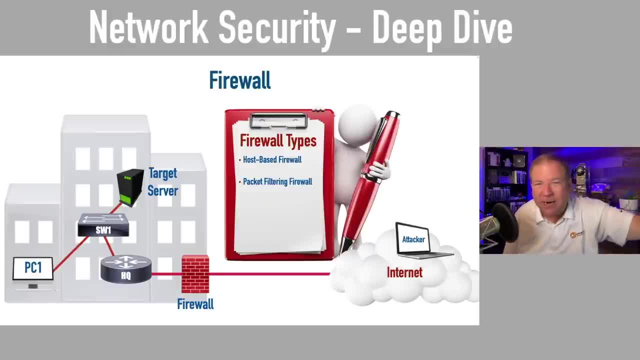 And you go to the internet website. The internet website is trying to send you the page that you requested back, but when that page comes back into the router, the router says no, no, no, you're coming from the internet. I don't trust you and it's going to drop that. You see, we're. 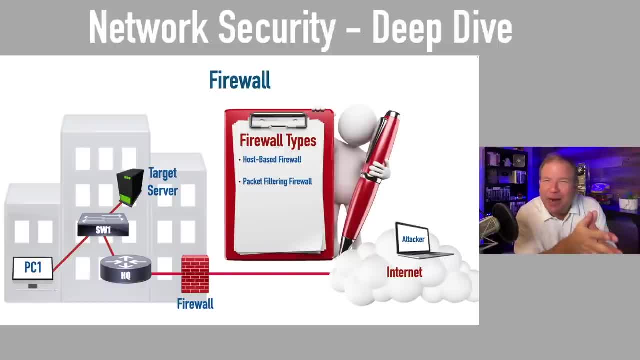 not getting two-way communication. so sitting at the boundary of our network, that's not a good place to use a packet filtering firewall. What we might do instead is use a stateful firewall. Now here we're, overcoming that issue that I just described. 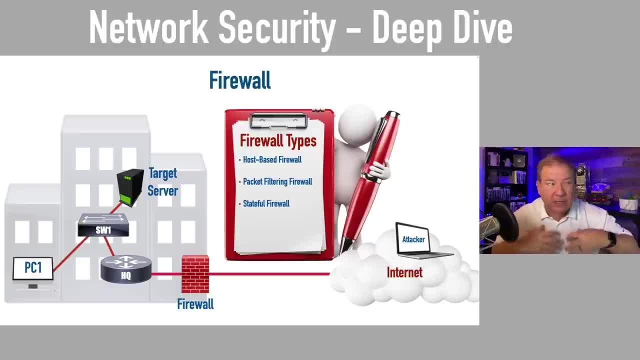 Remember the state of a session. Again, I'm on the inside, I'm trying to get to a device out on the internet somewhere and when I go into the router or into this stateful firewall, it's going to make a note of this. It's going to say: oh, I see this IP address on the inside of the network is going. 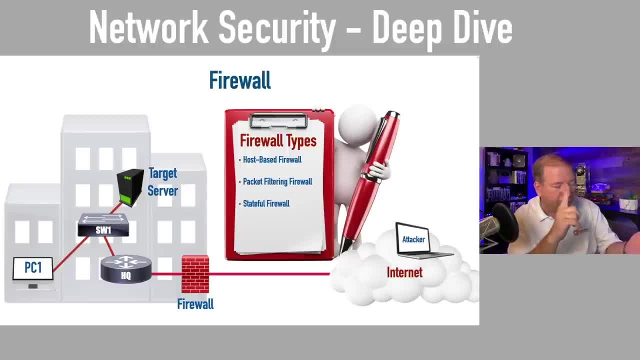 to this other IP address on the outside of the network, They're using this source and this destination port number. I'm going to remember that. Then, when that web server, in this example, returns that web packet, I'm going to remember that. I'm going to remember that. I'm going to. 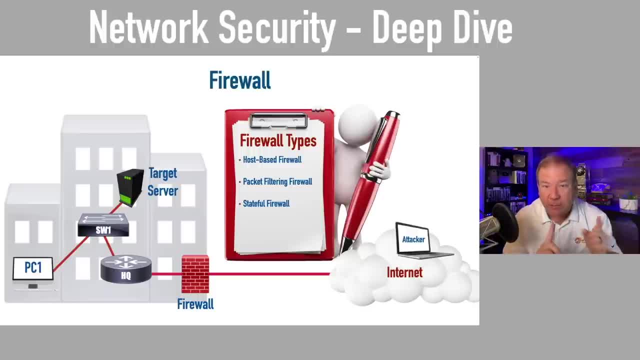 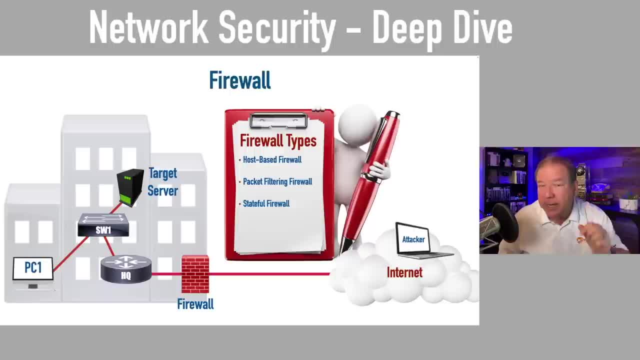 that's return traffic from a session- that here's the key- a session that originated on the inside of the network. I'm going to allow that traffic back in. That's a stateful firewall and that's what we used really for decades. In recent years that's been improved even more. 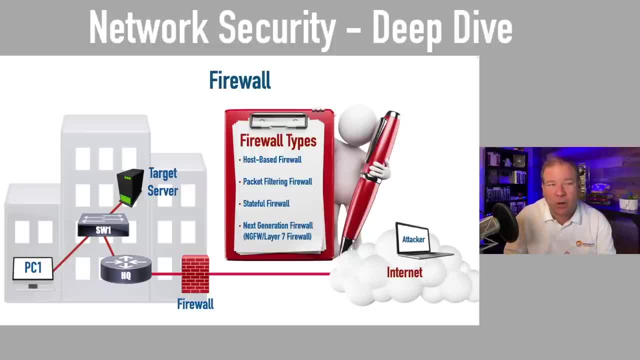 Now you might hear about a next generation firewall or a layer seven firewall. Here the firewall appliance can examine more than just IP address information. It can get into, as the name suggests, it can get into- layer seven information. It can understand how different protocols work together, For example. 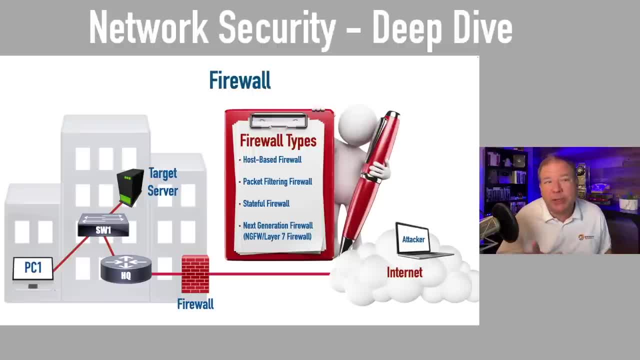 here's the first one that comes to mind. I do a lot in collaboration and when I'm setting up an IP phone call with a Cisco IP phone, I might be using a protocol called SIP, a session initiation protocol, to set up the session to make the phone call. But then once 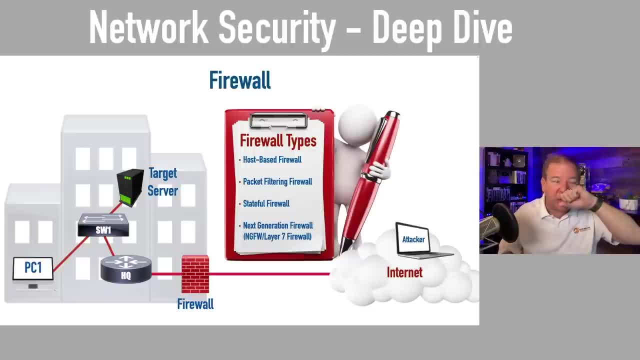 I start talking, that SIP session is going to let me start streaming my voice, and that's going to be done using the RTP protocol, the real-time transport protocol. Well, a stateful firewall is just the first example that comes to mind- is going to understand that. oh yeah, if a session. 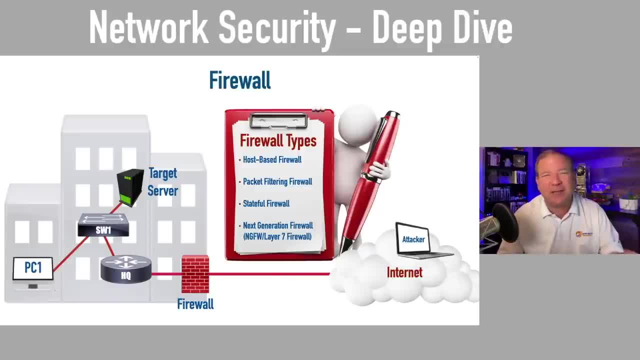 begins using SIP, then it might transition to RTP and it's going to realize: okay, that's still part of the protocol, So we can look into protocol-specific things in our streams and permit or deny traffic based on that. Something else we might want to do- and this is what we did at a university where I 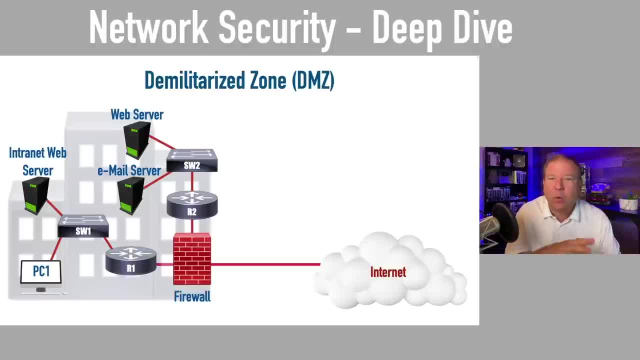 used to work years ago. we can divide the network into different security zones. What we had at the university was we had a connection out to the internet and one firewall port pointed out to the internet. We had another section of the university that was connected to the internet and 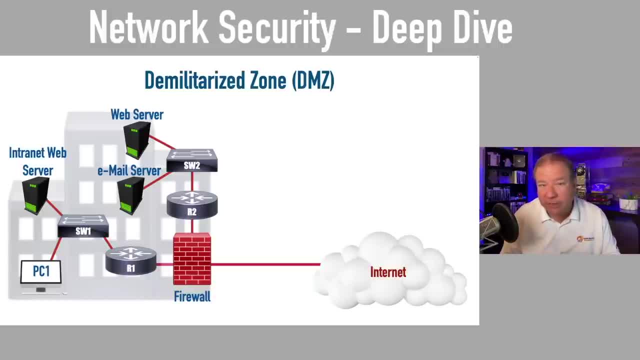 that contained the residence halls where the students lived, And we had another section that contained the faculty and the staff, the classrooms. We wanted to prevent somebody from sitting in their dorm room at night from getting into, maybe, a faculty computer. We wanted to put that in a different. 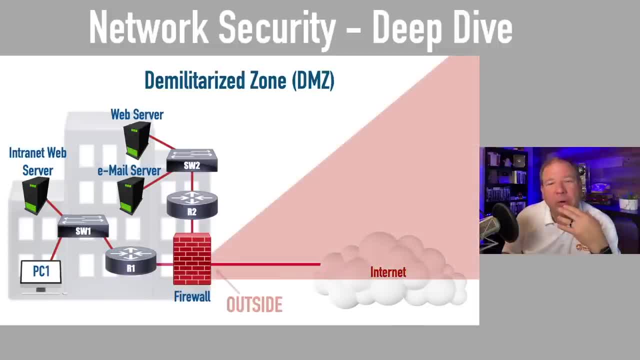 security zone. So what we did is we created what some people call a DMZ or a demilitarized zone. We had one firewall port going out to the internet. We had another firewall port going out to the internet. We had another firewall port going out to the internet. 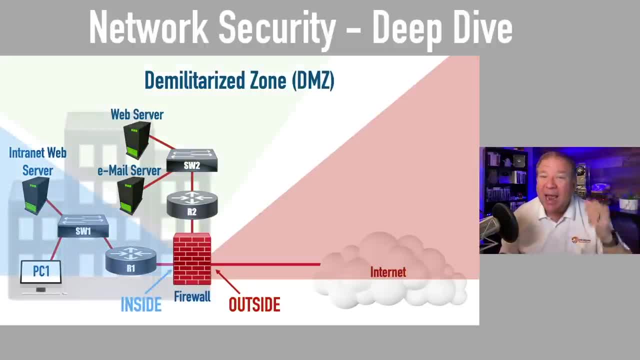 We had another firewall port going into the faculty and staff inside of the university and another firewall port connected out to the residence halls within the university. Another example: in the corporate setting we might have servers that we want to be available from the internet. 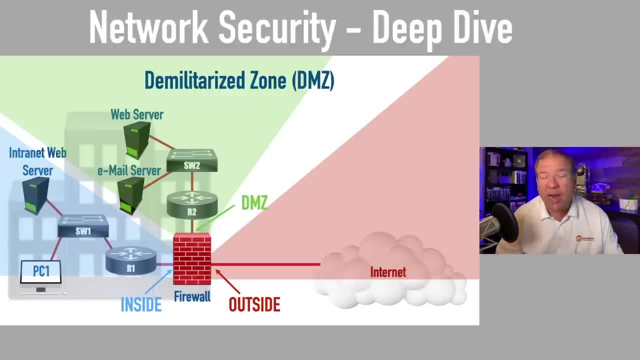 Maybe we have our own web server that we host locally. We have our own email server that we host locally. It's in our data center. People on the internet need to be able to access those servers, at least on social media. So what we might do is put those publicly available servers in a DMZ. We could still limit. 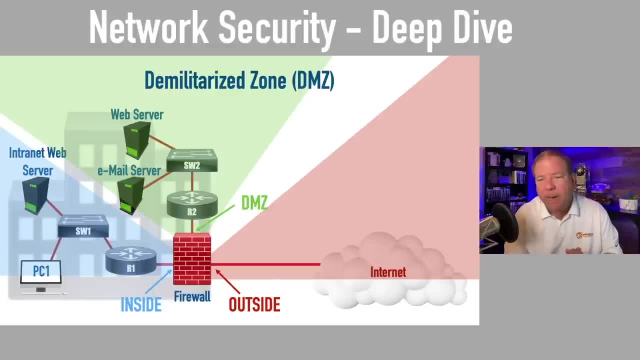 some things. We could limit what ports are going to be used. But if somebody were to compromise that web server, we don't want that to become a hopping off point to get in and compromise something in the inside network. So we can create this DMZ which is not going to have permission to start. 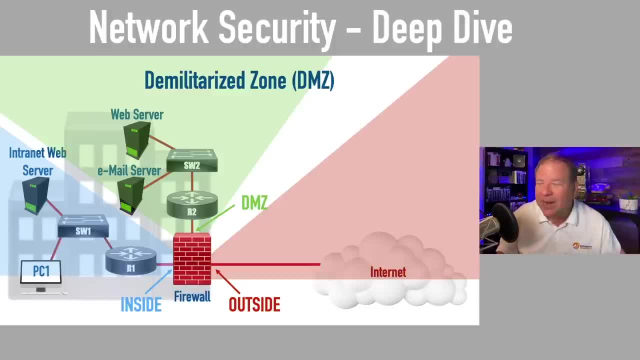 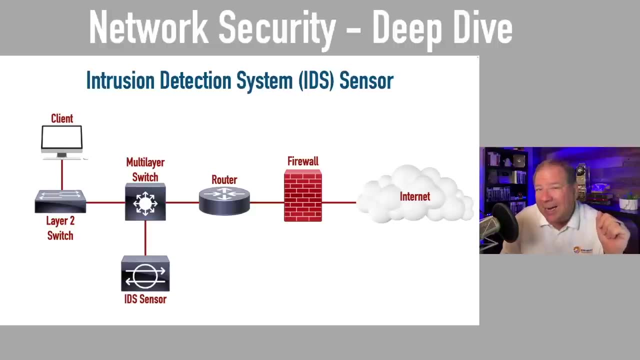 a session in the DMZ and then come in to the inside network So we can have these different layers of security. So a firewall. that's one appliance that we might have. Another appliance is called an IDS sensor, an intrusion detection system sensor. Here you'll notice that my IDS 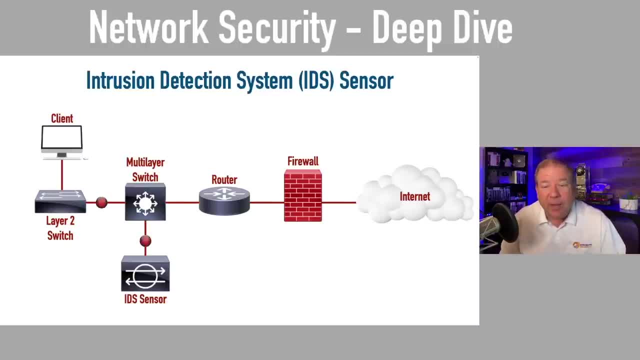 sensor is connected in to an ethernet switch And when a packet coming in from the internet hits that switch, the switch is making a copy of it. One copy is sent. well, the original packet is sent on to its destination, the client you see in the upper left-hand corner of the screen. 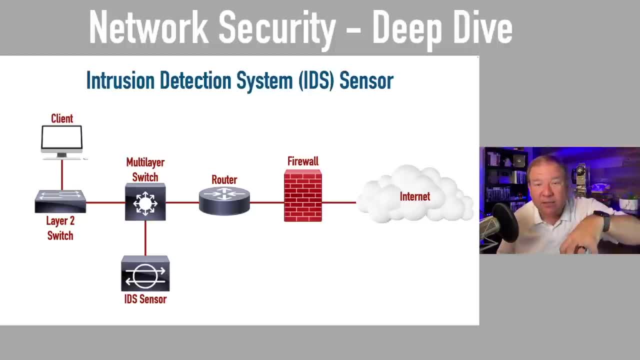 But the copy that it made. did you see? it went down to the IDS sensor. So the IDS sensor is monitoring traffic flowing through that switch And it's monitoring it for malicious patterns. There is what's called a signature database that the IDS sensor has And if it sees that there's 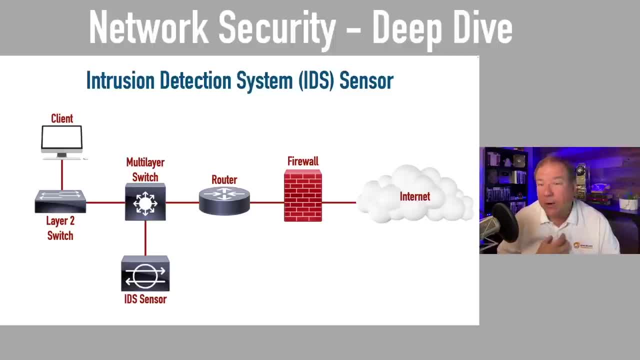 potentially malicious traffic coming in, it can alert us to that. In fact, some IDS sensors can even go out and speak to the front end of the IDS sensor and say you know what? I'm going to the firewall and say, hey, we're being attacked from this network or from this IP address. I want. 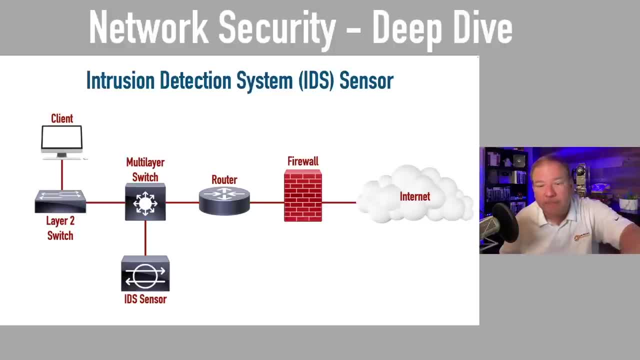 you to create a rule that says block that IP address from coming in. But notice the packet. originally that might've been a malicious packet that originally came in. it did make it to the client. There are some attacks- they're called atomic attacks- where an attacker can do damage. 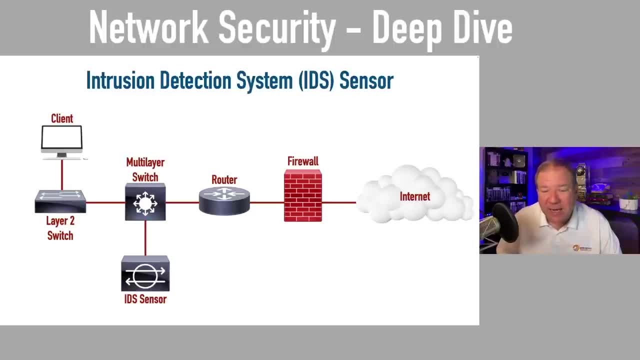 to a system with just one or two packets. In a case like that, the IDS sensor might realize we were attacked, But we weren't preventing the attack. To overcome that issue, what we can do is use a different type of sensor called an IPS sensor, And an IPS sensor is an intrusion. 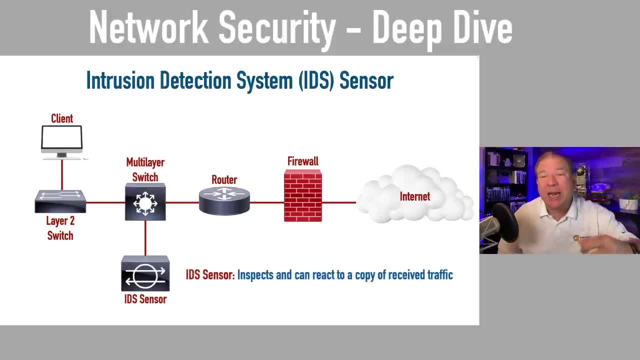 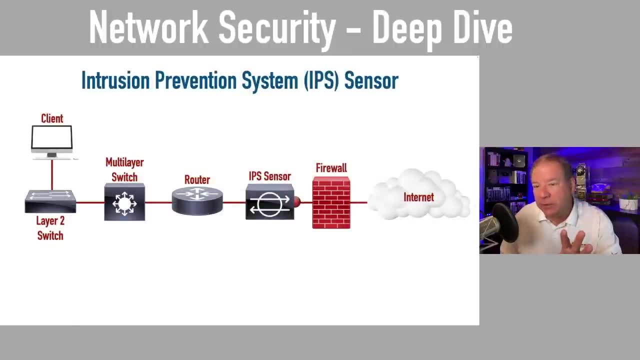 prevention system sensor. So again an IDS: it inspects traffic and it can react to a copy of the received traffic, But an intrusion prevention system sensor. it's going to sit in line with the traffic So when that traffic comes in from the internet, if it detects that there's an attack. 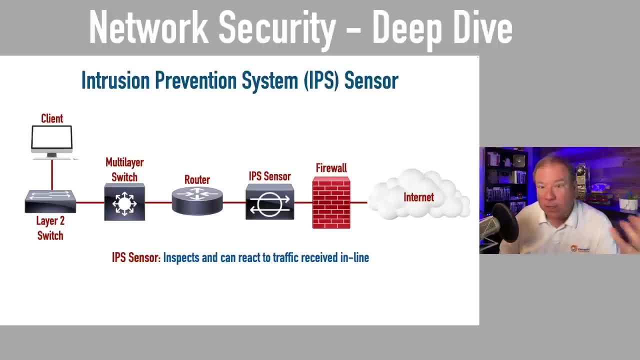 based on its signature database that this is malicious traffic. it's going to be able to react and potentially drop that traffic in line. It takes a look at that and says, oh, you match this well-known attack type in my signature database. As a result, I'm going to drop you. 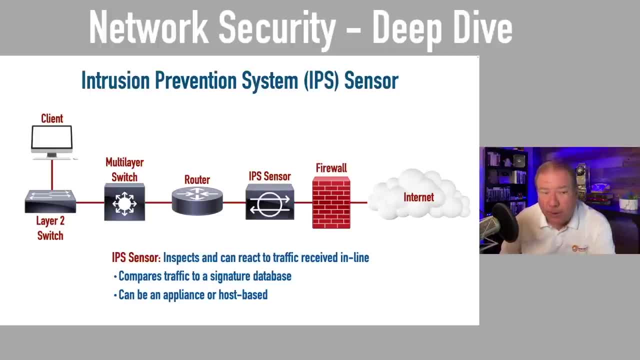 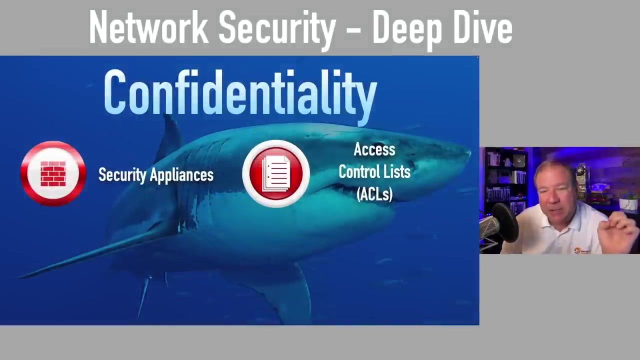 And sometimes, just like we can have a host-based firewall, sometimes we can have a host-based IPS system, an IPS sensor, where we can, on our host, block traffic coming in our network interface card before it can ever do any damage to our system. So that's the distinction between an IPS and an IDS sensor. So firewalls, IDS sensors. 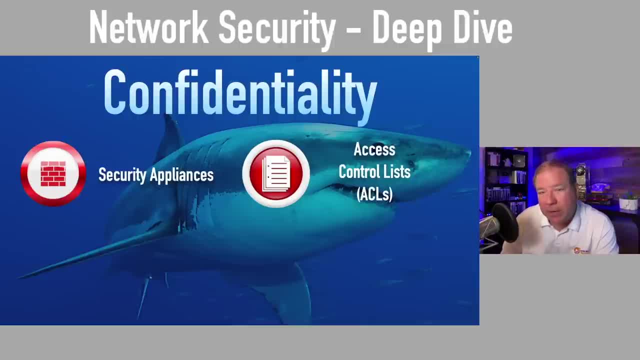 IPS sensors. those are some of the security appliances that we might use. Another line of defense is an access control list or an ACL. If you've gone through your CCNA studies, or perhaps Encore studies, then you've probably heard of the CCNA studies. And if you've gone through your CCNA studies, 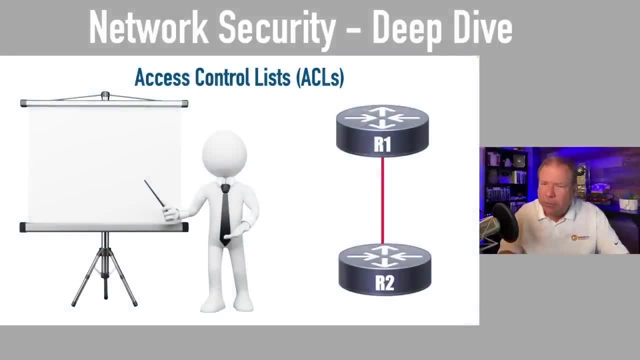 or perhaps Encore studies, then you've probably heard of the CCNA studies or perhaps Encore studies learned about these access control lists. Let's do a bit of review. To begin with, a lot of people think that an access control list is basically a traffic cop holding up a go sign or a stop sign. 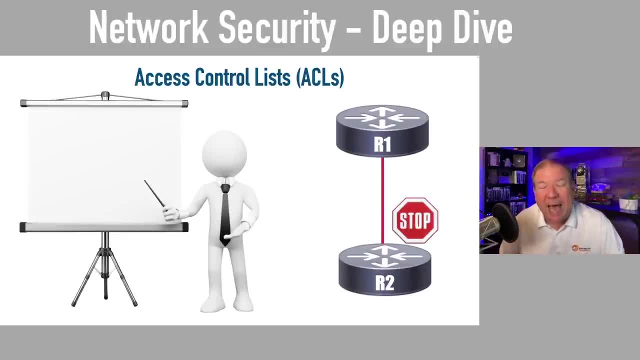 based on traffic coming into a router interface or going out of a router interface, And that's true, It can do that. An access control list? it's a list of rules. Each rule is called an ACE, an ACE, an access control entry, And that ACE is going to be able to say: yes, permit this or 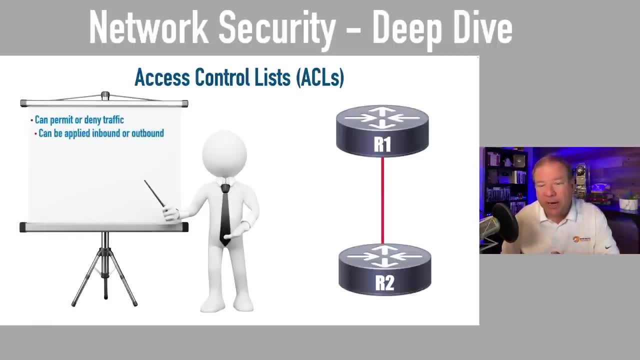 deny this And, in addition to permitting or denying traffic, I want you to understand that it can be applied as we send traffic into a router or as traffic is going to exit a router. We can apply it inbound or outbound. So when we're setting up these access control entries as part of our 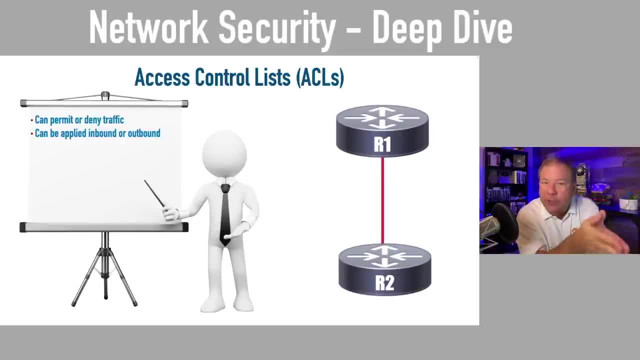 access control list. we need to think about in which direction is the traffic coming? Is it coming inbound, Is it coming outbound? Is it coming outbound? Is it coming outbound, Is it going into the router or is it going out of the router? And in addition to just permitting or 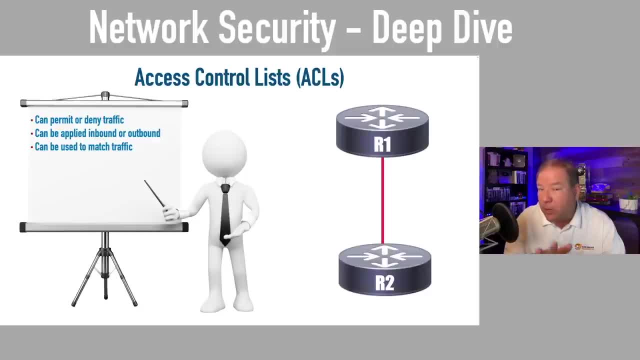 denying traffic. we can also use- and this is a concept often overlooked- we can also match traffic. If I'm doing something like a quality of service or a network address translation, I might want to match traffic that's coming from a certain subnet. I could do that with an access. 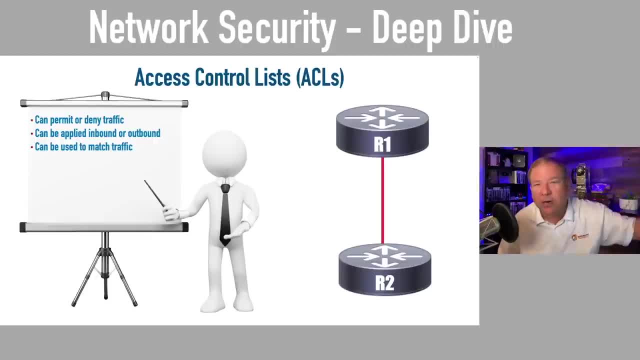 control list. And to do that, I would say I want to permit this network address with this wildcard mask. Well, just because I'm permitting, that doesn't mean I'm blocking everything else In the context of using this with quality of service or as network address. 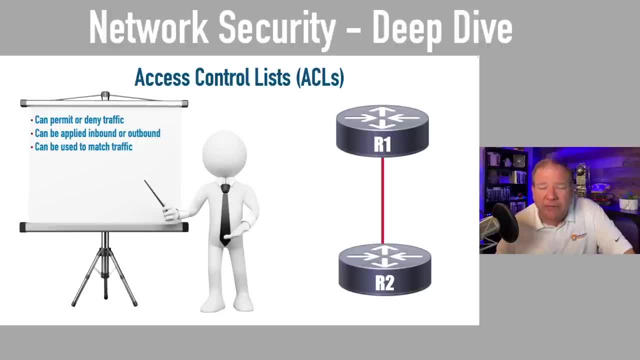 translation. I'm using it to match traffic, So it's not always used to block or drop traffic or let traffic through. It can be used to match traffic And it's a list and it's processed top down. Let me give you an example. Let's say that I've got a rule that says: 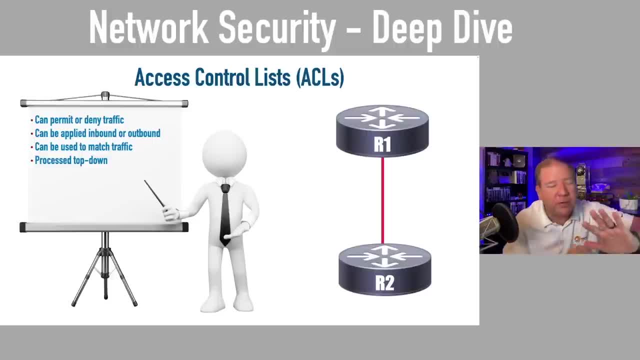 everybody in this subnet is prevented. They're denied access to this particular corporate server because of the sensitive information on that server. So nobody in this subnet gets access to the server, with one exception. We've got a network administrator that lives in that subnet. 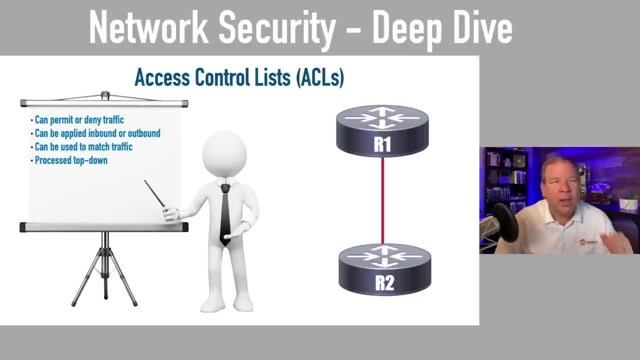 What we can do is set up a rule to say, well, I want to allow that network administrator's IP address to reach that system, to reach that server. Well, in my list, if I first say deny the subnet and then I say permit that one network administrator who belongs to the subnet, 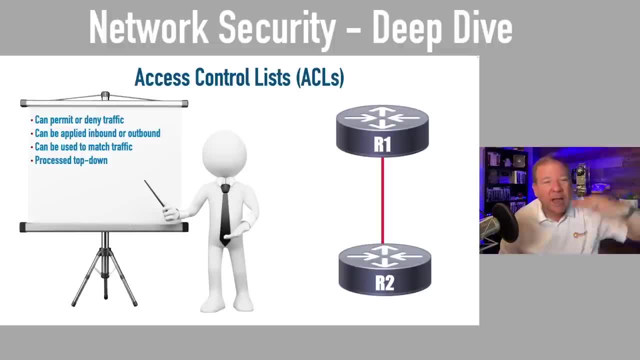 they're going to be denied because we're processing top down. As soon as we look at and evaluate that first ACE that says deny the entire subnet. well, the administrator is part of the subnet. Ding, ding, ding, we've got a match And that administrator's traffic is going to be dropped. 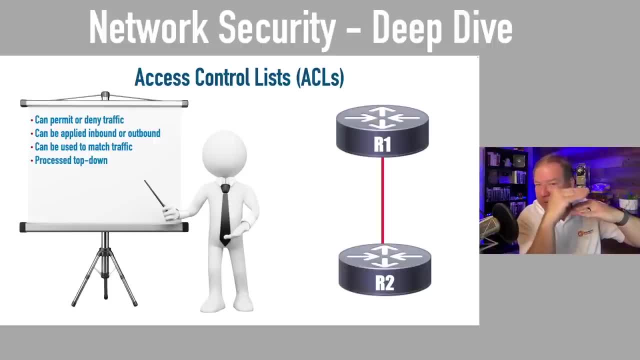 So we need to move their entry that says permit that specific network admin user. We need to move them above the subnet. So we're going to have to do that. So we're going to have to do that, So we're going to have to get a line that says deny the subnet traffic. So, as a general principle, 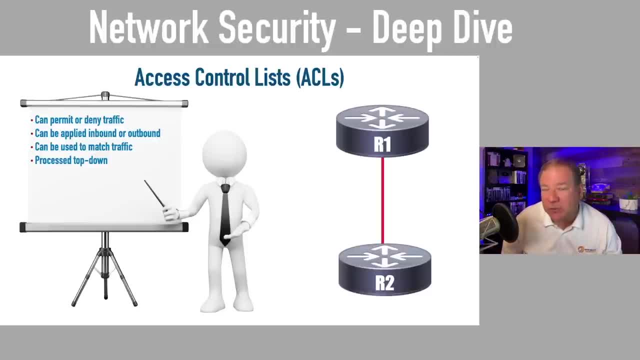 we should put more specific entries in our access control list higher in our list, because these are processed top down And then, once we have a match, we're going to ignore the rest of the entries in that list. But let's say that we go all the way through the list and we don't have a match. 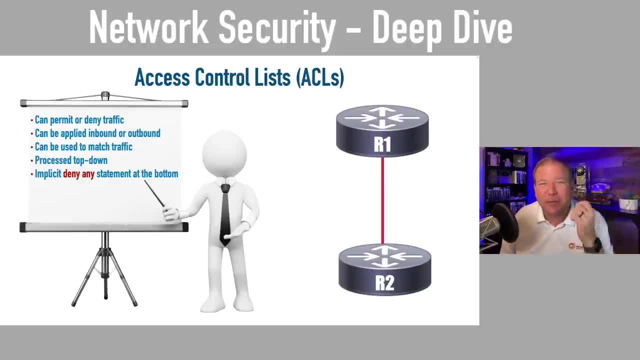 nothing. We didn't have a single access control entry that matched a particular packet. What happens in a case like that? Well, at the bottom of our access control list, of every access control list. We don't create this, It's there by default. We cannot. 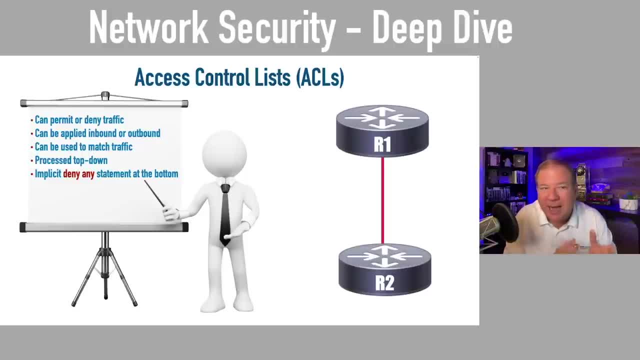 delete this. There's an implicit deny everything rule that says if it was not permitted by a previous access control entry, it's going to be implicitly denied. So we need to keep that in mind And when we're setting these up. you can use numbered ACLs. You can use named ACLs Personally. 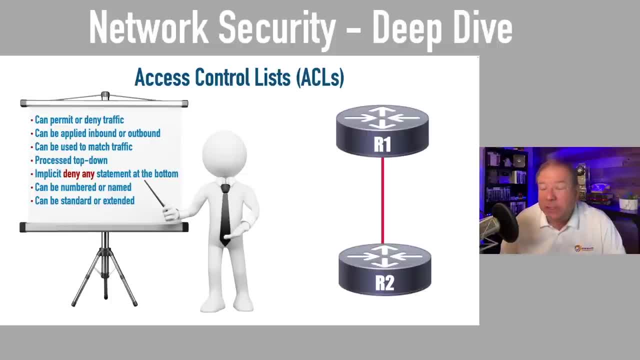 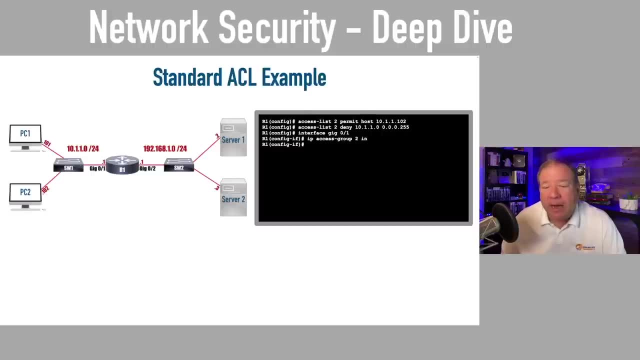 I'm a kind of a fan of the named ACLs, And they can be standard or extended, And I'll give you an example of each coming up in just a moment. In fact, let's go ahead and take a look at a standard ACL right now. Here I've got a couple of subnets off this router- PC1, PC2, they belong. 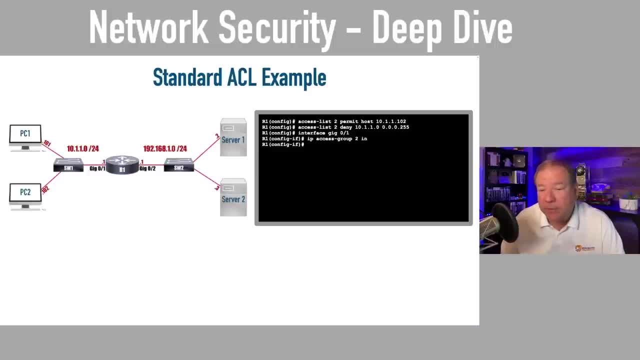 to the 10.1.1.0 slash 24 subnet. Got a couple of servers, 192.168.1.0- slash 24.. And the goal for our ACL here is: I want to prevent traffic from PC1 from reaching the subnet that contains. 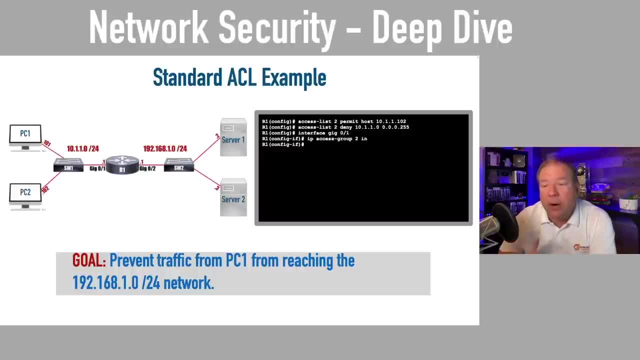 the servers. So in other words, PC2 should be allowed And notice what we're doing. First I say, if you'll notice the configuration syntax on screen, I'm saying access hyphen list 2.. Now numbers in the range of 1 through 99,. 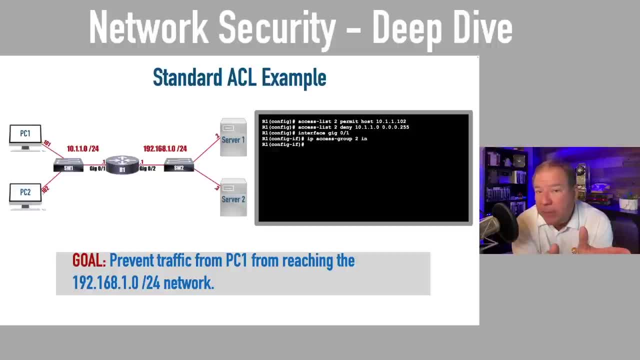 those are going to be used for our standard ACLs- Now a standard ACL. by the way, that's only going to match the source IP address, not a source TCP port number, not a destination address. It's only matching the source IP address, That's it. So it's not. 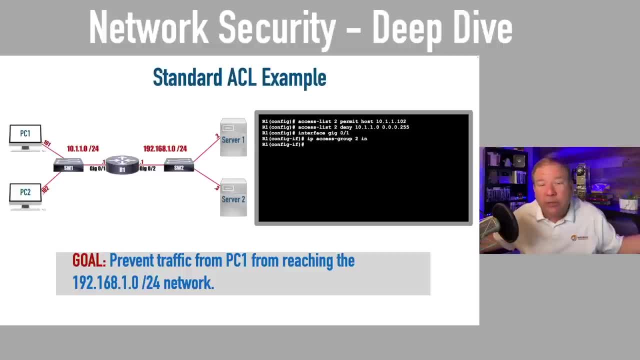 it's granular Still. I probably will use a standard ACL every time when I'm setting up NAT, because I'm trying to match addresses that are sourced from a subnet. So I don't need something else. But here I'm saying I want to permit the host of 10.1.1.102.. That's PC2.. Then I follow. 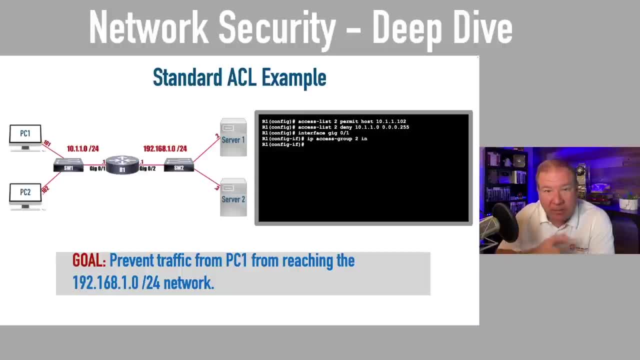 that up with the next ACE, which is access hyphen list 2.. Notice, I'm giving the same number, It's part of the same list. I'm saying I want to deny that entire subnet. It contains PCs 1 and 2, 10.1.1.0.. And instead of a subnet mask we give the reciprocal of that. 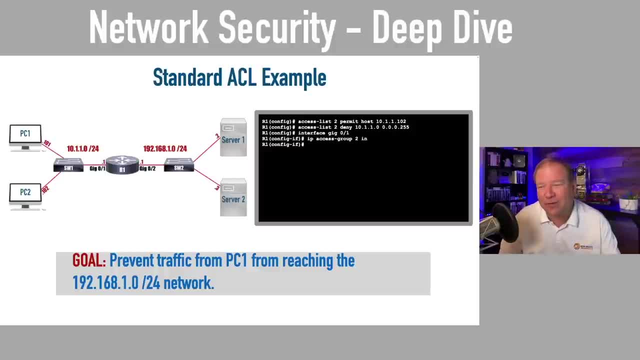 the wildcard mask and that's going to be 0.0.0.255.. Would I necessarily had to have given that second access control list entry? Actually, no, It's denying traffic. Well, if traffic is not implicitly- or I should say explicitly- permitted, it's going to be implicitly denied. So I could. 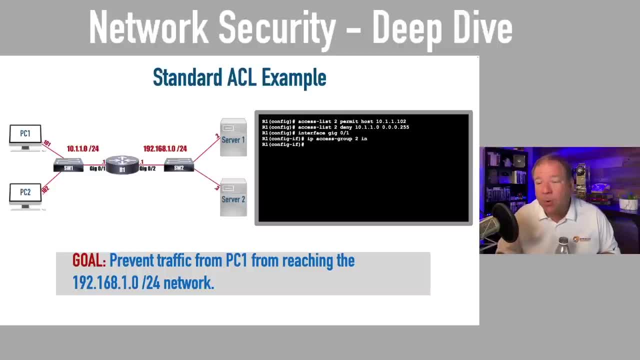 have omitted that second rule and it would have been just fine. Now we're going to apply it. We're going in to interface gig 0, slash 1.. That's the interface facing the PCs And we say IP access, hyphen group, And we give the group number of 2 or the list number of 2. And we say in So as: 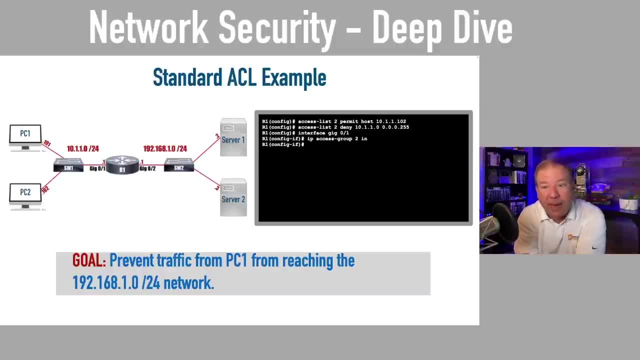 traffic is going into that router. that's where we're going to evaluate the packets And that's going to meet our goal. Let's take a look at an extended ACL. Here, the goal is for PC2.0.1.0.0.. 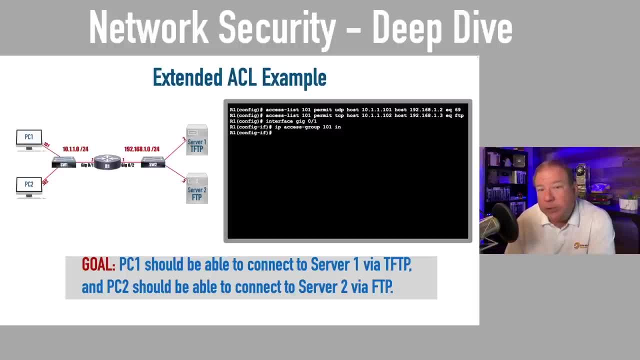 PC1 to be able to connect to server 1 using TFTP, the trivial file transfer protocol. PC2 should be able to connect to server 2 using FTP, And I'm guessing that everything else is going to be denied. Let's take a look at our entries: Access list 101.. So, starting at 100 through 199, those 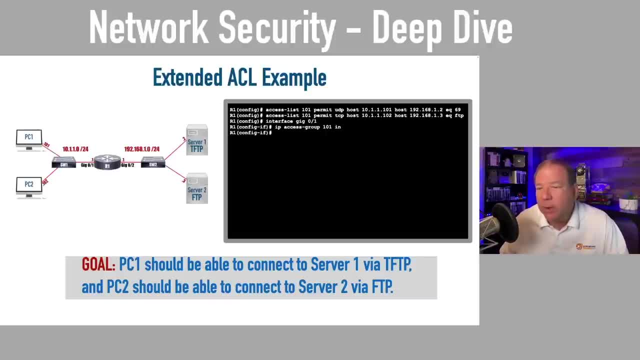 can be used for extended ACL numbers. So access list 101, permit. And here I don't have to match an entire subnet or an entire not a subnet, but match an entire protocol suite. like IP, I can match particular protocols. Here I'm going to match trivial file transfer protocol, That's UDP. 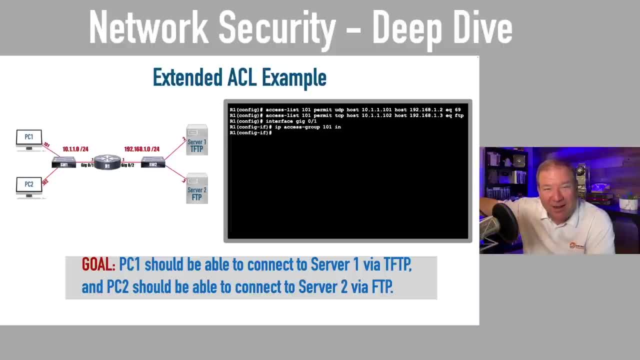 based. So I say: permit UDP. And later on in this line you'll see that I specify the UDP port number. But I wanted to permit the host of 10.1.1.101, that's PC1, to go to a destination. 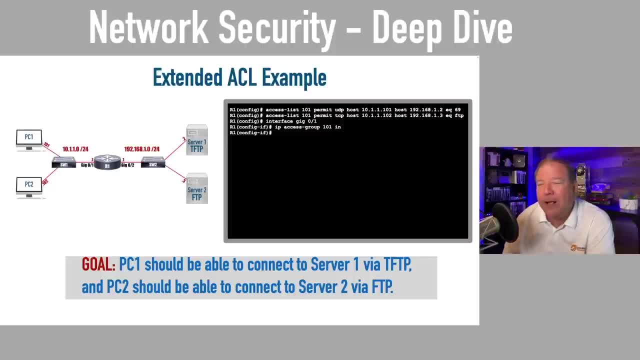 We couldn't specify a destination, So standard ACLs. but we can't here. We're going to go to a destination of 192.168.1.2.. That's going to be server 1.. And then we say EQ69.. That is equaling UDP port 69.. That is TFTP. 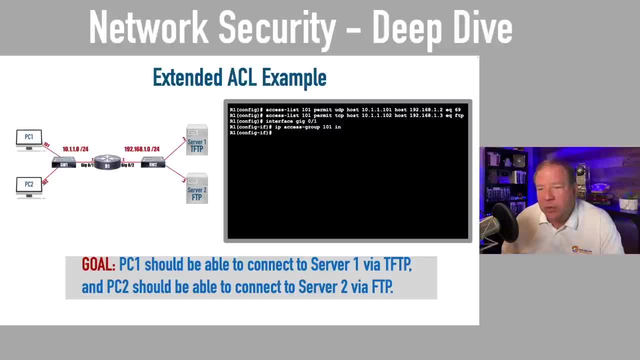 We do something similar in the next line. We say: access list 101, permit TCP. this time for FTP from the host is PC2 and the destination is server 2.. And we say EQ FTP, And I did this to illustrate that sometimes we can specify an individual port. 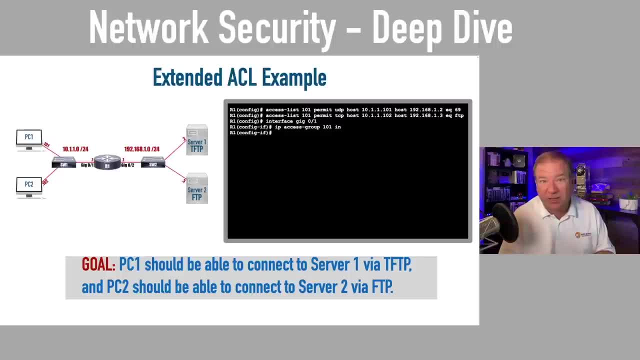 number. but Cisco IOS knows about the names of a wide variety of protocols. Check it out sometime with context sensitive help. So I don't necessarily have to give a port number. I can give a protocol name like FTP, And I did not say deny anything else. 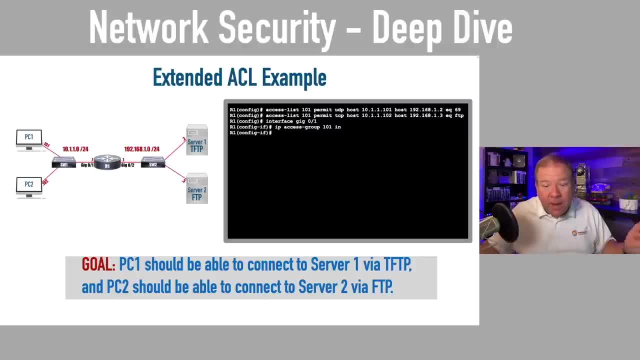 even though I said everything else should be denied. Do you remember why? The reason was: everything else is going to be implicated. If I don't explicitly permit it, then I go into interface gig 0, slash 1 and I say IP access hyphen. 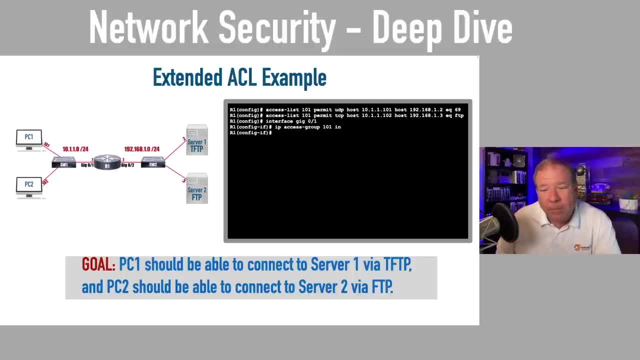 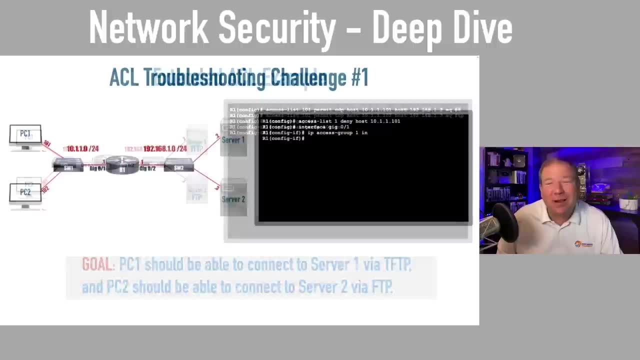 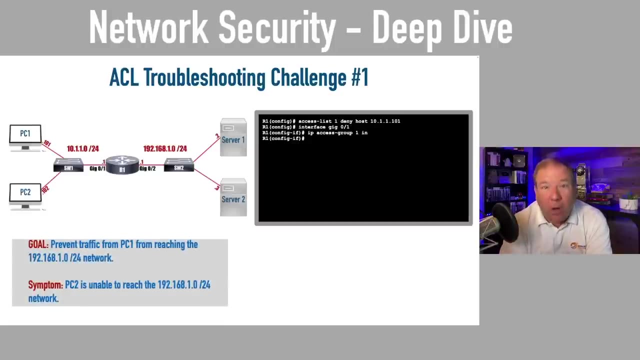 group N. So I'm- I'm specifying coming into router R1 from the subnet containing the PCs. Now let me challenge you with a few examples. here You see the syntax currently on router R1 and the goal is to prevent traffic from PC1 from reaching the subnet containing the servers. 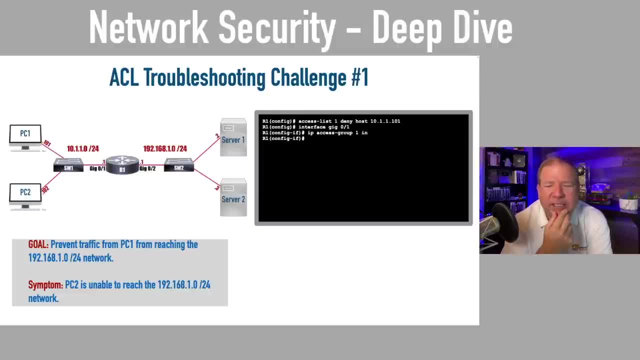 But the symptom we're having huh Curious. PC2 is unable to reach the 192.168.1.0 slash 24 network. So PC1 should be denied, but the symptom is both PC1 and PC2 are denied, In fact. 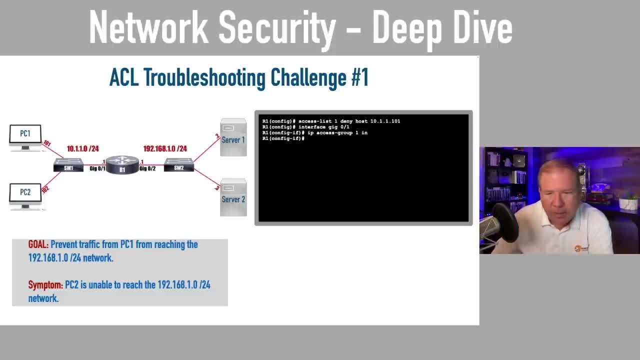 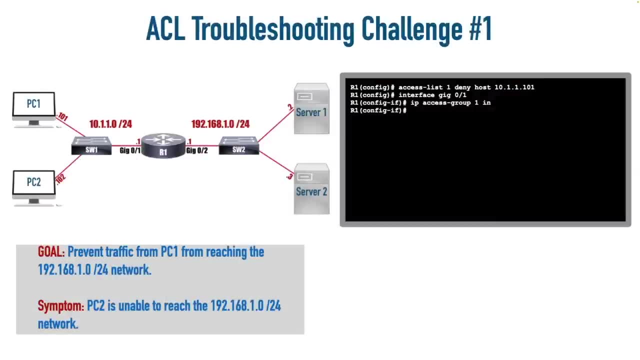 so you can see the syntax a bit better. I'm going to make this full screen for you. That'll let you get a better look at it, And I'd like you to to tell me in the chat if you would, and we have chats coming in on different. 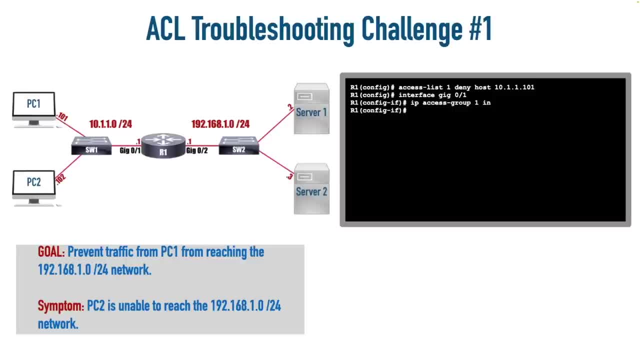 interfaces here. So, uh, I need to be looking around at more than one interface. but uh, and by the way, there's a delay from the time I speak something to the time you hear it. there can be a 15 second delay, So I'll try not to drag it on too long, but I want you to go ahead and chat in. 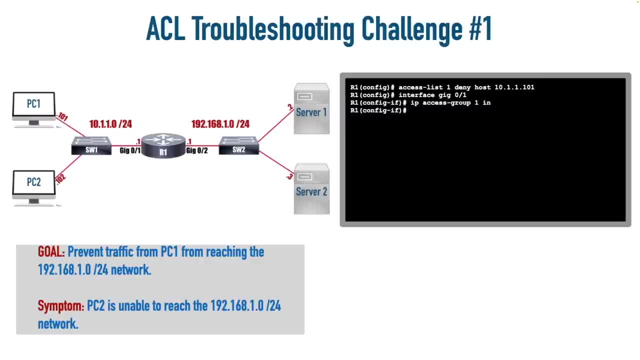 If you would. what's wrong with this? What's wrong with this syntax on screen? I'll give you a few seconds and you can chat it in when you spot the issue. All right, Starting to get some responses coming in, Let's go through it here. 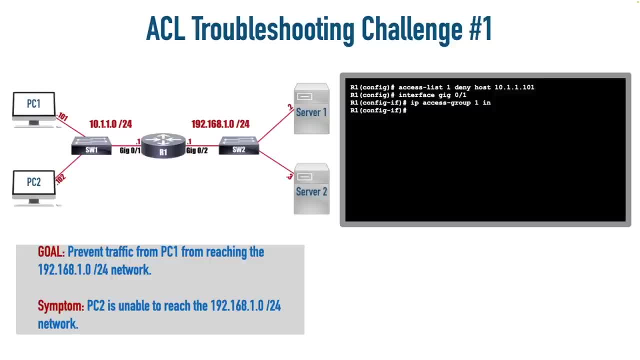 First it says access list: one deny host 10.1.101 or 10.1.101.. That's PC1.. We're denying all traffic from PC1.. That's that's what we want to do, Awesome. Then we're going into interface gig. 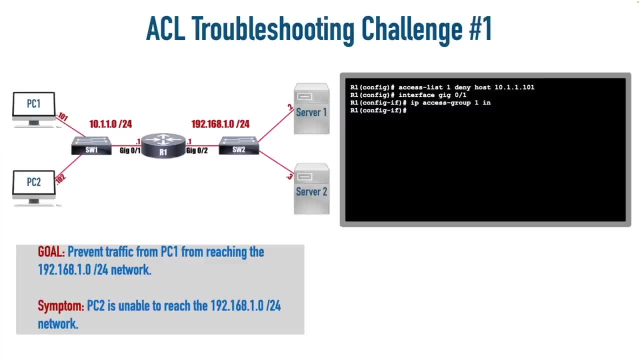 zero slash one and we're saying: block traffic coming into this interface that matched access list one which is blocking PC1. It seems like we're doing what we were told to do. How come it's not working? And yeah, so many of you are getting this right. It's. 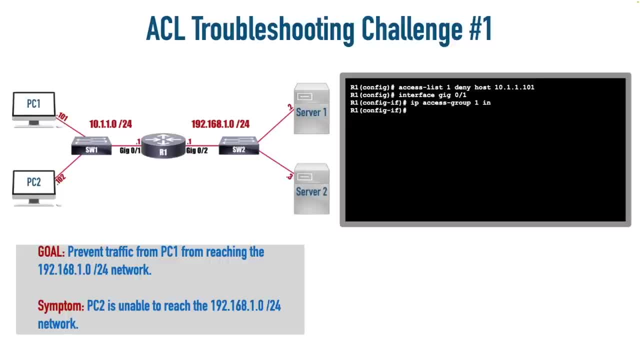 it's that implicit deny down at the bottom. I wanted to permit PC2 to get to that subnet and it's not. it's because that implicit deny anything down at the bottom of our ACL. Awesome work on that one. Let's take a look at another one. In this example, traffic from 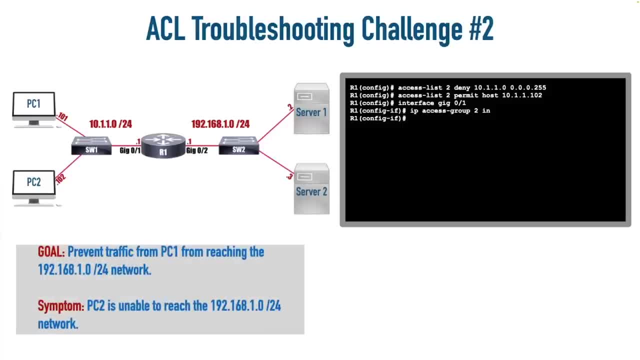 in fact it's the same goal and the same symptom. PC1 should be prevented from reaching the server subnet. PC2 is unable to reach it as well, And we didn't want that. We want PC2 to be able to get there And, if you'll notice, in the syntax I did what you said. You said that we should. 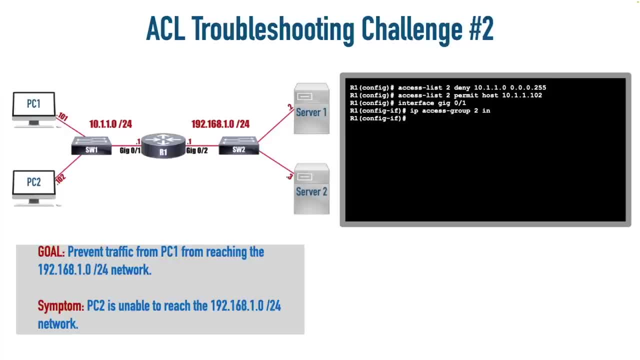 explicitly permit PC2.. So I did Check it out. It's that second line right there. I added a line that said permit host 10.1.1.102.. That's PC2.. So chat it in again if you would. How come that's? 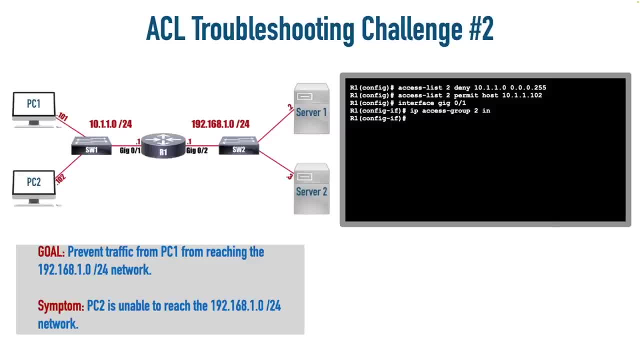 not working? Yeah, great job. It's because this is an access control list And this list is processed top down So that first ACE, which is denying the entire subnet of 10.1.1.0.24,, it matches both PC1 and PC2.. So before we explicitly say PC2,, 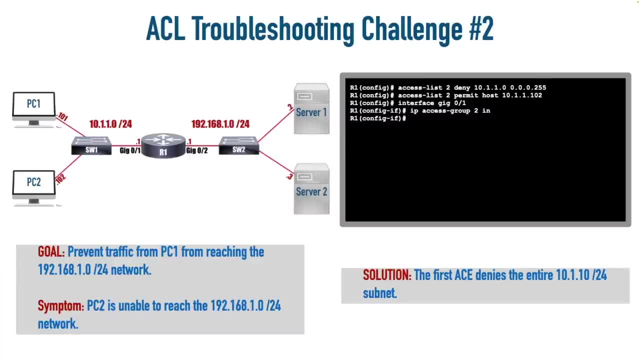 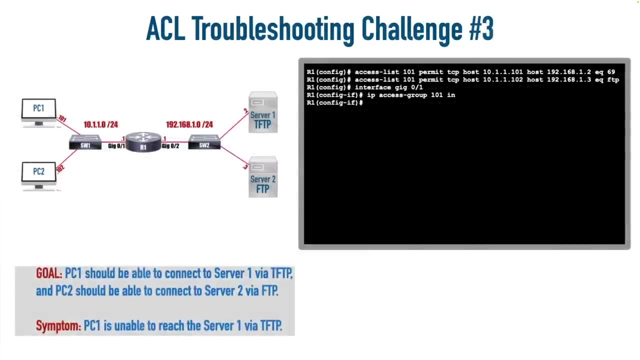 is allowed. we explicitly said: block the entire subnet that PC2 belongs to. So because we were processing top down, we never got to the rule permitting PC2. And therefore it was blocked. All right, let's move to an extended ACL, now A little bit more challenging. Here's the goal. 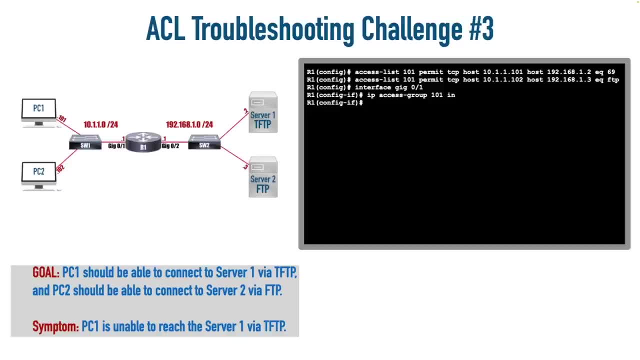 PC1 should be able to connect to server 1 using TFTP. PC2 should be able to connect to server 2 using FTP, And PC2 is fine. It's working just fine- But PC1 is not. PC1 should be able to reach the server via TFTP. This is kind of like what we saw in our example a. 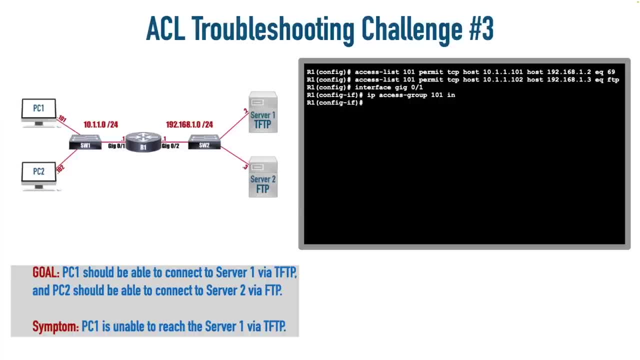 few moments ago. Again, I'll give you a few seconds to peruse the syntax and chat in your response. What is going wrong here? Yeah, this was a little trickier, wasn't it? In this example, everything looks really good, except we have to know that TFTP. 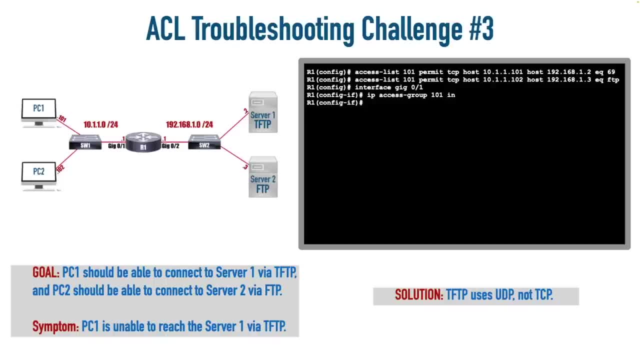 is a UDP protocol, It's not a TCP protocol. And remember that a standard ACL it's going to match an entire protocol suite like IP. But with an extended ACL we can match specific ports And a port is going to be typically either a TCP or a UDP port And here that first line says TCP. 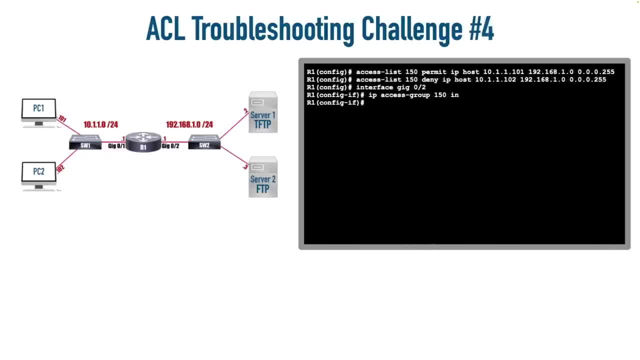 it should have said: UDP. You guys are doing awesome. Let's do one more. Here we want to allow PC2 to connect to server 1 using TFTP. And here we want to allow PC2 to connect to server 1. 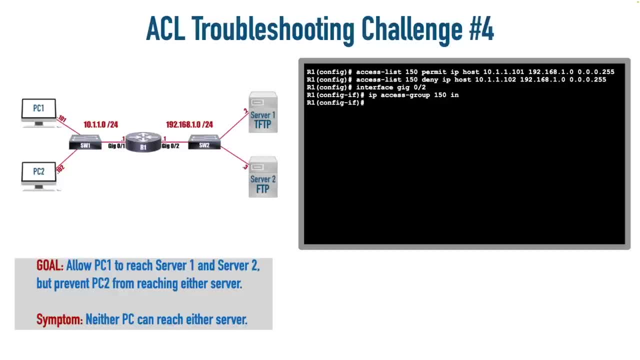 to reach server 1 and server 2.. And we want to prevent PC2 from reaching either server. So PC1, go to the servers, PC2, don't go to the servers. The symptom is neither PC can reach either server. 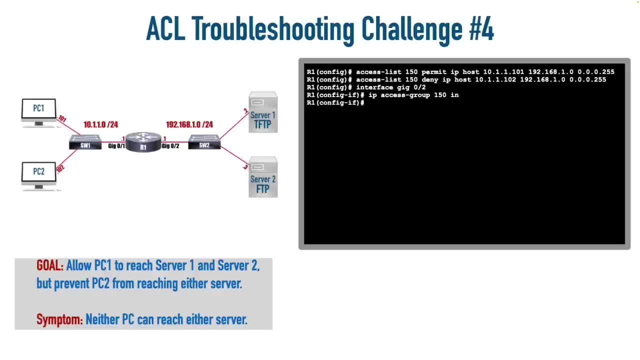 And let's take a look at the syntax here. It's an extended ACL access list 150, that's in that range of 100 through 199, permitting IP. So I'm permitting all IP traffic. TCP and UDP are included. 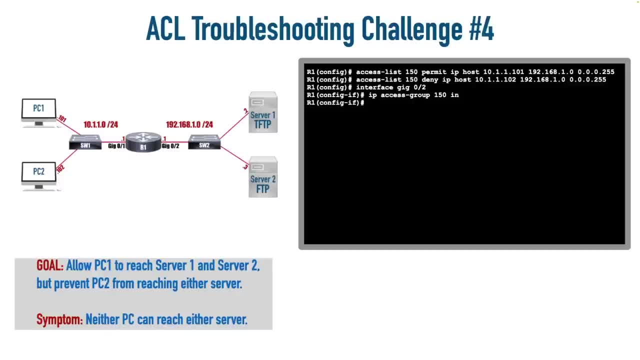 I'm saying: permit host 10.1.1.101, that's PC1, to go to that subnet containing the servers 192.168.1.0 with a wildcard mask of 0.0.0.255.. That looks right. Then I'm explicitly denying. 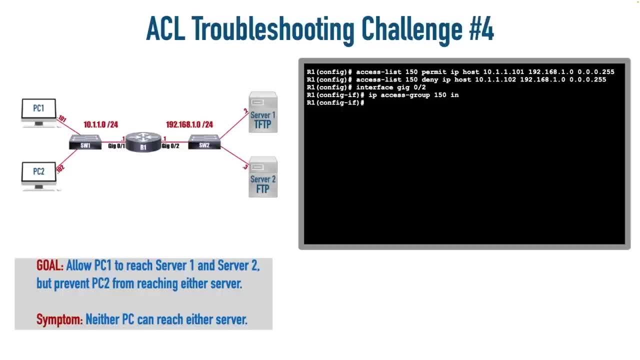 PC2.. I'm saying deny host 10.1.1.102, going to that same subnet. That looks right And you see I'm going in and I'm applying it. What's wrong here? This looks pretty good, but it's not working. Can anybody you know what? I don't even need. 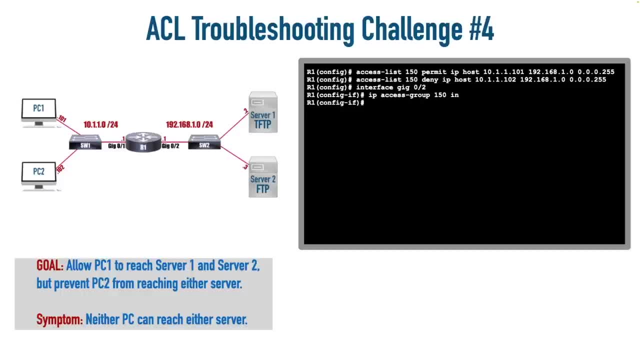 to pause here. Fantastic job. Lots of people are spotting that I've applied it to the wrong. well, actually, I've either applied it to the wrong interface. I can fix it that way. Notice I'm saying I want to apply this inbound coming into the router on gig 0.2. Well, 0.2, that's. 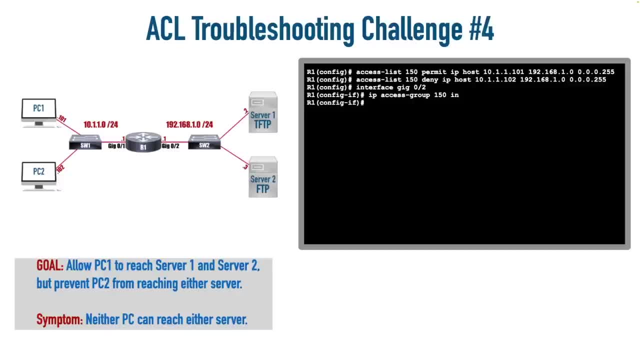 the port pointing out to my servers So I could apply it to gig 0.2.. That's an option, But if I did that I would have to apply it in the outbound direction as I exited router R1. So one fix would be to just change the direction, change the in to an out The other. 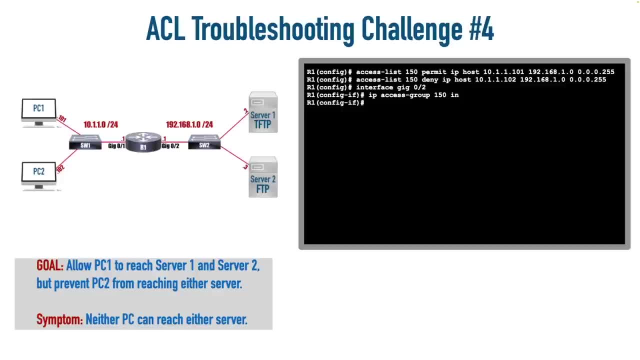 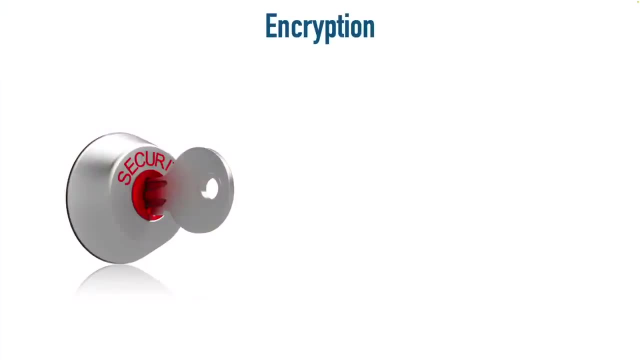 fix would be to change my interface to gig 0.1, because there I am coming in from the PC. So either one would have fixed that issue. So we need to apply the access list in the correct direction on the correct interface. Next up, let's talk about encryption. We said 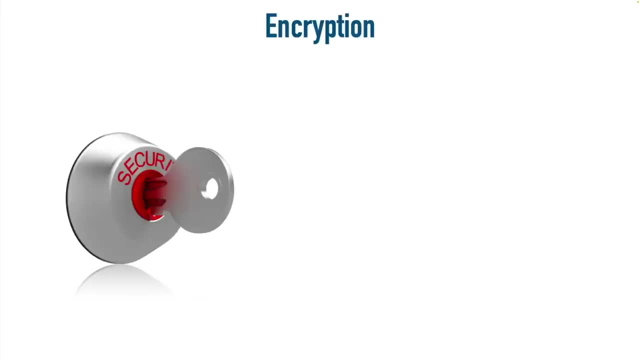 encryption is going to scramble our data up such that if somebody intercepts it, they're going to be able to read it. And we have two basic types of encryption: There is symmetric encryption and there is asymmetric encryption. Now symmetric encryption. 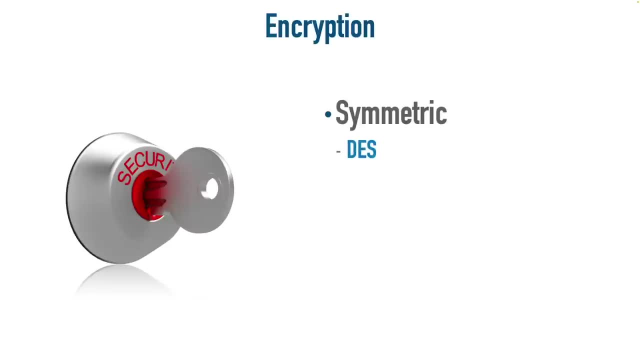 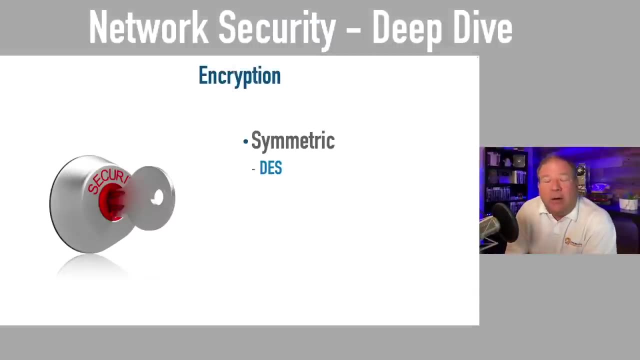 let me give you a few examples. A really old example that we definitely do not want to use today. In fact, let me put my face back on screen that we're not looking at our syntax anymore. One standard that we don't want to use today- it was developed back in the 1970s- is DES. 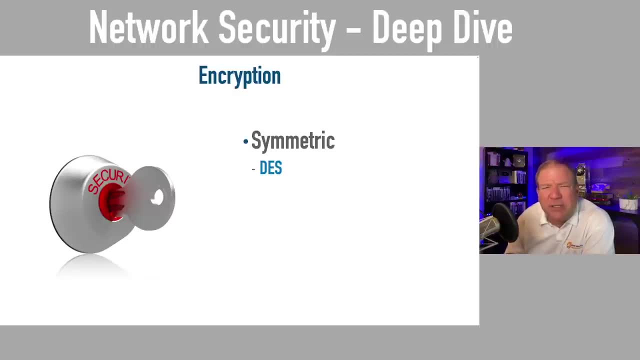 The Data Encryption Standard. It uses a 56-bit key length. There is actually hardware out there that you can build yourself or buy that will crack a DES encrypted string. You don't want to be using that Now. better than DES is Triple DES. they call it 3DES That uses three of those. 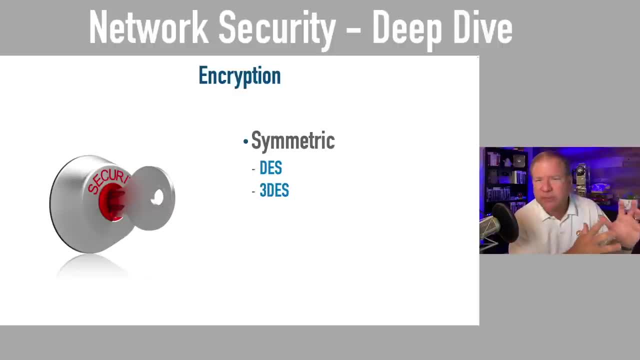 keys and there's different ways of implementing this. You can use 56 bits for one key. You can use 64.. There's different ways of implementing this. You can use 56 bits for one key. You can ways of doing it. You can combine keys together. Bottom line is: it's a lot better than DES. 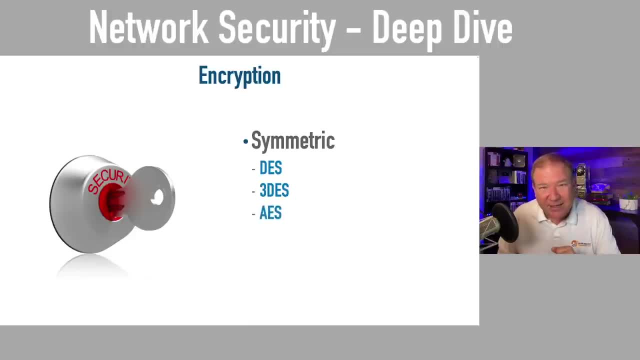 but you know what's better than triple DES, AES, the Advanced Encryption Standard, And that is really today the flagship symmetric encryption algorithm out there. We're going to see it on our wireless networks, We're going to see it in our IPsec VPN setups. 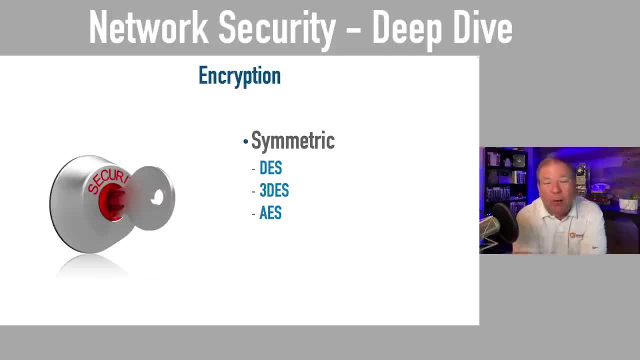 AES. that's probably what we want to be using today. Now, when I say symmetric encryption, that's where we have a shared key. In other words, we're sending data back and forth- you and I- and we want to encrypt the data that we're sending, So we each have this secret key. 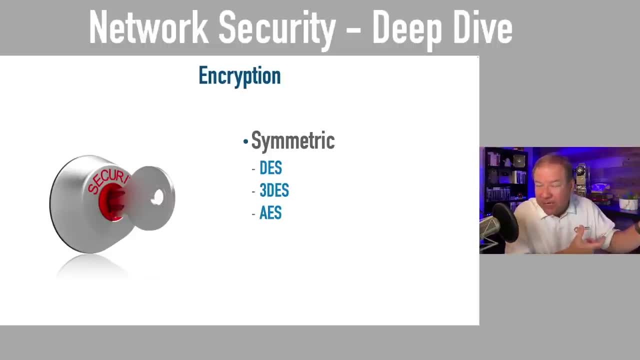 and we've got the same one. The key is symmetric. in other words, That means we both have the same key. This symmetric key is going to be used in the algorithm like AES that is going to encrypt our data, And if somebody were to intercept that data, they would not be able to interpret. 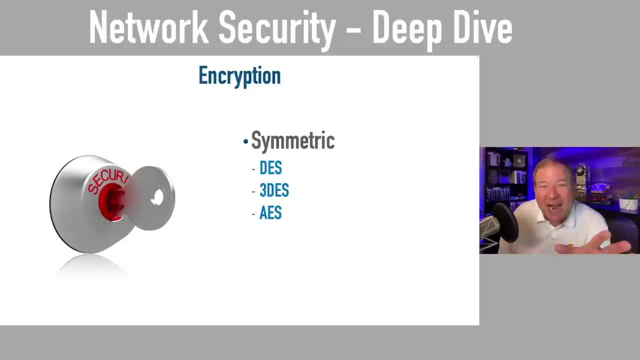 that data. They would not be able to encrypt that data. They would not be able to encrypt that data. They don't know our secret. They don't have our secret key. That's what gives us confidentiality through encryption. Another option is asymmetric encryption. Asymmetric encryption and by the 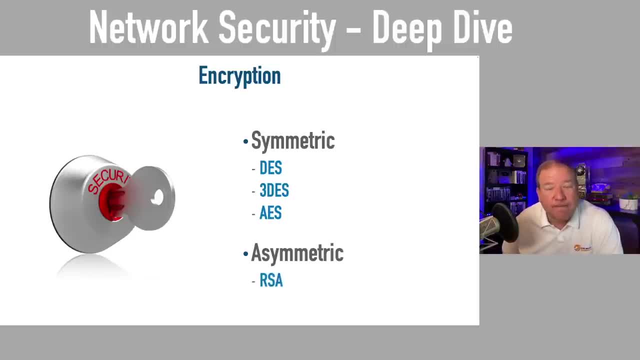 way. the standard out there for that that you'll run into is RSA. That stands for the people that developed it- Revest, Shamir and Adelman- But with asymmetric keys. we have keys that you and I use to communicate, but they're different. They're called a public-private key pair. 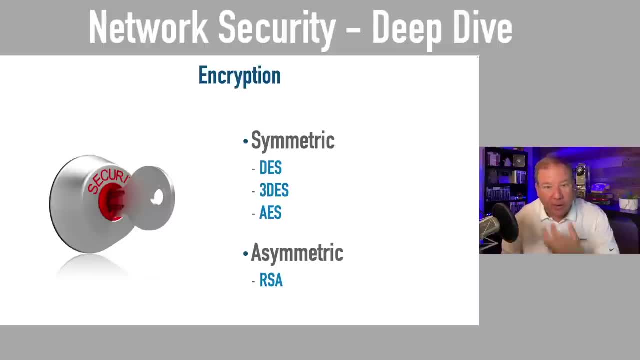 Here's the idea. If we want to communicate asynchronously or asymmetrically, I'm going to have a private key and I will give you my public key. Now, here's the way this works. You might want to put this in your notes If I encrypt something with my public key. 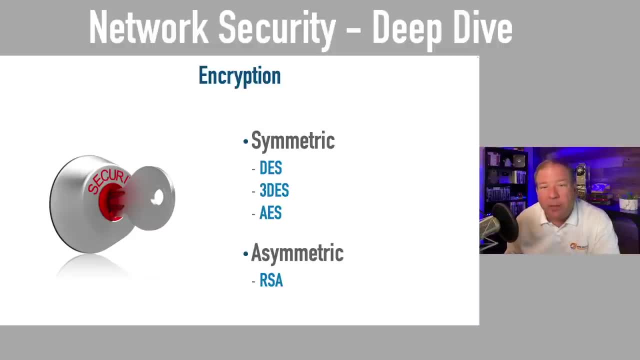 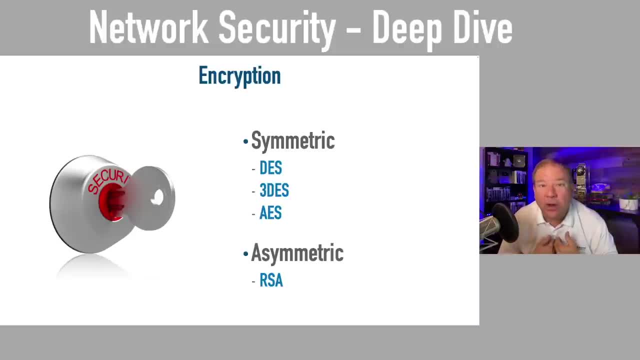 with the public key that I gave you. I'm the only one that can decrypt it, because I don't give my private key out to anybody. I will give my public key out to anybody that wants it. So let's say that I gave you my public key and I gave a bad actor, a malicious user, my public key. 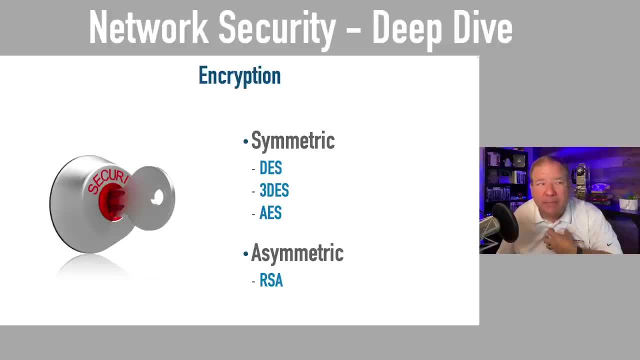 and you want to send some data to me confidentially. Well, you use my public key and I give you my public key and I give you my public key and I give you my public key. to scramble things up, What if that malicious user intercepted your traffic that you encrypted? 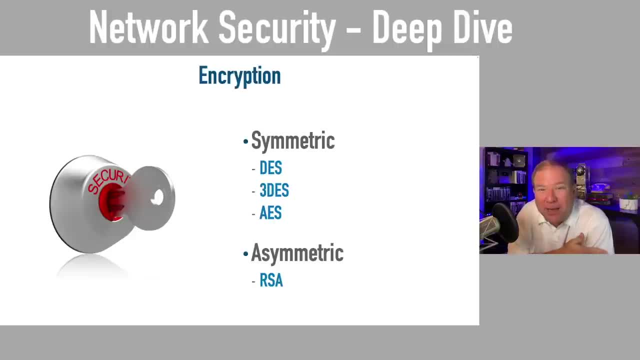 with the public key that I gave you. Well, they've got my public key too. Is that bad? Does that mean that, because they have the same key that you have, they can now decrypt the data? Well, that would be true with symmetric, but not with asymmetric. With asymmetric, anything encrypted with the 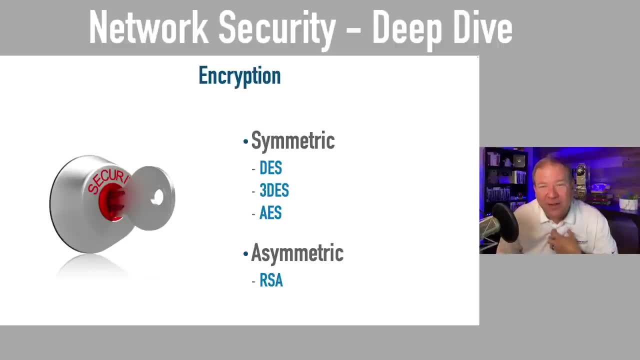 public key can only be decrypted with the private key, which only I have. So even if they intercept the traffic, they could not. they could not decipher it. And the reciprocal of that, though, is true as well: If something is encrypted with my private key, it can only be decrypted with. 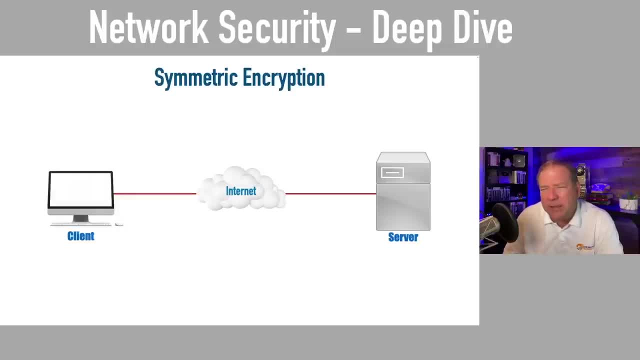 my public key. Let me give you some examples to make this more real world for us. Let's say that we're trying to communicate from a client to a server, or maybe a wireless access point to a wireless client would use this as well- perhaps Symmetric encryption? we've got a key that is. 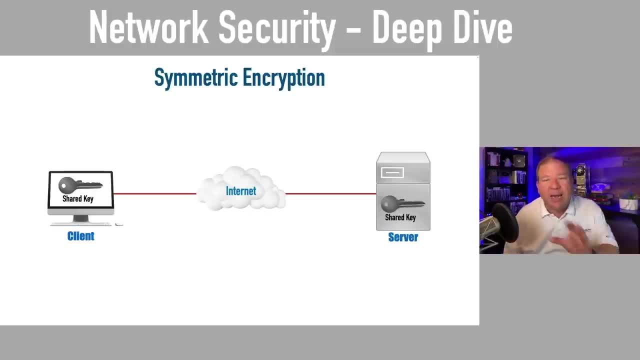 shared. We put it on the client, we put it on the server and, as they're sending data back and forth, the encryption algorithm we're running- whichever one it is- is going to use as part of that calculation. it's going to use that shared key And if somebody were to intercept that data, 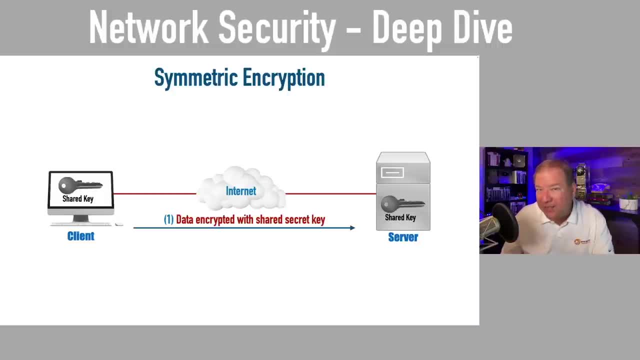 they would not be able to interpret it unless they also had the shared key. So we want to make sure this key is kept secret. But this really doesn't scale very well. does it Think about this If I had 5,000 users in the company and we gave everybody the same shared key? 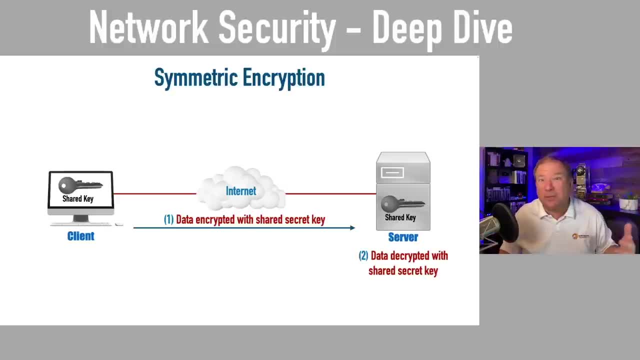 on their device. what if we had a disgruntled employee that left and they took their key with them and maybe they knew what key they configured on their PC? Suddenly we've got to go around and change the keys on all our thousands of devices. That's no fun. So this is not going to be something. 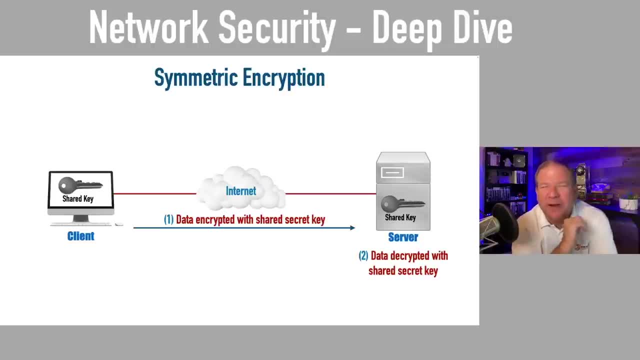 that we want to, that we can scale really large. if we have to go to every device individually and configure it with a key, Well, couldn't we just use asymmetric encryption? Yeah, here's the deal with that, something I didn't mention. 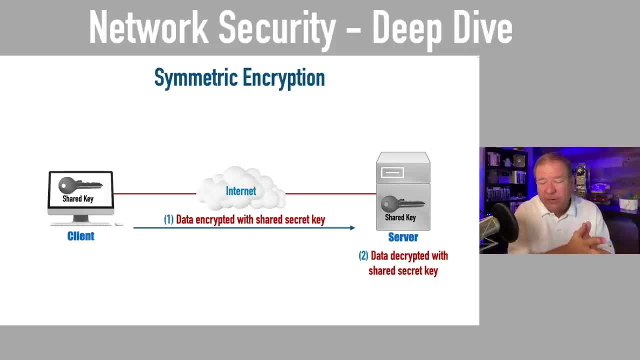 Asymmetric encryption is compared to symmetric. slow. I mean it's slow, Like I'm talking 100 times slower or it takes 100 times longer to do asymmetric encryption as compared to symmetric encryption. So asymmetric, we can scale that a bit better. 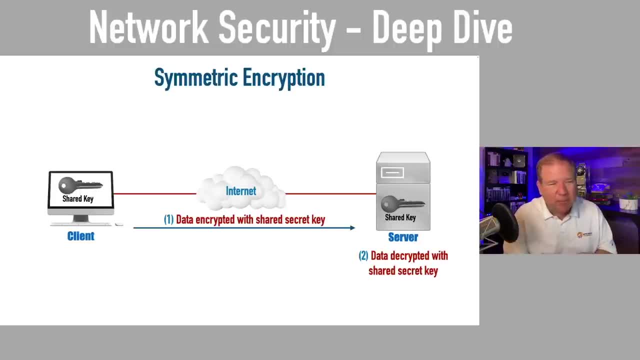 as we'll discuss. That's what we use on the internet oftentimes, but it's a lot slower than symmetric, So let's consider asymmetric. A common example: I buy stuff from Amazon almost on the daily. The Prime truck pulls up in my driveway very, very often In fact. 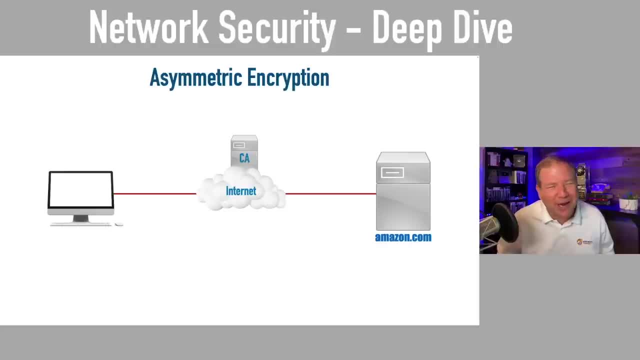 probably before class is over today. I'm probably going to have a delivery come. So if you're a doorbell, probably probably Amazon. But let's say that we're going to go out to Amazon and we want to purchase something and we're going to give our credit card information. 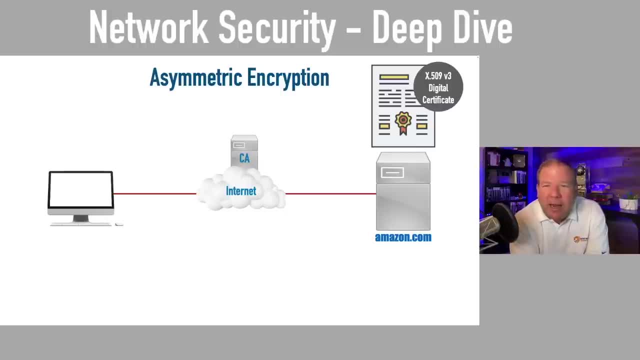 so, yes, I want it to be secure. Here's what Amazon has. They have something called a digital certificate And a digital certificate. technically it's probably going to be called an X.509 version, But this is something that proves that they're really Amazon. So when I'm sending them my 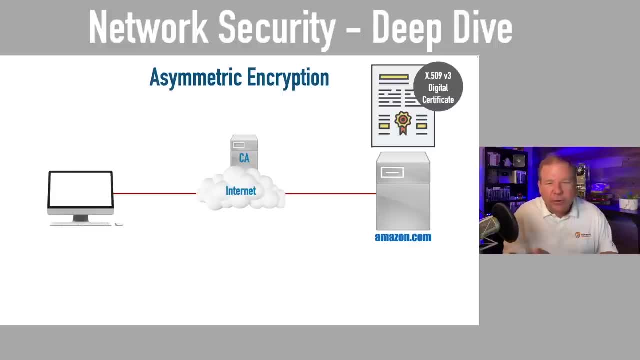 information. I know I'm truly talking to Amazon. Now you'll notice on screen. we also have this server, this entity on the internet, called a CA, And it depends on what literature you read. Sometimes a CA is said to stand for Certificate Authority or Certification Authority Bottom. 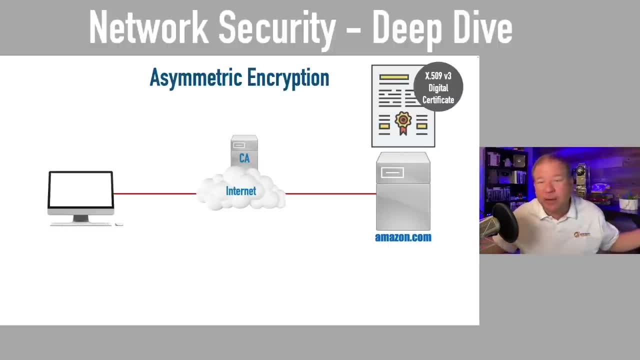 line is it's a trusted third party. The first company that comes to mind is Verisign. If Amazon wants to have this digital certificate to prove its identity to the internet, it can get with Verisign and say: hey, I want a digital certificate that you have approved, that you've. 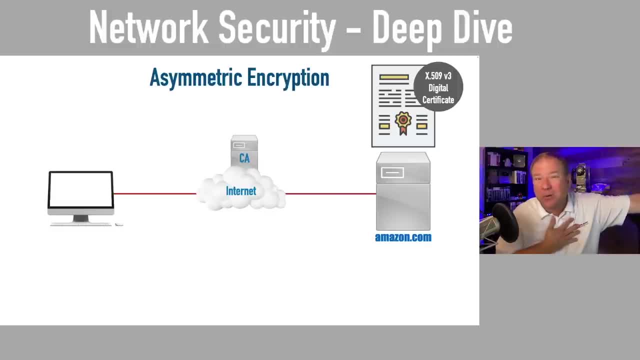 given me. So if I give it to somebody else- one of my customers- they're going to know what you really mean. So here's what happens. Verisign says: all right, Amazon, here is your digital certificate And here is your private key that I'm giving you. So we're using a key pair here. 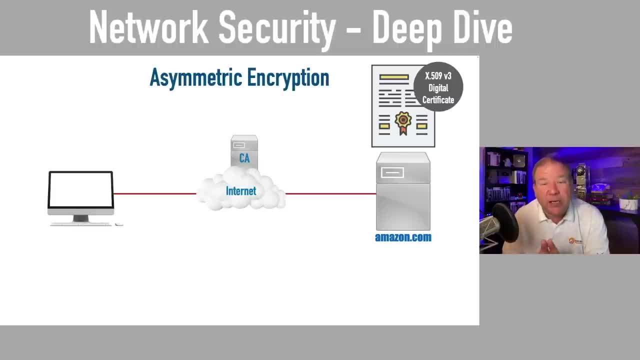 We're using the public-private key pair. Now, as part of that digital certificate, we have Amazon's public key. We'll freely give our public key out to whoever wants it, but we don't give out our private key. So Verisign says all. 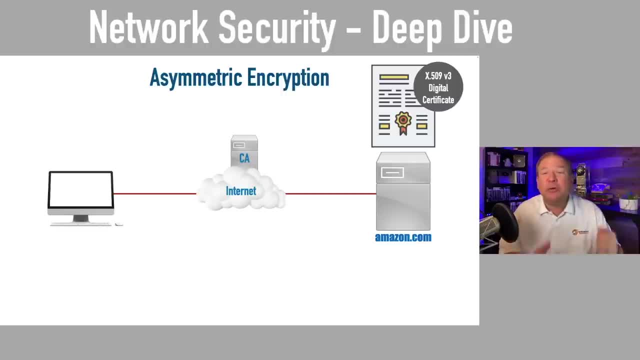 right. here's your private key. Don't tell anybody what it is. Here's your digital certificate containing your public key. Give that to your customers And then when I want to go buy something from Amazon, when you see the, depending on your browser, but if you see that little padlock icon. 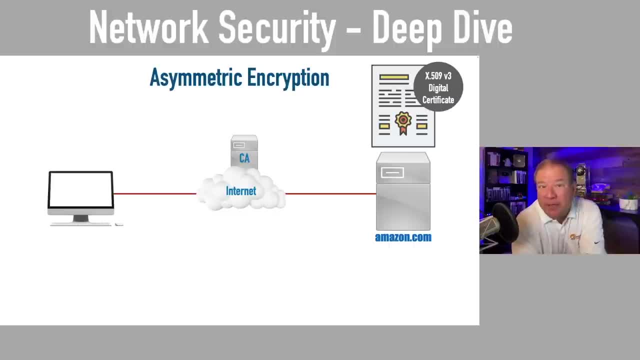 URL bar. that's saying that this data is encrypted or it's a secure communication. Here's what's happening. Amazon sends us their digital certificate. Their digital certificate contains their public key. The question is: how do I know this digital certificate that I just 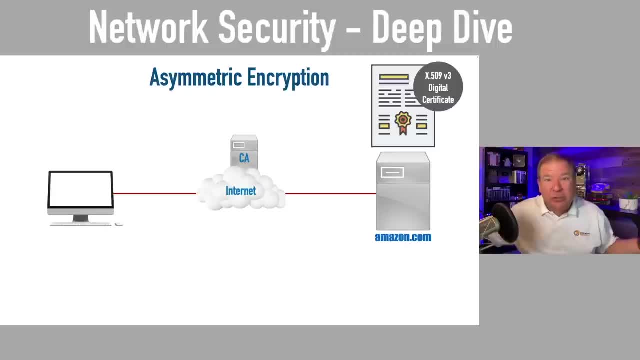 received is really from Amazon. I mean, there could be a malicious user out on the internet that that's pretending to be Amazon. that I got redirected to And they said: here's my proof, Here's my digital certificate. Well, the way I know it's really Amazon is that. 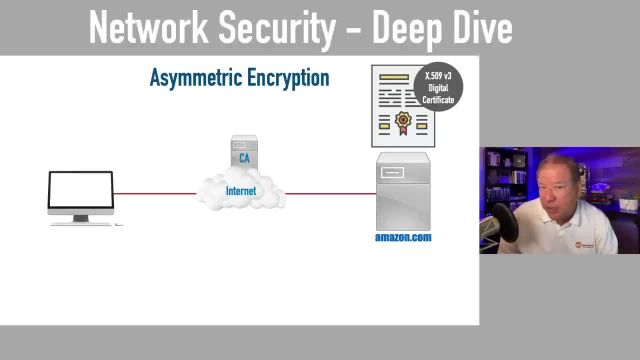 this certificate was signed by a trusted third party. In my example, I just picked Verisign. I don't know if Amazon uses Verisign or not, but Verisign has signed the digital certificate to say: I validate. this is really Amazon you're dealing with. What does it mean to sign a digital? 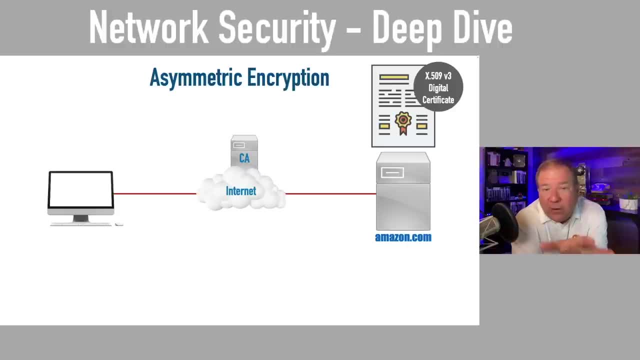 certificate. Well, the Verisign or the, they have encrypted that digital certificate with their private key. Remember the rule: if something is encrypted with somebody's private key, it can only be decrypted with their public key. And we have Verisign's public key. Let's go through this one step at a time, So Amazon. 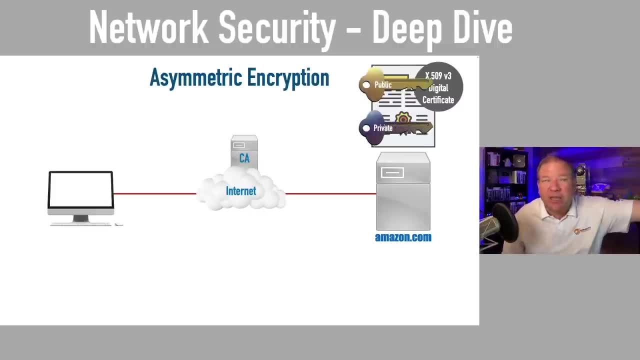 they've got a public and private key pair. Verisign has said: here's your private key. Don't tell anybody. Here's your public key, Put that in your certificate, give it to whoever you want. And they've got a public and private key pair. So, Amazon, they've got a public and private. 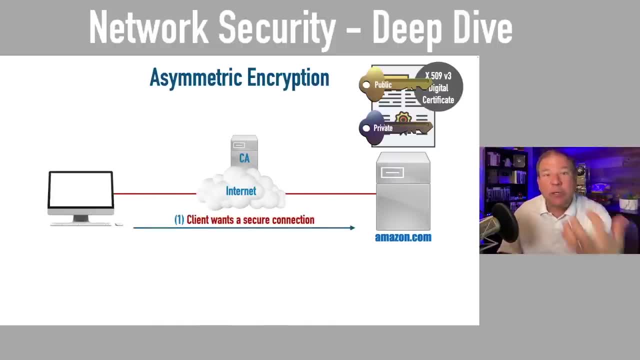 key pair. So I say I want to go to Amazon to buy something. So I say I want to establish a secure connection so I can send my credit card info. And Amazon says: okay, here is my digital certificate. And this digital certificate contains the public key of Amazon. I've highlighted it for. 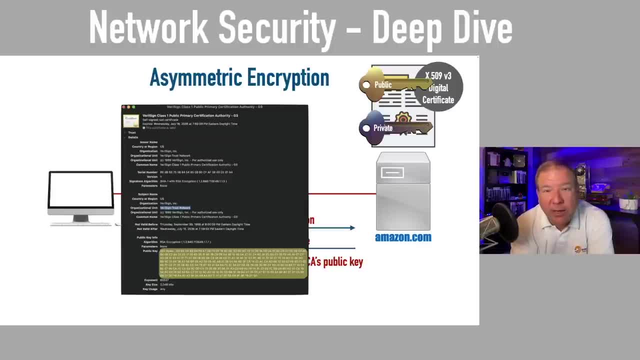 you here on screen. Now, how do I know this is really from Amazon? Well, notice, it says it's signed by Verisign And built into my browser. depending on what browser you use, I've got a few security settings And you can actually see the digital certificates from these trusted 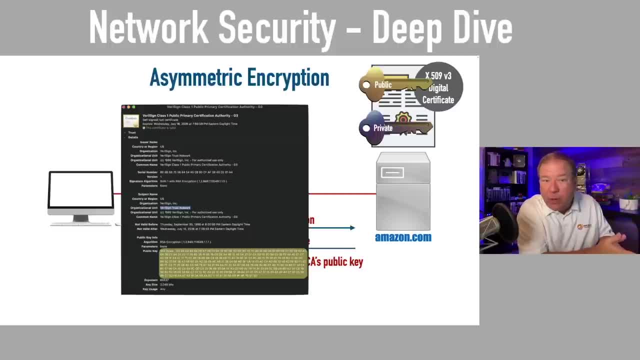 third parties like Verisign that are literally built into your browser. So you're given. when you install your browser, you're given the public key for Verisign, And Verisign has signed this certificate from Amazon. They've encrypted it with their private key. You've got Verisign's public. 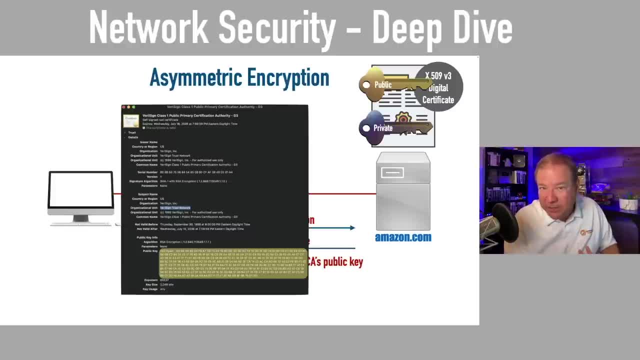 key. So if you can decrypt this certificate coming from Amazon, you realize based on Verisign's public key, you realize, oh yeah, this is really from Amazon, Because I used Verisign's public key to unlock it. 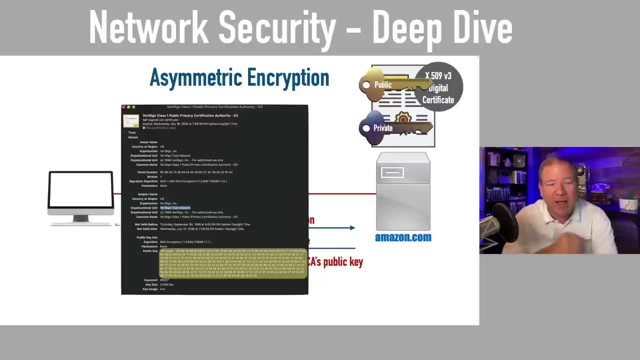 Because they locked it or they signed it with their private key. So now I know for a fact this really came from Amazon And I have Amazon's public key in my possession right now, But I don't want to use symmetric encryption. Like I said, it's slow. 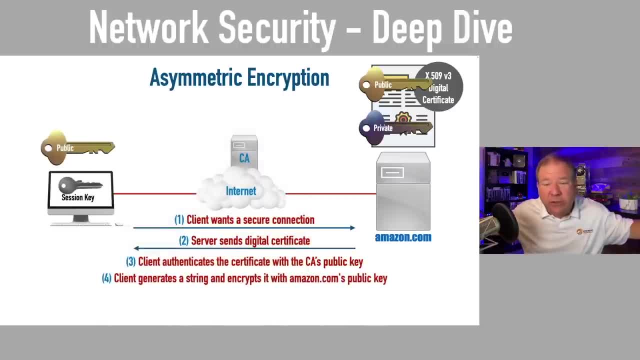 So let's set up a shared key just for the duration of this session. What I'm going to do is I'm going to generate- my PC is going to generate- some big string, Some big random string, And I want to use that as the symmetric key that Amazon and I will use. 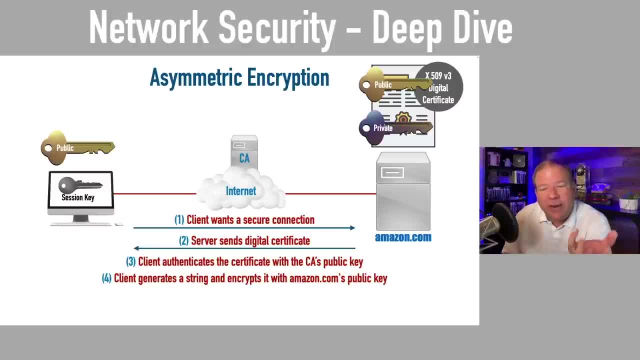 during this session. So what I'm going to do is take this string of data and I'm going to encrypt it using Amazon's public key, And if I do that, if somebody intercepts it, is that a problem? It's not a problem, Because if I encrypt it with Amazon's public key, it can only be. 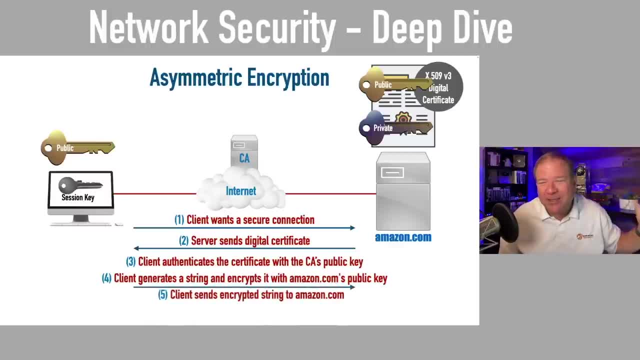 decrypted. So I'm going to encrypt it with Amazon's public key And if I do that, if somebody decrypted with their private key and they don't give that to anybody, So we send this over to Amazon And if anybody intercepts it, they don't have Amazon's private key. it's still secured. 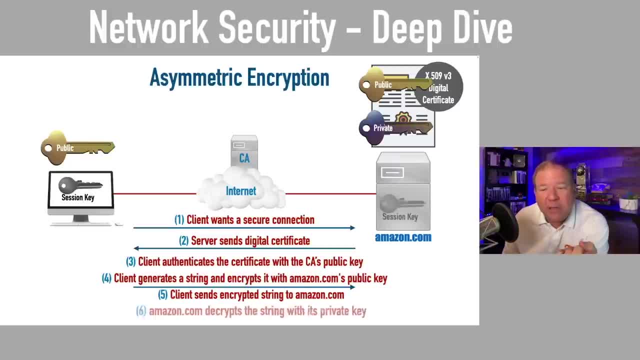 But Amazon, they've got a private key. So Amazon is going to be able to decrypt this big random string that my computer came up with And, based on that, it's going to say: oh, here's the key that I see you want to use for this session. So now I've got the same session. 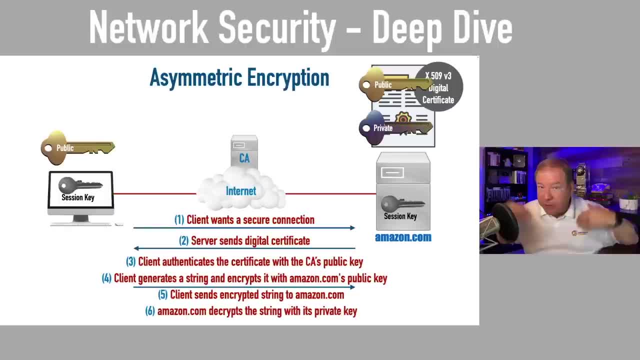 key that Amazon does for the duration of the session. And, just with me, Amazon and I are going to use that to do symmetric encryption. So you see what we're saying here. It's really the best of both worlds. We don't have to give everybody on the 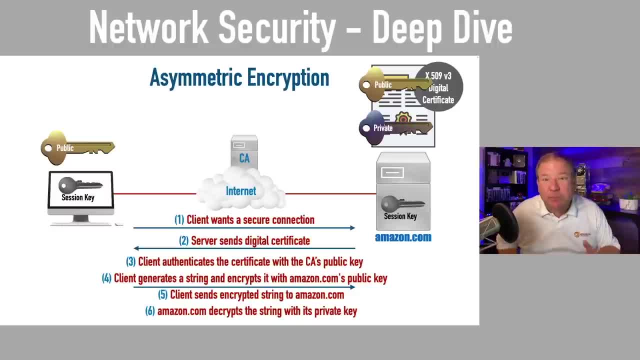 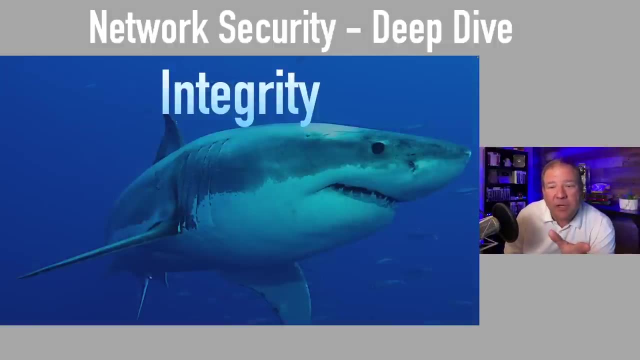 internet, a symmetric key to talk to Amazon. We use this public-private asymmetric key pair And then, based on that key pair, I can generate a symmetric key. All right, I think that's just amazing how that works. But another goal of security you said was integrity. We want to 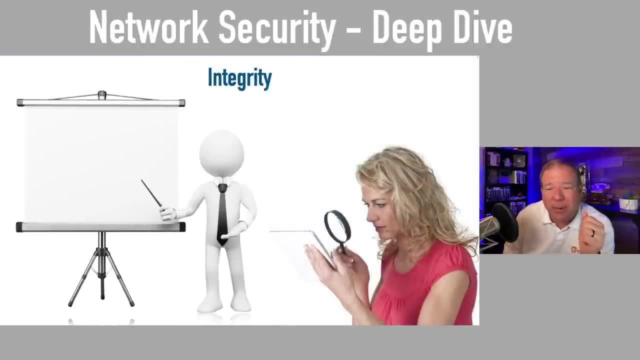 make sure that data has not been modified or scrambled up, And when I say integrity, we can run a mathematical check. It's called a hashing algorithm, And a lot of people confuse hashing with encryption, So let me distinguish between those for a moment. 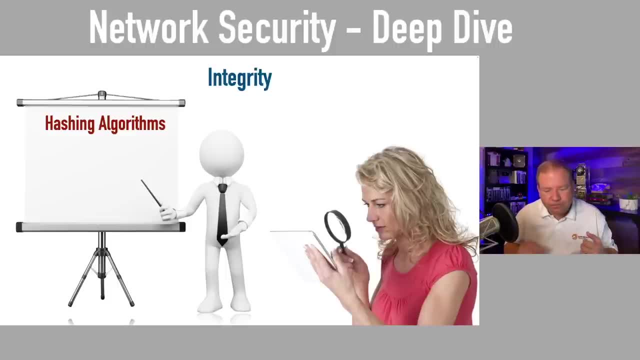 Hashing and encryption are quite different. If I have a big, if I take one of those Cisco Press books off my bookshelf, for example, behind me, and I encrypt it, it's going to be a big, thick book pretty much as well. It's going to be huge because I'm encrypting like 600 pages. 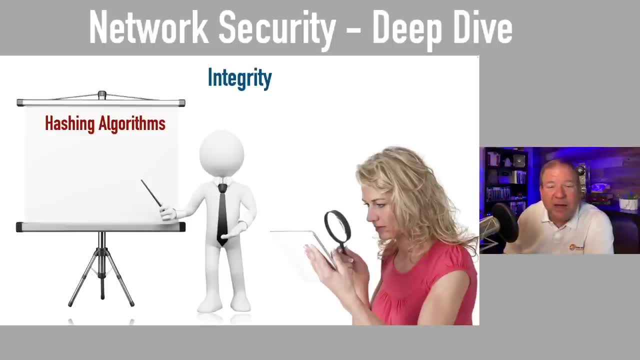 But if I run the hashing algorithm like the MD5 algorithm, the Message Digest 5 algorithm on one of those Cisco Press books, it's going to generate a 125-bit- excuse me, 128-bit result. That's called a hash digest. Think of that as a fingerprint. It's not an encryption. that can be. 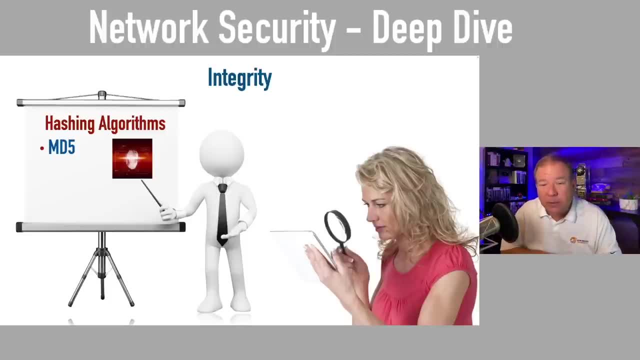 extracted or decrypted. It's a fingerprint And one hashing algorithm is MD5, Message Digest 5.. And the idea is, if I take the fingerprint and I say here's the Message Digest that I calculated, and I send the data to you. 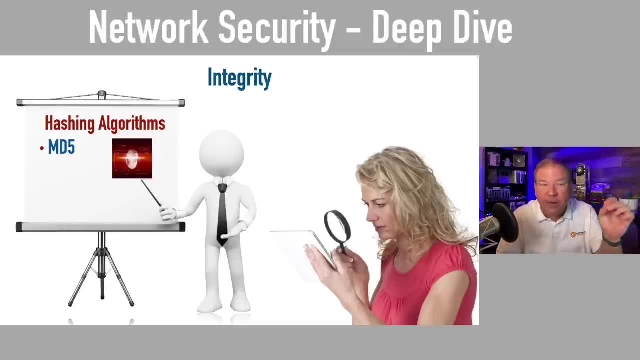 you run that same algorithm and you come up with the same fingerprint. if the fingerprints match, that's a good indication that the data has not been modified in transit. If I took, instead of a book, let's say I took a three-letter word like cat. 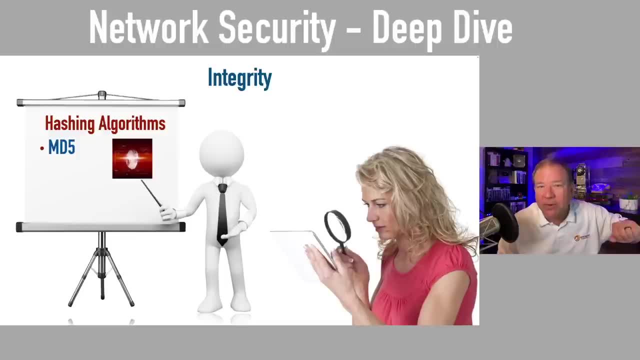 and I did a hashing algorithm like it would also result in 128 bits. See, it doesn't matter how big the string is that we're hashing. If we're using MD5, the result is always going to be a 128-bit hash digest. 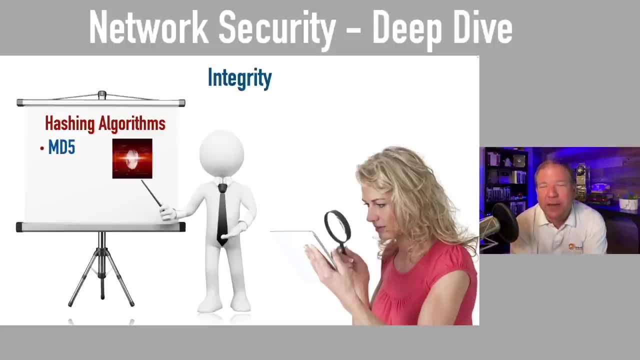 So this is not something that we're going to decrypt. It's just to make sure that the fingerprints match MD5, pretty good. Cisco's used it for decades. But even better than MD5 is SHA. That stands for Secure Hash Digest, And it's going to be a 128-bit hash digest. 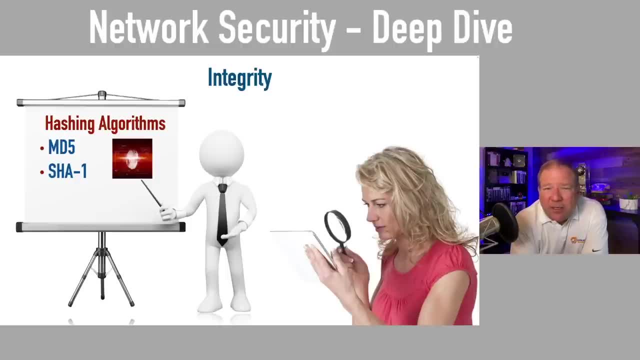 So you've got the option. I'd probably use SHA. It's considered to be more secure. Here's a challenge we have, though Let's say that you're sending me some data And you said: oh, by the way, here's the MD5 hash that I've calculated for this file that you're downloading. 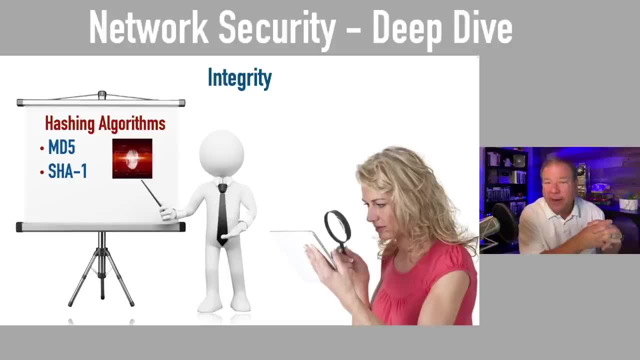 So you give me your string and you give me your file. Well, I'm going to run the MD5 algorithm on that file and I'm going to generate my own, And if my string or if my MD5 hash matches your string, your hash, then that's a good indication. 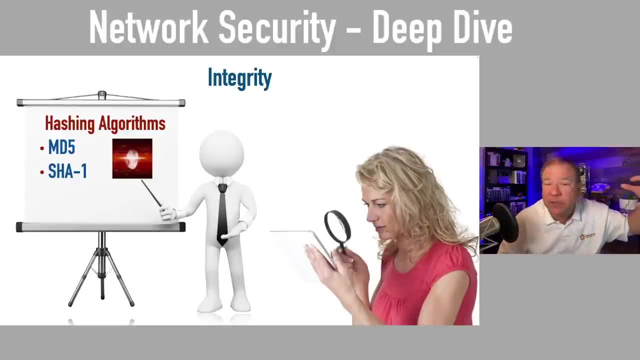 that things have not been modified. However, what if you send me this file and midway through that transmission a malicious user gets that file, they change it up and then they run the MD5 algorithm themselves. They've got a key or not a key. they've got a hash digest based on that. 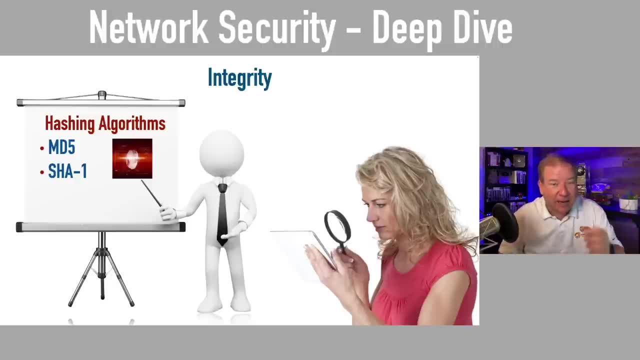 altered file And they send me that file and I'm going to generate that file And they send me that to me saying here's the file and here's your message digest. Well, I'm going to run my MD5 algorithm on that same file that they've altered and I'm going to get the same hash digest that. 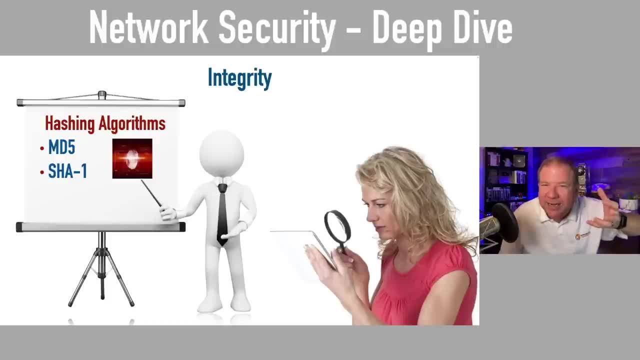 they got. You see, somebody has encrypted or somebody's altered it in transit and they changed the digest. What do I do to fight that? Well, to overcome that limitation, there's something called HMAC- hash-based. let's try that again: hash-based. 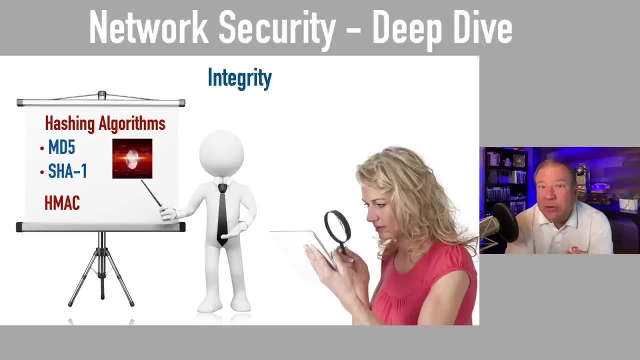 message authentication code That adds a secret key to the mix. So when that hash is being calculated with HMAC, it's going to use that secret key And somebody that intercepts that. they intercept our file and they try to run the algorithm on the file. they don't know the secret. 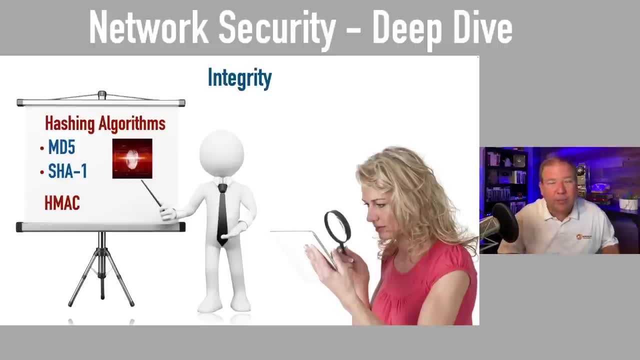 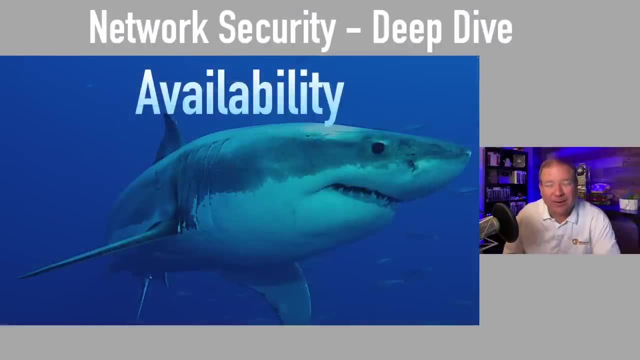 key that we're using, So they're not going to be able to create a believable or a valid hash digest And I'll detect that when I Receive the file and their string. And finally, as we're talking about the three big goals of 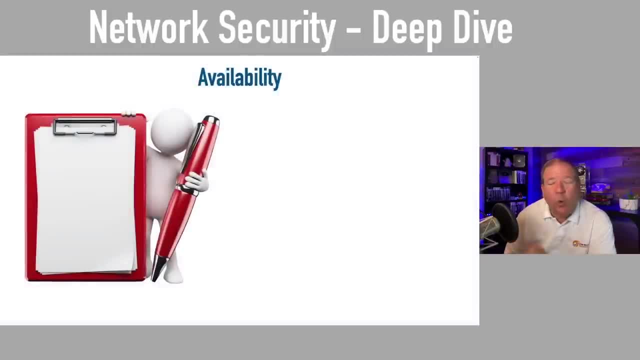 security. there is high availability. We don't want to be denied access to our systems. We want our systems to be highly available. But what does highly available really mean? I was, I heard some- I forget what it was- some service. the other day I heard advertised and they said something like: 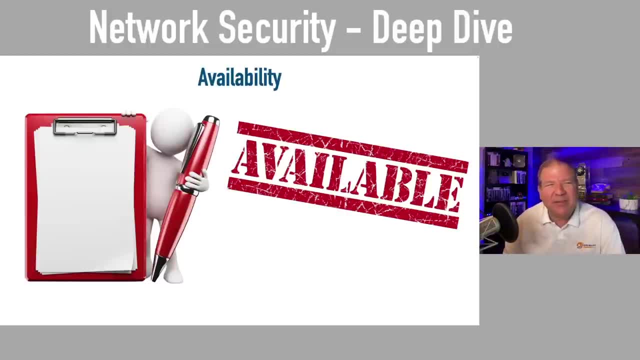 we've got 99.9% availability And I thought 99.9, that's really not that good, That's a lot of damage. And I thought, well, that's a lot of damage. And I thought, well, that's a lot of damage. 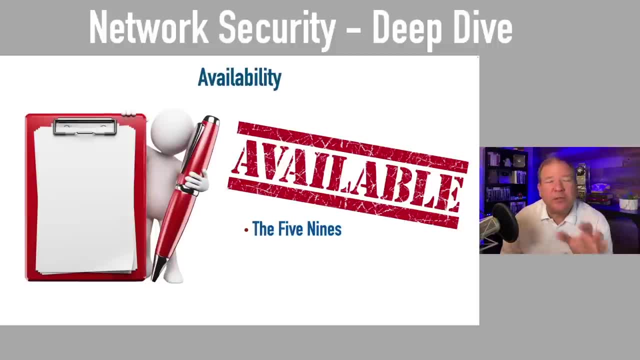 over the period of a year. Really, the sort of the goal standard for availability is called the five nines of availability. That means that we're up 99.999% of the time And if you translate that into amount of time we might be down per year. It's about five minutes. It's really hard to. 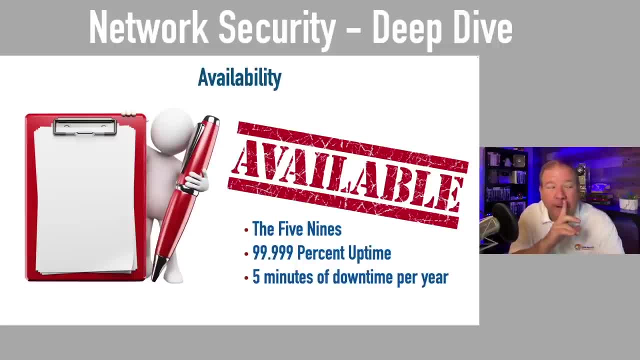 achieve. by the way, it can be very expensive, But really that's kind of the goal standard There. you may have also heard the six nines of availability. That means you're up 99.9% of the time And that's going to give you only about 30 seconds of downtime per year. That's, that's for. 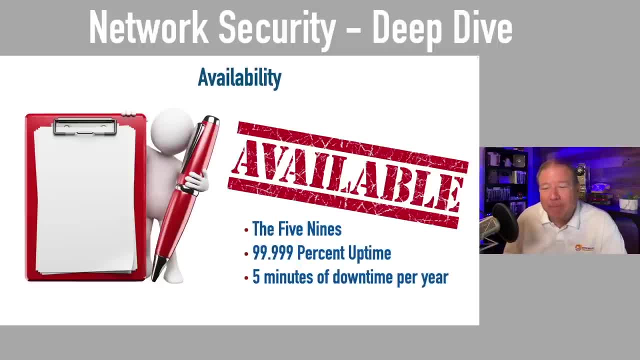 your really super high availability systems. But generally five, nines. that's what we're shooting for, And some things that could get in the way of that is malicious users. they might send us some improperly formatted data that can maybe cause an operating system to crash. We're going to talk. 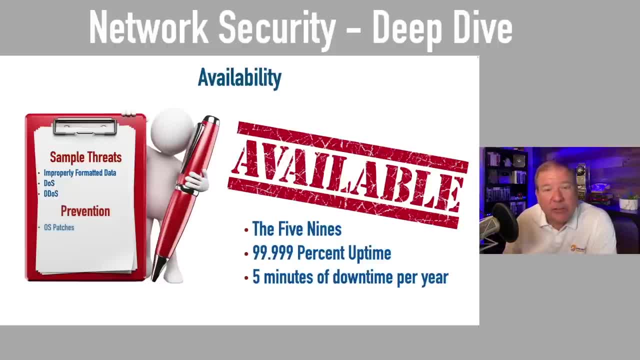 later today about DOS and DDoS attacks And to prevent that, we want to make sure that our operating system is in good condition And we want to make sure that our operating system is up to date. We might want to use some of those firewall appliances like we talked about. 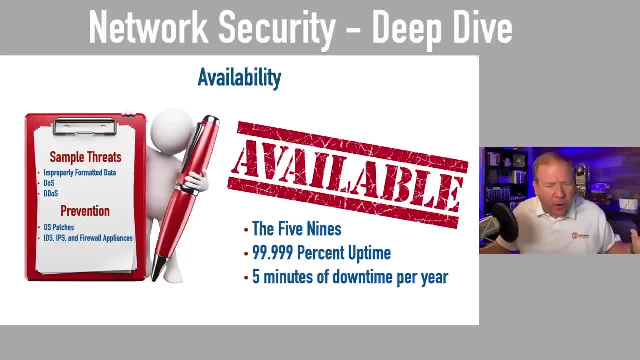 In fact Cisco uses the term that I love the metaphor. They talk about security in depth. They talk about overlapping layers of security. Another: I use the metaphor of: I'm in bed on a cold winter's night and it's really cold in the room And I've got a blanket over me, but my feet 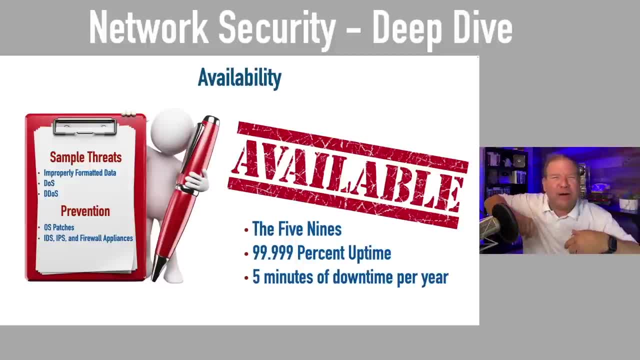 are sticking out, So I put another blanket over my feet. Oh, I got an elbow over here that's sticking out And I'm sorry, I tucked that up. I'm going to put another blanket over my feet, Another blanket. I've got these overlapping blankets, So there are some areas that are. 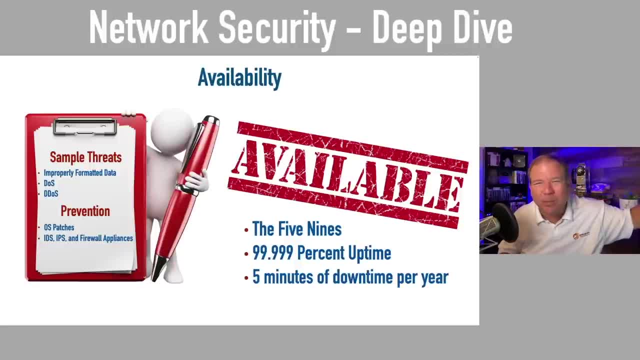 covered by multiple blankets. Some of them might just be covered by one blanket, But by giving overlapping layers of protection, I'm completely protected. Same thing with the network. We don't just buy a firewall and say we're protected, I have a security appliance. No, we want to have. 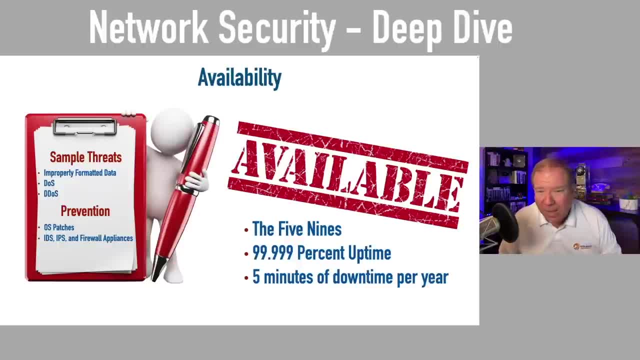 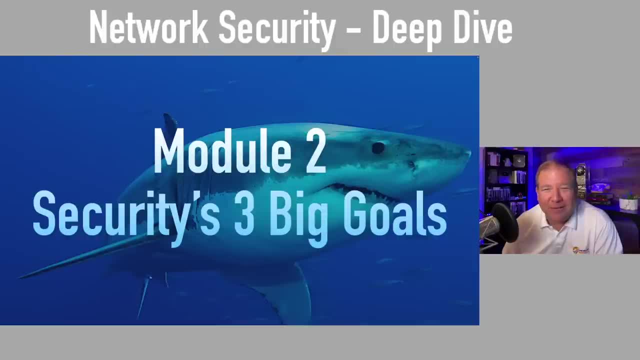 overlapping layers of network security And we talked about some of those. We'll talk about more as the day goes on. But that's going to wrap up module two, the three big goals. In module three we want to take a look at just again at sort of a high level, some common network. 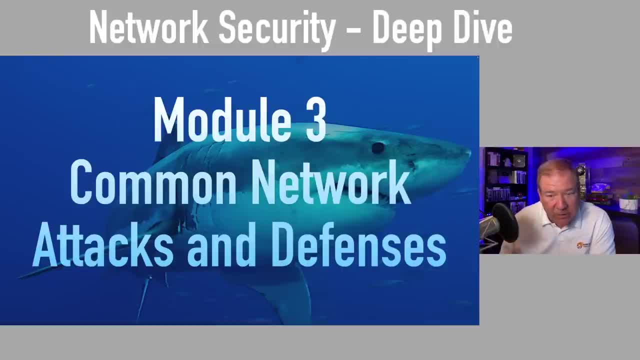 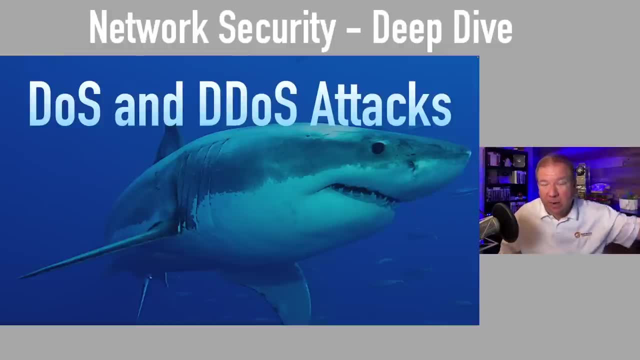 attacks and how we might defend ourselves against some of those attacks. And let's get started with why. I would say one of the more popular attacks out there that you hear about on the news a lot DOS, or denial of service, and DDoS- distributed denial of service attacks. First let's talk. 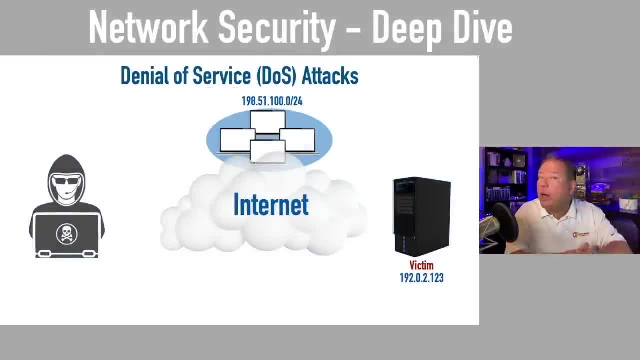 about a DOS attack, a denial of service. This is where we've got one individual malicious user and they're trying to deny service to a system. So here we've got our malicious user. I'm trying to avoid using the word hacker as much as I can, because I realize hackers aren't inherently bad. 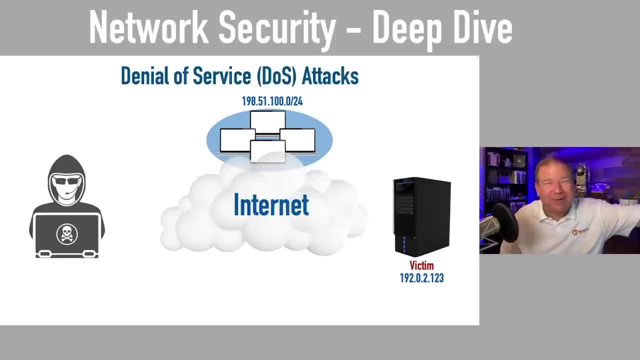 There are white hat hackers. They're good people that are hackers. The term hacker can take on different meanings in different contexts, So I don't want to come across as saying all hackers are bad. That's not the case. So I'm trying to say malicious user, but if I slip up and say hacker, 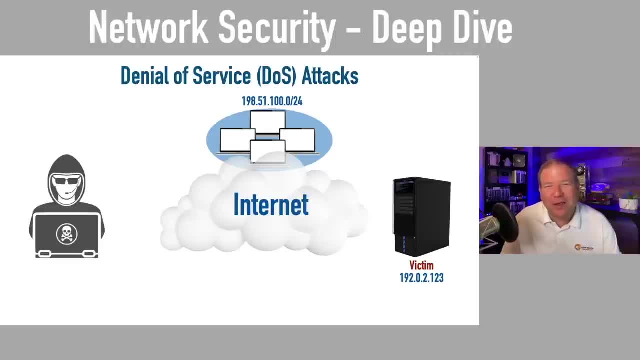 I'm probably meaning a malicious user, But we've got a malicious user on the left hand side of the screen and they're targeting this victim at an IP address of 192.0.2.123.. And there's different ways that we might do this, but this attacker is going to send what is called a ping of death. 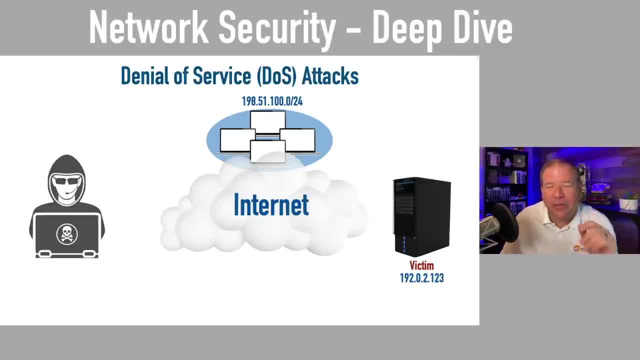 That's a dramatic name, isn't it? It's going to send a ping of death to this victim Specifically. the attacker is going to lie about who they are. They're going to spoof their IP address and they're going to claim to be our victim's IP address. They're going to claim to be 192.0.2.123.. 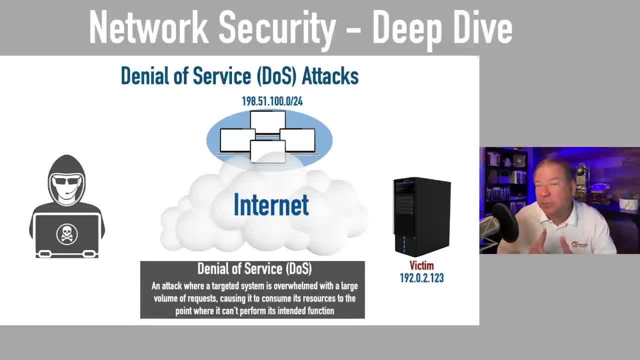 And they're going to do a ping not to a specific IP address, They're going to ping an entire subnet using the directed broadcast of a subnet. Remember: a directed broadcast address goes to everybody within that subnet. So they're saying they're spoofing, they're lying about their source IP. 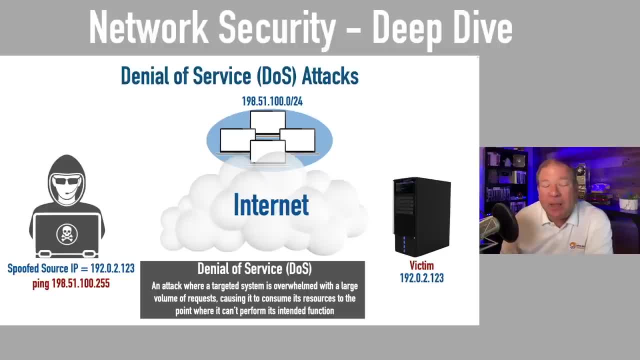 address. They're saying it's 192.0.2.123 and they're pinging the broadcast, the broadcast address Of that network. they're pinging 198.51.100.255.. And when they go to that directed broadcast. 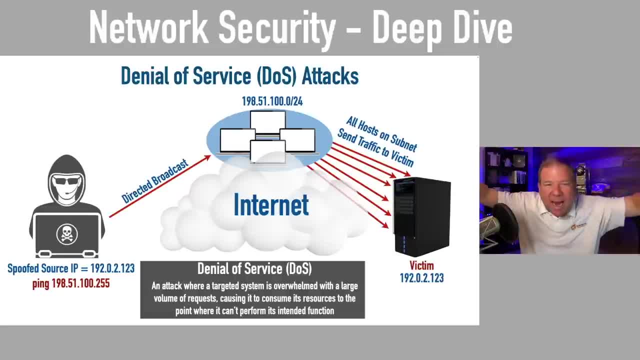 the response from every device in that subnet comes out and bam, they all hit that victim at once. And this can just continue on and on. And that poor victim machine. they're so busy trying to deal with that onslaught of ping responses They might not be able to do their regular job. 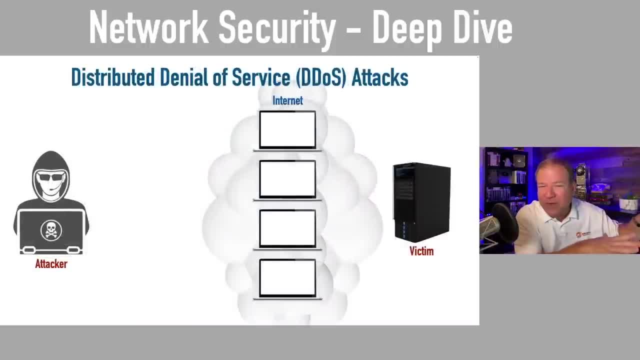 Now that's with one attacker trying to flood a victim with a lot of traffic, and they were leveraging a directed broadcast, But we hear a lot. probably a more destructive type of attack than a DOS is a DDoS or a distributed denial of service attack Here, instead of just one malicious user trying to flood a victim with. 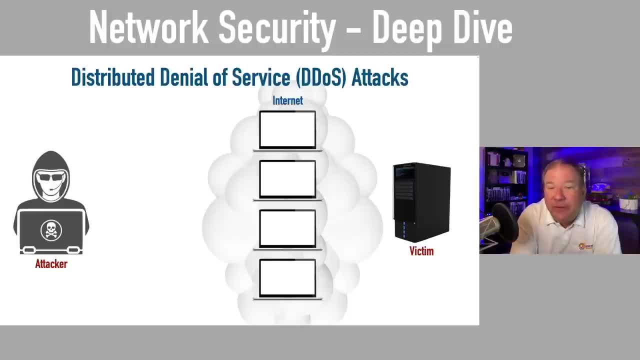 lots of traffic. they, over time, can infect devices around the world, maybe tens of thousands of devices around the world, And they're going to be able to infect them with malware perhaps, but they're going to become under the control of our attacker. Now, these infected machines? 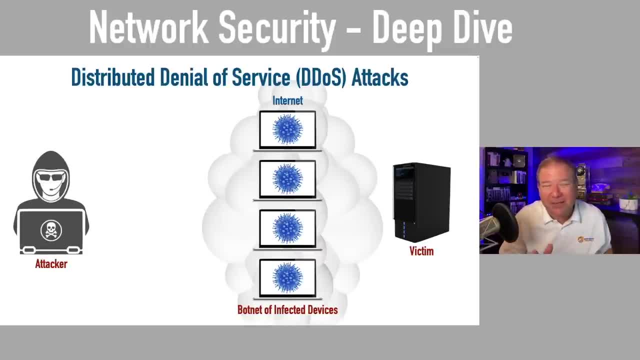 sometimes are called bots, Sometimes they're called zombies. And this attacker, when they get ready to launch the attack against their intended victim, they're going to talk to a server that they have called their command and control server That's going to coordinate. 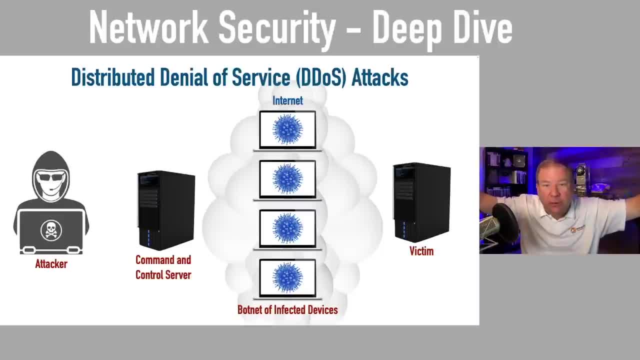 instructions going out from that command and control server to these infected bots, or these zombies. It's literally the rise of the zombies here. We're talking from the command and control server to these infected bots, Computers around the world, and we simultaneously have them all rise up and start attacking our 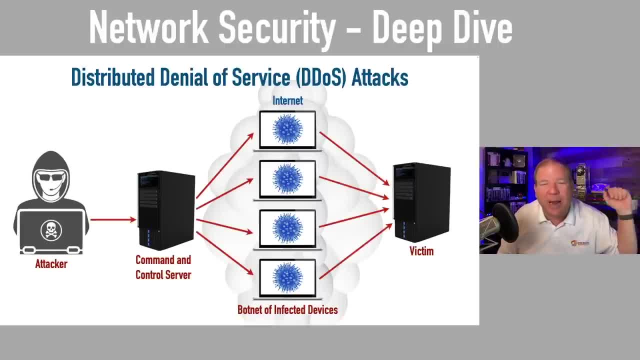 intended victim. So by maybe getting some malware into the hands of users around the world, pretending to be maybe a game, some sort of other application, or maybe we have some malicious code on a webpage that infects them, we can then, or the attacker can, control them and say, all right. 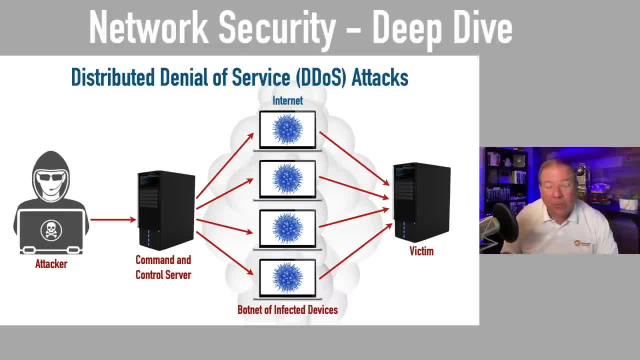 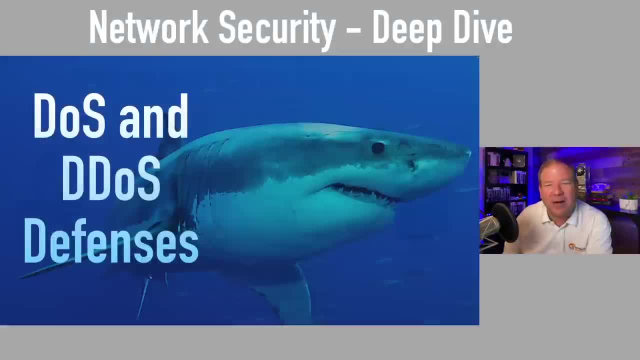 attack And simultaneously they all attack the victim, And if we've got tens of thousands of computers around the internet, that's more likely to do that. So we're going to have a lot of damage than just a single user trying to generate a lot of traffic targeting a system. How do we? 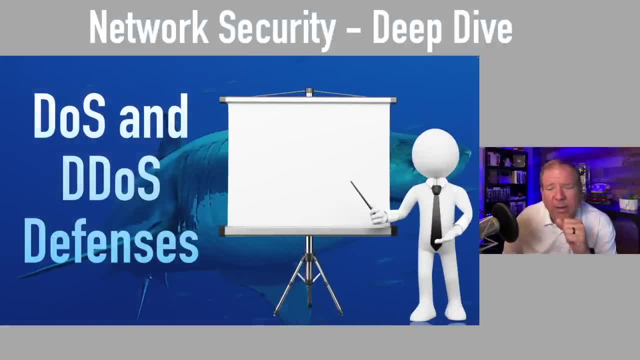 protect against that. It sounds pretty bad, doesn't it? Well, here are some. here's some general guidelines, And this is some content that I've taken from CEH. Charles taught some of those modules. I taught some of the modules. This is from a module that I taught, and it's talking: 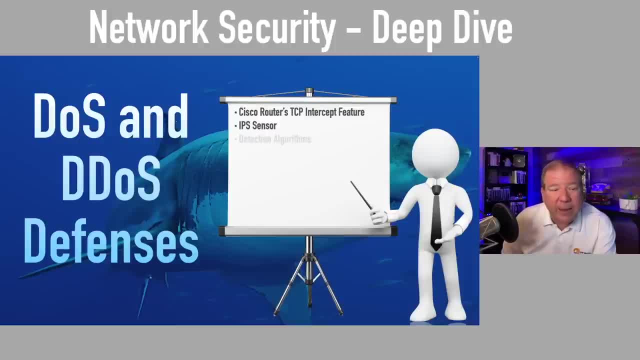 about how we can defend against DOS and DDoS attacks And we'll talk about each of these. TCP routers have a TCP intercept feature. We've already talked about the IPS sensor. There are some detection algorithms. We might want to give more bandwidth than we need to handle the excess traffic during. 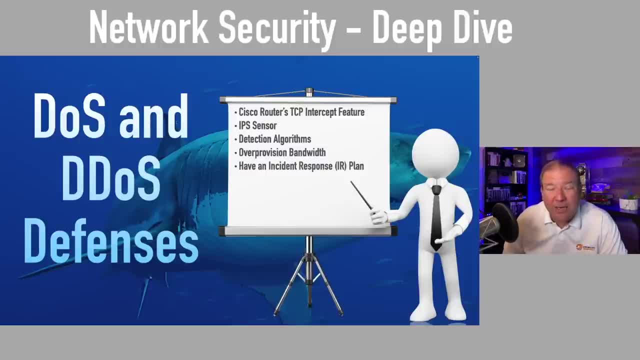 an attack. Know what we're going to do in response to attack with an incident response plan, And we might want to pay somebody to attack our network that we know about so that they can detect any weaknesses before the bad actors detect. detect any weaknesses, But let's talk about these one. 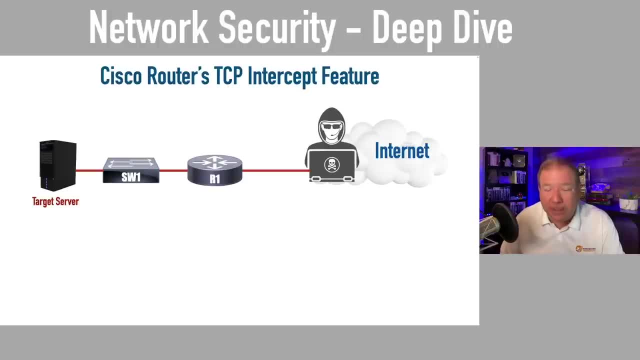 at a time, beginning with this TCP intercept feature. Remember how TCP works. It's a three-way handshake. If I want to set up a conversation with you, I'll send you a synchronization message, an SYN, a SYN message, And I'm saying: Hey, I'd like to talk to you, And you respond with an. 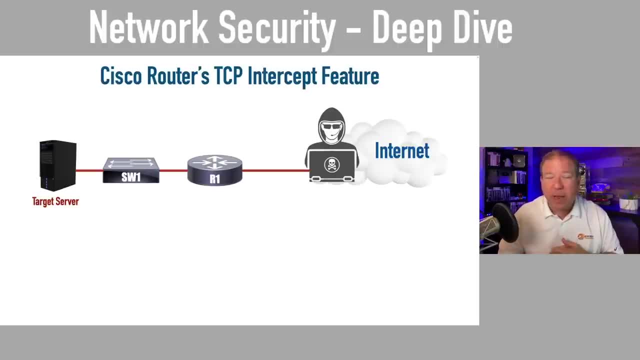 acknowledgement saying: Okay, I'm willing to let that happen. You can talk to me. Oh, by the way, I want to talk to you too, So you'll send me a SYN of your own. So I send you a SYN saying: 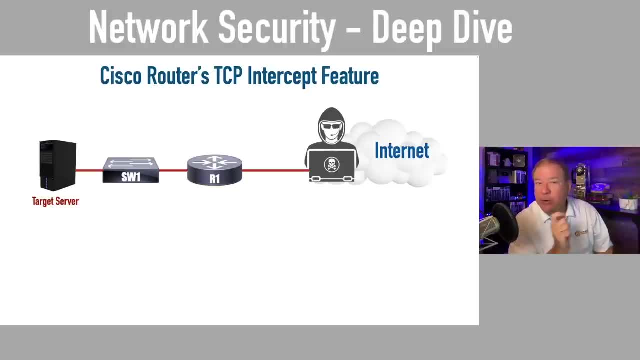 let's talk. You send me a SYN ACK saying I want to talk to you And yes, I acknowledge your SYN. And then I'll acknowledge your SYN with my own ACK. So the three-way handshake- SYN, SYNAC, ACK. That's how a TCP session is set up. Now the attacker. 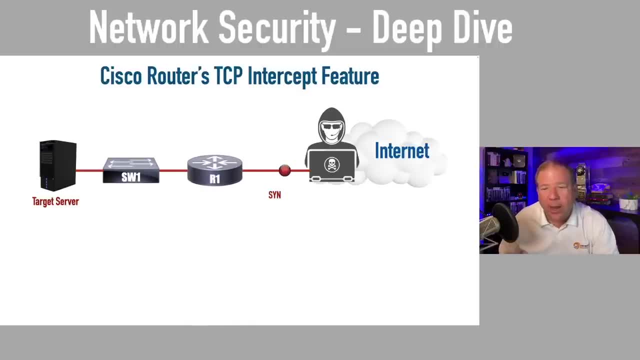 is sending a synchronization message into router R1, and with the TCP intercept feature, R1,, before it passes the traffic onto the target server. one option for setting this up is to have the router itself participate in that handshake. So the target server, anybody on the 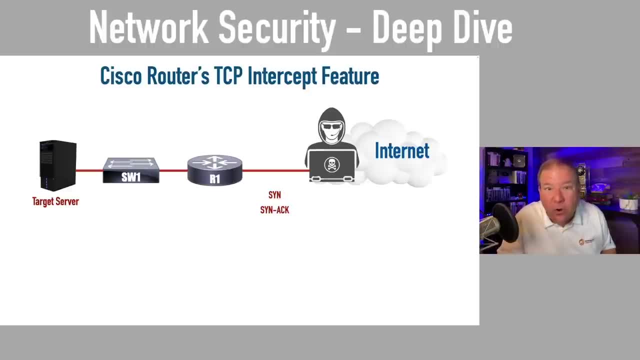 inside of the network. they don't even become involved until the router has confirmed that this session is fully established. So, on behalf of our server, in this example the router is responding with a SYNAC and the attacker responds with an ACK, and once the three-way handshake is, 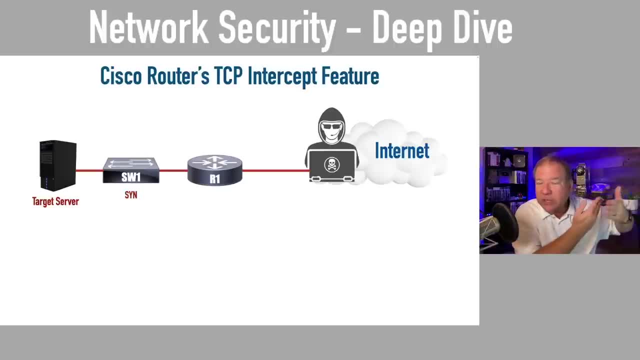 set up, then the message or then a session is set up between the router and the target server and they're tied together. So the attacker or the person on the internet- we don't know if they're bad or not- yet they're then talking to the target server. 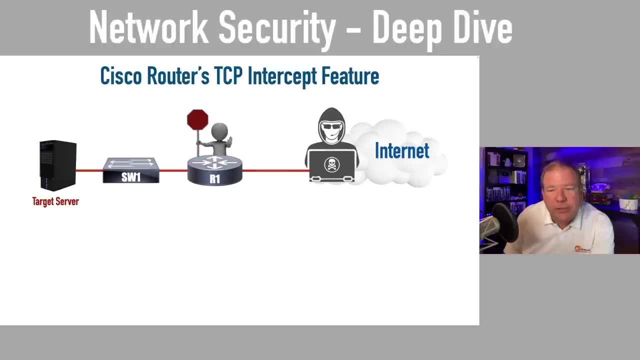 But what that malicious user might do is send a flood of synchronization or SYN messages saying, hey, let's set up a session, let's set up a session, let's set up. they just flood it over and over, and every time they do, the poor router's saying, okay, here's my SYNAC, okay, here's my. 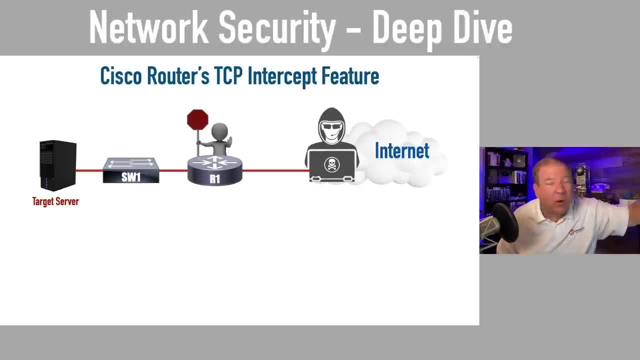 SYNAC. If we flood this router with all these SYN messages but we never respond to the SYNAC that they send back to that the router sends back to the attacker, then the router resources are being consumed. They've got what are called half-open connections. 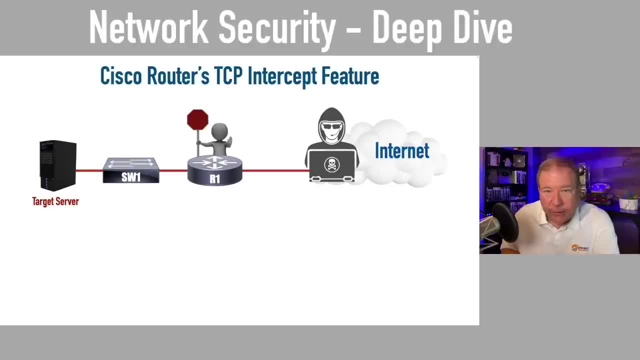 or sometimes in the literature they'll be called embryonic connections. they're not fully formed connections And these connections, if there's enough of them, will consume our router resources, thus giving us a denial-of-service attack on the router. So here's something I used to do. 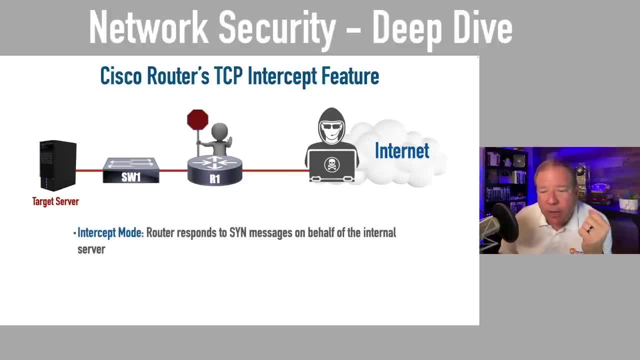 years ago back at the university where I was the network engineer, we set up this TCP intercept feature and there's two modes we could operate. the intercept mode is what we saw in the animation a moment ago. that's where the router is going to make sure this is a valid session, before we ever get somebody on the. 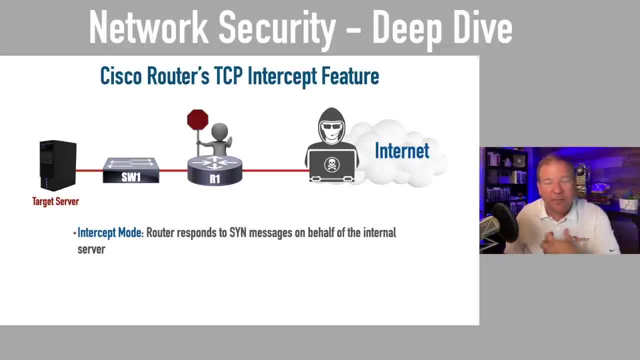 inside of the network involved. they're going to respond to the SYN messages on behalf of the inside users and if it's not set up, we don't have to have the server on the inside deal with all these half-open connections. the router's going to deal with that, Or we could be more. 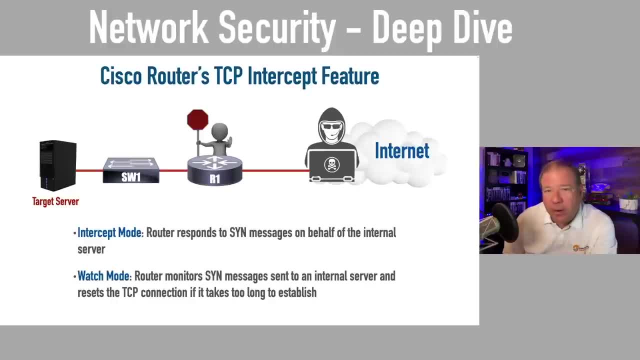 passive. the router could be in a watch mode and in watch mode we're. we're looking at what's going on. we're watching the traffic go. we see the SYN message. I see you, SYN message. you're going to that target server on the inside. we made a note of that. 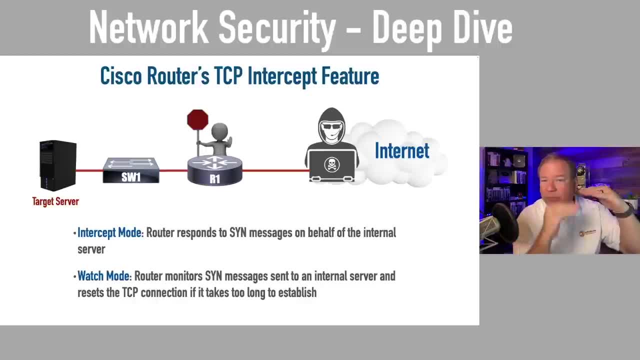 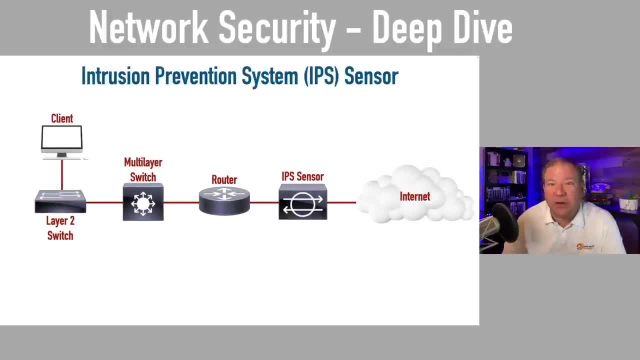 and we'll let it happen until we exceed some threshold where there have been too many SYN messages sent within a certain period of time. At that point the router gets involved and starts blocking things. Another way to prevent or to mitigate those DOS and DDoS attacks. 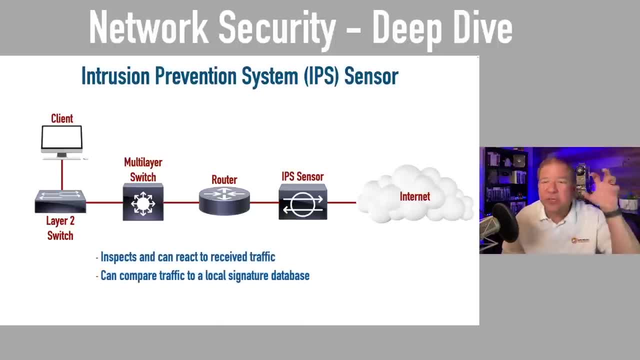 something we've already talked about: an IPS sensor where we can have a signature of well-known attacks and those well-known attacks, if we, if they match a signature in that signature database, we can block them in line. And this signature database. 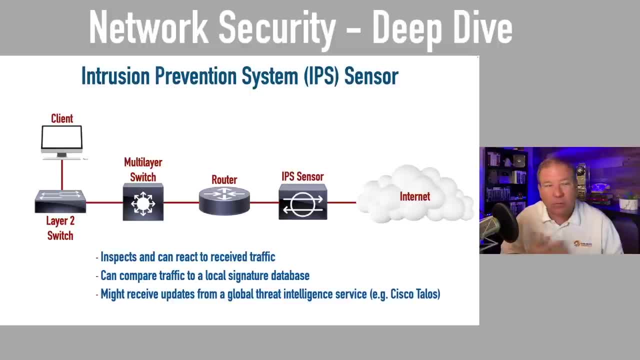 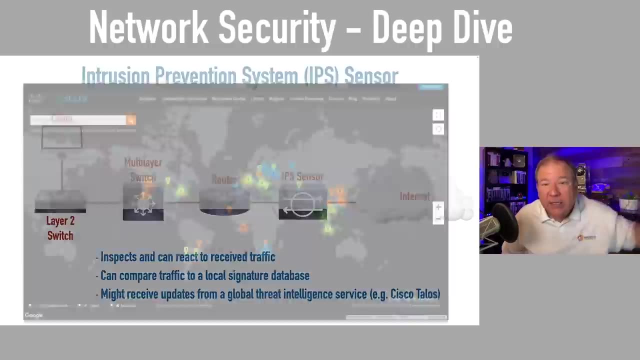 could be something that we update regularly as as part of our weekly routine or sometimes. sometimes we can integrate our IPS sensor with an online service that keeps up-to-date information about threats like day zero attacks that are emerging on the internet. Cisco has something called Cisco Talos, and we can integrate our Cisco IPS sensor with Cisco Talos. 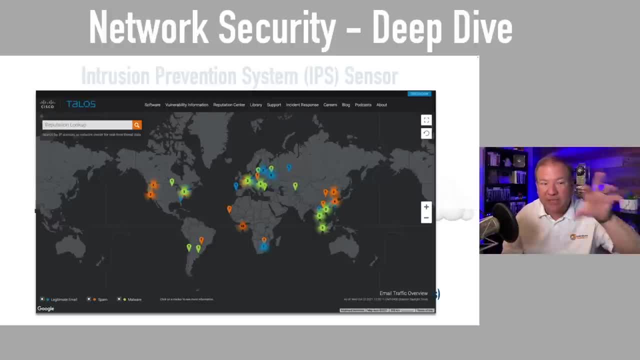 and it's going to tell us, and it's going to give us information about these hot spots around the world that are having security breaches and we can see what, what the current signatures are that we're trying to protect against One of the toughest things to block with a DOS or DDoS attack. 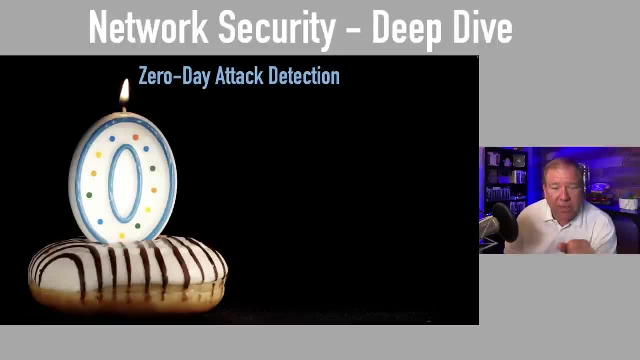 is called a zero-day attack. This is where a user for the very first time, or a malicious user, they launch for the very first time an attack and it's not in our signature database. How do we detect something that we don't have a record of? Well, there are zero-day attacks, can. 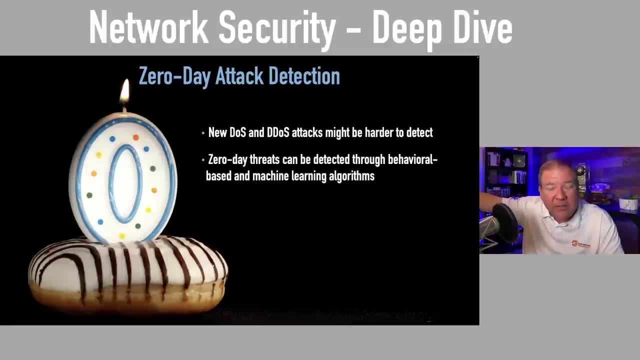 be somewhat mitigated by integrating with an online system like Talos. that's going to give us very quick updates when those are detected. But even beyond that, Cisco can use as part of their Firepower Firewall series. they can use machine learning to detect. 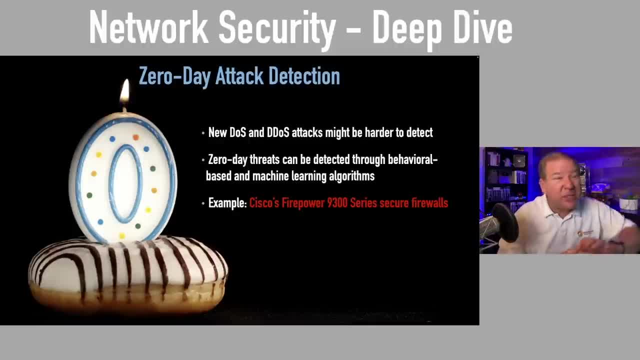 what it estimates to be malicious traffic, Even though it's never been detected, and long before it's not in our signature database. yeah, Cisco Firepower might be able, through machine learning, again to detect what it suspects to be malicious traffic and then isolate or block that traffic. 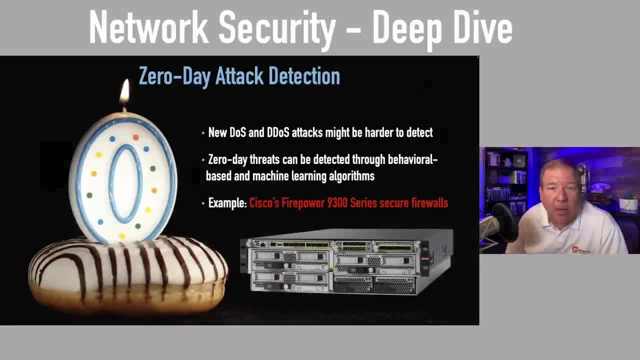 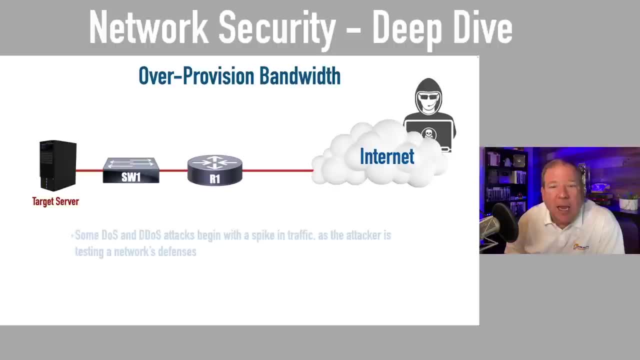 And that's available on the 9300 series as an example: Cisco Firepower Firewall. Cisco also recommends that to protect against a DOS or DDoS attack, we can over-provision our bandwidth, because when we are being attacked with a flood of traffic coming in, that flood of traffic is. 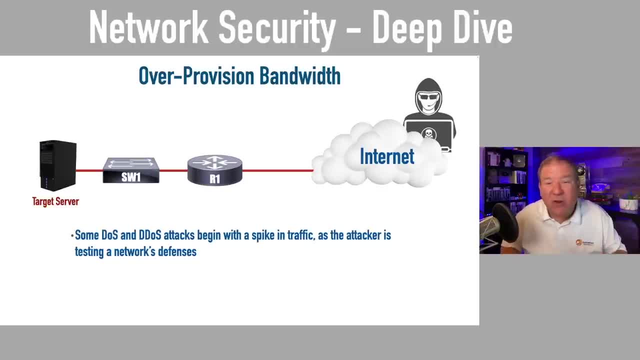 going to be consuming extra bandwidth coming into our network. So even if our router is keeping a log of all those send messages and we're blocking stuff and we're recognizing malicious traffic, it's still coming over the pipe to us. So during the time where we're detecting and responding to 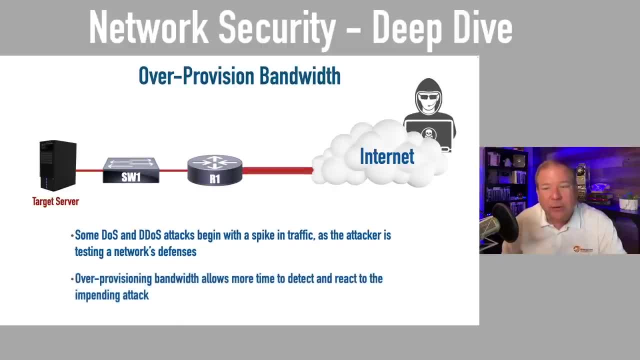 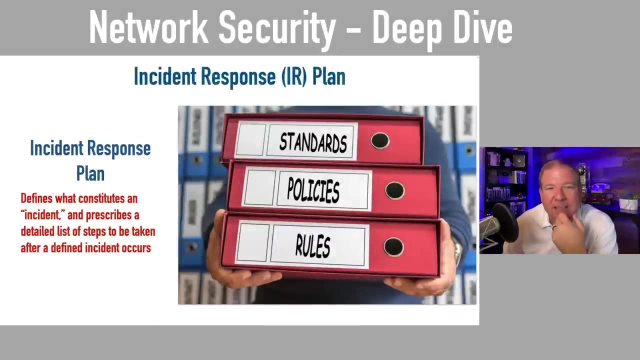 that attack. it might be a good idea to have some extra bandwidth on that link. So if we do have that flood of traffic coming in, we're better able to handle that and we're not getting a denial of service on our internet link as an example, And when we are under attack, it's great. 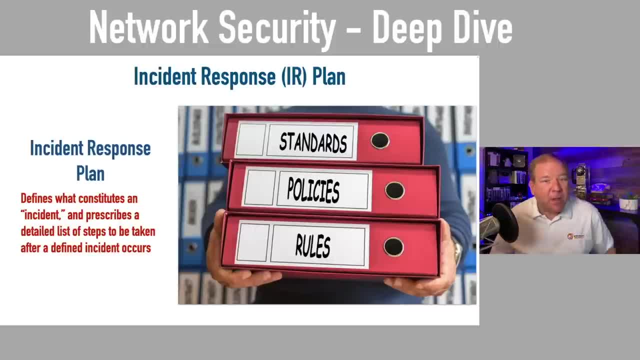 if we know what we're going to do in response, Because sometimes, honestly, I see a lot of emotion in networking when things go wrong or when attacks happen. Some people can kind of freak out: Well, we're under attack, What do we do now? Let's unplug everything Now. it's a lot better that. 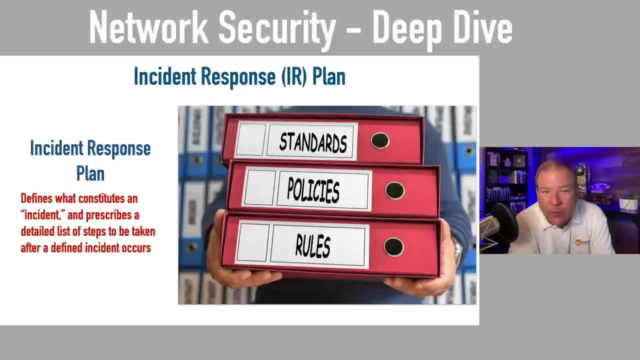 instead of trying to come up with a response in the heat of the moment, we're going to be able to under the pressure of we're under attack. If you have previously, with a clear mind, documented what you're going to do in response, you've got a plan of action. So, oh, we're under attack, Let's. 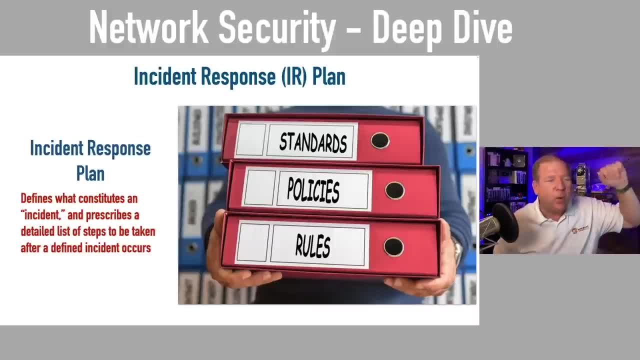 execute this plan. Bam, We're going to do this, this and notify these people. We're going to set this up. We're going to make this rule. We're going to update this. We're going to have a step-by-step plan of how we've pre-decided to respond to any future attacks. It's going to. 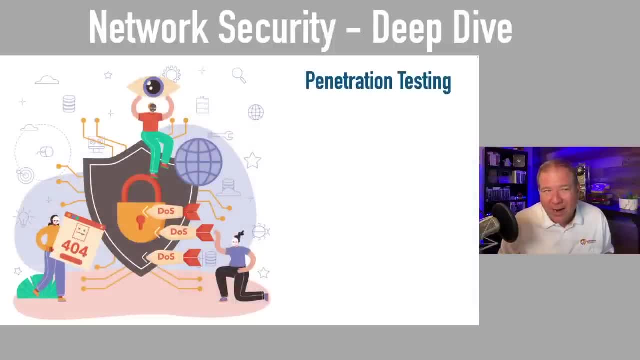 make things go a lot quicker, a lot smoother, with a lot less stress. And another option for protecting against these DOS and DDoS attacks is to recognize any vulnerabilities before the bad people recognize your vulnerabilities. You might see this in a movie or a TV show, sometimes where in a bank maybe. sometimes a bank will pay somebody to. 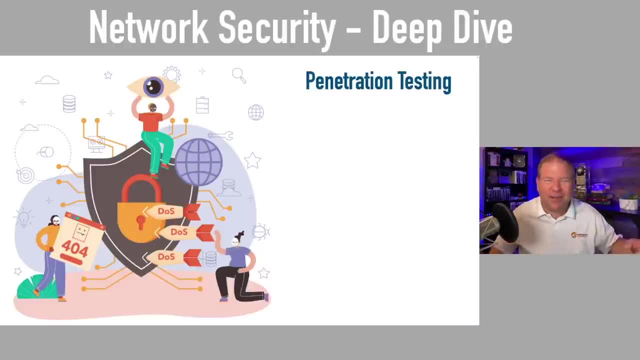 see if they could break into their bank, And if they can, they come into the conference room, they put down the big duffel bag and it's full of this money. Yeah, I got all this from Revolt and here's what I did to get in. You might want to patch these security breaches. Well the same. 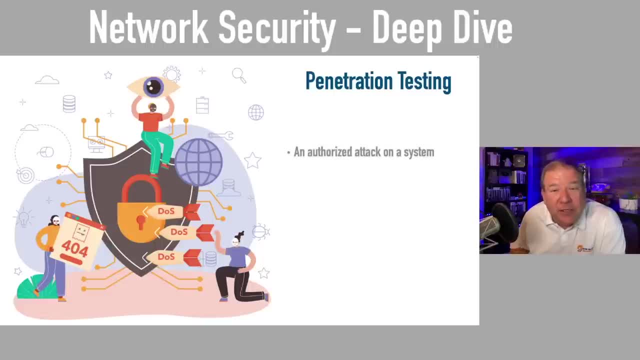 thing with our networks. We can pay somebody to do penetration testing. In fact, there's a certification- PenTest Plus- from CompTIA that trains you to be a pen tester. But this is an authorized attack on a system. We know somebody's attacking our system and it's not to do bad things. 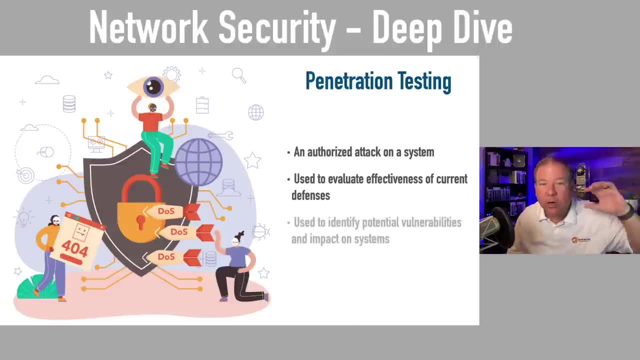 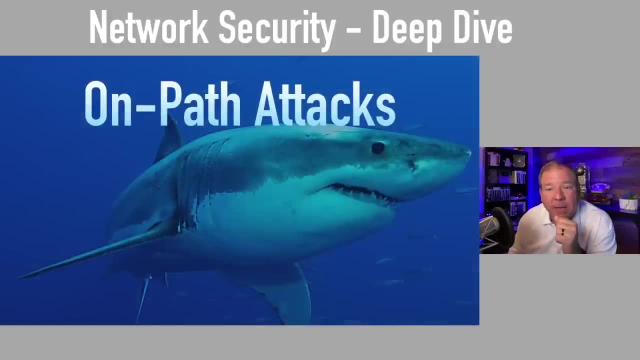 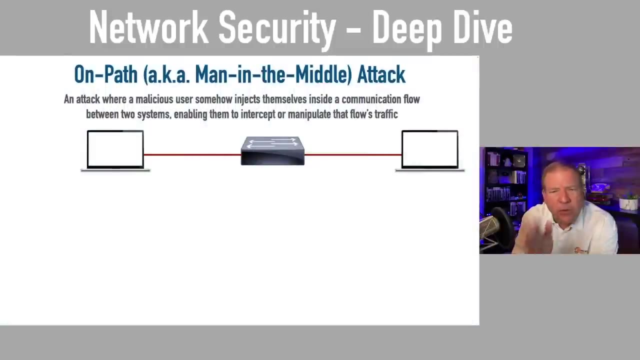 to our system. It's to evaluate our current posture, our current level of security and identify any vulnerabilities that we might need to address. Another type of attack is an on-path attack, or sometimes this used to be called a man in the middle. You'll hear it called either. 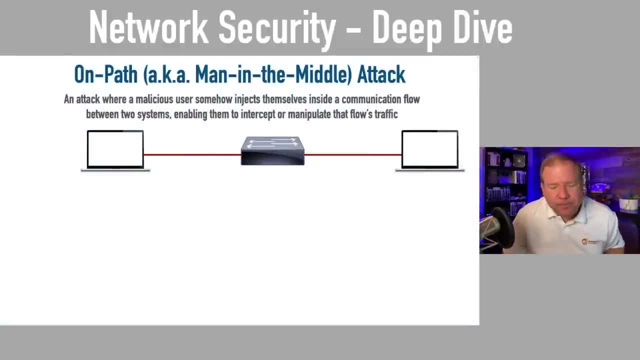 one on-path or man in the middle. But the idea is we've got somebody sitting between the source and destination of our communication flow. And here I've got a couple of computers are talking back and forth to each other, no problem. But what if an attacker comes along? If an attacker comes, 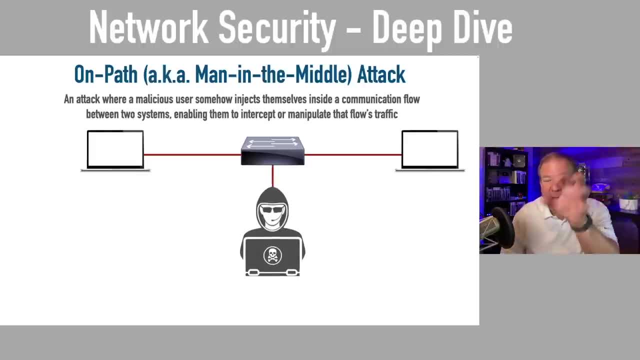 along and plugs into this switch and it starts getting copies of traffic going between those PCs. they might be able to decrypt that traffic. Maybe that traffic's not even being sent in clear text. Maybe they can have one system send their traffic to them, They modify it or they capture it and 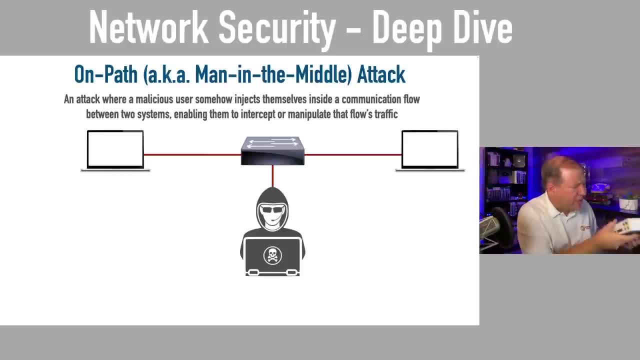 then they send it to the destination. But how would that work? I mean, think about this. One of the great things we love about a Cisco, or an Ethernet switch in general, is that the switch is going to build a MAC address table. It's going to learn what MAC addresses are available off of. 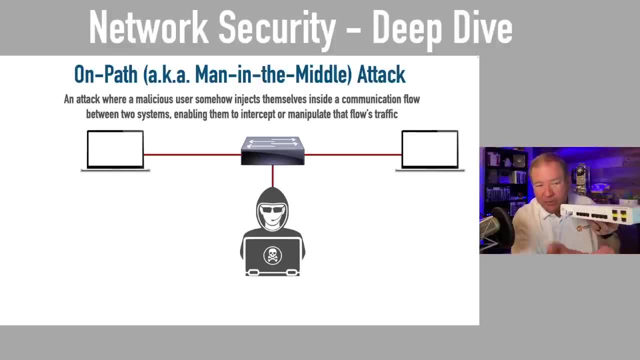 different ports. Then when traffic comes in, let's say from one of these laptops, and it looks at the destination and the destination is the other laptop, it's going to say, oh, that lives off this port, So I'm only going to send the traffic out of that port. 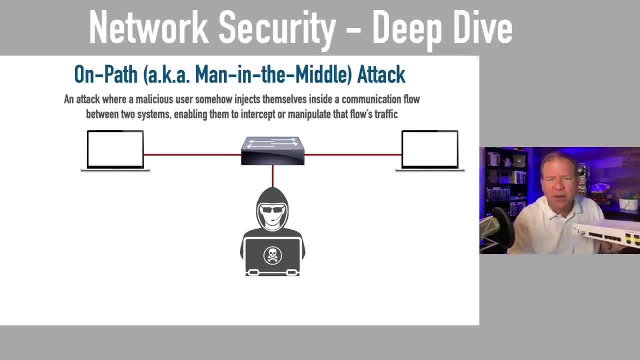 We're not going to send anything to this attacker that just plugged in. How would that even work? How can that attacker inject themselves into this conversation when a switch by its nature prevents that? That's what we're about to talk about. I want to talk about three different ways. 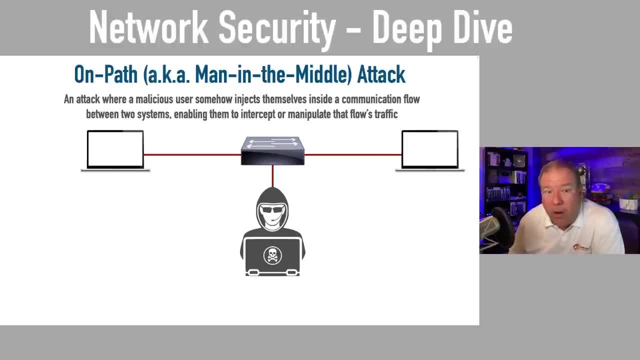 that an attacker might launch a man-in-the-middle or an on-path attack. One option is to flood the MAC address database of this switch. Just to give you a preview, this switch, I think, holds a little over 8,000 MAC addresses in its 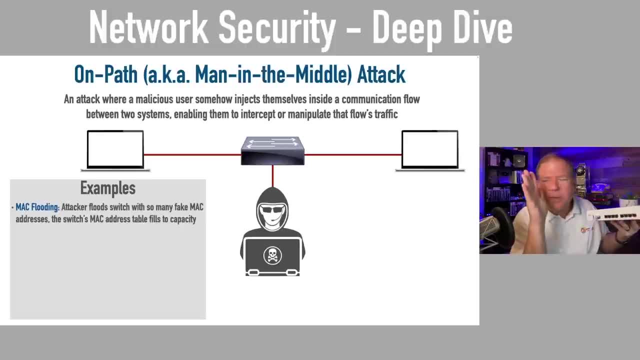 MAC address table. What if it were full? If that MAC address table were completely full and somebody plugged in, would their MAC address be learned? No, There's no room to store that newly attached machine's MAC address. So if I'm sending traffic to 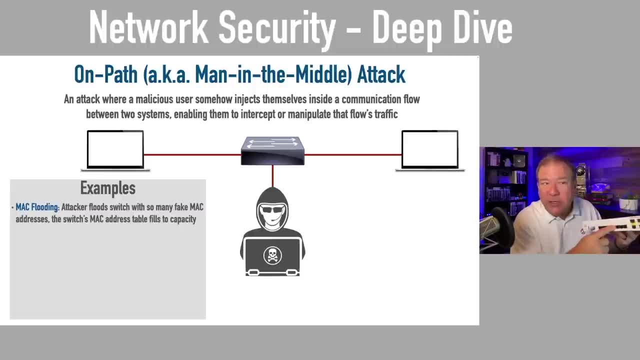 that new machine that just attached and I did not learn its MAC address. how do I get it to that machine? I don't know where it lives. I'm going to flood it. The switch is going to flood that traffic out of all ports other than the port on which that frame arrived. So that's one way that 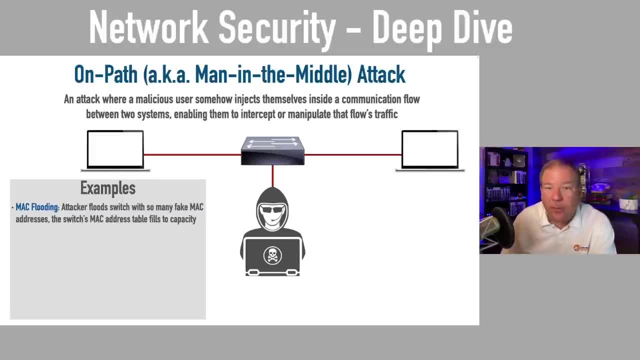 an attacker might inject themselves. They fill up the MAC address table of a switch. So a newly attached device. that traffic going to that newly attached device is going to be flooded out of all ports, including the port to which the attacker is attached. We'll also talk. 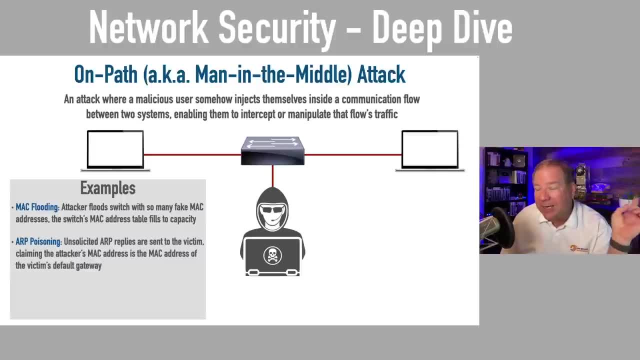 about ARP poisoning, Where we might actually convince an end system and convince a router that they should send our traffic to us instead of the router or that end system, And if we can use our DHCP server to inform a client about IP address information and DNS information and default gateway information. 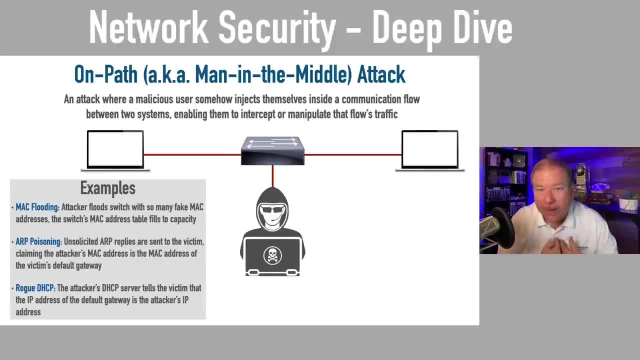 we could direct them to us as their default gateway, Or we could direct them to our DNS server. So if they're trying to go to a social media site, perhaps direct them to what looks like a social media site, But it's really something under our control. 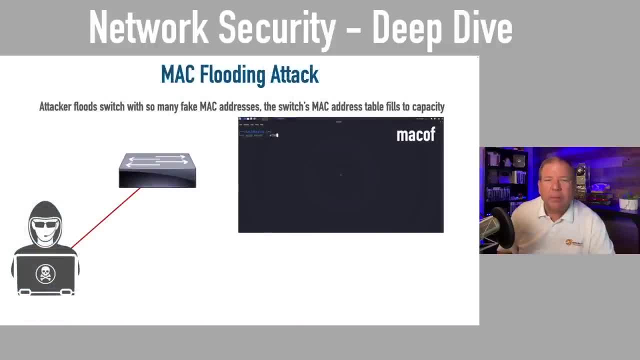 and we're capturing their credentials when they attempt to log in. So let's talk about each one of these. First, I discussed how we can fill up the MAC address table of a switch, And if we do that, a newly attached device is not going to have their MAC address learned. Here's what an attacker 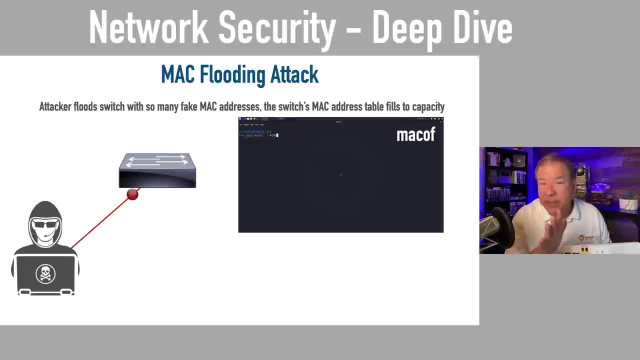 might do. The attacker might send from their one PC a series of frames into the switch. But using an application, MACAW, they're going to send a series of frames into the switch And they're going to send thousands upon thousands of frames within just a matter of seconds into the switch. 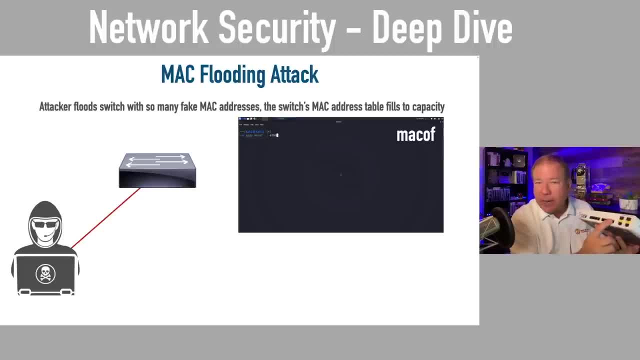 And we're going to claim that each frame is from a different MAC address And it's going to think that there are like 8,000 MAC addresses living off of this one port, which is possible, I mean, if that one port connects into a switch that connects into a bunch of other switches. 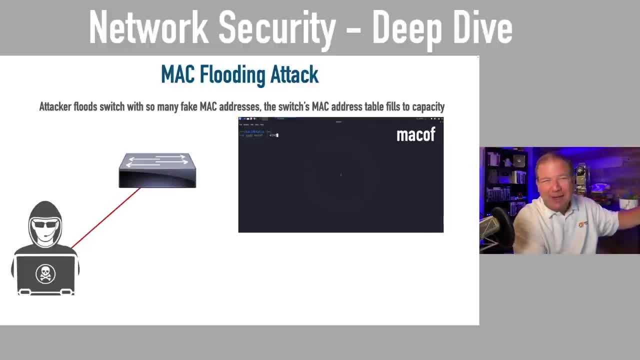 that connects into a bunch of other switches. they have PCs. Yeah, we could potentially have 8,000, not likely, but we can have 8,000 devices off of a single port in a case like that. But an attacker might use this application called. 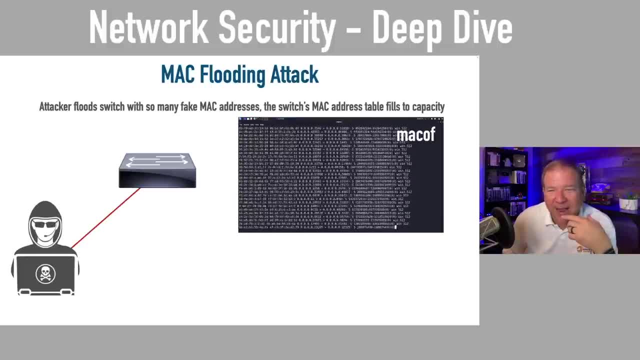 MACAW. that comes built in with Kali Linux. I think. Here's a little video of me doing it on Kali Linux And within about three seconds I fill up the MAC address table of this very switch. And here is a show: MAC address table count. 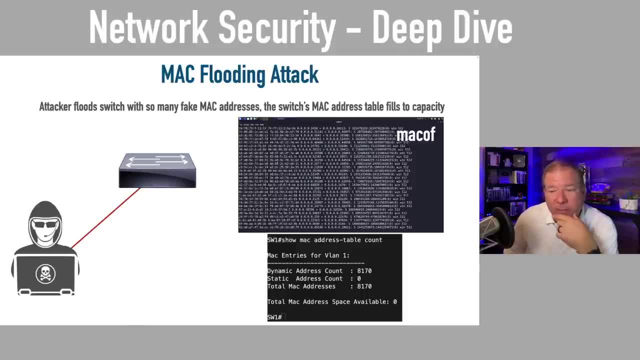 that I did after about three seconds of this flooding, using MACAW, And it says that this switch was capable of storing 8,170 MAC addresses. And right now, how many are available? Zero, In about three seconds, I sent over 8,000 frames into that switch, each claiming to be from a 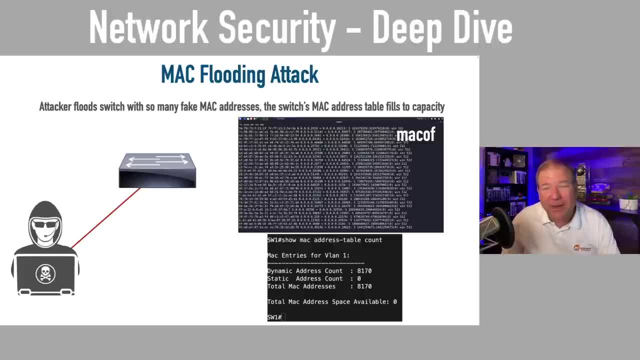 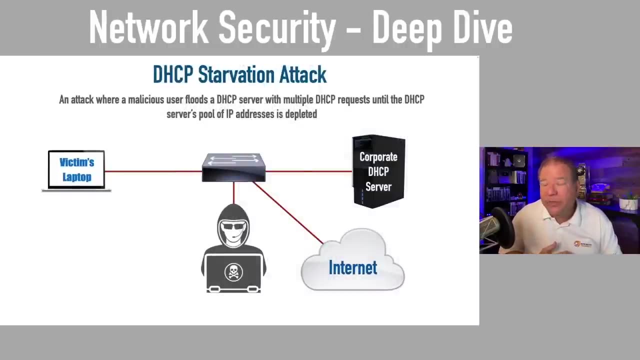 different MAC address And it completely saturated and filled up that MAC address table. By the way, I'm about to show you in a live demo how we can fight against that using a feature called port security. Something else that might happen is a DHCP attack With the DHCP. 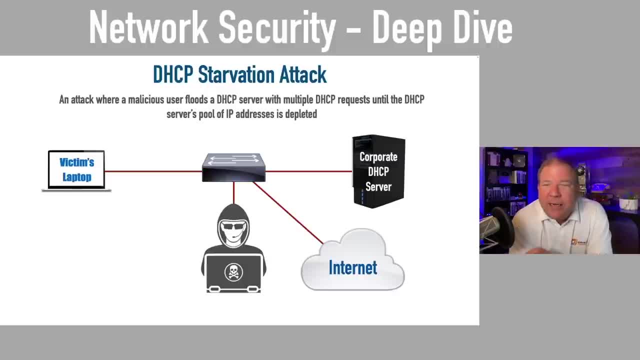 attack. we're trying to convince a user to come to our rogue DHCP server and get information from us. If we can send them information saying here's your IP address and here's your default gateway, what if we give, if we're the attacker? what if we give our IP address as the default gateway? 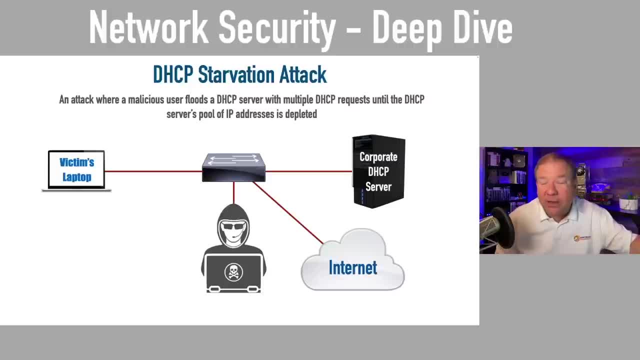 Well, suddenly, that poor suspecting victim, all the traffic leaving their subnet they're sending to us. We might capture it, we might alter it, and then we'll send it on to its intended destination, so that they're none the wiser, Because it does get to the destination after we captured it. 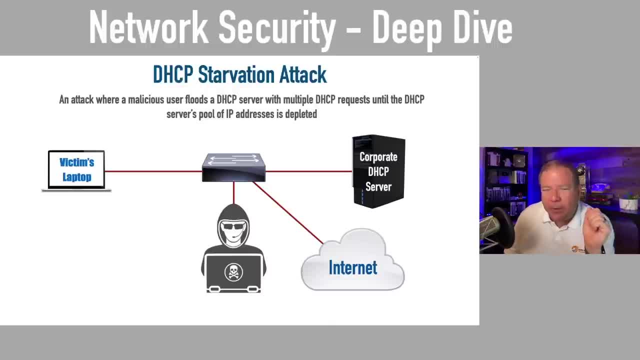 So we don't want to have a rogue DHCP server be believed. But here's one way that an attacker might launch a DHCP starvation attack, Sort of like using all the MAC address space in the MAC address table with the MACAWB utility. the attacker might use a utility. 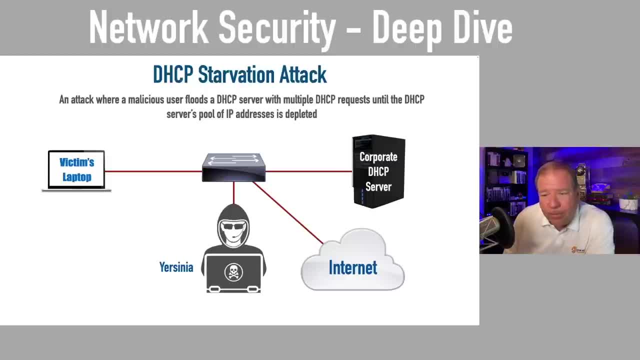 called Yersinia. that comes with Kali Linux And this Yersinia utility can send just a flood of DHCP discovered broadcasts out on the network And those might reach the corporate DHCP server and they say, yeah, I'm a DHCP server. 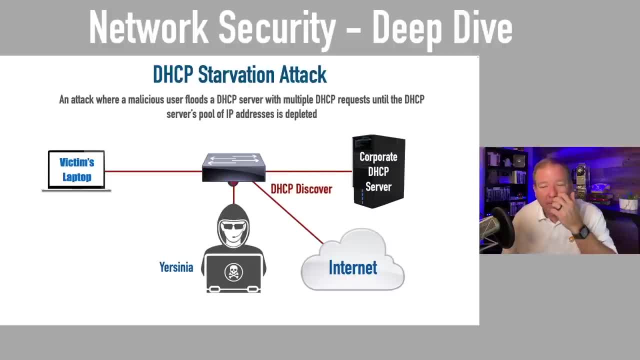 And we could say, all right, give me an IP address and here's my MAC address. So kind of like that MAC address flooding attack. we're sending a bunch of traffic again into that DHCP server saying: give me an IP address. give me an IP address because I'm giving all these phone numbers. 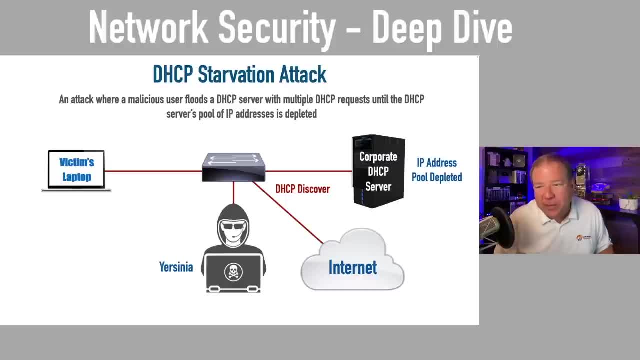 Mac addresses. Well, that corporate DHCP server. it's only got so many addresses in a pool to hand out And in a matter of just a few seconds we could completely deplete that pool. So now if somebody, if the attacker, adds a rogue DHCP server to the network, what's going to happen when a 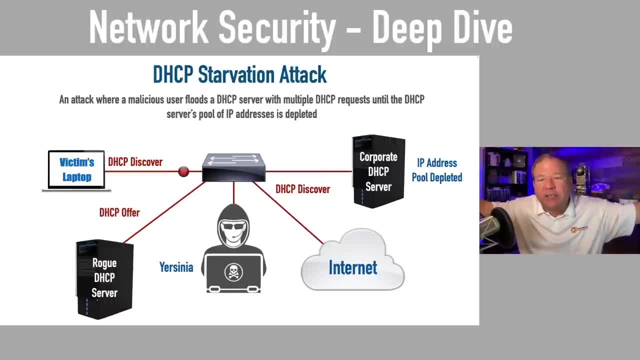 laptop boots up, It's going to send out that DHCP discover broadcast saying, hey, are there any DHCP servers out there? Well, the corporate DHCP server is not going to respond because it's full. It has no addresses to hand out, But the attacker's newly introduced rogue DHCP server it's going to. 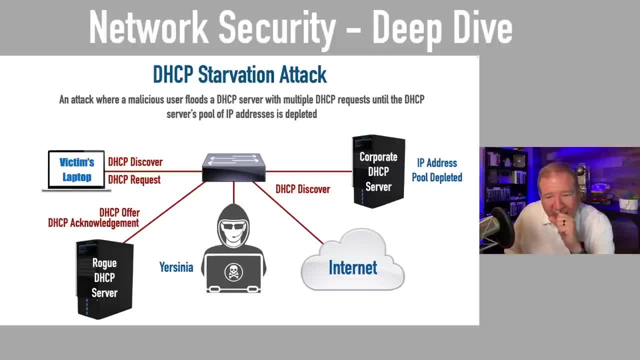 respond, And that's going to be an issue for us- And then the victim might be told to come to the attacker first, as their default gateway, The attacker captures the traffic and then the attacker forwards the traffic out to the internet. A defense against this? and I'm going to show you. 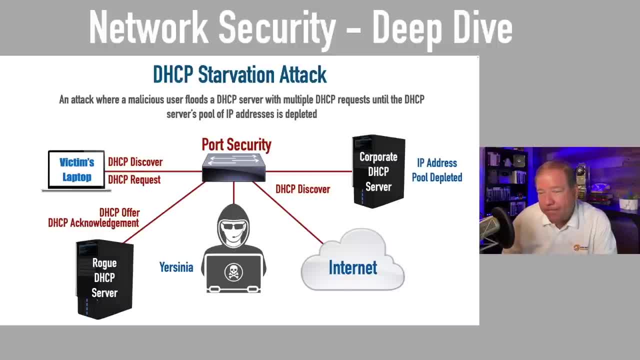 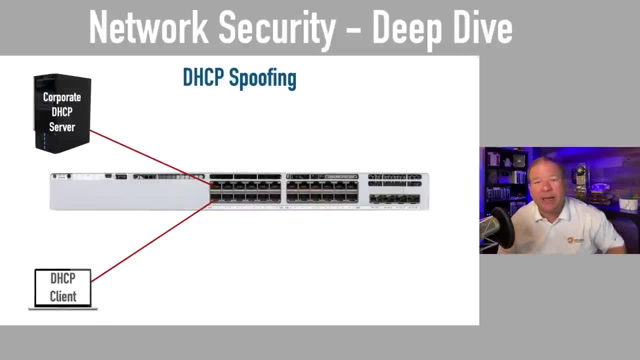 a defense against this is port security- Port security, which is also going to be how we defend against that MAC flooding attack. Another type of DHCP attack is DHCP spoofing. This is similar and it can be used in conjunction with the DHCP starvation attack. But let's take a moment and review. just make sure we're all on the same. 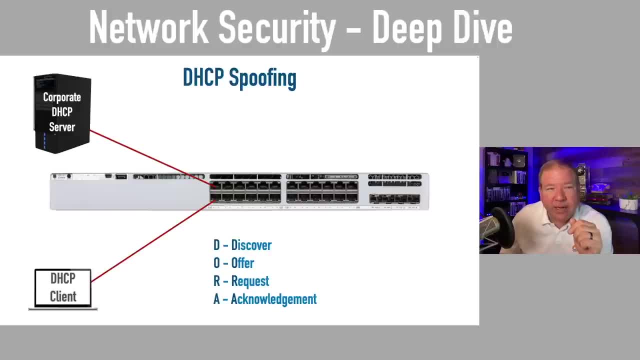 page how DHCP works. If you ever watched Dora the Explorer on- I think it was Nickelodeon, my daughters used to watch that when they were young, But Dora had, there was Backpack and Map and maybe there was a new Dora, like some sort of lost gold temple. I forget the name of it, But 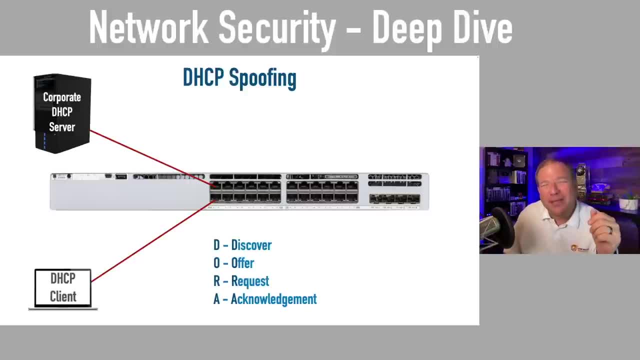 there's a live action Dora the Explorer movie. that came out And I thought, oh, I bet that would be cool. It's like Indiana Jones, only with Dora the Explorer. I know my kids love that. That'd be fun to watch. Yikes, I made it about: okay, here's my movie review. Don't watch it. I made it about 10. 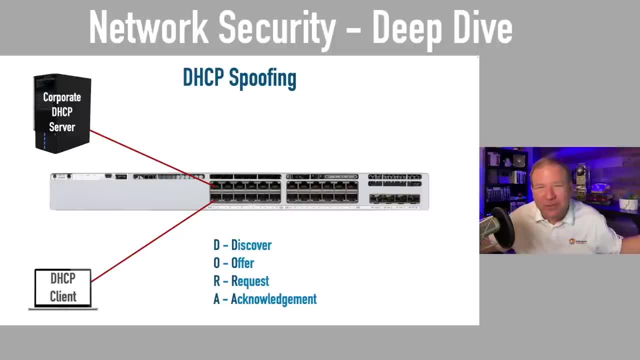 minutes and it was so boring I couldn't stand it. Maybe it's made for children. Maybe that was my bad, but did not enjoy the movie. But in general I got fond memories of my little girls watching Dora back in the day And I think of Dora every time. I think of DHCP. 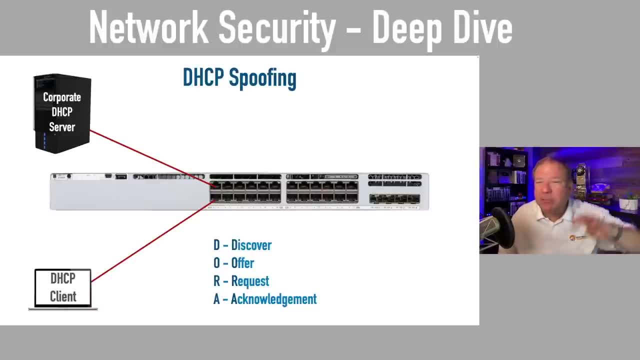 because Dora D-O-R-A. that reminds me of the four-step process of how we get an IP address. The D is the discover. We send out a broadcast saying, hey, are there any DHCP servers out there? And every DHCP server that hears that discover broadcast is going to respond with the O in Dora. 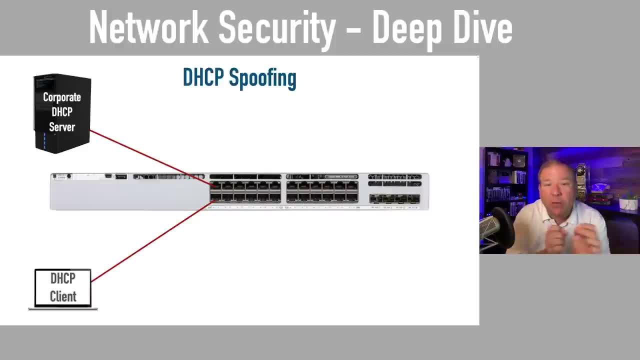 and offer saying yes, I'm a DHCP server And whichever offer we receive first, if there are multiple responses, that's what the client's going to use. It's going to then send the R in Dora a request saying: could you give me some IP address? 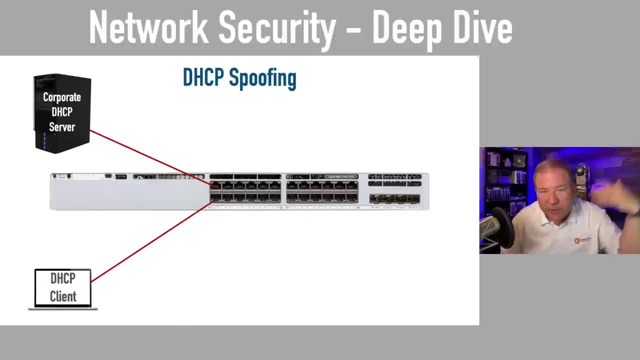 information. And then that server responds with the A in Dora, the acknowledgement, saying: yeah, here's all your IP address information, Here's your address, Here's your subnet mask, Here's your default gateway, Here's your DNS server, and on and on and on, And normally the client is going. 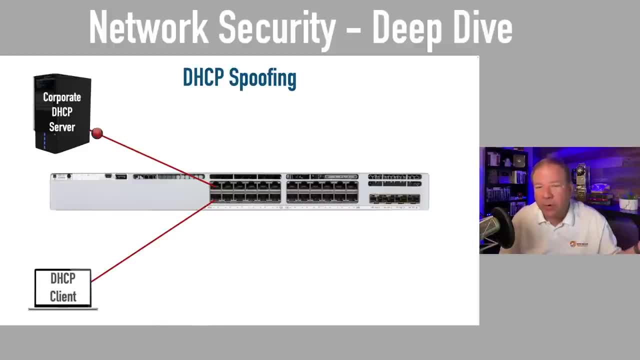 to send out the discover broadcast. It's going to go to the corporate DHCP server. It's going to say: yes, I'm a. I'm a valid DHCP server. Feel free to use me for your IP addressing needs. The client's going to say: okay, I would like to formally request some IP address info. 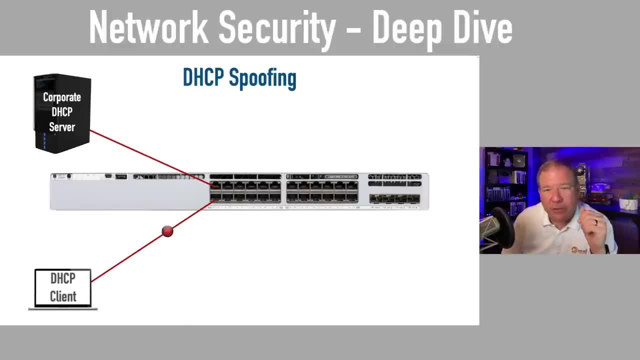 And the server is going to give it to us in the form of an acknowledgement message. But what if an attacker attack attaches their rogue DHCP server to this switch? When the client sends out its DHCP broadcast, it's going everywhere within the subnet. Or if we have a DHCP relay agent set up, it might be going to a different subnet. 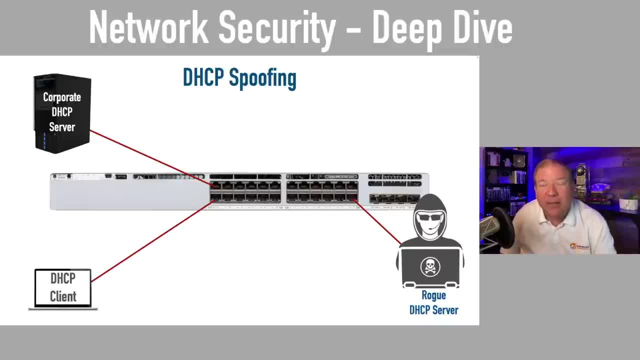 but we're. the rogue server attaches to the same subnet that the corporate DHCP server is attached to, and it receives the discover broadcast as well. Now, not every time, but a percentage of the time its offer message might reach the client before the 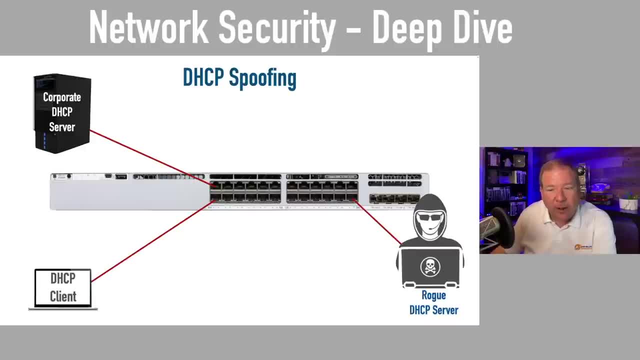 offer message from the legitimate corporate DHCP server And since, in this case, the client received the rogue DHCP server's offer message first, it's going to say: all right, I'm choosing you because you're quick on the job, We're going to ask you to give me information and we're giving false. 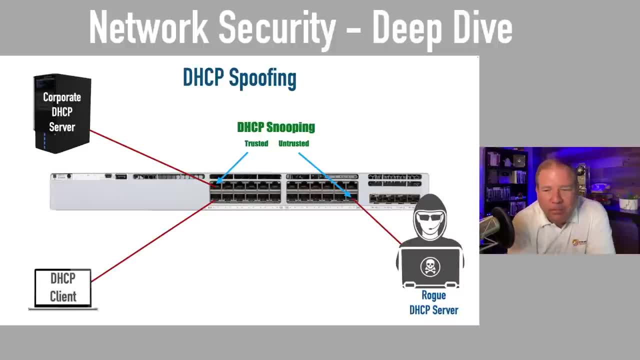 information. How do we protect ourselves against that? Well, we can set up a feature called DHCP snooping on our Cisco Catalyst switches. What we do there is: we say what port is trusted and what port or ports are untrusted. We'll say that a port is trusted if it does connect out to 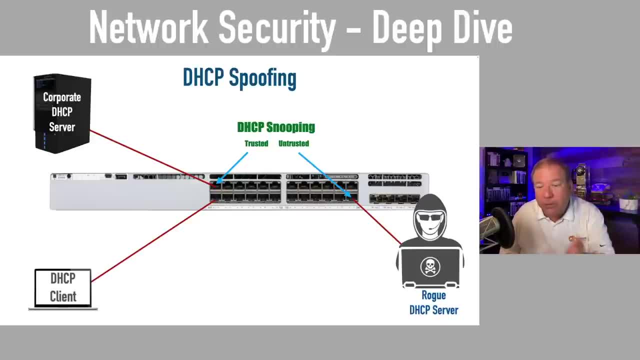 our legitimate DHCP server. So here the first port on the switch that connects to my legitimate corporate DHCP server and we'll say it's trusted. Everybody else is going to be untrusted. Now what does untrusted mean? Untrusted means if I receive a DHCP offer message coming into this port. 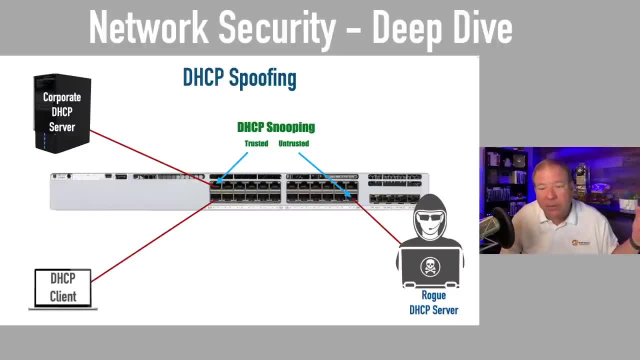 it's going to be dropped if it's untrusted. So in this case, the discover broadcast goes out. both DHCPs- the good one and the bad one- they both respond. But when the offer message from the attacker tries to come into the switch, bam, it's going to be dropped because it is coming. 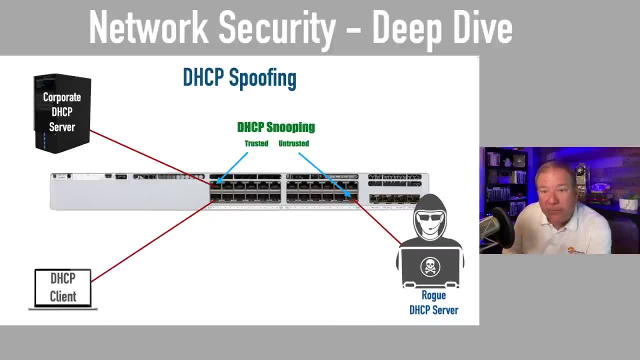 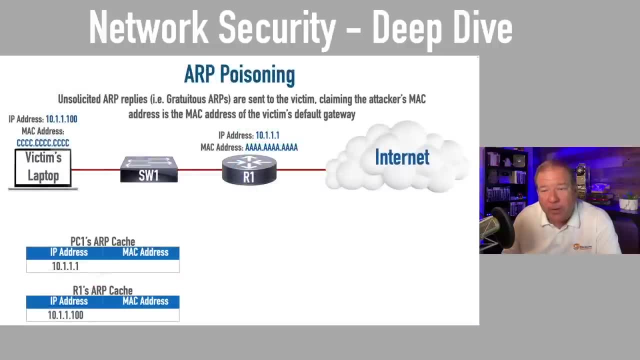 trying to come in on an untrusted port, And I'm going to show you the live interface in just a few moments. In fact, we'll configure it on this switch. I'll show you how to set up DHCP snooping. I think you'll really enjoy that. Another way that an on-path attack might be. 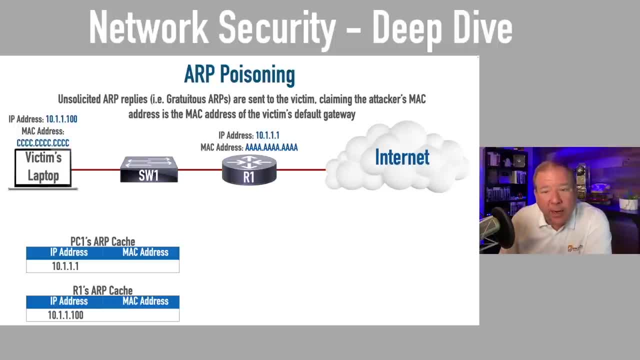 launched is with ARP poisoning. Remember how ARP works. when a PC gets its IP address information and it wants to go out to the internet, for example, It knows- in this case the victim's laptop knows- that its default gateway is 10.1.1.1.. But the very first time it tries to, 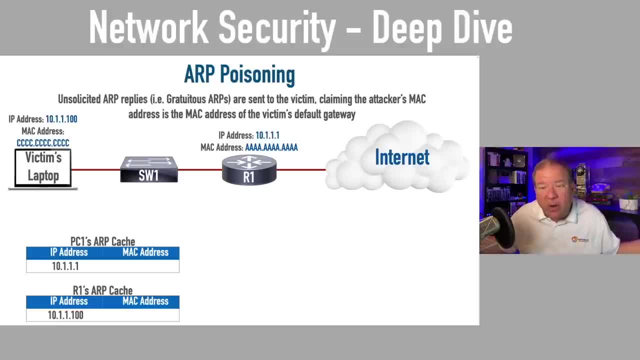 get to 10.1.1.1,. it doesn't know the MAC address of 10.1.1.1.. How does it learn it? It learns it by using an ARP, an address resolution protocol broadcast. It says, hey, can anybody tell me? 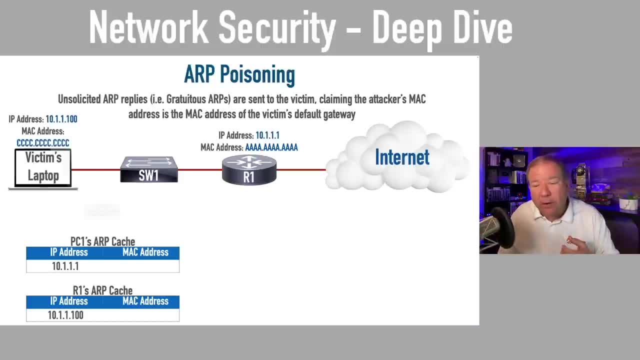 the MAC address of 10.1.1.1?. And the router says: oh yeah, that's me, I have the MAC address of all A's. we'll pretend. And, by the way, that frame that came in from the victim's laptop. 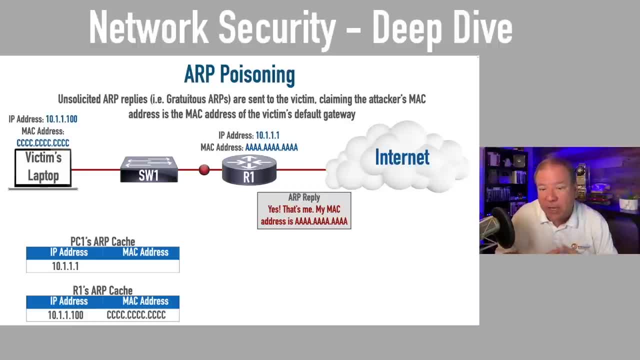 it came in from the victim's laptop MAC address of all C's. So the router just updated its ARP cache to know that the victim's laptop- at 10.1.1.100, it's got a MAC address of all C's. 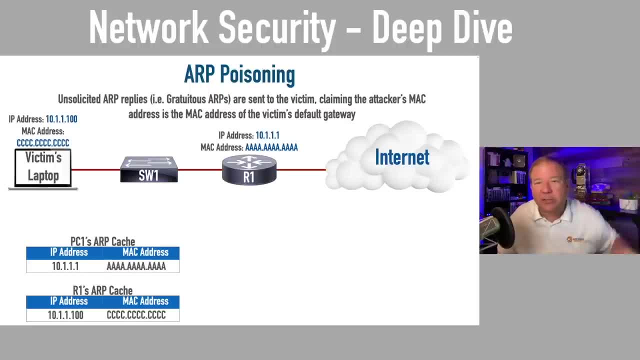 Well, the router responds and says: yep, I'm the old A's MAC address, I'm 10.1.1.1.. And the PC says, thank you very much. And the PC updates its ARP cache. So now the laptop and the router. 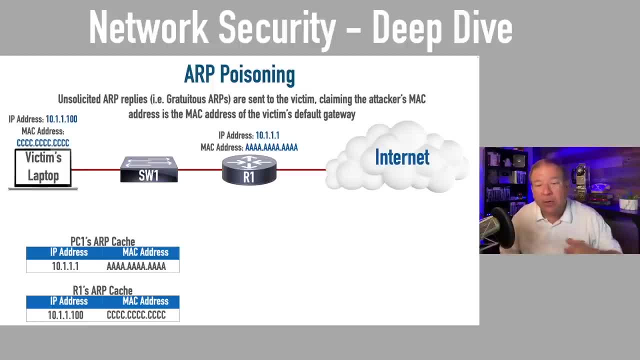 they know one another's MAC address, and the laptop sends a frame to the MAC address of default gateway, which is then going to get it out to the internet. What if an attacker comes along, though, and that attacker is able to convince both the PC? 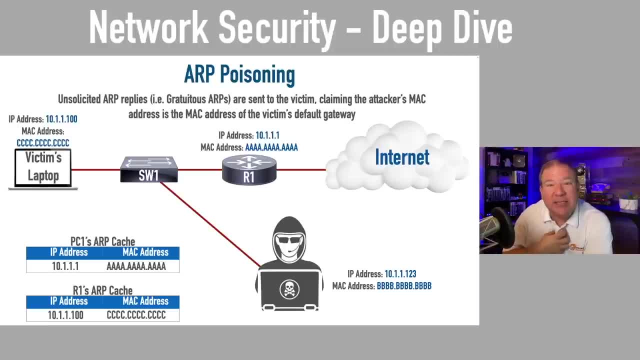 and the router that traffic should be sent to it. Here's what I mean: The attacker is going to send what are called gratuitous ARP replies. In other words, the PC is not asking for MAC address information. It's good, It's populated, It's IP, it's ARP cache, It's all good. 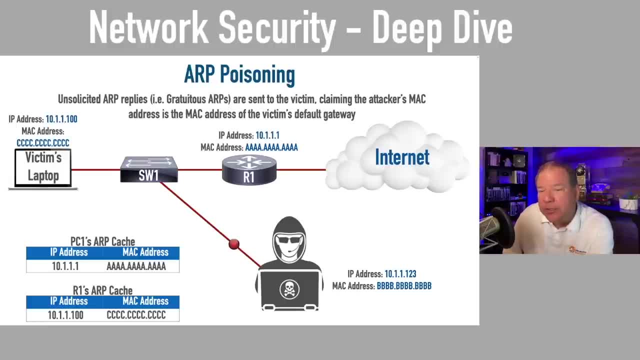 But the attacker sends unsolicited or gratuitous ARP replies saying: ahem, Now the attacker also wants to convince the router that it is the laptop. So it's going to send a gratuitous ARP to the router saying 10.1.1.100,- that's me, I've got the old B's MAC address And the router says: 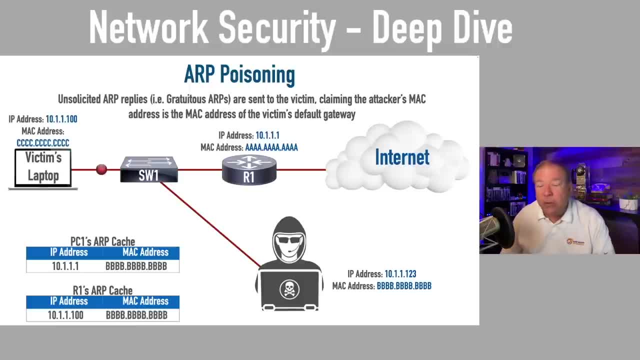 oh, thanks for the update. And it updates its ARP cache. So now, by just lying about this, the attacker has logically injected themselves into this path and traffic going between the PC and the router, As you can see, it's flowing through the attacker's laptop, where they might. 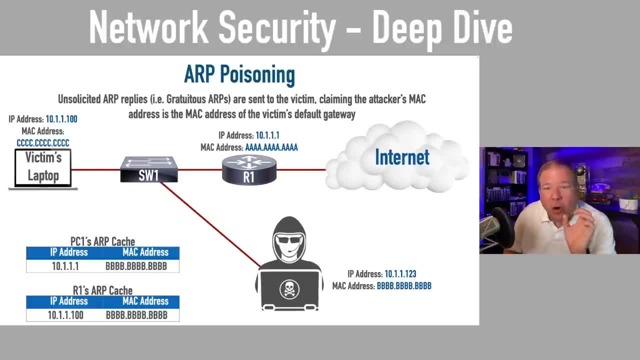 be capturing traffic. They might be altering traffic. They might be altering traffic. They might be altering traffic. This is called an ARP poisoning attack. And I'm going to show you. there's a feature that works hand-in-hand with DHCP snooping, called dynamic ARP inspection. that can prevent. 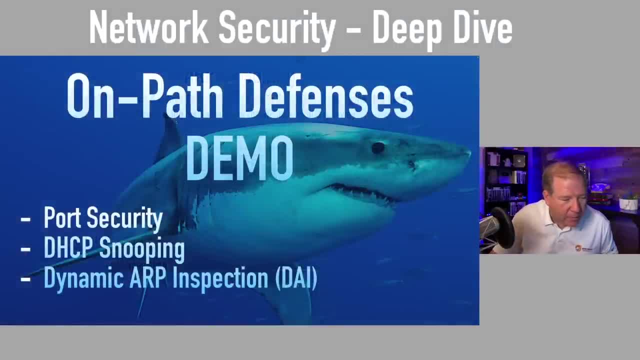 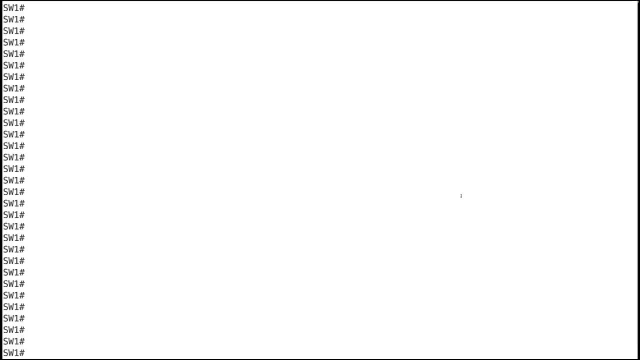 this type of thing from happening. In fact, let's go out to a live interface right now. I'll make this full screen so you can see it a bit better. And here we're sitting on a Switch: SW1.. That's the Cisco Catalyst 2960 CG that I've been showing you throughout today's session, And let's set up. 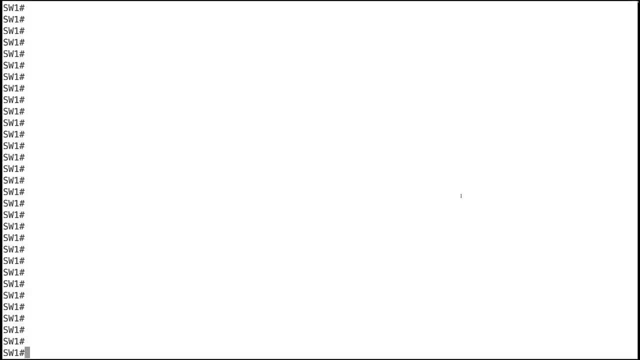 these three features. First of all, is port security. That's going to help us defend against that MAC flooding attack. It's going to help defend us against the DHCP starvation attack as well. What it does, it's going to limit the number of MAC addresses that can be learned off of a single interface. 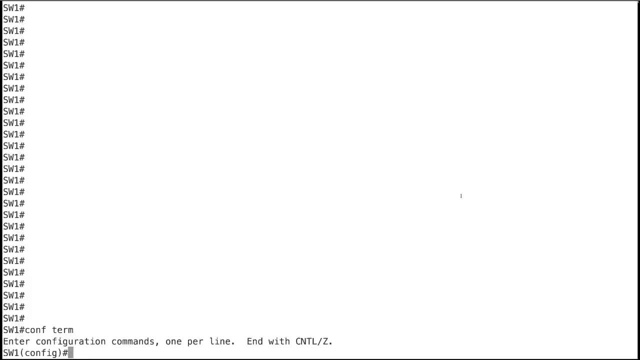 Let's go into global configuration mode And let's just set up the first port on the Switch. Let's go into interface gig 0, slash 1.. And there's a requirement of a port to do port security And it must be an access port. So I'm going to say switch port mode access as opposed to dynamic or 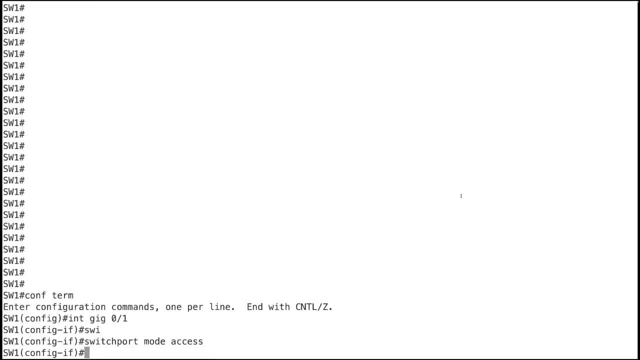 as opposed to trunk. It's going to be an access port. Now I can turn on port security with the command switch port port hyphen security. Now with port security, we said that we could specify the maximum number of MAC addresses that are learnable off of a single port. Let's set that to. 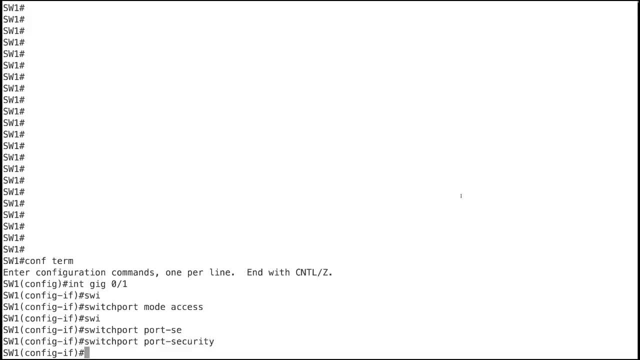 I don't know. Sometimes we're running virtual. I've run a lot of virtual machines on my Mac. If I want to run like Microsoft Windows 11,, for example, I like to give myself about four or five MAC addresses per port, just to account for. 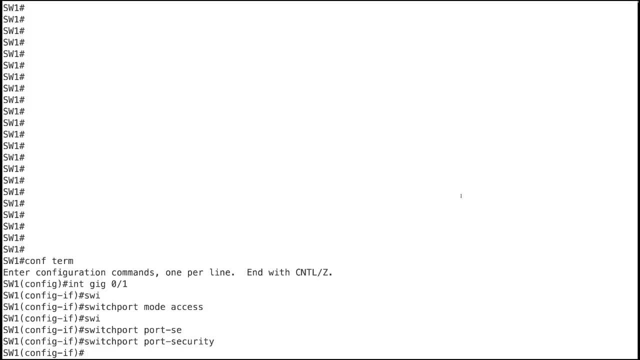 things like that. So let's set this up to allow, let's say, four MAC addresses. I'll say switch, port, port security, still in interface configuration mode, And I'll say maximum. no, let's say maximum four. I'll allow four MAC addresses to be learned. And now that we've said we're going to learn a, 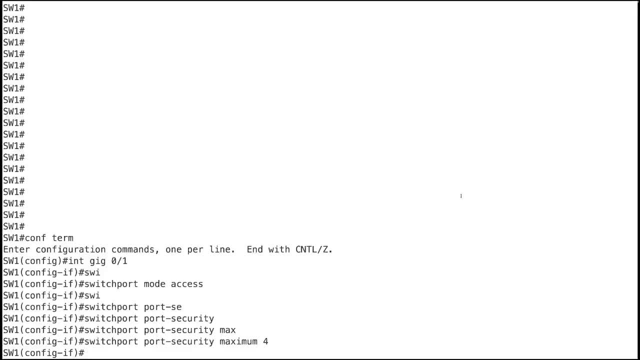 maximum of four MAC addresses on this port. the next step is to set up a port security. The next decision we have to make is: what if a fifth MAC address shows up? How do we respond to that? Well, we've got options. We could say what our violation action is going to be, And I'll show. 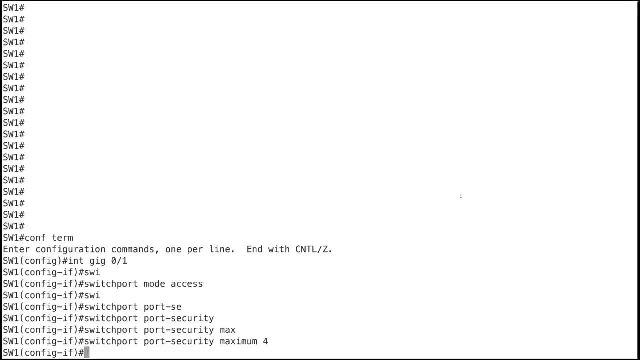 you that in just a moment. but I want to show you something else. first, Those maximum, the maximum number of MAC addresses. do they have to be specific MAC addresses? Well, they could be. Let me show you. I could say switch port, port, hyphen security, and I could give a series of MAC. 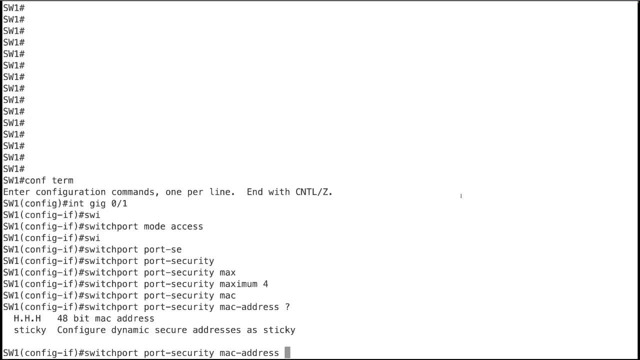 addresses. I could say MAC hyphen address, And I could configure one MAC address. I could enter the command again to configure another one, and another one, and another one. I could. that's a lot of work. I probably don't want to do that. 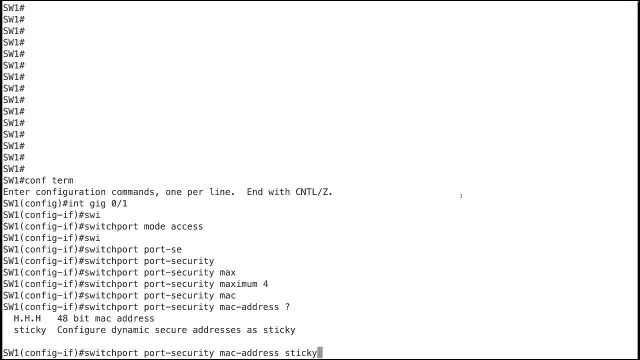 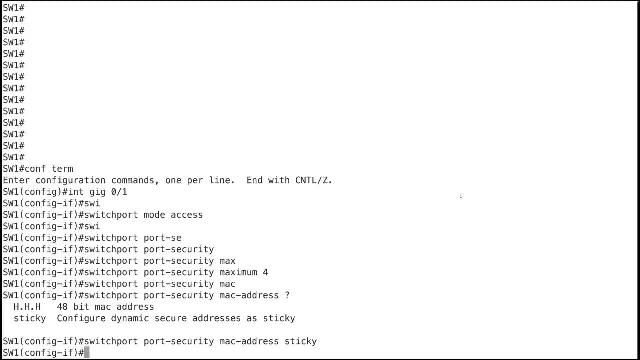 manually. What I can do instead is say sticky. If I say sticky, then it's going to dynamically learn the first four MAC addresses that it sees on this port and it's going to put it in the running configuration. So later, after that's happened, maybe I come back the next day and I save my 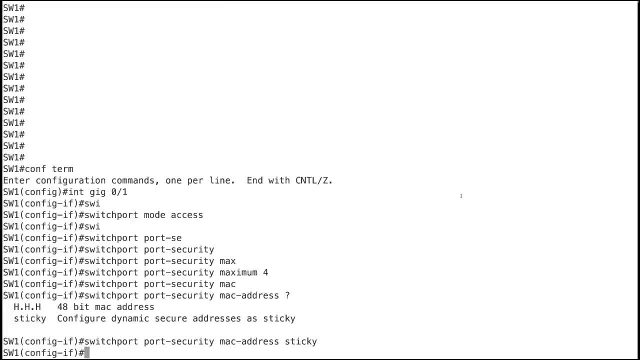 configuration. It's the first four MAC addresses that we're learning And then I can say: sticky learned. So we'll assume those are the four MAC addresses that should be on this port So we can manually configure them. We could sticky learn them or we could just let whoever the first. 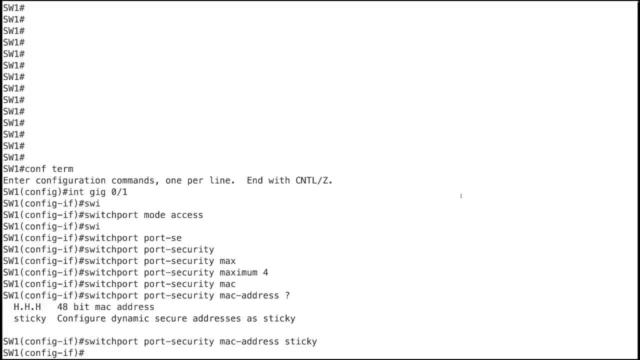 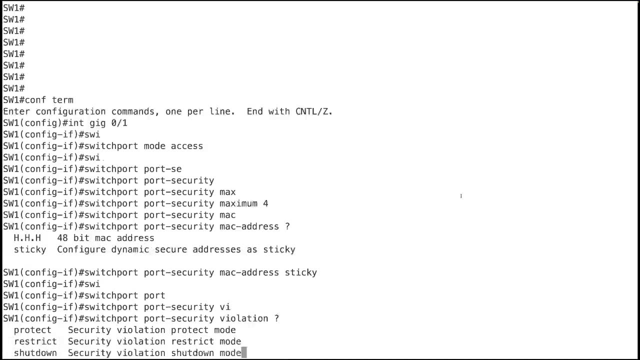 four are be the first or be the four that are allowed. But I was hinting a moment ago at making a decision as to how we respond to a violation. What if a fifth MAC address shows up? Well, what's our violation options? Let's say, switch port, port hyphen security violation. 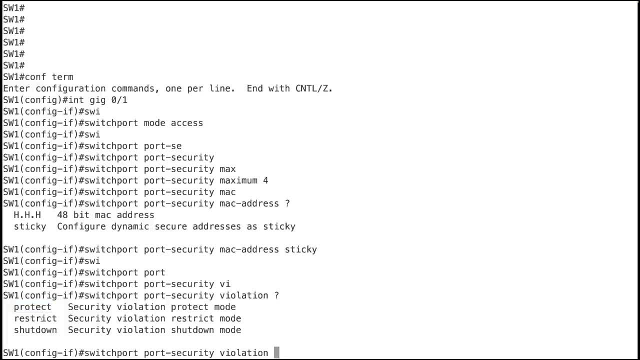 I've got three options: protect, restrict and shut down. First of all, let's let's talk about protect Now. protect says in this case I'm learning- a maximum of four MAC addresses If a fifth MAC address shows up and tries to send traffic into that switch- traffic coming from. 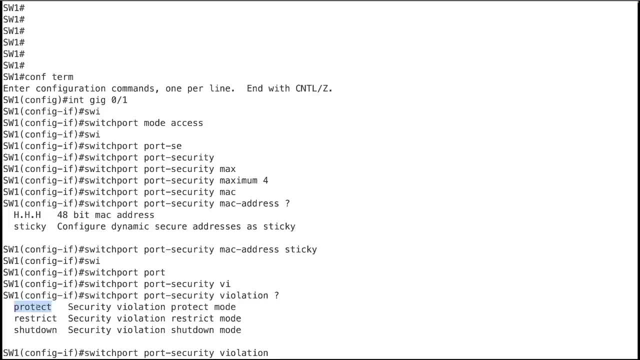 that fifth MAC address. we're going to drop traffic from it. Everybody else from the other four MAC addresses- we'll leave those undisturbed so that nothing gets interrupted. We'll just block traffic from that fifth MAC address. that shows up The restriction. 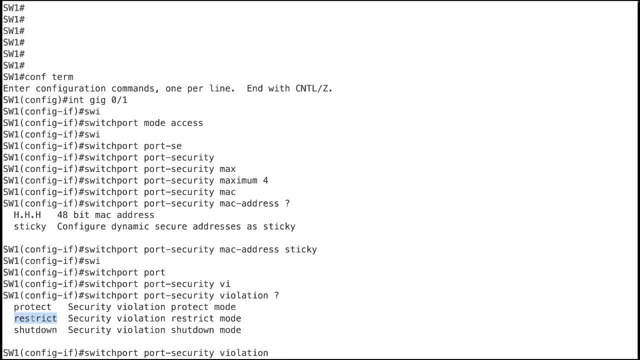 restrict option is very, very similar to protect. With restrict. we're still going to drop frames coming from MAC address number five or MAC address number six. We're still doing that. We're still not interrupting anybody else, but we're going to increment something called the switches security. 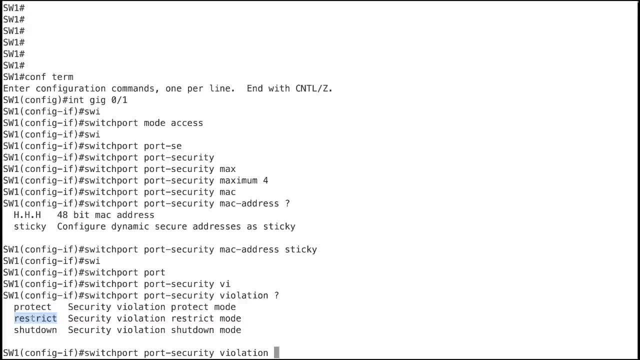 violation counter. So there's going to be a log that a violation did occur. We're not interrupting the first four legitimate MAC addresses, but at least we'll have a record that a violation did occur. I'll show you how to how to view that here in just a moment. But 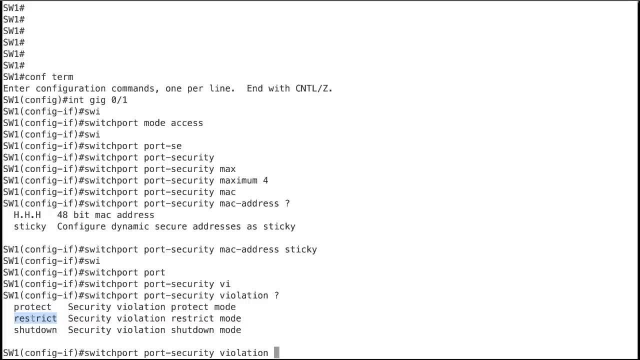 in fact, let me just show you that right. Well, I'll show you after I give the violation option. but I'm going to say my violation option is restrictive. I want to make a log but not interrupt the first four MAC addresses. or I can be very restrictive and say: 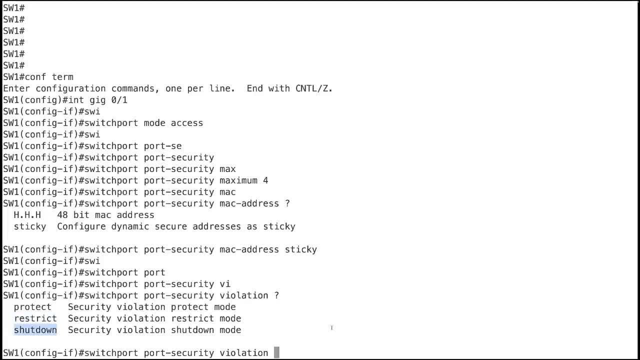 I can say shut down. Shut down says if there is a violation, then something must be up. Something, something's not good in the system. So I'm going to say shut down. So I'm going to block everybody. I'm going to put this port into what's called an air disabled. 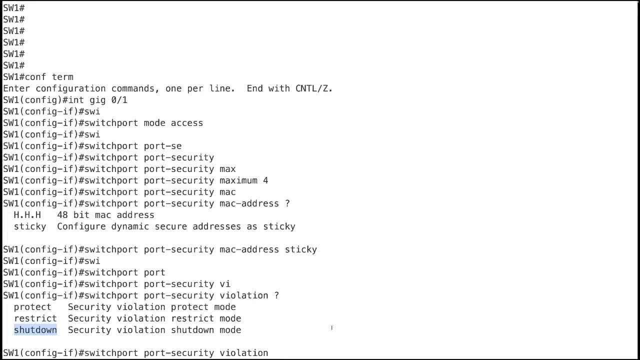 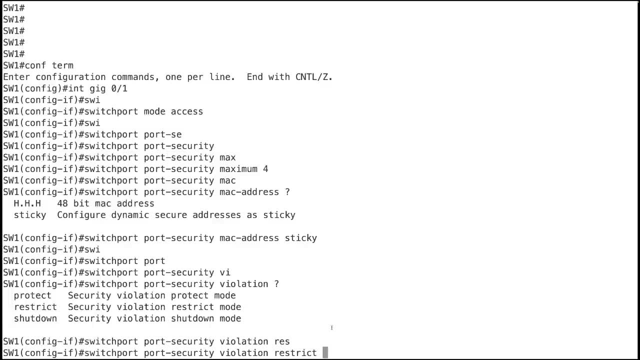 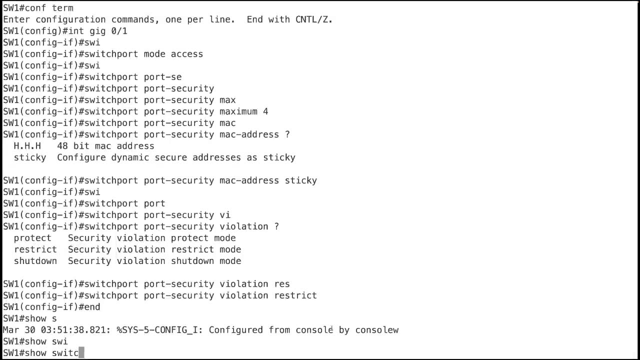 state And we're going to remain in that state until we either, after a period of time, try to come out of that state or somebody bounces the interface. Now I'm going to say restrict- That's kind of my go-to one- And I can say show switch port or actually show port hyphen security. 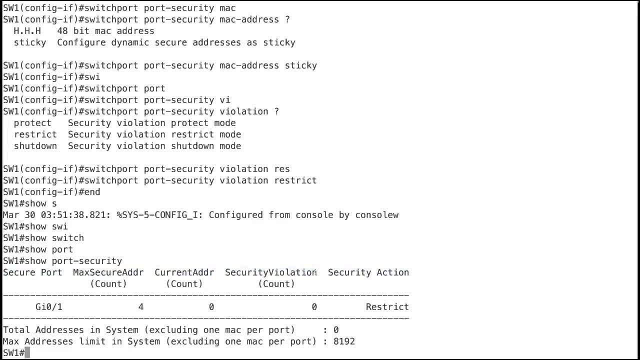 And here's that Security violation counter that I was talking about. So if we did have a violation- somebody tried to exceed the four MAC addresses on port gig zero slash one that would be. that would be recorded here in the security violation counter. So again, that's how easy it is to set up port. 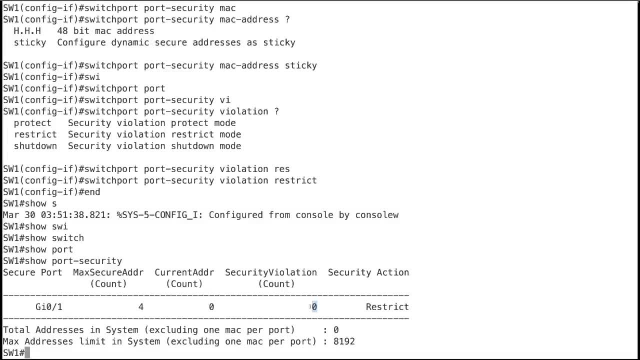 security And that could defend us against that MAC flooding attack. It could defend us against that DHCP starvation attack. Next up is DHCP snooping. Remember, with DHCP snooping we want to say what port we're going to set up. So if we set up port security, we're going to set up port. 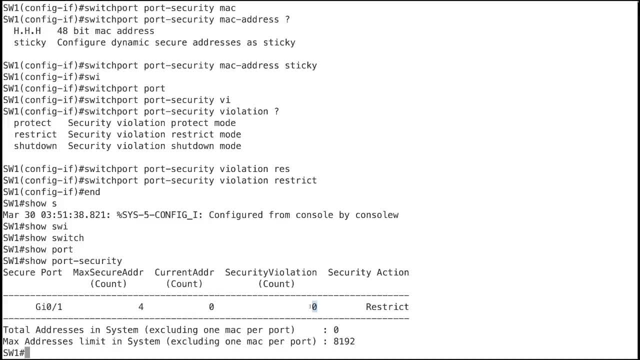 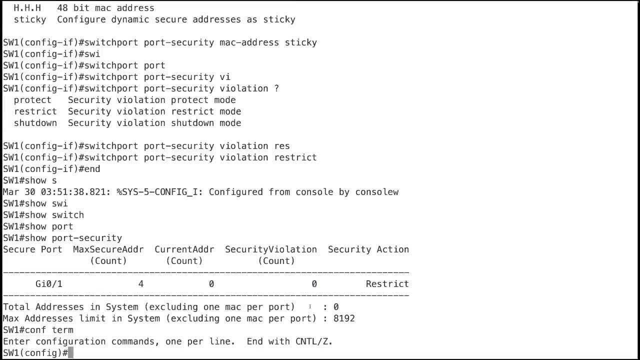 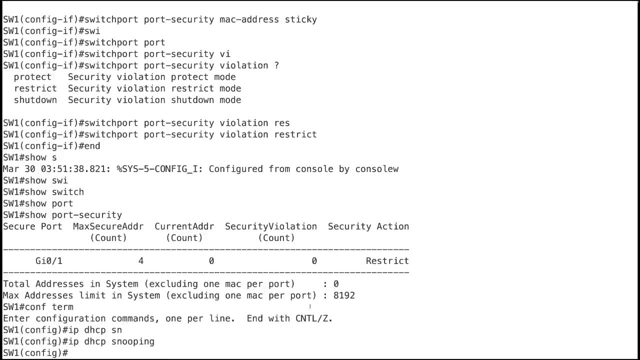 security, And if a port is trusted or untrusted, we're going to drop any DHCP offer packets coming into that port. So here I'm going to turn it on globally. I'll say IP, DHCP snooping and that turns on globally. But the thing is, even though I've turned it on globally, it's not yet active for any. 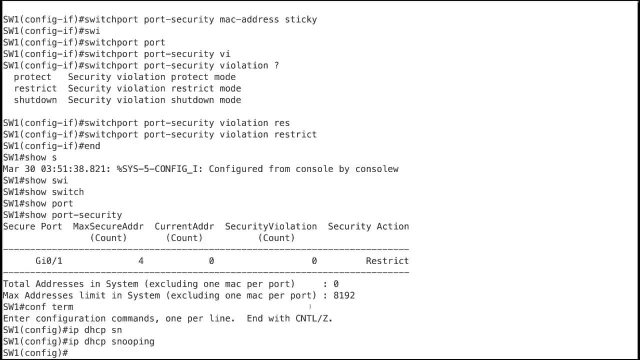 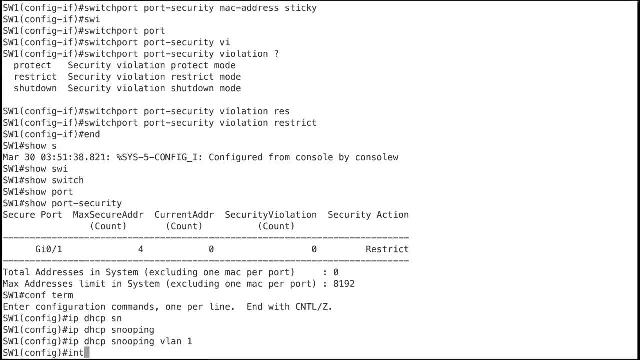 of our VLANs. You have to turn it on for a VLAN at a time. Now, in my case, I've only got one VLAN, It's VLAN one. So I'm going to say IP DHCP, snooping VLAN. And let's go into interface gig zero slash. one again that we were using And I'll say IP DHCP. 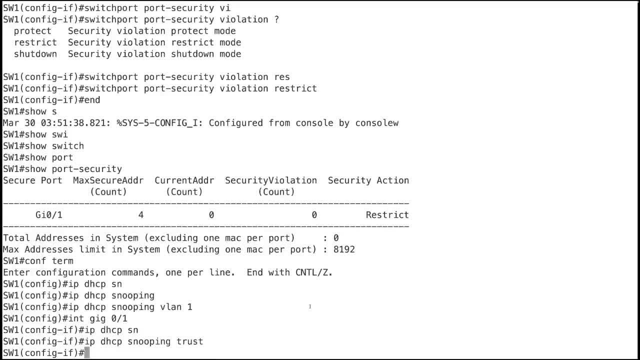 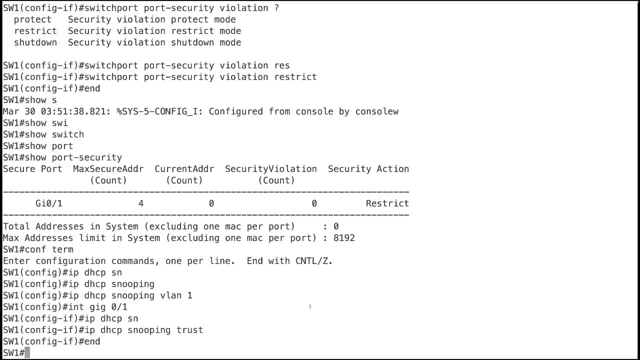 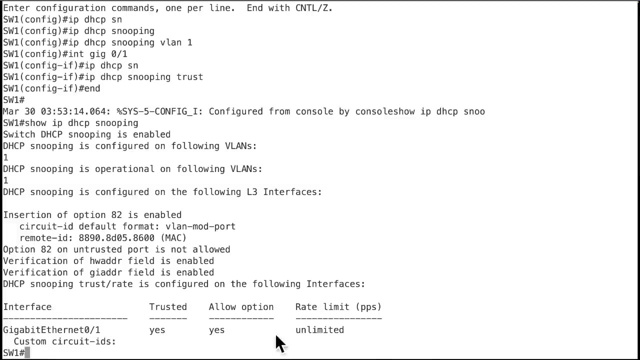 snooping trust. Let's pretend that gig zero slash one that's the port off of which my legitimate corporate DHCP server resides. I can then start dropping traffic that comes in any other port. I can say: show IP DHCP snooping And you can see that I am trusting gig zero slash one. Everybody else is going to be untrusted. 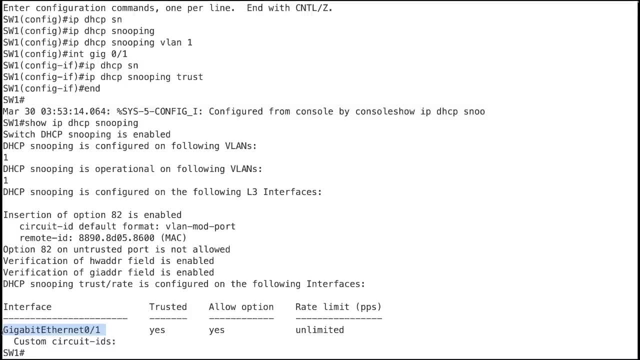 which means I'm going to be dropping any traffic that comes in any specifically DHCP offer messages that try to come in any other port other than gig zero slash one. There's one other feature, By the way. this is going to help fight that DHCP spoofing attack. But remember the ARP poisoning. 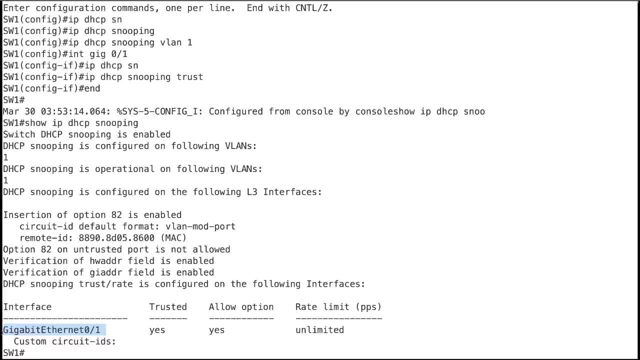 attack. Let's see how we can defeat that or better, defend against it. So let's go ahead and do that. We can use something called DAI, Dynamic ARP Inspection, And with Dynamic ARP Inspection we're actually leveraging a table that gets built with our DHCP snooping configuration. 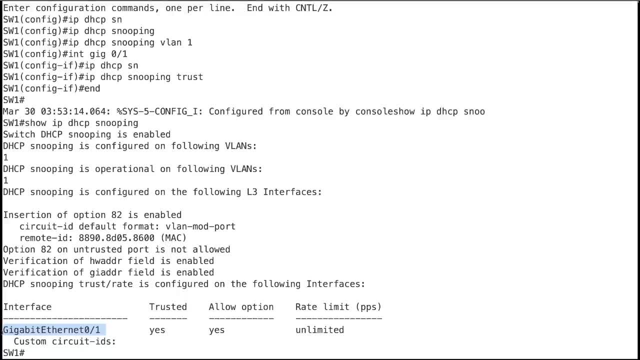 I mean the DHCP snooping configuration that I set up. it was pretty simple. I turned it on, I enabled it for a VLAN and I said what port was trusted. We're done. But in addition to just blocking offer messages coming in other ports, there is a table that it is going to be able to. 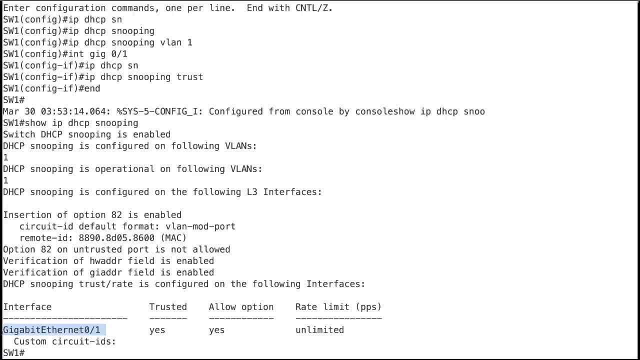 construct in the background And that table is saying what it's snooping in these DHCP messages. It's not just looking for offer messages, It's actually reading the contents of these DHCP messages. It knows that a specific IP address with a specific MAC address lives off of this. 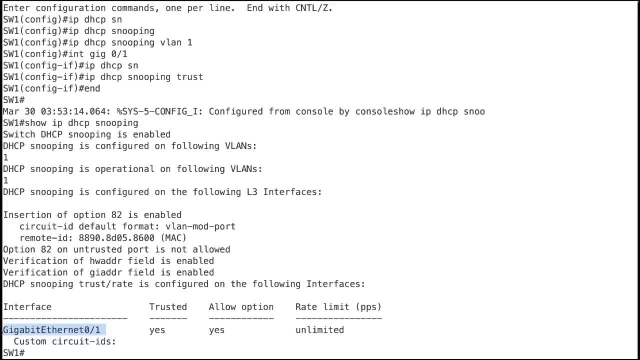 specific port. So it can with Dynamic ARP Inspection. if it starts to receive information that is inconsistent with what has been learned via DHCP, it can drop that traffic. Let me show you I'm going to turn that on. Let's go back into global configuration mode And I'll say: I want. 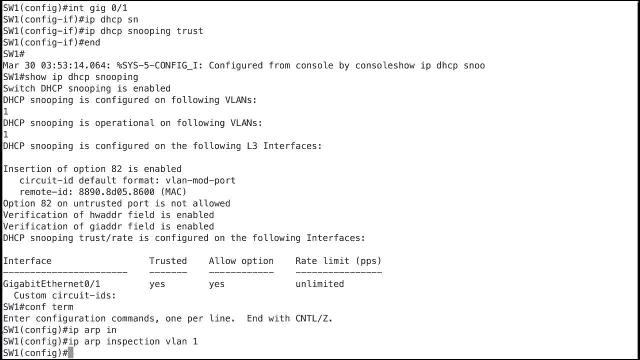 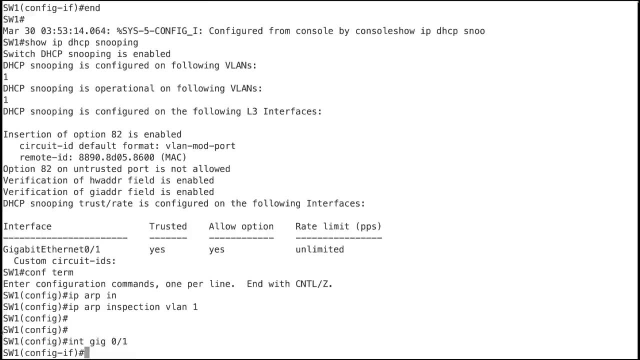 to turn on IP ARP Inspection for VLAN 1.. And let's say that I want to trust just that first port again. I'll say interface gig 0, slash 1.. So don't examine traffic off of this port. I'll say IP ARP. 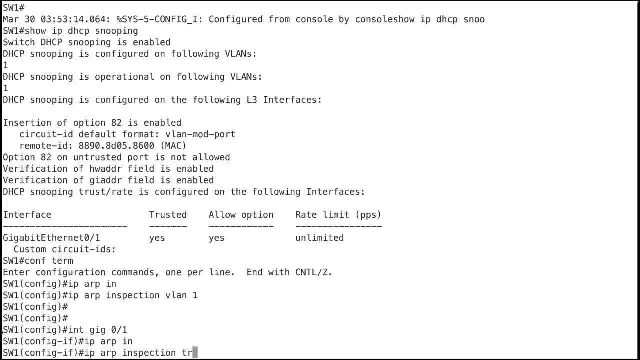 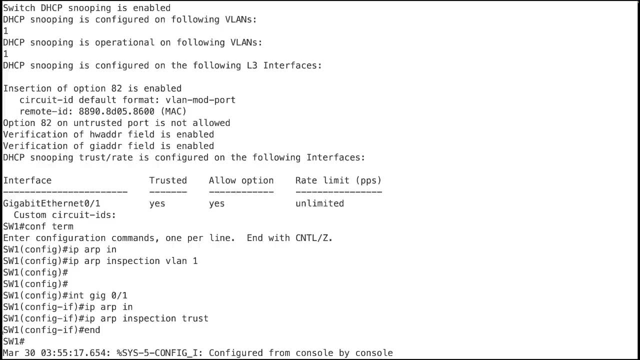 Inspection Trust. Everybody else is going to be untrusted. So now DHCP snooping is going to be snooping that table And if there's information or packets showing up on a particular port that's inconsistent with the MAC address IP assignments that have been handed out by the DHCP server. 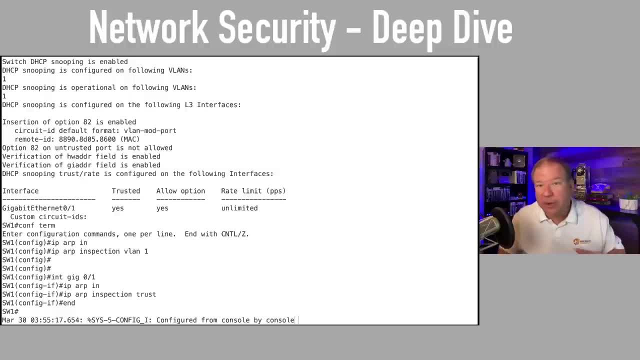 like, if somebody's falsifying their MAC address, then that's going to be denied, It's going to be blocked. So that's a look at three different tools that we can use to better defend ourselves against these kinds of attacks, these on-path attacks. We took a look at how to configure. 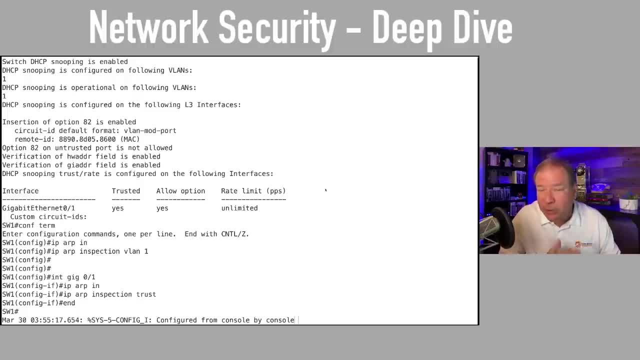 port security. We took a look at how to configure DHCP snooping And build-in. we took a look at how to configure DHCP snooping And build-in. we took a look at how to configure DHCP snooping And build-in. 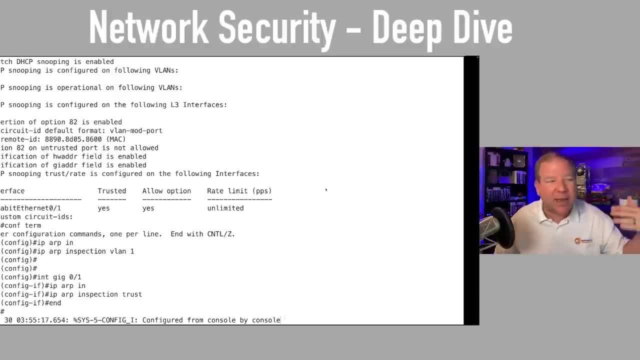 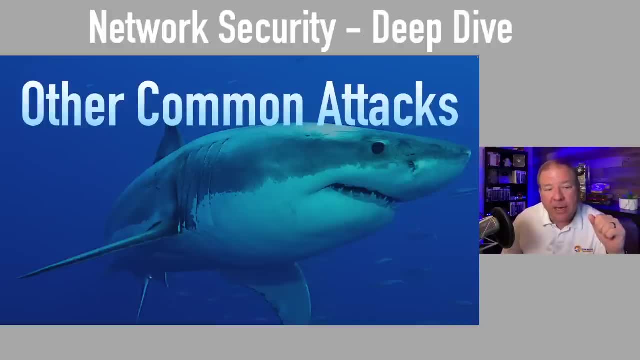 on that. we configured DHCP snooping first, But building on that, we then configured DAI Dynamic ARP Inspection Next up. let's take a look at a few other attacks, And we are going to be taking our first break here coming up in just a moment. I realize we've been going for a while. 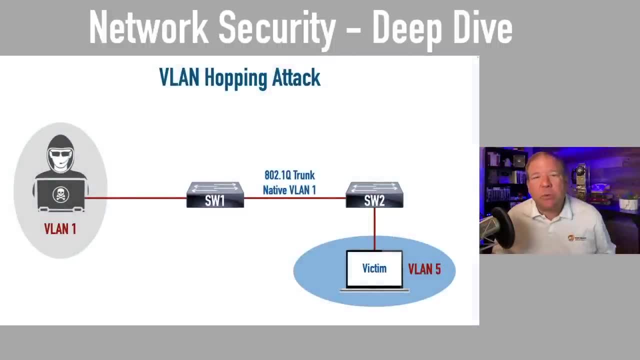 But I want to take a look at a few other attacks first, And the next one is a VLAN hopping attack. With a VLAN hopping attack, an attacker might be trying to get access to a VLAN that might contain some secure server that it should not have access to, So we're going to take a look at that. 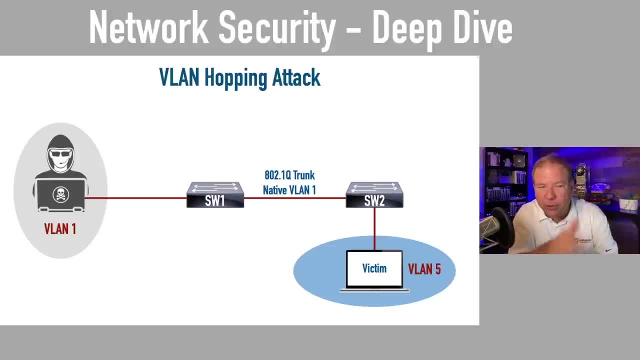 with a VLAN hopping attack. an attacker might be trying to get access to a VLAN that it should not have access to. So there's security in place that says you're not allowed person in VLAN 1, from getting over here to VLAN 5.. One way of getting access to a forbidden VLAN is to do switch spoofing, In other words. 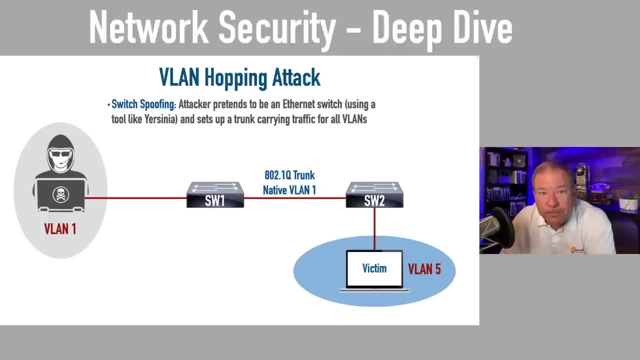 the attacker's machine. it can pretend to be a switch. Do you remember the protocol that's used by a Cisco Catalyst switch to dynamically form a trunk? Go ahead and chat it in. if you remember that, What protocol is used by a Cisco Catalyst switch that can dynamically form a trunk, Go ahead. 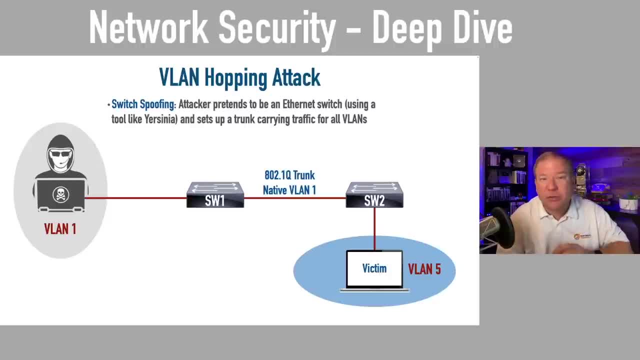 and chat it in. if you remember that, What protocol is used by a Cisco Catalyst switch that can dynamically form a trunk And remember a trunk by default allows traffic for all VLANs to flow over that trunk. Yeah, it's DTP, the Dynamic Trunk Protocol. Great job, The Dynamic Trunk Protocol. So using a 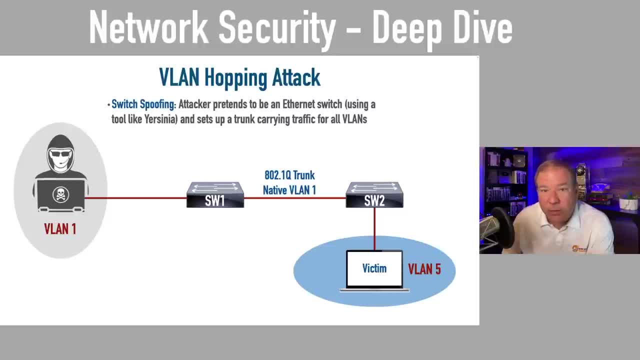 tool like Yersinia. that's one of those tools that's available in Kali Linux or you can install it on other versions of Linux. But using Yersinia, the attacker might send out DTP frames and switch one. in this case. 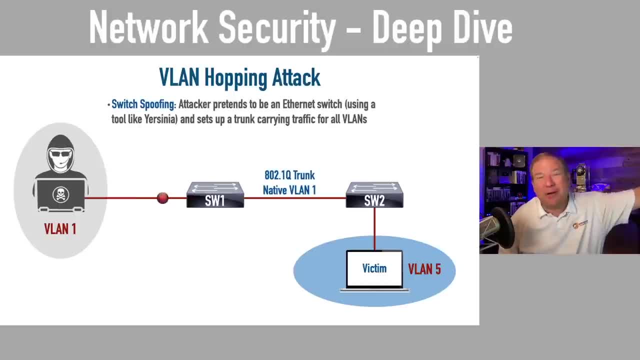 That it's a switch Switch. one says I'm talking to another switch, They just sent me a DTP advertisement. So we form a .1Q trunk over that switch which gives me access to VLAN 5.. I'll just tag my VLAN or tag my frame with VLAN 5.. It goes over to switch. one sends it over to switch two. 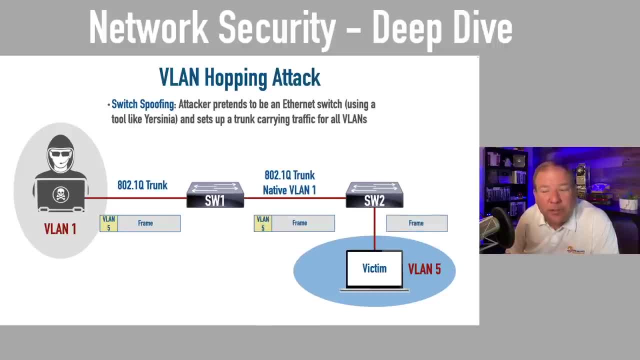 Switch two says: oh yeah, I'll send this at my VLAN 5 ports And we reach the victim. Another option is to do something called switch one. Switch one is a switch, that's a switch. that's a switch. that's called double tagging. So, even if I'm not pretending to be a switch, maybe DTP is turned. 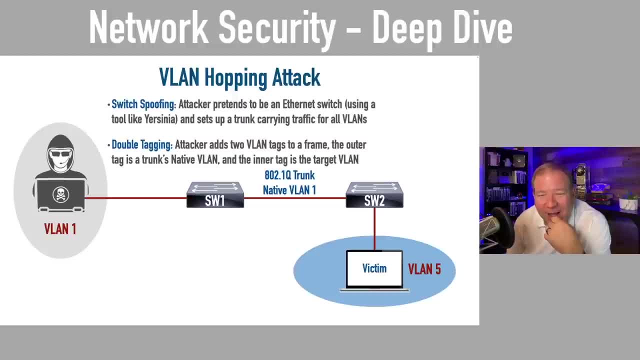 off on a particular port For security? maybe we should, But we could do something, or the attacker could do something called double tagging. if they know the native VLAN, I should say between switch SW1 and switch SW2.. Remember on a .1Q what a native VLAN is, on a .1Q trunk A native VLAN is the one. 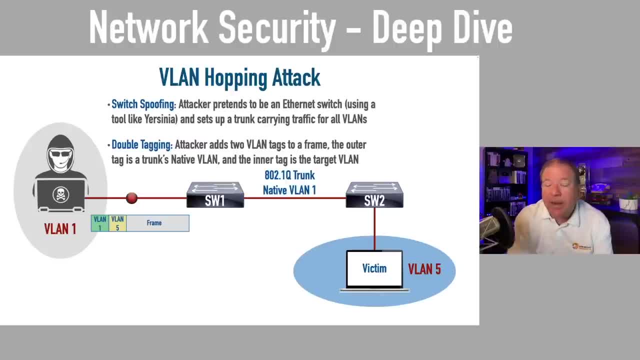 VLAN that does not get tagged Now. by default it's VLAN 1.. But for every other VLAN there's going to be four tag bytes added to every frame And there are a few bits in those tag bytes that identify our VLAN membership. 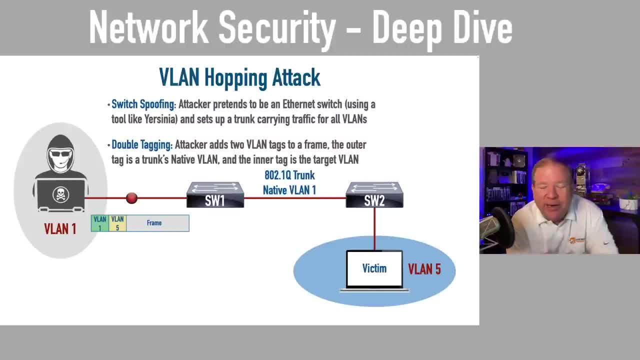 except for the VLAN that we call our native VLAN, And again by default, that's VLAN 1.. So what if we did this? The attacker knows that the native VLAN between switch SW1 and SW2 are there, And so they're going to do a switch switch, And so they're going to do a switch switch. 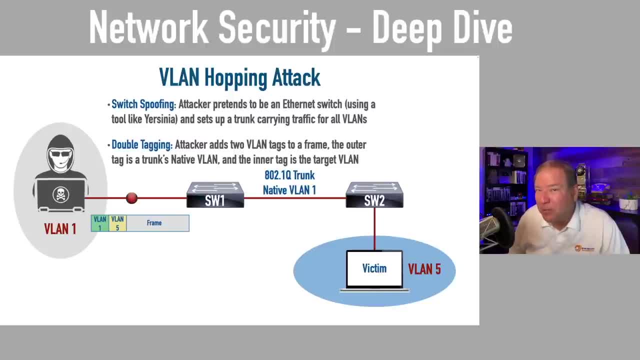 switch, And so we're making a guess that they left it at the default. We should probably change our native VLAN, But they might be assuming that the default VLAN 1 is being used. So what they'll do is they'll take their frame and they'll tag it with VLAN 5.. That's the destination We want to. 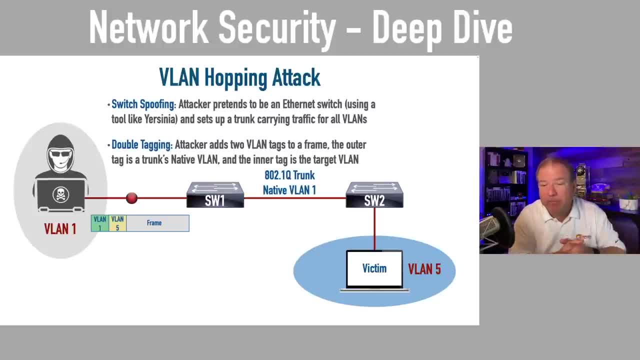 go to VLAN 5. And that's where the victim lives. But we'll put another tag on the outside that says VLAN 1.. So here's what happens. This goes into switch SW1.. It says: oh, I see your tag. 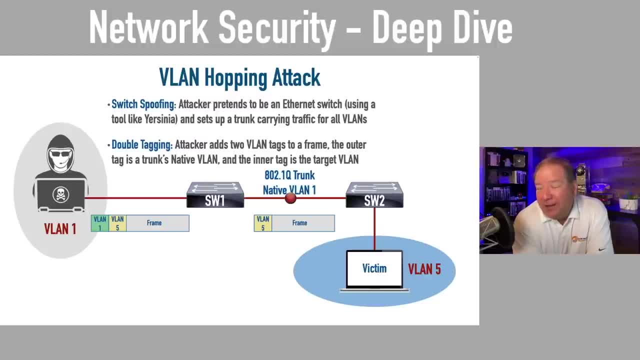 VLAN 1.. That's actually a native VLAN of this port going over to switch SW2.. So let me take that off. We don't label VLAN 1 traffic. We don't add those four extra tag bytes. So now that exposes the VLAN 5 tag, which does make it to the victim system. Now, in this case, unlike with switch, 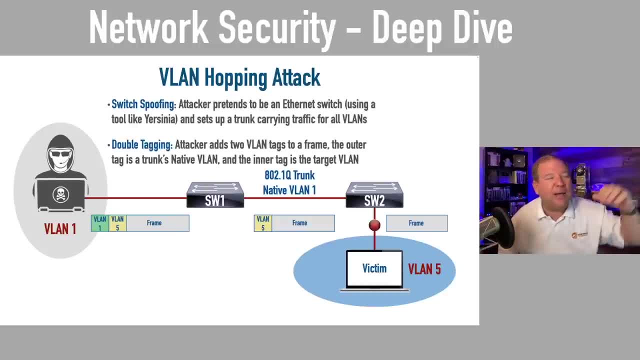 spoofing, there's no return path. If we try to get information from the victim, double tagging is not going to do it for us. Double tagging can get us to that VLAN, but it's not going to allow return traffic to come back. 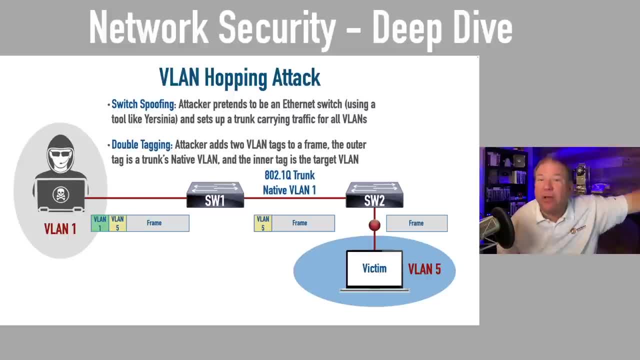 So this might be used for a denial of service attack If we're trying to flood that victim system. the victim belongs to VLAN 5.. We don't have access to VLAN 5.. The attacker could double tag their frames perhaps if they can correctly determine the native VLAN between a couple of 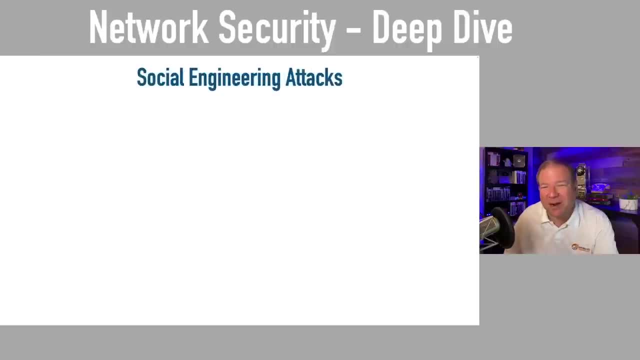 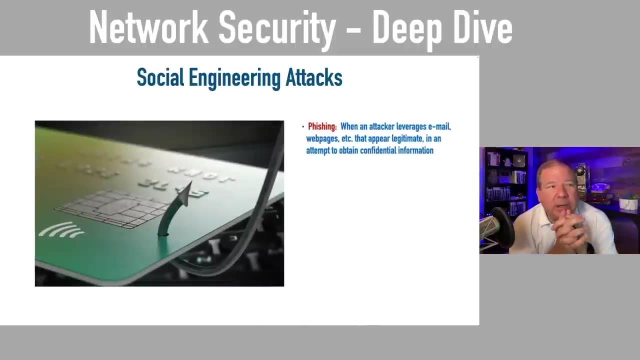 switches And they can start flooding that victim with lots and lots of traffic. Another very, very common type of attack is a social engineering attack. This is where somebody uses basically social skills to get information, to get access to information they should not have access to. In fact, one of my favorite, in fact, it is my favorite. 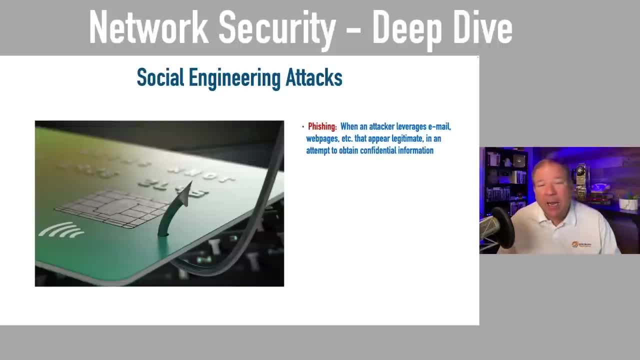 book talking about hacking and phone freaking. It's by Kevin Mitnick. I've got it on audio. I've listened to it. I don't know. maybe three times It's called. it's called Man in the Wires. No. 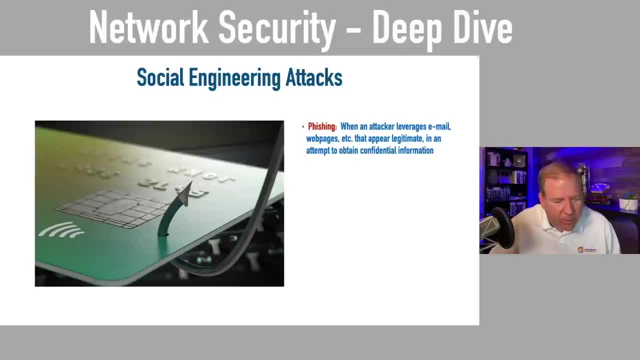 or Ghost in the Wires, In fact, you know what? Let me look that up. I want to make sure I get that right. Yeah, I think it's Ghost in the Wires. Let me open this up really quick. Yeah, I'm a big fan of Kevin Mitnick. I've got a few of got a few of his books. Let's see. 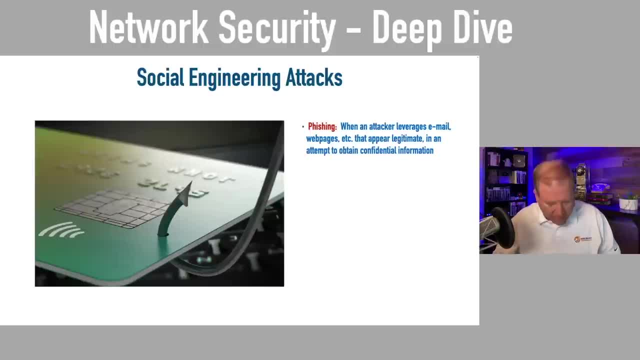 let me just go to Amazon really quick here And let's say I think it's Ghost in the Wires. Yeah, that's it, Ghost in the Wires. I would recommend that book if you want to just hear some real life war stories, if you will, from. he was known as the world's number one most 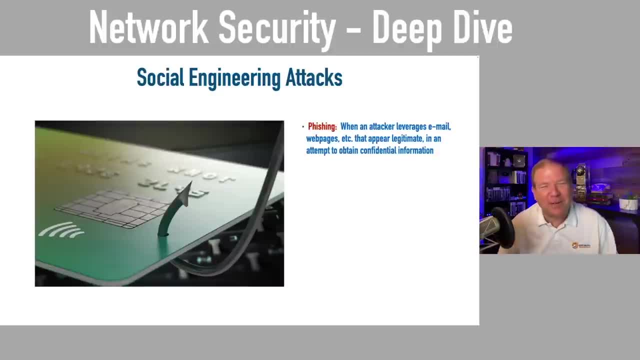 wanted hacker for a while. He's turned good. now He's got a cybersecurity company. but yeah, some really cool stories in there. The reason I thought of him was just a tremendous amount. tremendous number of the attacks that he was able to carry out were based on social engineering. He would 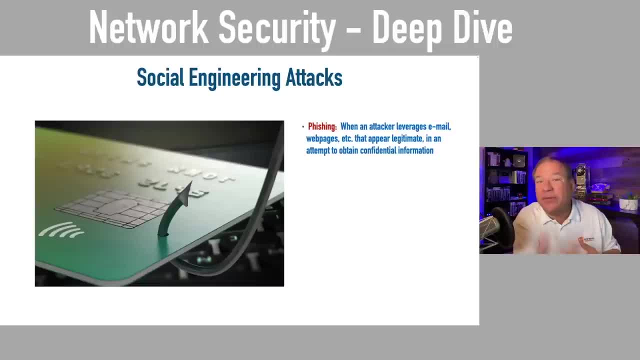 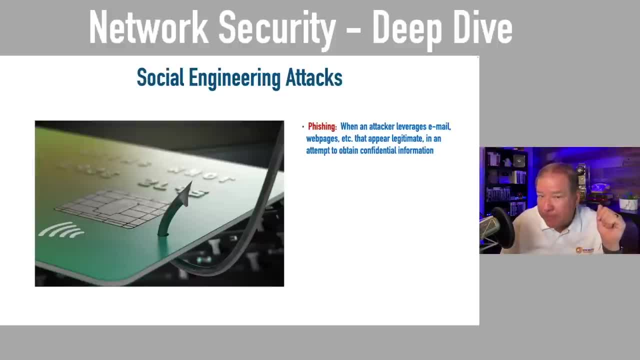 One type of social engineering attack. we see a lot is phishing. You might've received an email that said something like this is your bank and we're going to reset your password. or maybe it's your media or your social media service: We're going to reset your password. You got to log. 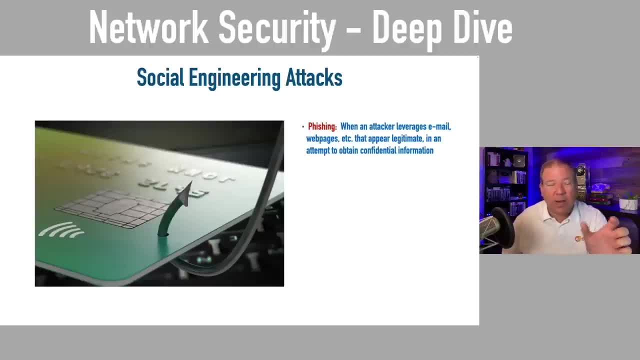 back in and they give you a link to go reset your password And you go to a page that looks like the bank's page but it's really not. It's a page the attacker has and they see you put in your old password and suddenly they have your username and password information. That's phishing We want. 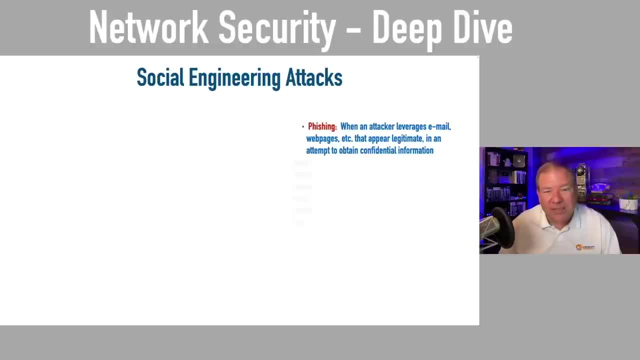 to be very, very cautious about clicking on any links that come inside of an email. We should not be doing that. A physical, a way to get physical access to an environment might be through tailgating. Let's say that there's a secure door where people have to badge in, maybe to get into. 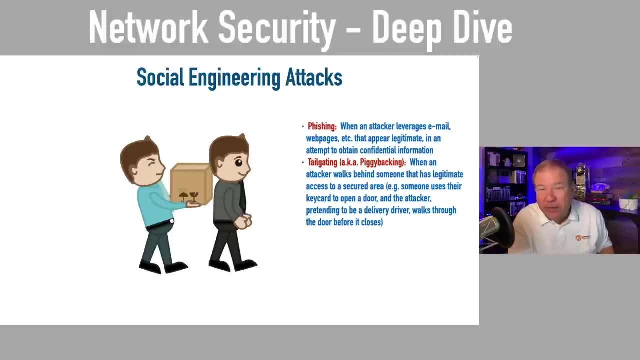 a data center and or maybe to get into a building. This is something that Kevin Mitnick would do when he would get access to buildings. He would do something like this: You can pretend to be a secure or delivery driver carrying a big box and you pretend it's really. 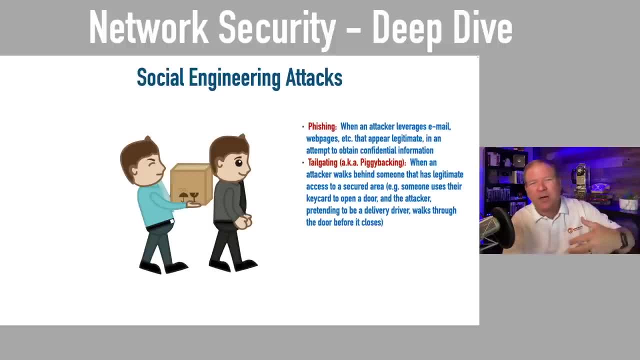 heavy And you see somebody going in, So you hop out of your car and you start carrying this box. You say, Hey, buddy, can you hold the door for me? And they humans, they're good people, A lot of people are good and just trying to help, as our nature. So that, oh yeah, let me help, Let me. 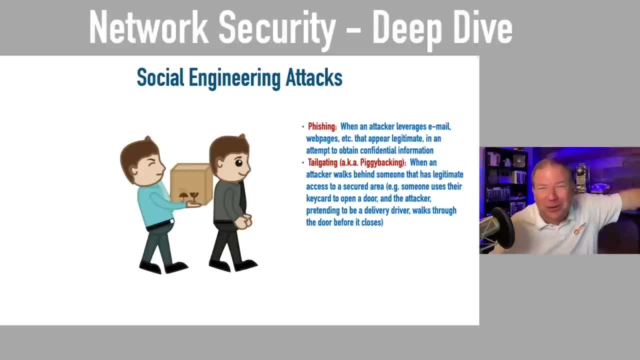 get that door for you And they'll hold the door open while the malicious user walks in with this box containing nothing, really, but they've got access to the building. That's called piggybacking. Another way that we might do, or an attacker might do, social engineering is called shoulder. 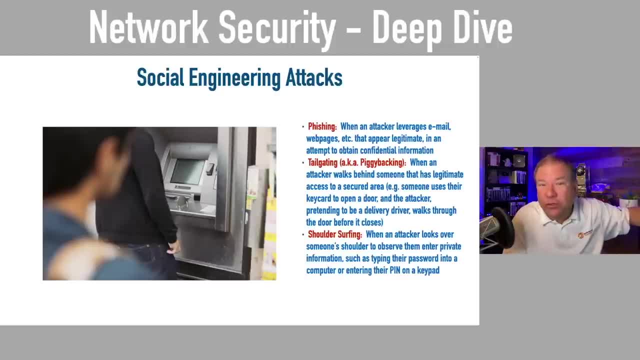 serving. Here they're looking over the shoulder of somebody entering a password or keying in the pin. Now, personally, I'm probably not. I haven't practiced it for one thing. but if I'm looking at somebody typing a password on the keyboard, I don't know what they topped, but some people that. 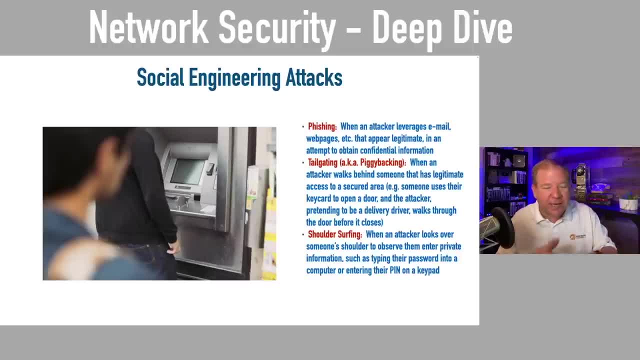 have practiced this. they are really, really good. They can watch you type something and eight characters. they know what you type just by watching your fingers on the keyboard, So you might want to be very cautious about who's around when you're entering password or pin information as an 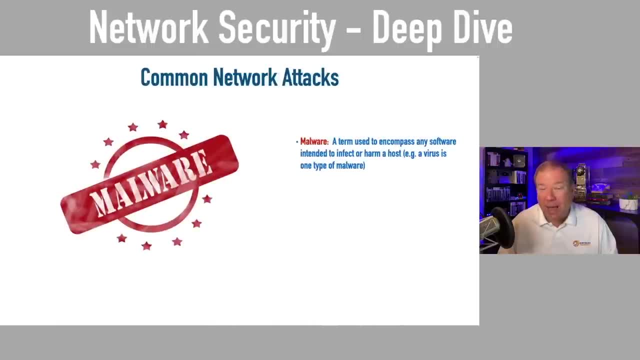 example. Another common type of attack is malware- Malware. it's different than a virus. Oftentimes a virus will be infected with a virus and it's going to maybe destroy things on our system. Malware could do that, or malware might be used for other purposes. I gave the malware example. 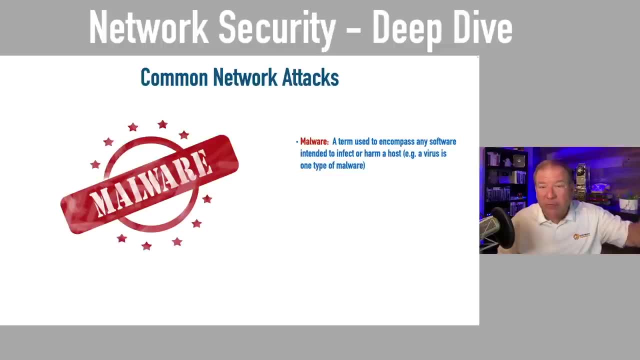 when we were talking about a DDoS attack with a distributed denial of service attack, We said we, maybe, through some sort of gaming app that people downloaded, we infected computers around the world with malware. Well, one feature of that malware: 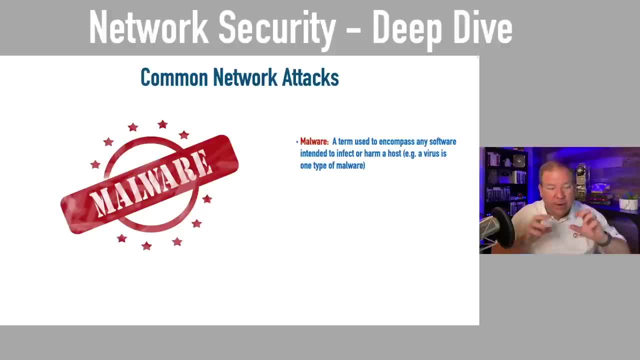 in that example was the ability for somebody to come in through a back door from that command and control server and get access to these PCs or smartphones or wireless routers that live around the world because they've been infected with malware. Now what they can do is right now for any other apps or apps in the world if they're not using a. 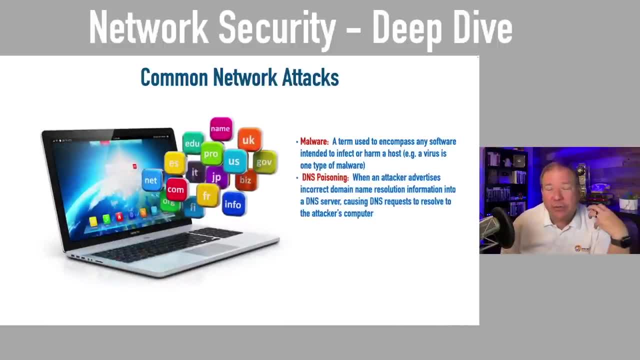 malware, they can instal it at a different level. right, That's been an example of a really good and effective attack. When we talk about a DDoS attack with a distributed denial-of-service attack might also do DNS poisoning If they can convince us to go to their DNS server, which they can if 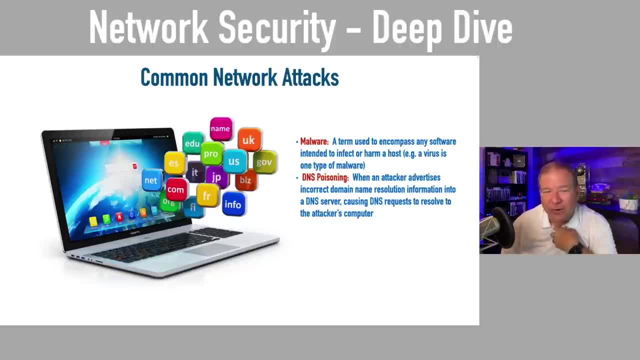 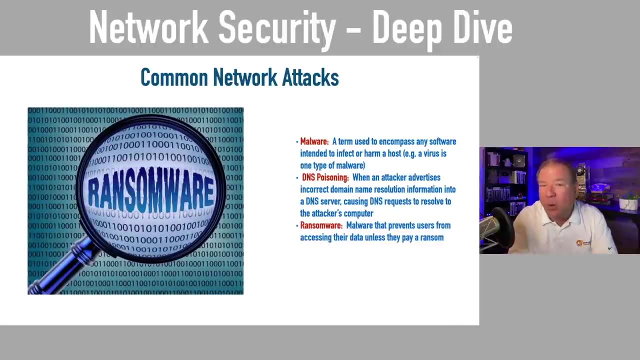 they're able to send us information from their DHCP server. we can do DNS poisoning, where they're trying to go to a popular social media site, but instead they're redirected to our site, which looks like that social media site, and we capture their password information- A type of malware. 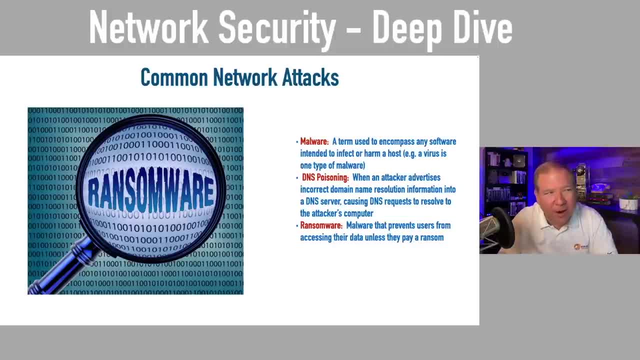 that's really, really ugly is ransomware. A few years back there was a really popular one on the news. It was called the WannaCry virus. WannaCry made you wanna cry because it would literally hold your data for ransom. You would get this big red screen that said the data on your computer. 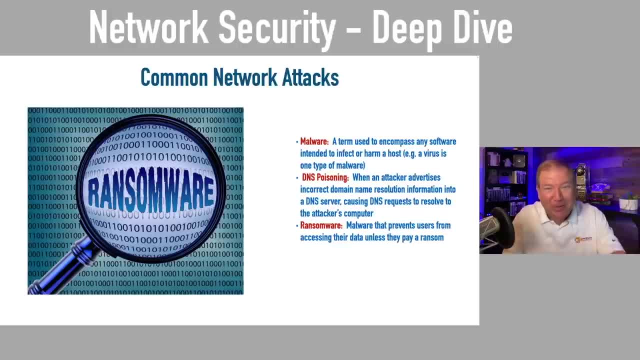 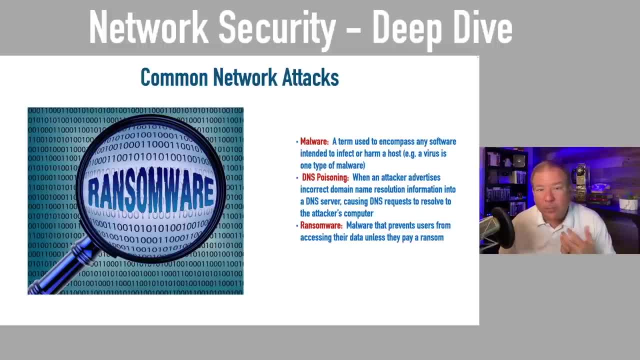 Law enforcement's response got to the point where they said: our only option is to pay it. We're not able to decrypt your data. If you want any chance of getting your data back, you're going to have to pay the ransom- Now a percentage of the time the people would pay. 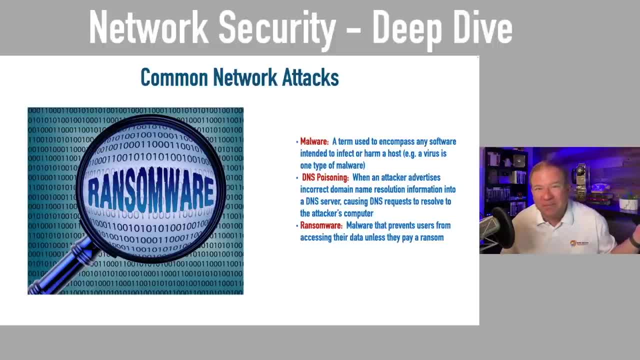 the ransom, They'd get their key. Sometimes they paid the ransom, They still lost their data. They never got a key. So, yeah, I'm a big proponent of having malware scanners or ransomware scanners and virus scanners on our devices. 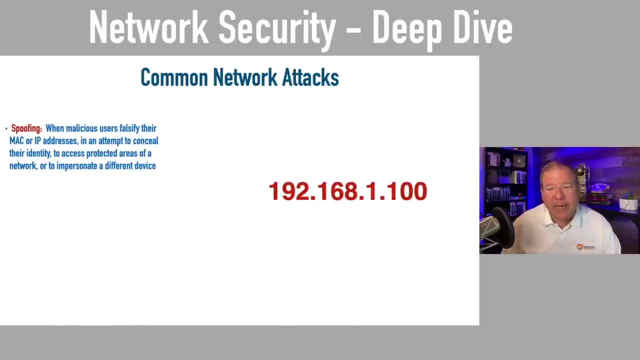 to better protect ourselves. Another type of attack is- and we saw this earlier is a spoofing attack, where an attacker claims to be coming from an IP address that they're really not coming from. This is where we were launching that DOS attack earlier. The attacker was claiming to be the. 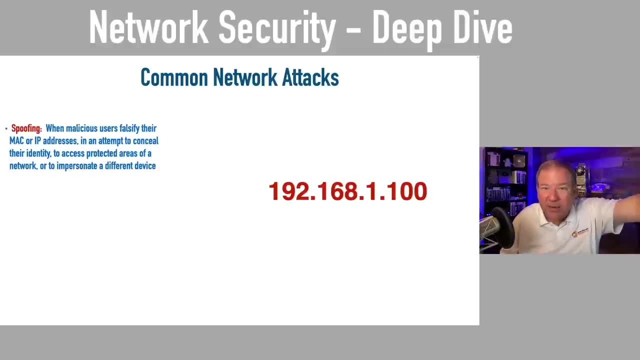 victim's IP address when they sent that directed broadcast out. when they did a ping to the directed broadcast, Yeah, they were spoofing their IP address. We can, by the way, prevent that on Cisco routers using a feature called reverse path forwarding. 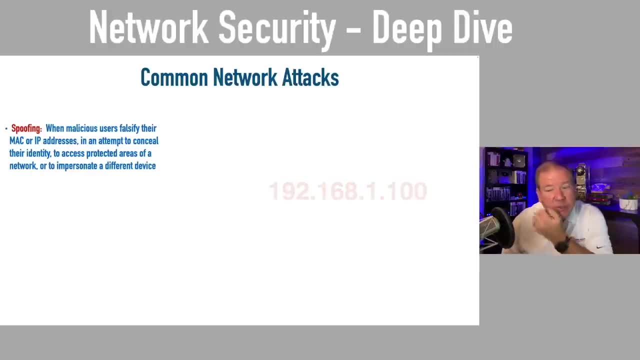 RPF. What RPF is going to do? it's going to make sure that we're not coming from an IP address that should not be seen on a particular router interface by taking a look at the source IP address of packets coming in an interface and comparing that to the router's IP routing table And the router. 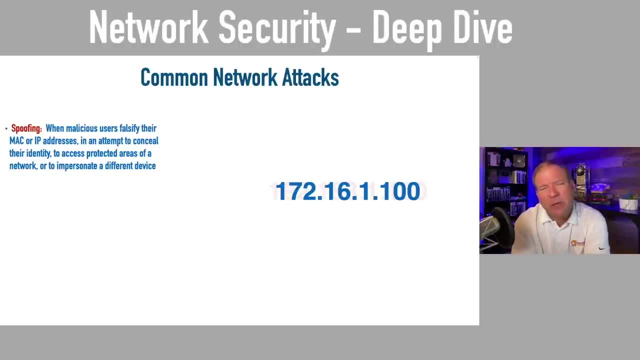 says: if I were going to send traffic back to that IP address, which interface would I use? And it's oh, I would use gig zero, slash two. Well, if that IP address came in gig zero, slash five, that's inconsistent with the IP routing table. And if we're running reverse? 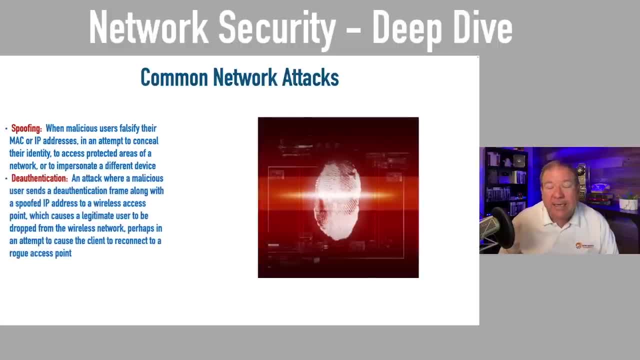 path forwarding on the router. it's going to block that traffic. Deauthentication is something we might use on a wireless access point. For example. here's a Cisco wireless access point And even though this is better with Wi-Fi six, most access points are not running Wi-Fi six. 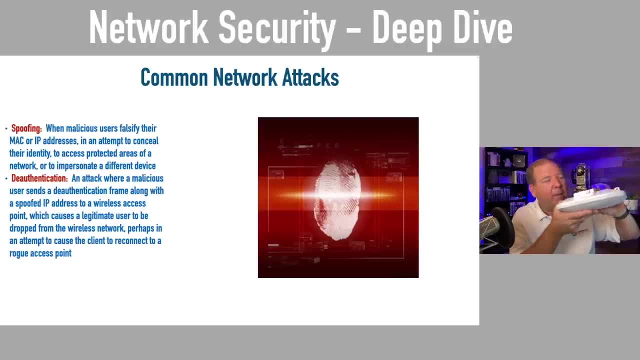 We're still running like dot 11 AC, which is Wi-Fi five, But let's say that I've got my- here's my smartphone. Let's see, I've got my smartphone authenticated with this wireless access point. Well as an. 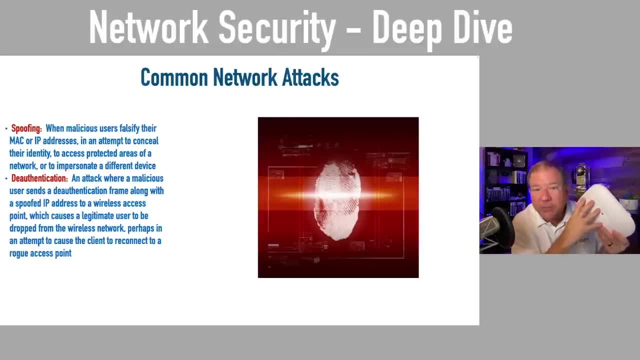 attacker. I can send deauthentication frames to this access point to knock that smartphone off And it's going to try to re-authenticate. In fact, if you join us for our certified ethical hacker training, I show you how to do that in Kali Linux. I have Kali Linux send out a bunch. 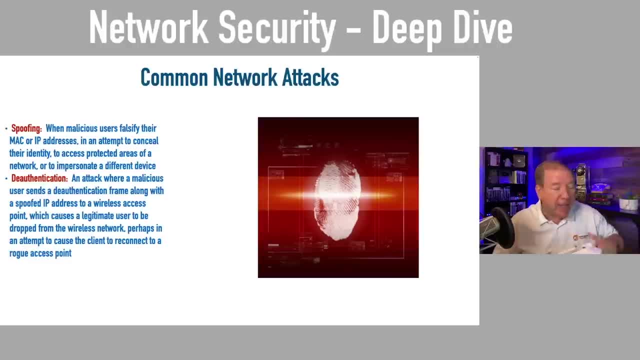 of deauthentication frames to a wireless access point, It kicks my phone off. when my phone tries to reattach, tries to re-authenticate, It goes through a not a three-way but a four-way handshake. I capture what's going on with that four-way handshake in the demo that I do in that. 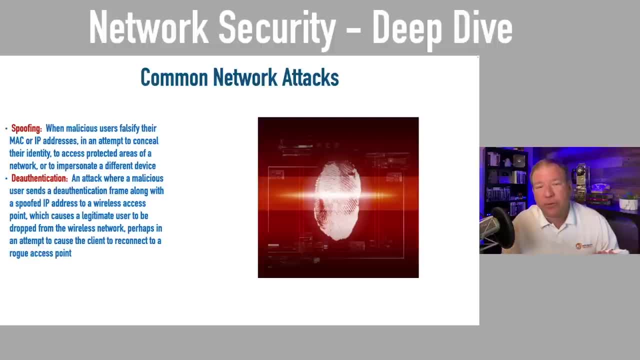 I think it's called our professional ethical hacking course, but it gets you ready for the certified ethical hacker exam. I take that information captured in that four-way handshake and I run a brute force attack against that, against a password list of like 14 million. 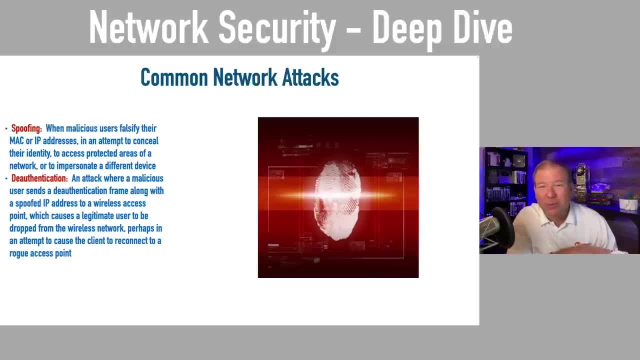 commonly used passwords And sure enough, that was one of the commonly used passwords, I think, in that I used my favorite Star Wars Sith Lord, Darth Bane- If you've ever read the Darth Bane trilogy, really really good reading there- But Darth Bane was the password I used in that example. 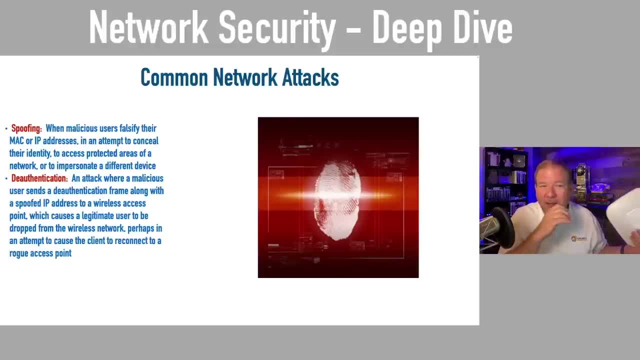 And wouldn't you know it, that was one of the commonly used passwords in that list that I used for my brute force attack And within about 20 minutes I was able to break into that access point. in that it was an isolated lab and it was my own equipment I wasn't breaking into. 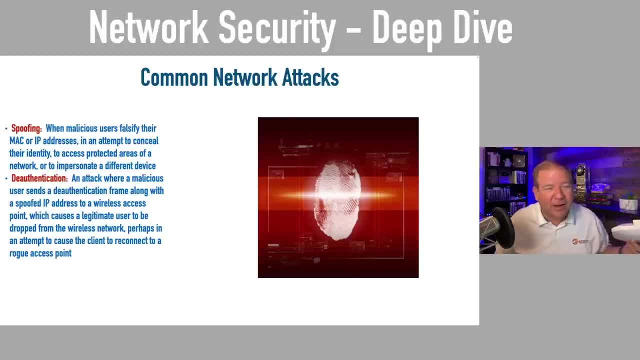 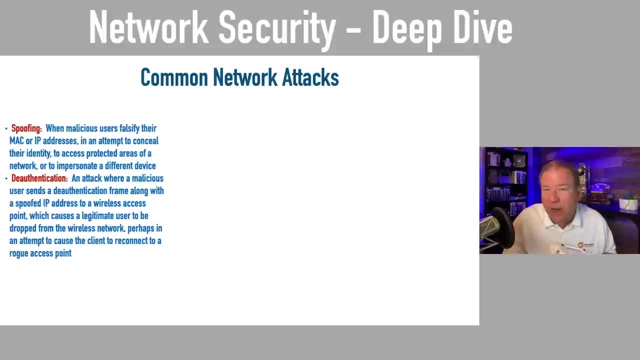 somebody else's network. I was doing it for demonstration purposes only on my own equipment, But that's what we can do With deauthentication frames, And again that gets better with Wi-Fi, version six we'll be talking about later today, But also some of the Cisco access points even prior to IP. 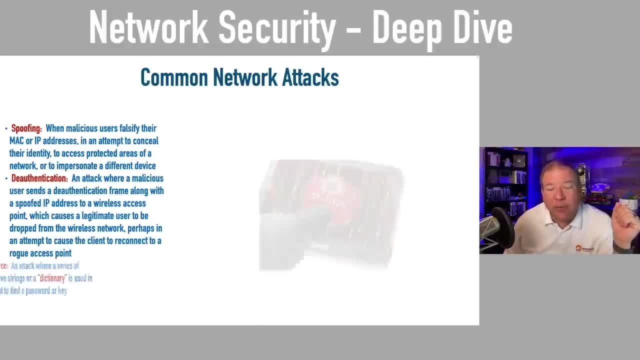 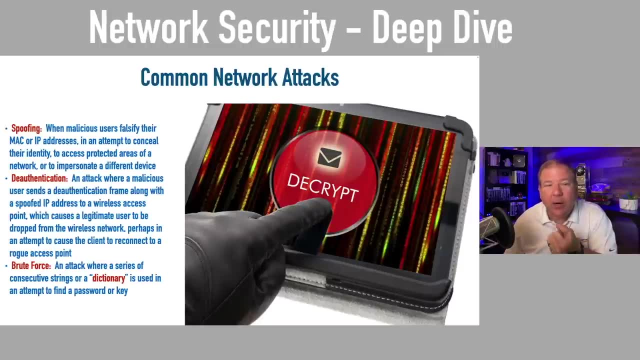 version six, they could prevent those deauthentication frames as well. And I mentioned that if we do get some data, we get a hashed string or an encrypted string or we watch that four-way handshake with a wireless network- we might run a brute force attack against that. 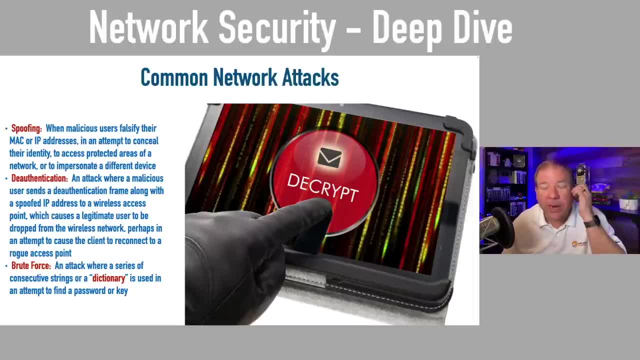 that capture data- MD5,, for example, our hash that we talked about earlier. I could take a bunch of different commonly used passwords. run the MD5 hash on them, see if it matches that string that I have, And if it does, that's probably the password. So, even though we cannot decrypt, 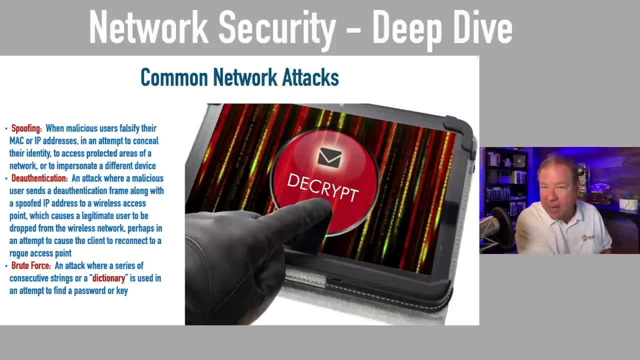 something that's hashed. we can run a brute force attack on a password list and see if that hash matches the hash that we have that we're trying to decipher. That's a brute force attack. How do we defend ourselves against some of these different threats out there? 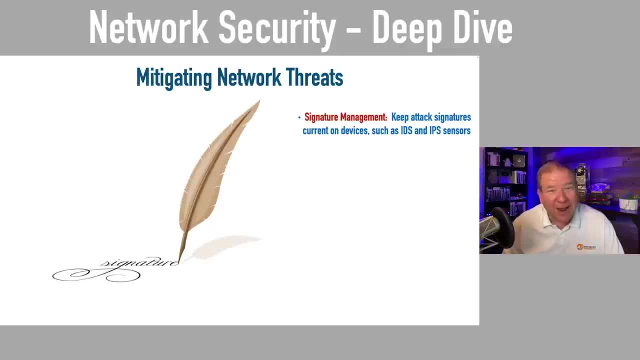 Just some best practices. A lot of these are common sense, but do we do them? As Brendan Bouchard says, common sense is not always common practice. We have things like our IDS or IPS sensors and I mentioned that they have a signature database. We need to keep that signature database. 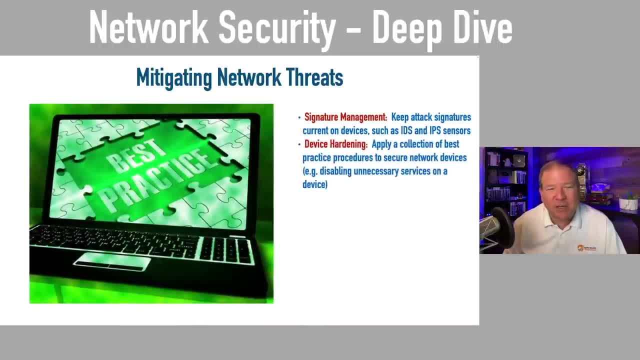 up to date. So let's make sure we do good signature management. There's also a collection of best practices to harden a device like turn this on, turn this off. Cisco has a macro that you can use on some Cisco routers. Do this in a non-production network when. 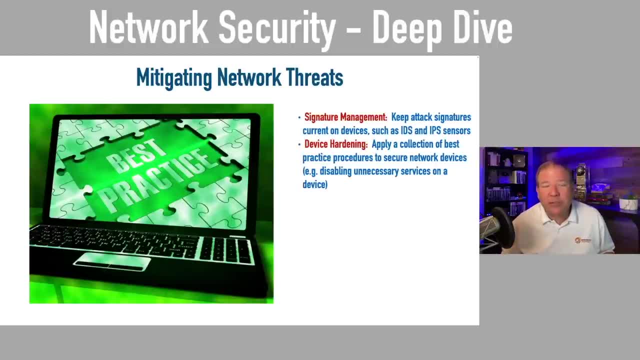 you're first experimenting with it, But you can go into global configuration or not even global configuration mode. You can just say. you can say auto secure and it's going to walk you through a wizard that's going to allow you to apply a bunch of best practice security recommendations. 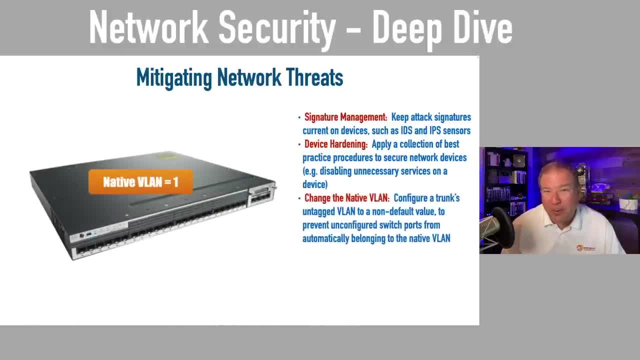 to a Cisco router. We should also probably change the native VLAN. I showed you a VLAN hopping attack earlier that was predicated on the attacker knowing the native VLAN that was being used on a .1Q trunk. We should probably change that to something. 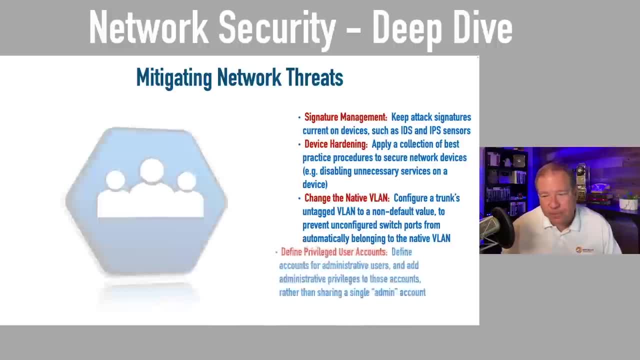 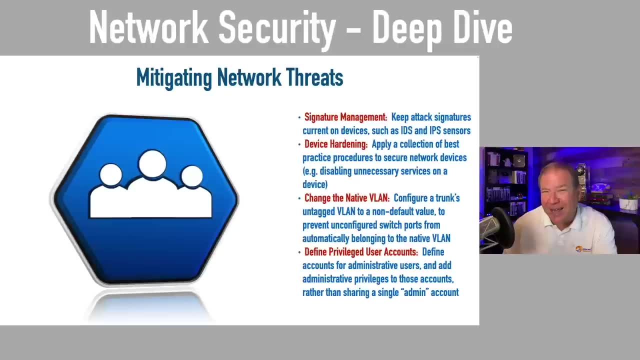 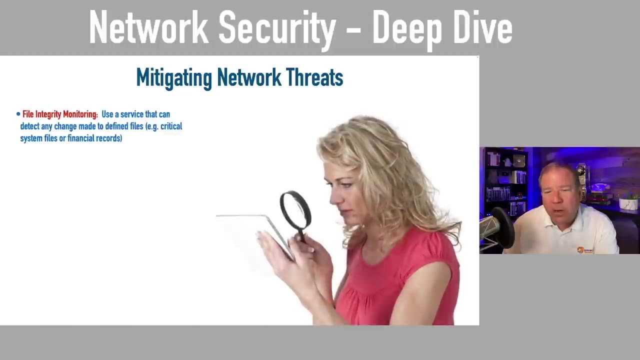 other than one- Maybe change it to 20 as an example- And something else we should do is not give users too much access to things they might not need access to. In other words, we want to define the privileges given out to different user accounts. And when we're talking about users, 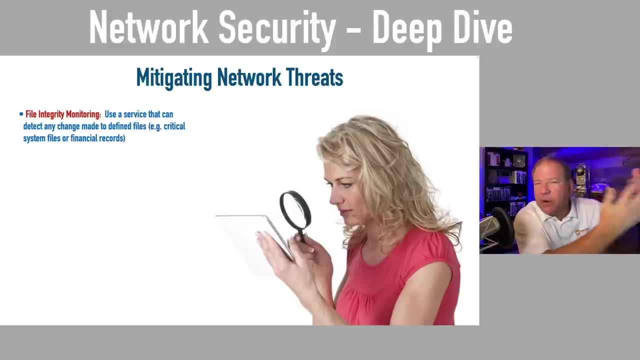 we might want to send users if we're sending them, if they're downloading a file. instead of just downloading that file, we might want to also send them a hash digest. Or we might use HMAC to say: you should be able to calculate this same hash digest by running it on this file. 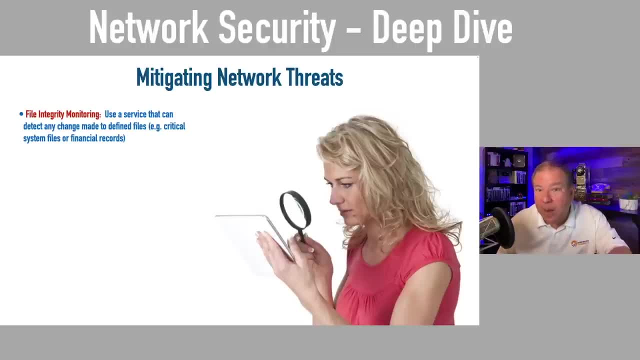 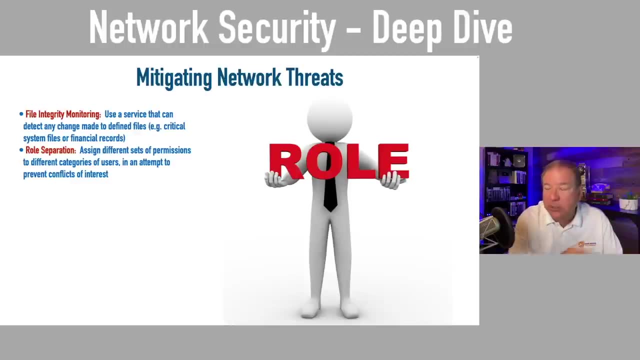 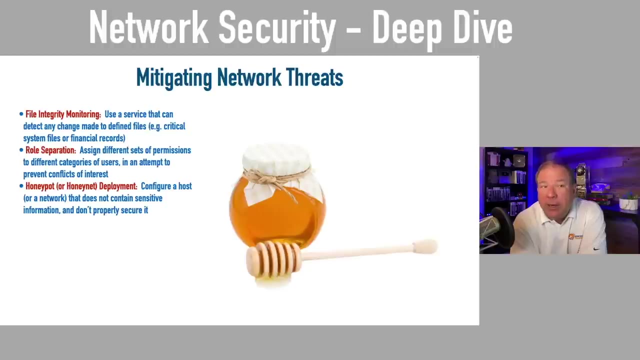 to make sure that file integrity has not been compromised- Somebody's not modified that file in transit- And when we're setting up users, let's give them different roles. Let's not give them more permission than they need. We can also protect our networks by installing. 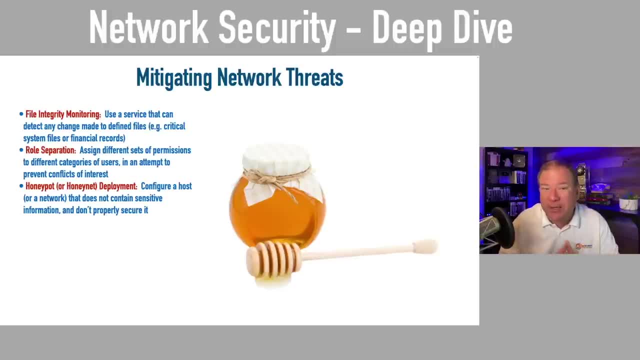 distractions. We can install a server called a honeypot, And a honeypot is a server that's very weakly protected. So if an attacker is trying to scan our network, looking for any weaknesses, they're likely to come up on this honeypot to say, oh, they've got these ports open. 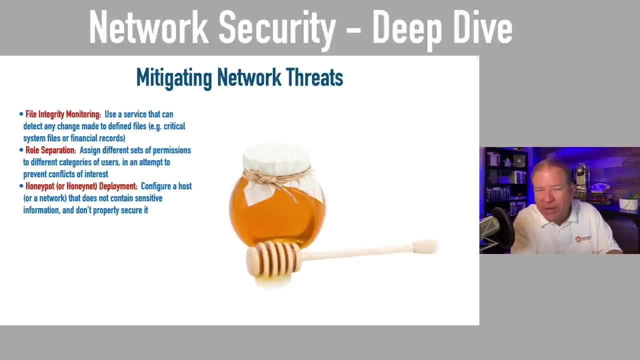 They don't have this patch applied to their operating system And the attacker breaks into that honeypot system. Well, once they're in there exploring around, we have data that might look like it's important, but it's really not. It's not secure data, It's a distraction. 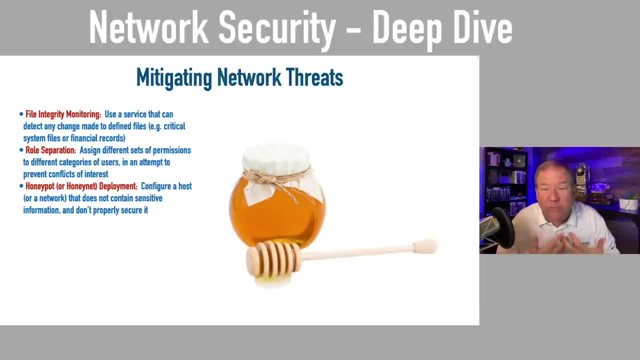 While they're in there. number one, we can see what sort of tools the attacker is using to get into our network, so we can better defend against those approaches. And also we're just wasting their time. They're spending all their time looking through a meaningless system, while 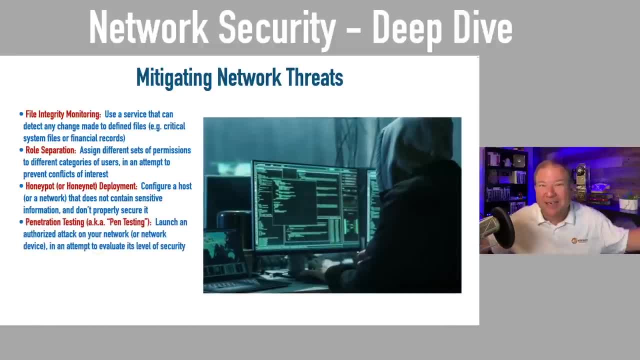 we're watching them, And on a larger scale you could have an entire network. that's a distraction and that's called a honey net. And something we mentioned earlier: pen testing. It might be worth having somebody internal or somebody external do a penetration test on our network to. 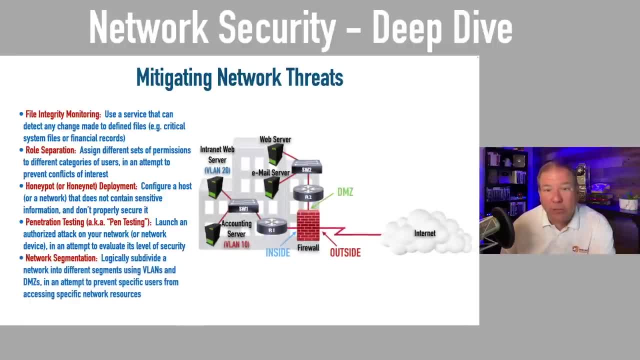 find any weaknesses or identify any weaknesses, And I gave the university example earlier of segmenting our network up into different security zones. Yeah, Maybe in the university example we want to protect students from the bad people on the internet, but we want to protect our faculty. 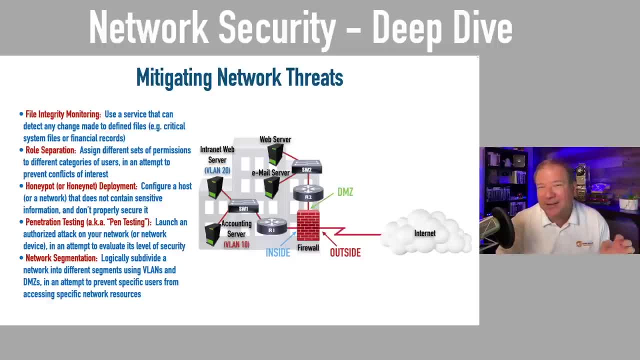 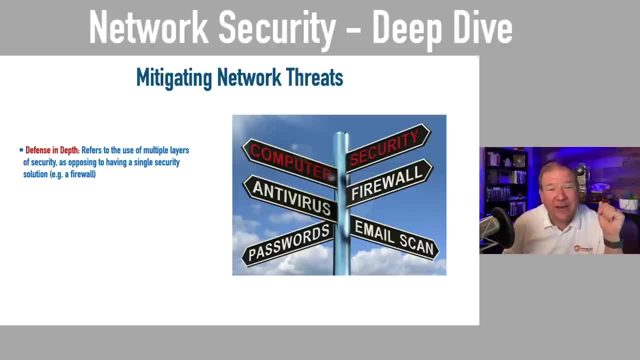 and staff from students who get curious and try to get in and maybe change their grade is the classic thing you see in the movies. Some other ways that we might defend against these attacks is what I talked about earlier. Cisco calls it defense in depth. I gave the metaphor of a blanket. 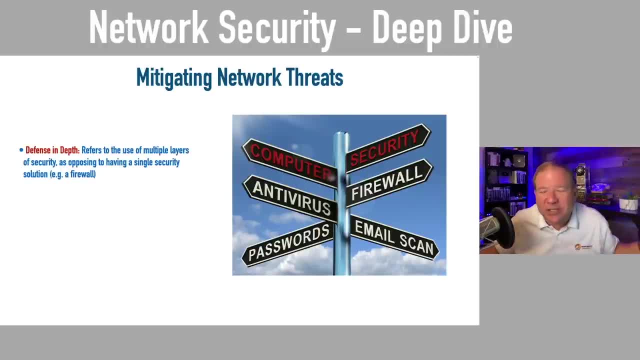 on a bunch of blankets on a cold winter's night. We don't just install a firewall. We don't just install an IPS sensor. We don't just install malware detection software. We do it all. We have overlapping layers of security. We want security in our defense in depth And when we 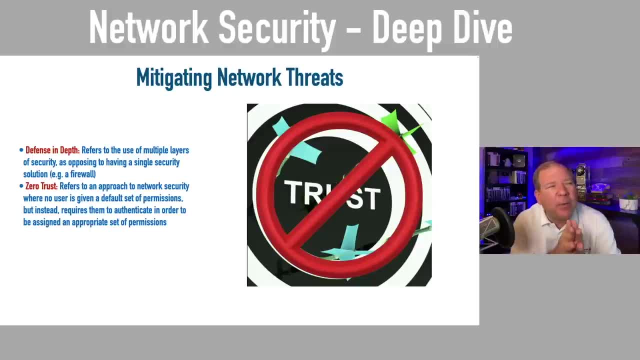 add it. we're talking about users again. When we add a user, we probably don't want to say: well, a user is going to have this default set of permissions, They can get to something, but we'll have to give them extra permissions to get to other things. 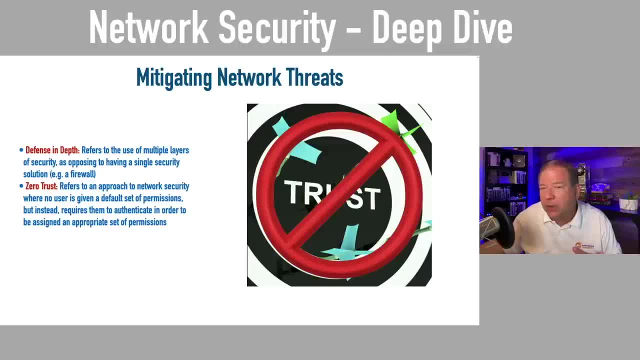 A lot of people in high security environments recommend using something called zero trust. When you add a new user, by default they don't have access to a default set of resources. They have access to zero resources. We don't trust them at all until we explicitly give. 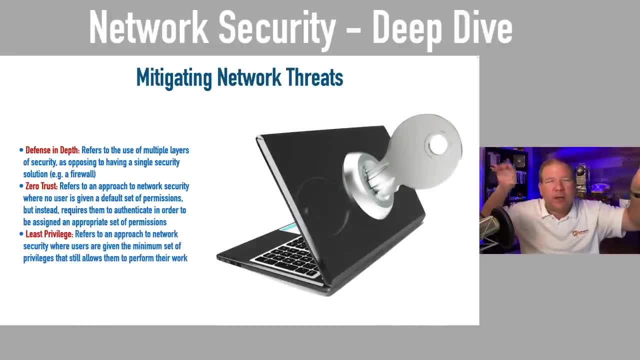 them permission. And let's say that a user belongs to two different groups. This group is not allowed to get to this one server. This other group is allowed to get to this one server. If we use the link, we're going to get to this one server. We're going to get to this one server. 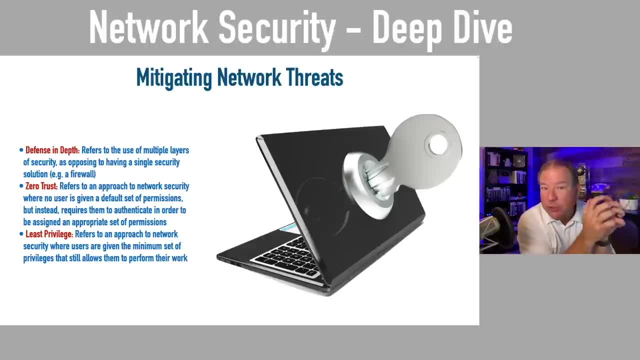 The least privilege approach the group that's most restrictive. that's going to be the rule that's enforced. So, even though the user belongs to these two groups and one group says, yes, you can get to the server with least privilege, we're not going to be able to get to the server. 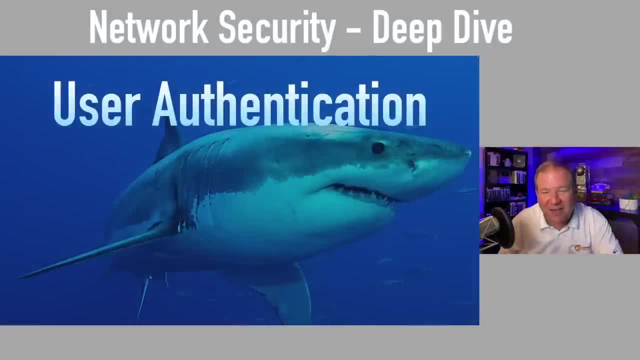 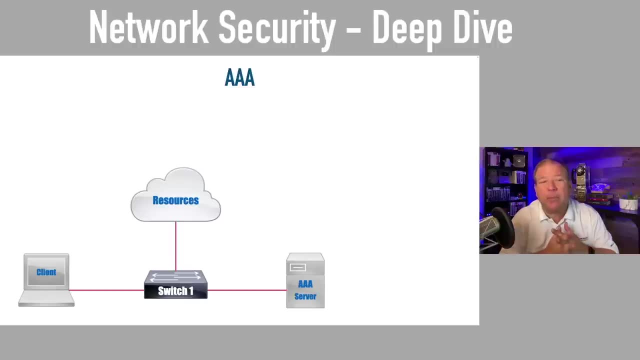 because the user also belongs to a group that should not have access to that server. We also want to be able to authenticate our users and prove they are who they claim to be, And you can set up a database on a router, for example, or a switch where somebody is going to. 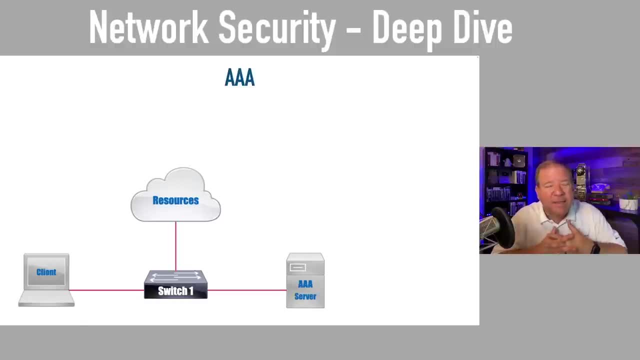 have to give a user a password And that's going to be the rule that's enforced And that's going to username and password along into that switch. But that's not very scalable. And if we had this on, let's say, 20 routers and we had somebody leave our networking department, maybe we fired. 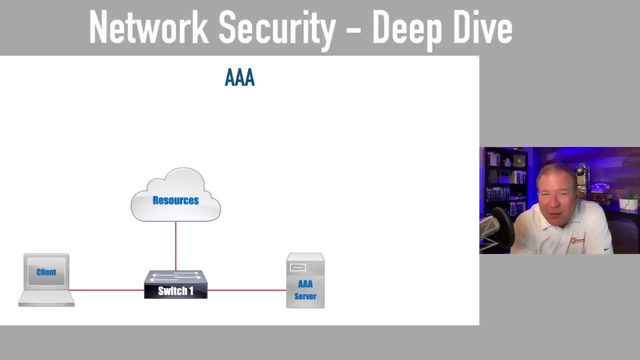 them. they know the password to our routers. We're going to have to go around and change it on all the routers. That's not scalable, So what we can do instead is use AAA Now. AAA, that's an acronym standing for authentication, authorization and accounting. Authentication is us proving we are. 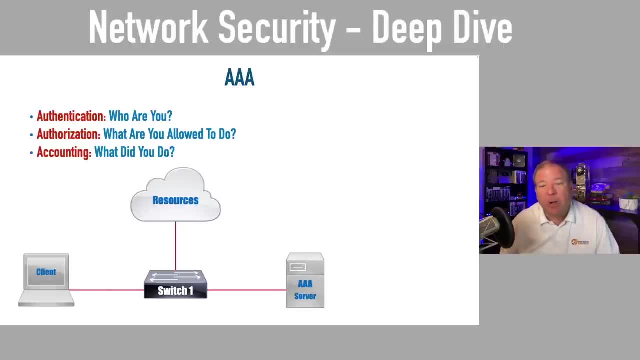 who we claim to be. like giving credentials, Authorization is asking what are we allowed to do once we get authenticated, And accounting is kind of keeping an audit trail. It's saying: what did you do once you got logged in? This reminds me when I went to work at Walt Disney World At Walt 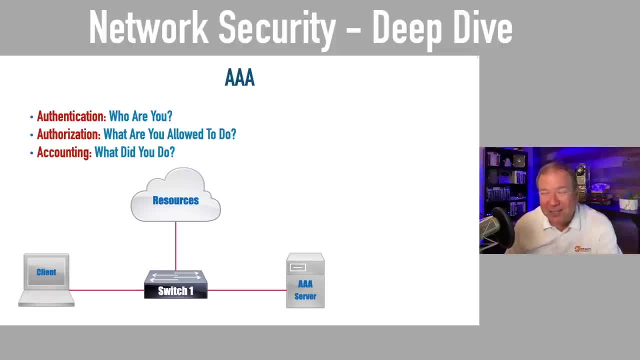 Disney World. they had over 600 Cisco routers and thousands of Cisco Catalyst switches. Well, they didn't want to give me a password, the enable secret password to 600 plus routers. What they did instead is they gave me an account on AAA server. I had a username and a password. 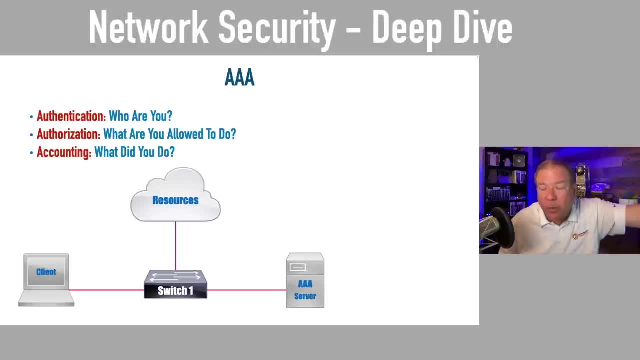 and I was given authorization to access the routers once I got logged in. Then, when I ended up leaving Disney, they didn't have to go reset the password on 600 routers, It just deleted my account. It's a lot more scalable in an enterprise environment. 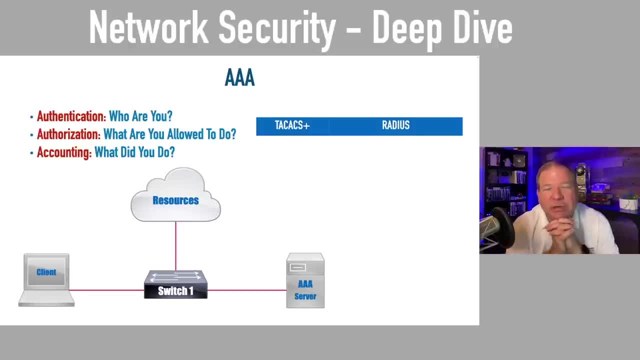 And there are two basic types of AAA servers that you might run into: TACX plus servers and radius, And on some exams you might want to know the difference between these. First of all, TACX plus. the plus means it's a Cisco proprietary implementation. 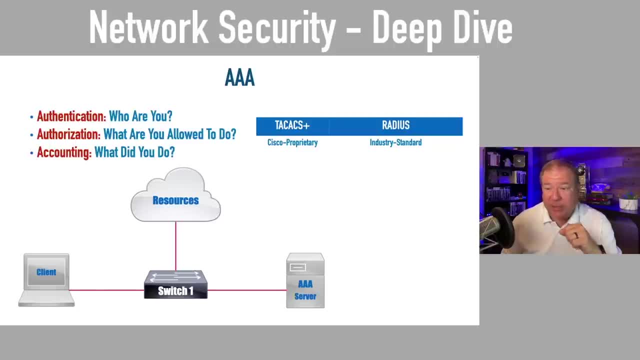 of the industry standard TACX Radius. that is an industry standard. It's interesting that TACX plus is based on TCP while radius is based on UDP. and UDP is connectionless: If we drop a packet it's not going to be retransmitted. something to keep in. 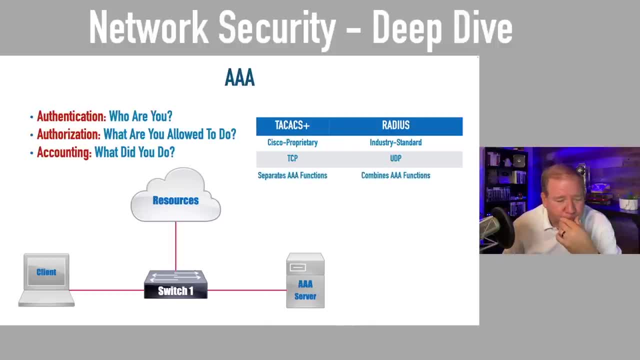 mind there. And with TACX plus the authentication, authorization and accounting- they're treated as separate entities, separate workers doing those three separate jobs. With radius it's kind of all lumped together in one big thing. And with TACX plus the server does not just authenticate the user, the user. 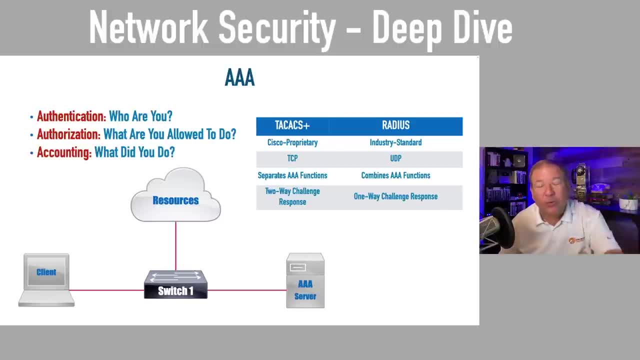 authenticates the server. So we know we're not talking to a rogue server. With radius, it's only one-way authentication. So I'm making a case that TACX is better in a lot of cases, but there's still plenty of times when I'm going to have to do that. So I'm going to have to do that. So I'm going to. 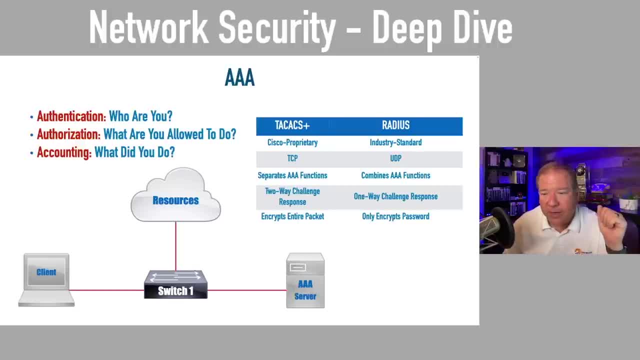 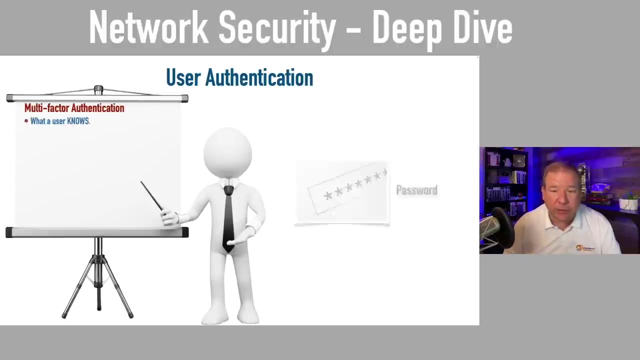 be using radius. Radius is often used in wireless networks to authenticate Something else. TACX is going to encrypt the entire packet, but radius only encrypts the password that's being sent when we're giving our credentials, And user authentication might be multi-factor authentication With multi-factor. 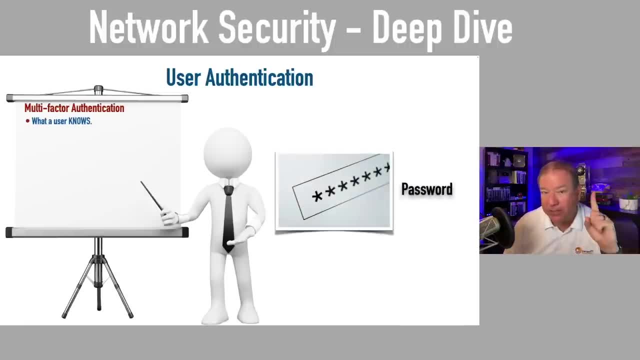 authentication. it's more than just knowing a password. That would be single-factor authentication. It might be something we know like a password, but it might be also something that we have, like some sort of a badge Or a key card. 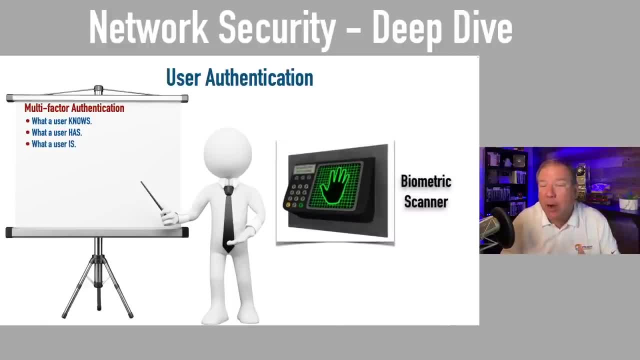 Or some sort of smart card, Maybe what a user is, Biometric scanners, Or maybe it's where a user is based on geolocation. We can have geofencing or what they do. Let me give an example With my smartphone. maybe I have to know a PIN to get into my phone. 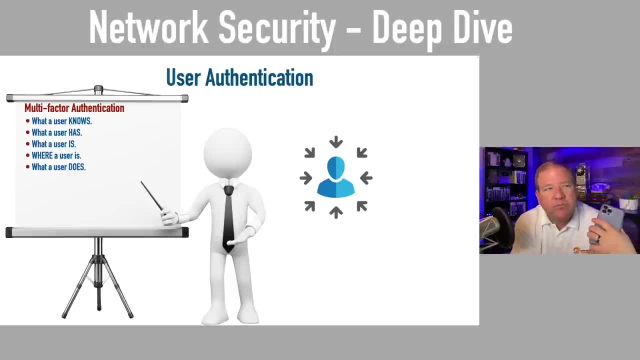 Or if I'm trying to go to. if I'm trying to go to, let's say, a bank, for example, or some other, some other online account, I'm going to have to know a PIN to get into my phone And I've got multi-factor authentication set up on that account. In addition, in addition to 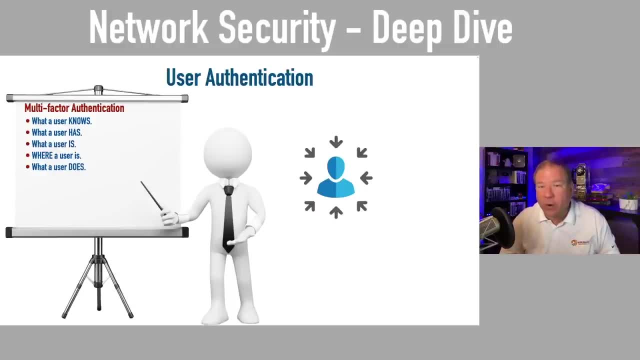 knowing a password, I might have to give some sort of a code. I have. I have the Google Authenticator app on my phone And the Google Authenticator app comes up with a- I think it's a six-digit string for these different sites that I have passwords on And if I try to attach to one of these sites, 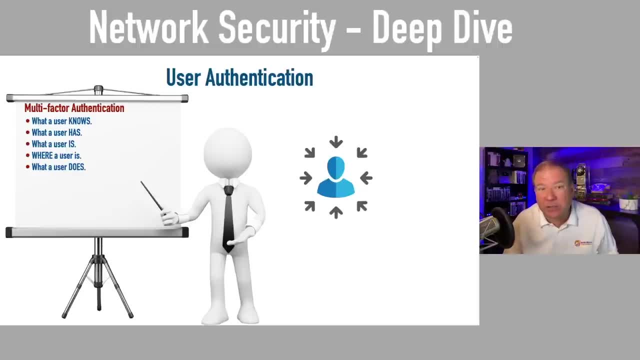 in addition to giving a correct password. I've got just a few seconds to put in the six-digit code that my authenticator has, And I've got a few seconds to put in the six-digit code that my authenticator has, And I've got a few seconds to put in the six-digit code that my authenticator app says that I'm 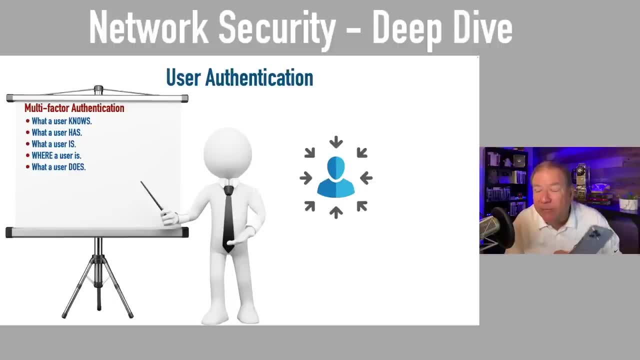 that I need to use. So, in other words, I have to have a phone with that app. So that's what a user has, What a user is. I can do facial ID. I can look at this and it's going to scan my- the LiDAR. 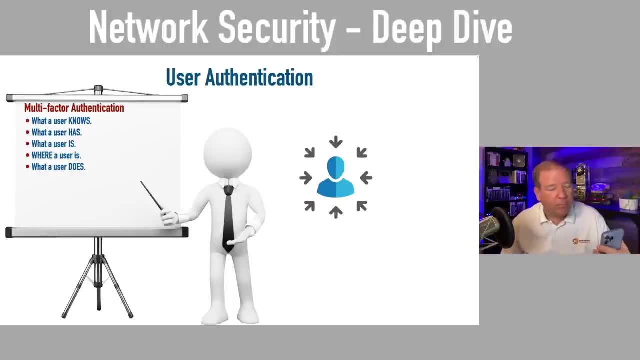 sensor It's going to scan my face and that's who I am. Or on my laptop, I've got a fingerprint scanner Where a user is. yeah, I've got GPS on my phone. It could. I don't think I have a system. 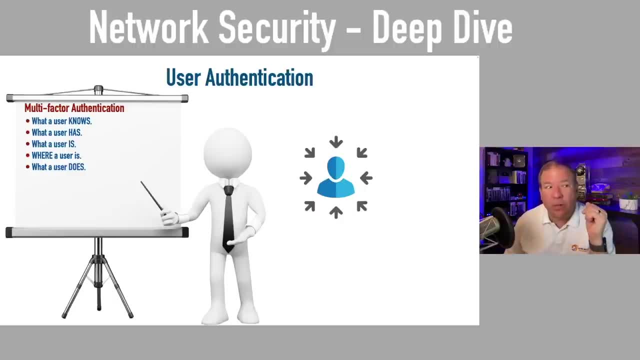 like this right now that I'm using, but we could restrict people to only using a service. Well, I'll give you a perfect example. Not too long ago, last month, in August- Yeah, In August, that was last month- My family and I we went on a Disney cruise. I told you we're big. 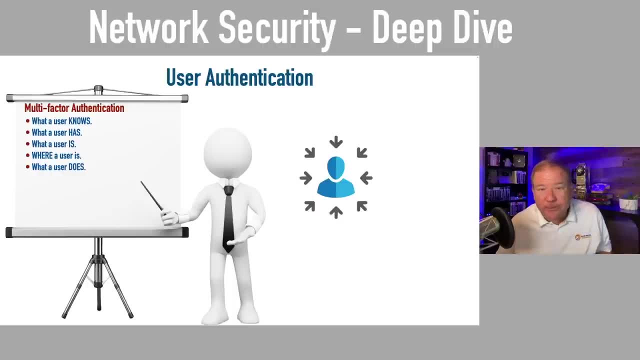 Disney fans And we went on the new ship, the Wish. Well, when you're getting on, when you're getting on the Wish, once you're there, you're able to get access to resources that you wouldn't have access to off off of the ship. So when you go to the app, it says: Oh, we see, you're on board. 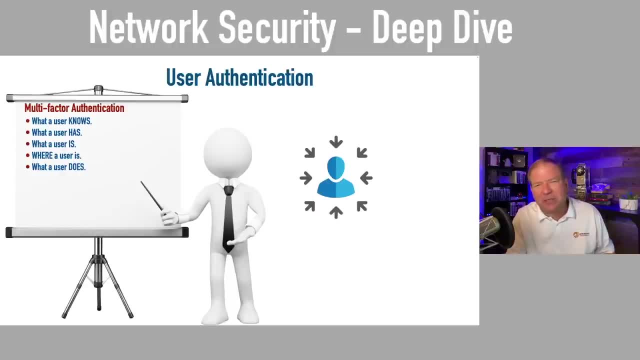 or we see you're not on board Basically. in that case it's not so much geolocation, It's more getting on their Wi-Fi network. But, as an example, one of the things that's hard to get on the Wish is access to their 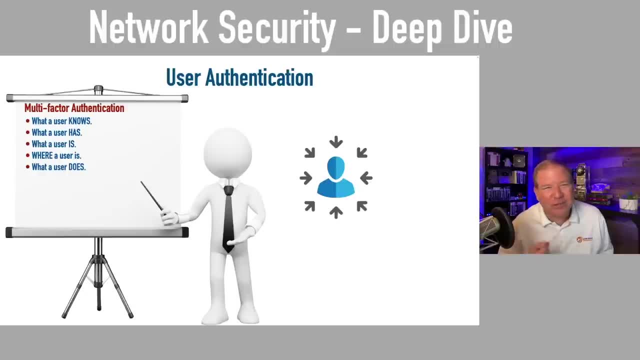 Star Wars lounge. It's called the hyperspace lounge and reservations go really, really quick. So as soon as we got through security and we got into the terminal, as soon as we're geolocated next to the ship, I'm able to get on their access point and I'm able to make our. we're able to make 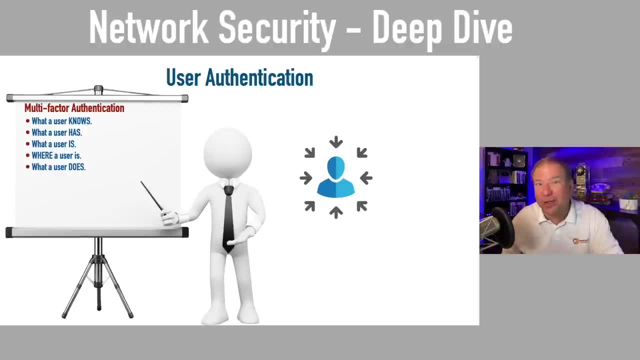 reservations for the whole family to go into the hyperspace lounge, which is really cool, by the way. Check out their $5,000 Kyber crystal drink. That's a whole nother story, But yeah, it could be. you only have access to certain resources, based on where you're located or maybe what a user does. 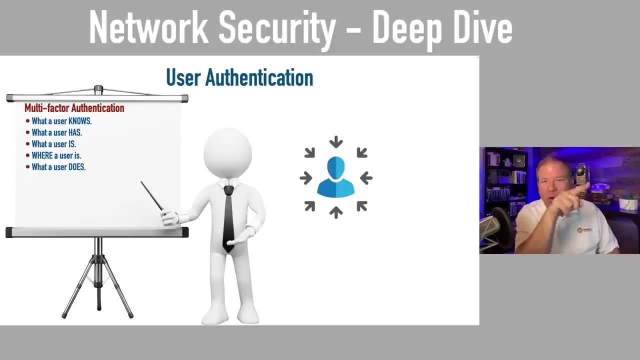 on. on some devices you have to give like draw a star or make some sort of pattern with your finger, maybe on a keypad or on a touch screen, to to prove you are who you claim to be. And one security acronym or standard you'll hear a lot about is 802.1X. This can be, this is used a. 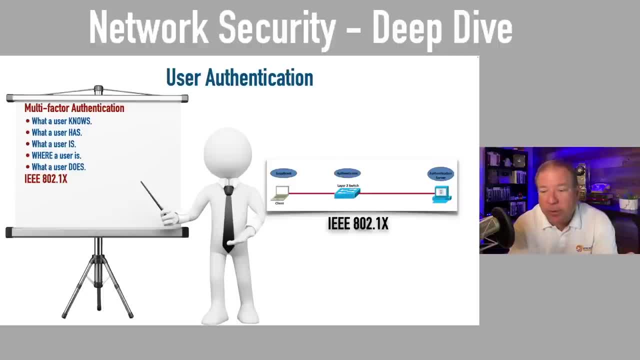 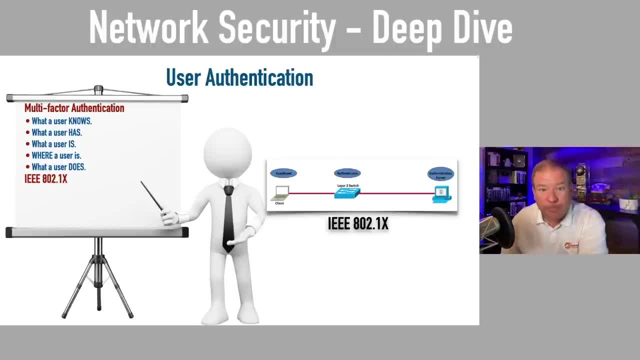 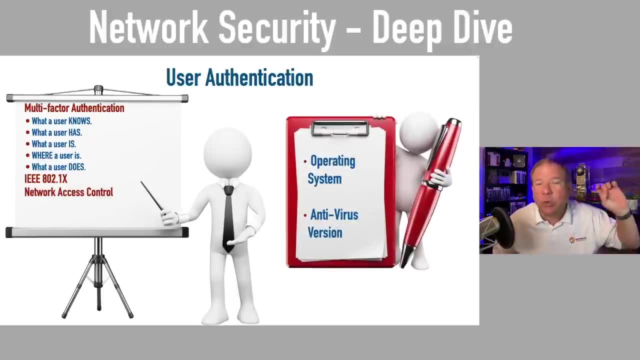 before they get access to a network. So we can set this up on a switch or we can set this up on a wireless access point. Network access control takes it a bit further. It checked, it does what's called posture validation. It checks the- uh, the PC or the phone. 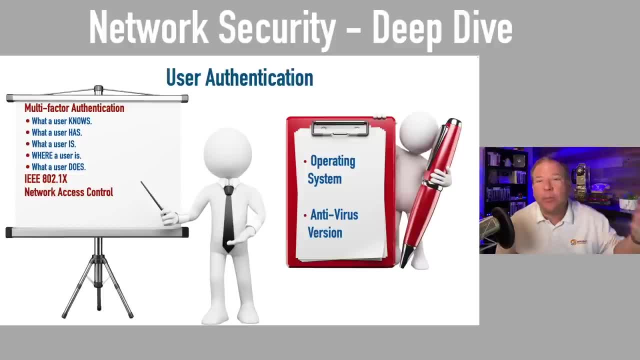 It checks the device to make sure that, for example, its operating system has a certain patch applied or the anti-version or the antivirus software is running a certain version. We make sure that the device that's about to be introduced to our network has a sufficient level of protection And if they do, they're allowed on the network If 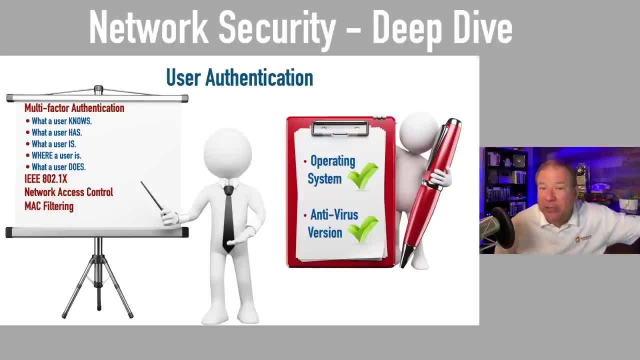 they don't. they're not going to be allowed on the network. We might filter MAC addresses, So somebody brings in a rogue machine. we don't let them get on our network. Or maybe we have a captive portal. This is what you oftentimes see in a hotel or maybe on a plane, If I'm flying. 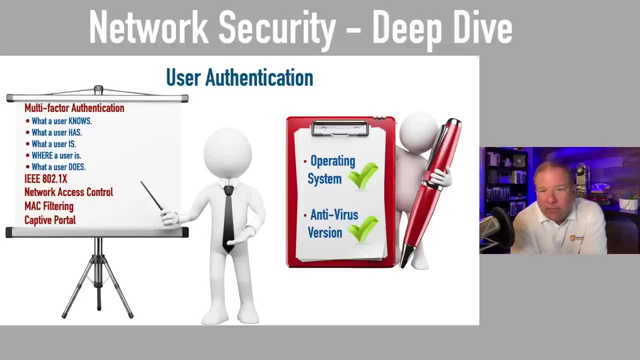 Delta, they have their, they have their, the Delta Wi-Fi that you connect to. So you get on the Wi-Fi on the plane And when you try to go to a website- not so fast- you have to go to their captive. 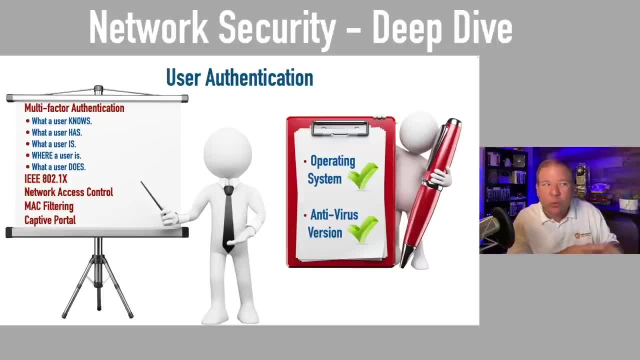 captive portal. They redirect you to one of their pages where you can pay for access to the internet Or in a hotel. you might get a page that says: give me your last name and your room number. If that matches their database, then you're allowed to get. you're allowed to get on the network. 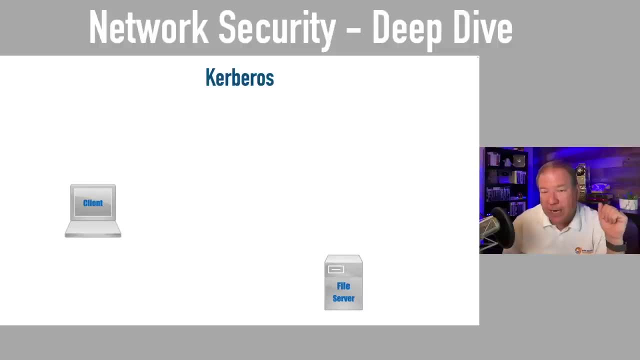 Besides AAA, another security server type that we have out there is called Kerberos, or some people pronounce that Cerberus. It's named after the multi-headed dog that belongs to Hades at Stansgard, at the gates of Hades, But it's. it's actually a little bit more complicated than AAA. You have to have a. 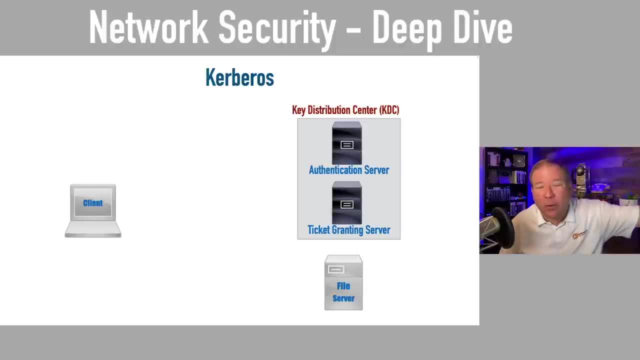 ticket to be able to try to authenticate with the file or to be able to get access to the file server. Metaphorically, you're saying: I have a ticket to access you. Well, to get that ticket you have to first authenticate yourself. So first we authenticate with an authentication server. 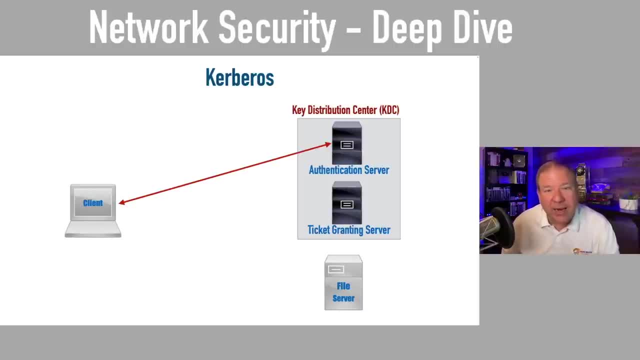 giving whatever credentials we're using, Assuming we're authenticated. we're then given permission to talk to the ticket granting server And if the ticket then or the ticket granting server gives us a ticket, we can then take that ticket and go talk to our file server And we say: we got a. 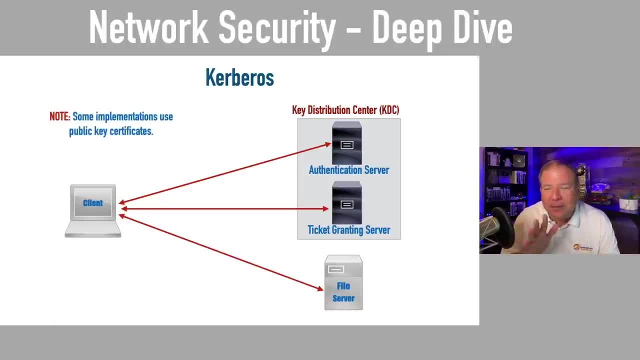 ticket, We're allowed to talk to you And in some cases this is going to use those public certificates or those, uh, digital certificates we were talking about earlier with the public and private key pairs. That's going to make it a little bit more scalable And when we're talking about users signing on, 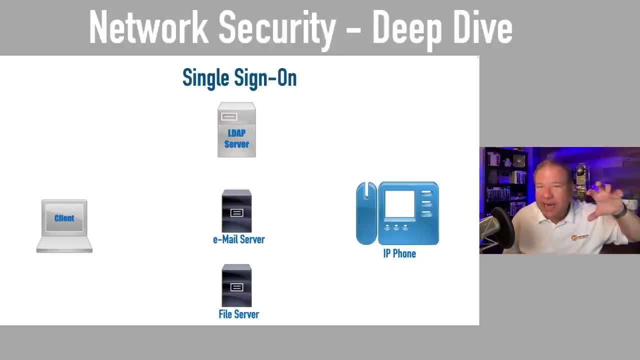 back in the day years ago, we would have one database, I remember, for email users. There will be another database for getting on servers or file sharing on a network. There might be another database for some other act, some other service on the network. That's hard to keep up. 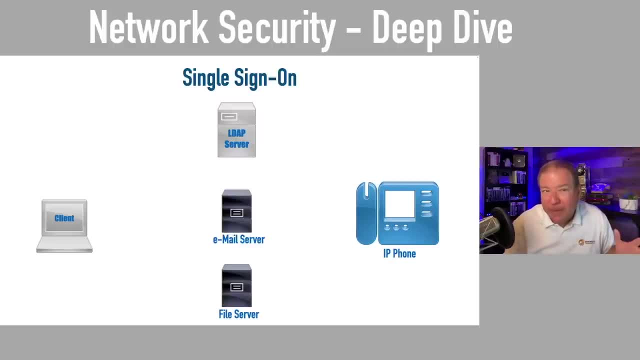 with. We've got multiple user databases for the same user And if they change their database and they're not going to match on one, it's now not going to match on the other systems. To get around that, a lot of people are using single sign-on. Well, single sign-on. 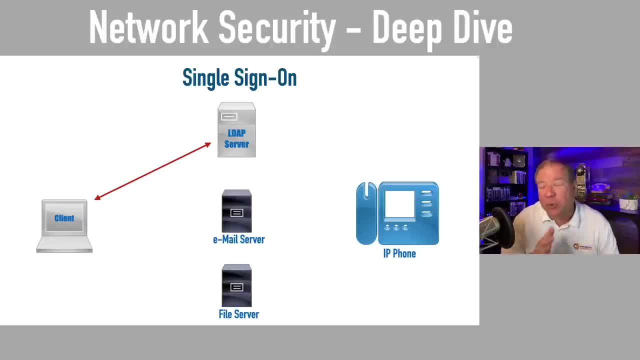 we can use an LDAP server That stands for a lightweight directory access protocol And that can be a single repository on our network for getting access to everything: email, file servers, whatever it is. Getting access to VPN services, we have to authenticate. 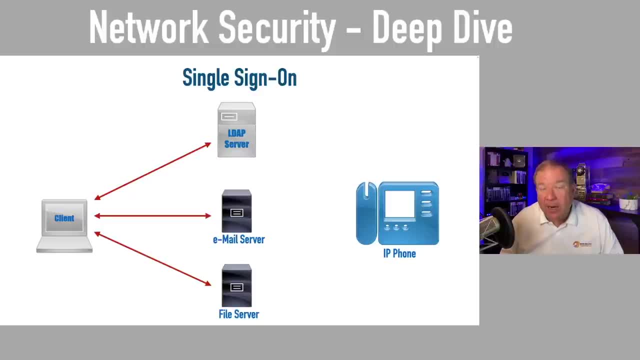 just one time to that LDAP server And I've asked my students over the years what LDAP server they're using And I would say well over 90% of my students have told me that they're using Microsoft Active Directory for their LDAP server. By the way, I've got a video on YouTube if you'd like to see how. 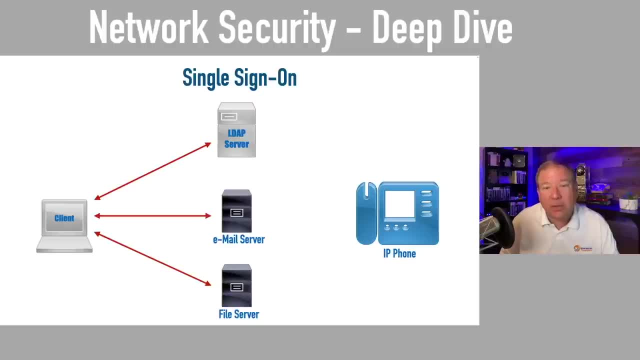 to set up for free, just in a test environment. Microsoft Active Directory: You can just search, I think, Kevin Wallace Active Directory and it should show up if you want to see how that is set up. And IP phones: I said I do a lot in the collaboration world. Yeah, IP phones they can. 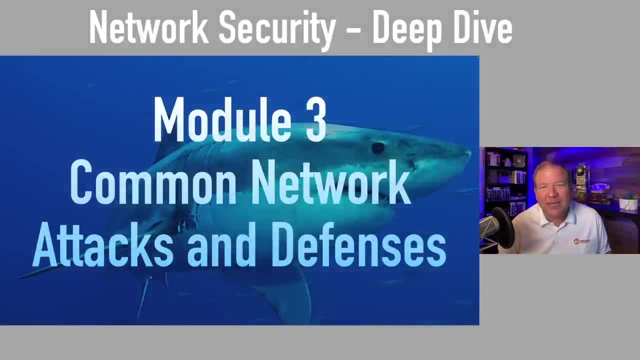 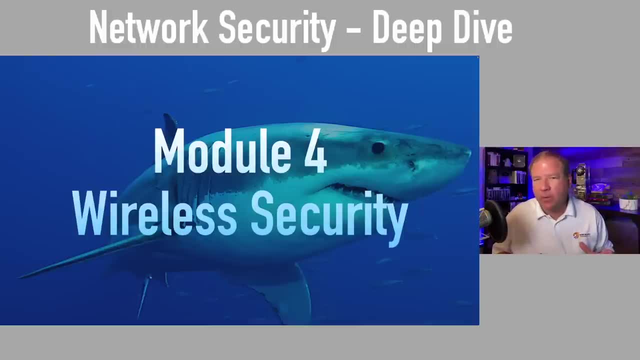 use those LDAP servers too. And that's a look at some common network attacks and common data, And I'll see you in the next video Bye to protect against those attacks. Here in module number four, we want to talk about some different aspects of how we can better secure these things. There are wireless access points. 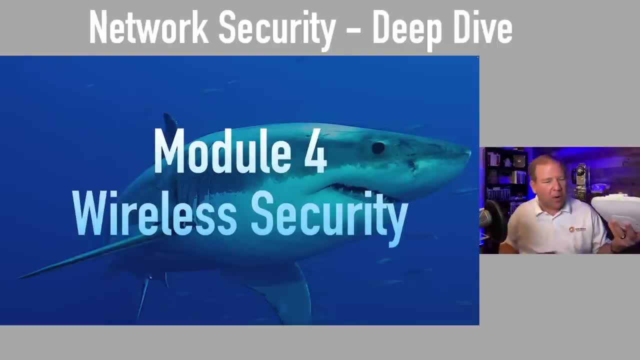 So when we communicate from- let's see, here's a wireless tablet- If I'm communicating and somebody were to intercept that communication, we want to make sure they're not able to read it. We've got basically the same sort of goals that we had, as we talked about earlier. We want things. 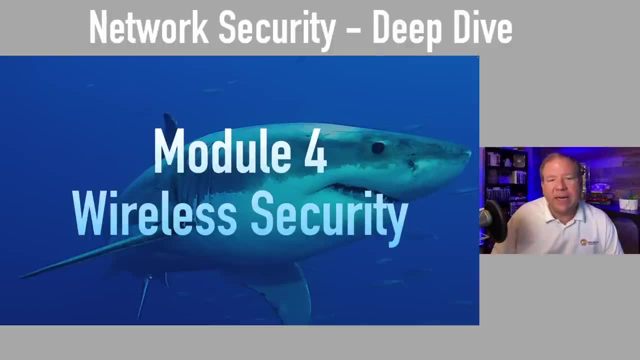 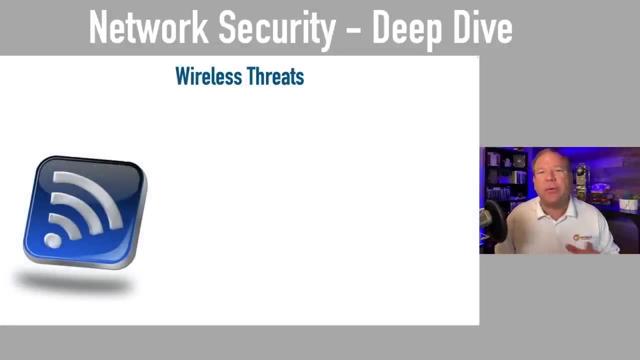 to be confidential. We don't want somebody to gain access to a wireless network if they should not have access to that wireless network, And that's going to be our focus. First, let's consider some different threats that we might have in the wireless environment. One is where somebody 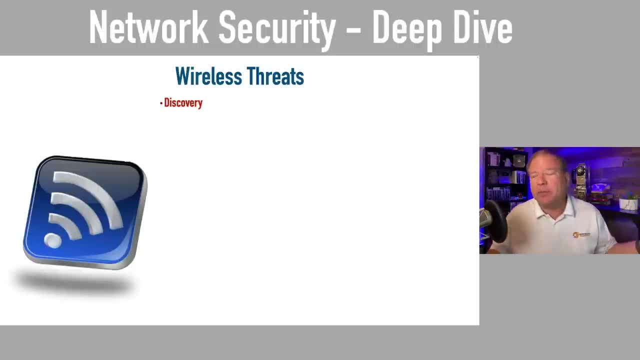 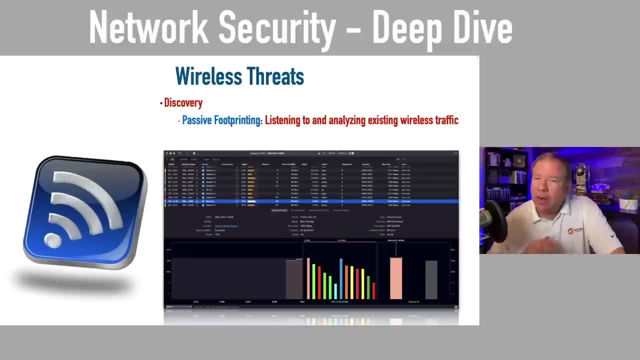 comes into an environment and they turn on the radio in their laptop, for example, and they just start scanning the airwaves to see what's out there. This is sometimes called passive footprinting. They're not actively sending any traffic out and trying to do malicious things, They're just. 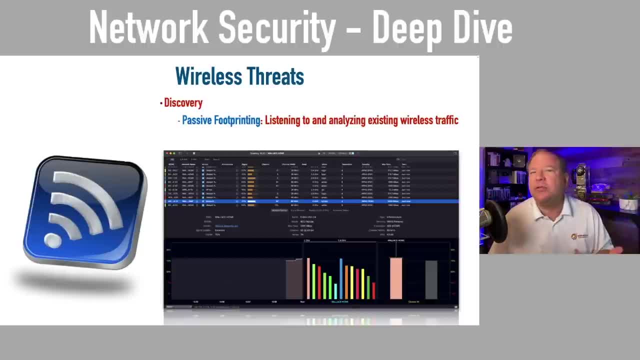 sitting back and watching and listening and understanding the terrain of the wireless network. What are the accesses, What are the access points, What are the MAC addresses or the BSSIDs of the different access points, What channels are being used? And by gathering that footprinting information, 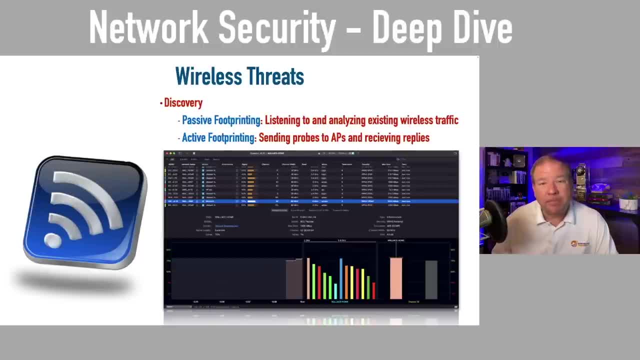 they might formulate an attack that they want to launch. They could also do active footprinting. This is where they're still trying to get a lay of the land, if you will, but they're practically sending traffic to an access point and getting replies from that access point to try to speed. 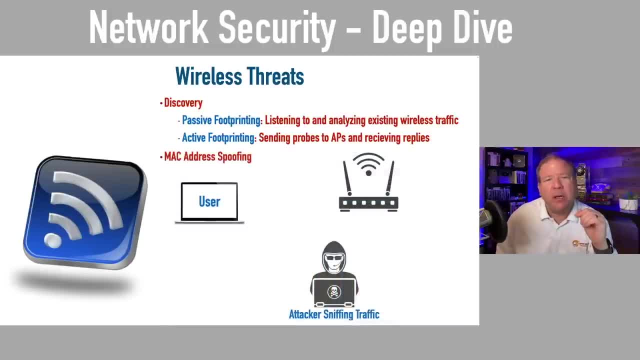 things up a little bit. We might also have an attacker that spooks the wireless network. We might also have an attacker that spooks the wireless network. Maybe we have wireless security set up that specific MAC addresses can get on the network and other MAC addresses cannot get on the network. Well, the attacker might set things up such that 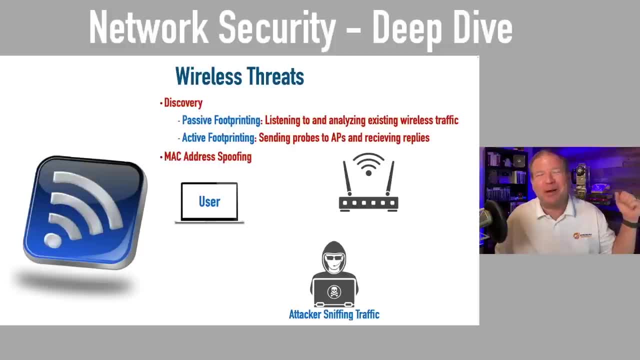 they're lying about their IP address. Earlier today we talked about spoofing an IP address. Well, they could be spoofing their MAC address And if they see that a user is going to an access point and they sniff that traffic, they say, oh, this user has this MAC address on their 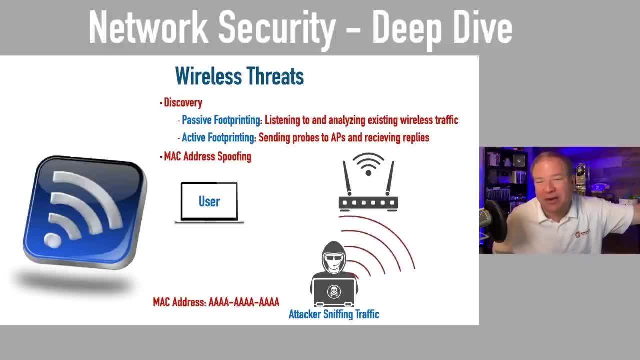 wireless network card. Well, I'm going to say that I have that MAC address now. I saw the user has it. The user had the old A's MAC address. I'm going to say I have the old A's MAC address, And then 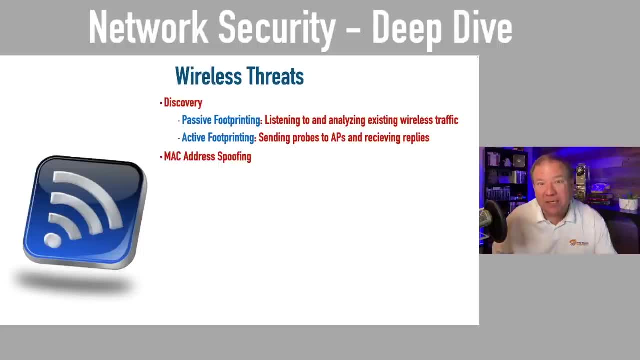 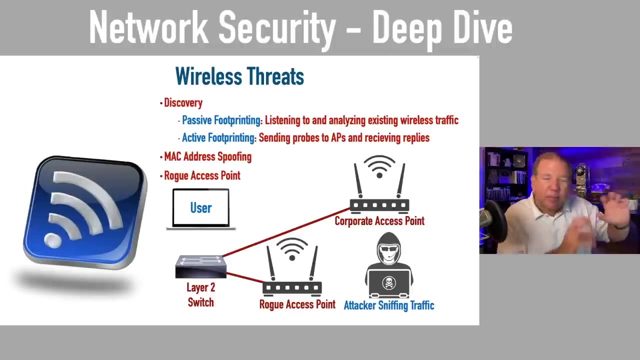 if we're using MAC address-based security, the attacker is going to be able to get on the network. Something else they might do is to insert their own rogue access point. They might hide it behind a desk or something where it's not obvious, or maybe a wiring closet, but they get connectivity. 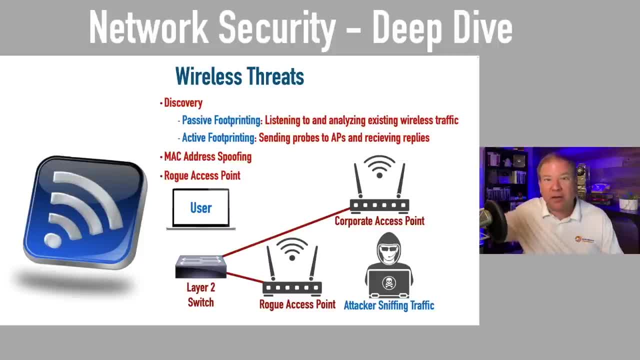 into the corporate network And then they can go somewhere else unnoticed and get access to that network. Maybe they're in their car out in the parking lot, but they put that access point up on the second floor and they can still reach that from their car. Yeah, they've inserted a rogue access. 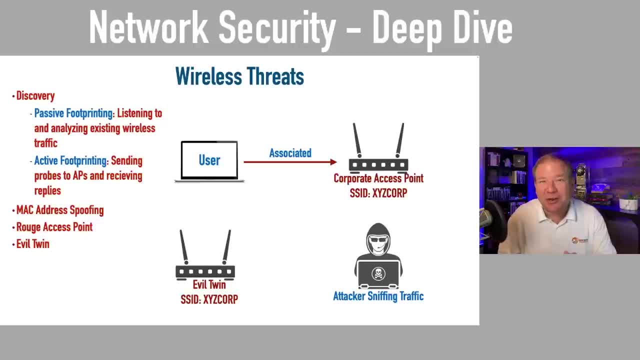 point giving them another way in to try to do dastardly things on the network. They might insert a wireless access point and have that wireless access point claim that its SSID is the same as the corporate SSID. That way when somebody goes to join the network and they see that, 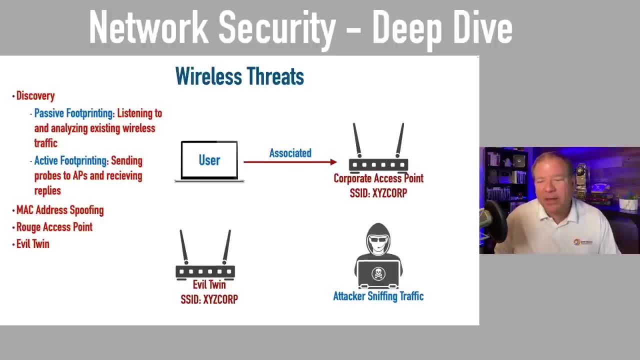 they're trying to join the network of XYZ. well, they might say, oh yeah, there's my network, I'm going to join that And a percentage of the time, they're going to be connecting to this evil twin. that's advertising the very same SSID as the legitimate corporate network. 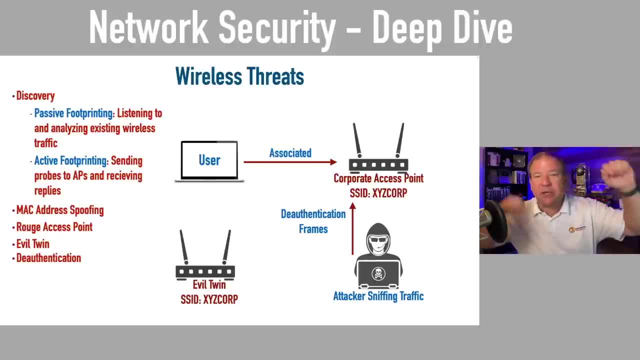 So what we might do, or what an attacker might do, is to send deauthentication frames to that access point, to knock off legitimate users, forcing them to re-authenticate and retry, to get back on the network And a percentage of the time- you guessed it, they're going to be. 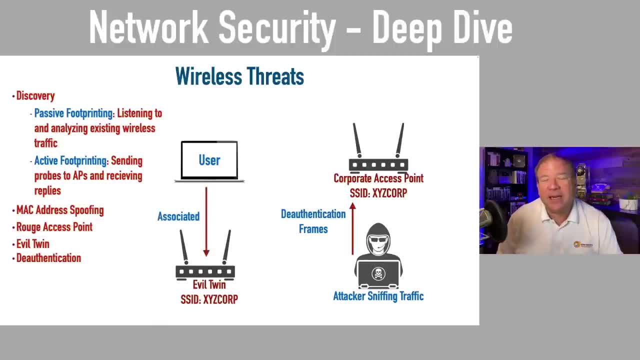 connecting not to the access point but to the corporate SSID. They're going to be connecting to our evil twin and become associated with that, where the attacker can then capture those frames. We talked earlier about deauthentication, where we could also capture that four-way handshake. 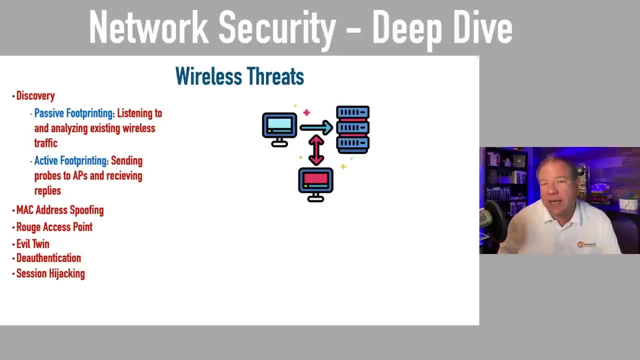 That's another deauthentication threat And we could run a brute force attack against that four-way handshake and determine what the password is for a user. They might also try to hijack an existing session. Session hijacking is going to be where somebody is already authenticating their network. They're going to be trying to hijack an existing. 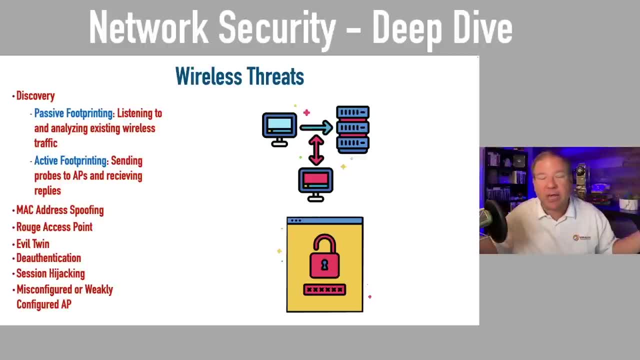 session. They've already authenticated with an access point, They've already provided their username and password credentials or whatever they're providing, And since they're already at that point, the attacker might just hijack that existing session instead of trying to figure out what the password is on their own. And one thing that we can do is better protect and better secure. 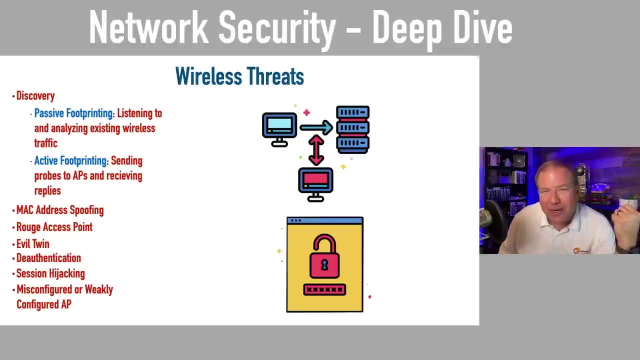 our access points. We don't want to be using default passwords. We don't want to say Linksys, Linksys, for example, in our home router as the username password combination. We want to use strong security and strong access points. We don't want to be using strong security and strong. 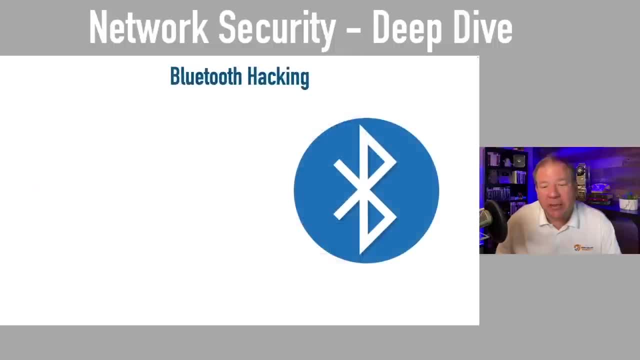 passwords. We'll be talking about those in this module. But in addition to wireless hacking in the Wi-Fi context, we also have Bluetooth hacking. I showed you earlier this little Ubertooth 1 adapter. This is something that lets me communicate for my PC using Bluetooth. 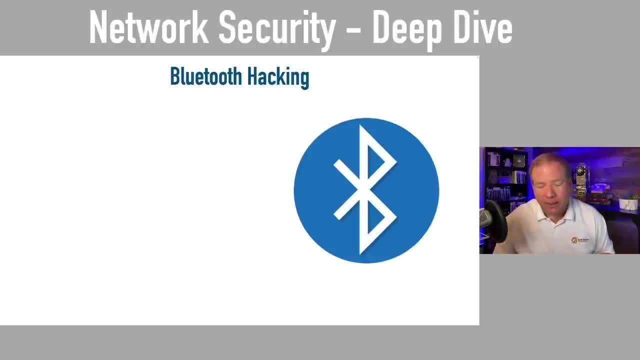 And in that professional ethical hacking course I was telling you about, I actually do a demonstration where I have this plugged into a machine running Kali Linux and I'm sniffing the Bluetooth environment And I'm sniffing the Bluetooth environment And I'm sniffing the Bluetooth. 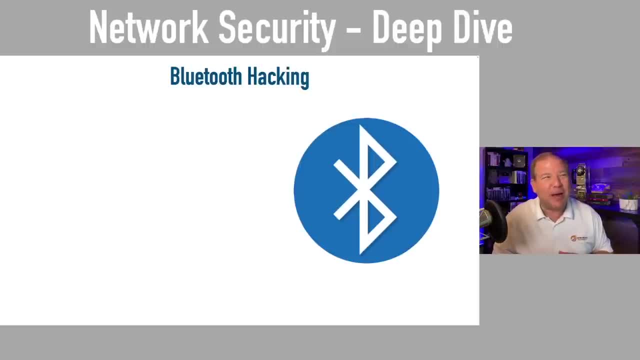 environment around me And to my surprise, it picked up my Ember coffee mug. I've got a coffee mug in my kitchen that can be controlled with an app where it keeps the temperature at a certain level, And I was able to detect that showing up on Bluetooth. So Bluetooth hacking- there are a few. 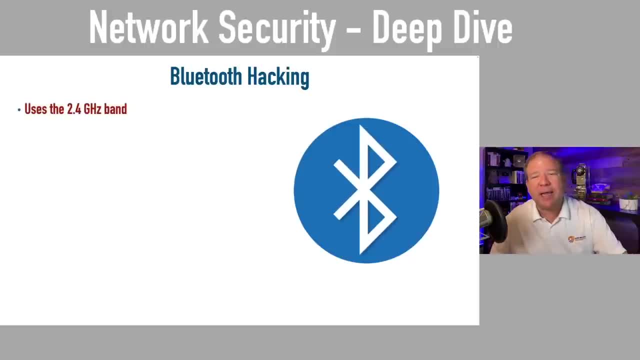 different flavors of Bluetooth hacking and we'll talk about some of those. But Bluetooth overall uses the 2.4 gig band And it's typically a one-to-one communication where one device, like my gaming controller, is talking to another device like my gaming console Or maybe. 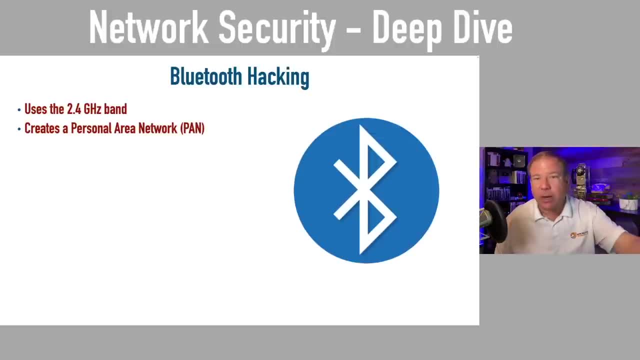 my phone is talking and my car is talking to my car's audio system using a Bluetooth connection. Examples of Bluetooth devices include things like your mobile phone, or here I have my Apple AirPods Pro that I put in my ear when I'm exercising and they connect to my exercise. 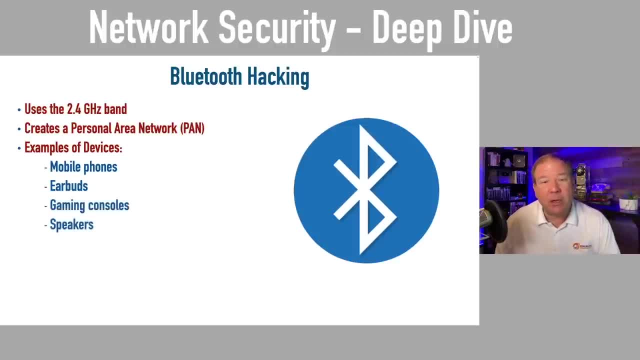 equipment via Bluetooth. We mentioned gaming consoles. We've got speakers, I've got some outside speakers And, yeah, I use Bluetooth for that- And I've noticed that if I have those outside speakers they're out by our pool area If I put my phone too far away. 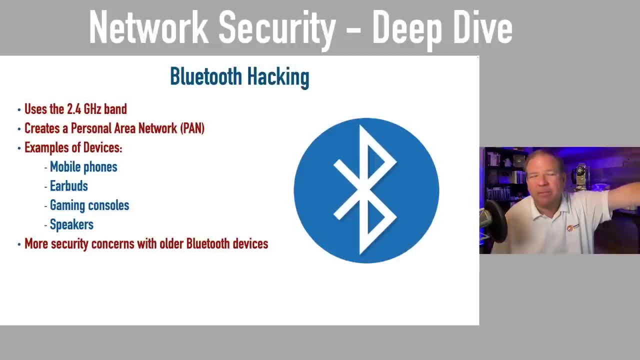 like on the other side of the pool or put it underneath a bunch of stuff that blocks that Bluetooth signal. Bluetooth signal doesn't go all that far And, yeah, it starts breaking up the audio. when I do that. Most of the security concerns. the good news is is usually with older Bluetooth. 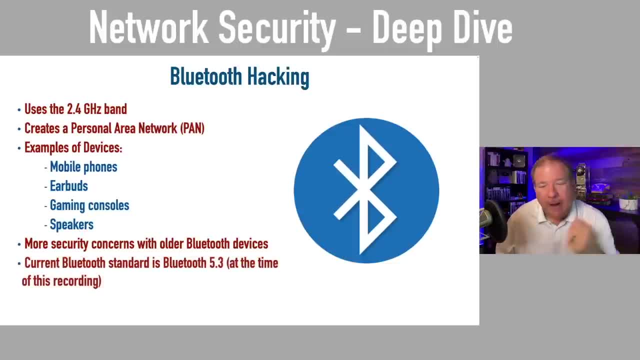 devices where we could do some things that maybe we shouldn't be doing. But let's take a look at some of the threats we might have with Bluetooth. And, by the way, the range isn't all that far. It's typically about 30 feet, about 10 meters or so, But one 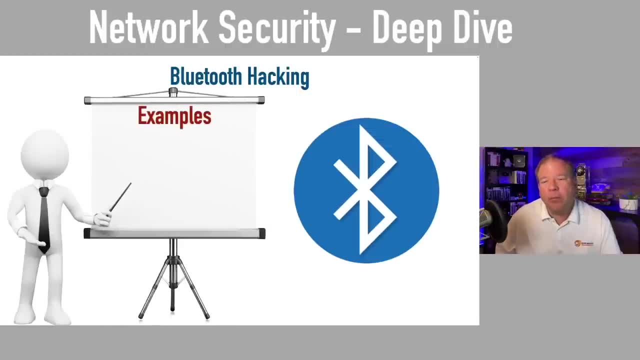 type of Bluetooth hacking is called blue jacking, And with blue jacking the attacker is sending information to a device. For example, I want to insert, maybe, a new contact card in somebody's contact list. Well, that will be an example of blue jacking, Blue snarfing. 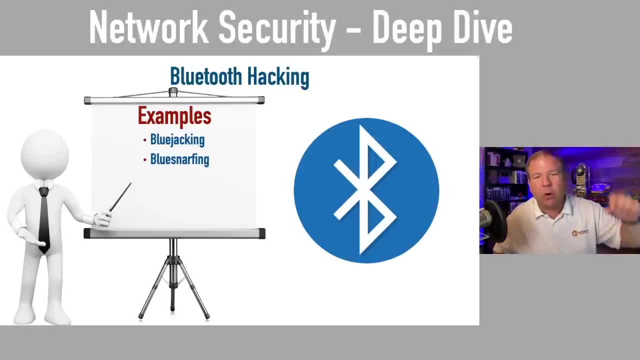 that's where we're learning information about a device. We're sort of doing some reconnaissance on that device and gathering information about that device. We could also launch a denial of service attack on that device with blue smacking. Blue bugging, as the name suggests, allows us to. 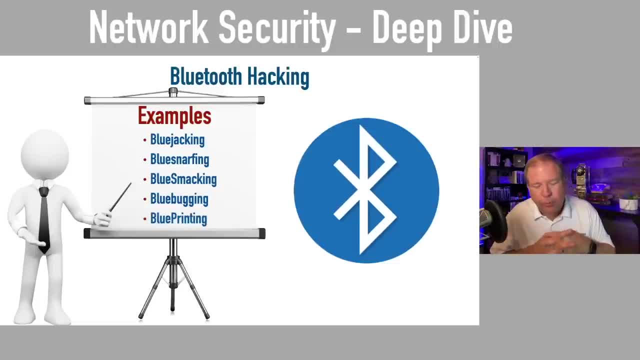 eavesdrop in, maybe on a phone conversation, And blue printing- that's where we're learning- is sort of a passive surveying. We're just sort of getting a blueprint of the Bluetooth landscape, Blueprint Bluetooth. no pun intended there, But I'm just learning what's out there with. 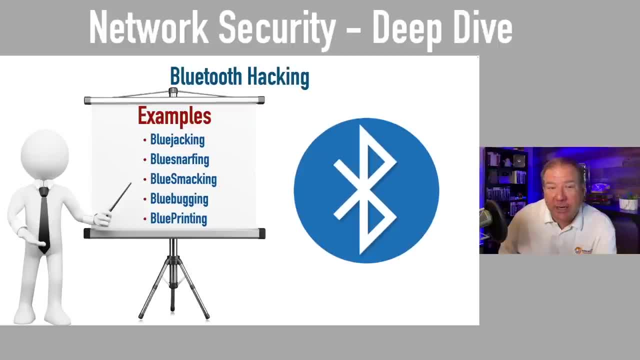 blue printing. But those are some of the things where we can inject data on a device, like a phone with blue jacking, gather information about that device with blue snarfing, blue smacking, launch a denial of service, attack, blue bugging- eavesdrop in blue printing. 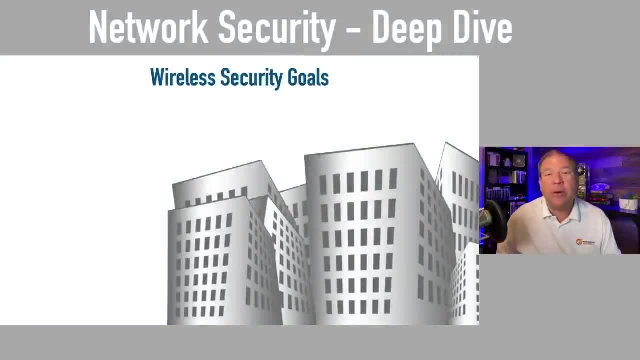 just sort of survey the environment. Now let's talk about how we can defend against different types of wireless attacks. And, getting back to our Wi-Fi discussion, let's say that we've got the goal of not wanting somebody to eavesdrop in on our data, or we don't want them to gain access to the network if they should not. 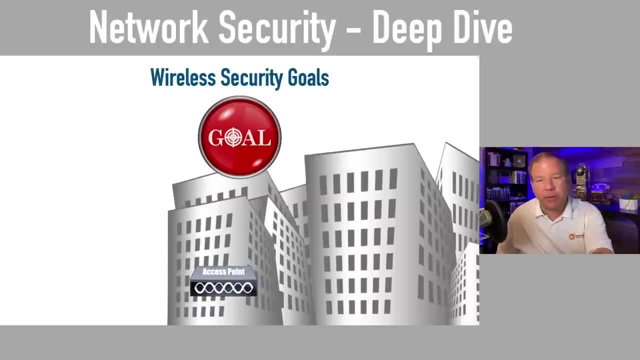 have access to the network And let's say I've got this access point in my building. Would you, let me ask you this: would you ever put an ethernet port on the outside of your building and let somebody drive up in their car and maybe plug into that ethernet jack? 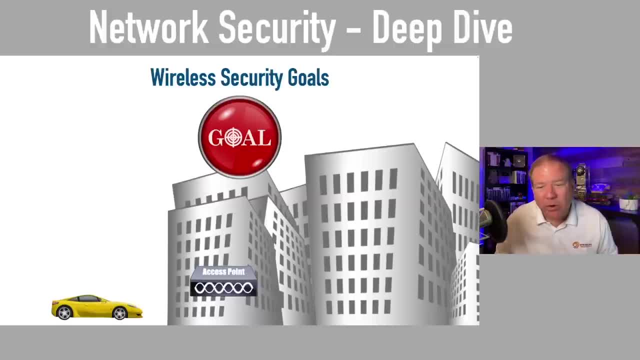 No, I would not be secure with it, But that's essentially what we're doing. if we have a weakly secured and poorly placed access point where the signal might extend out into the parking lot, Somebody could drive up and they could get access to the corporate network. 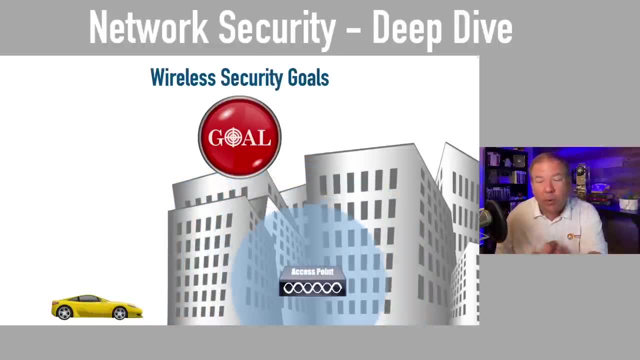 To prevent that, we might want to reposition the access point, We might want to reduce its power level so the coverage area doesn't have as big of a radius, But we want to make sure that somebody is going to have to authenticate themselves before they can gain access to. 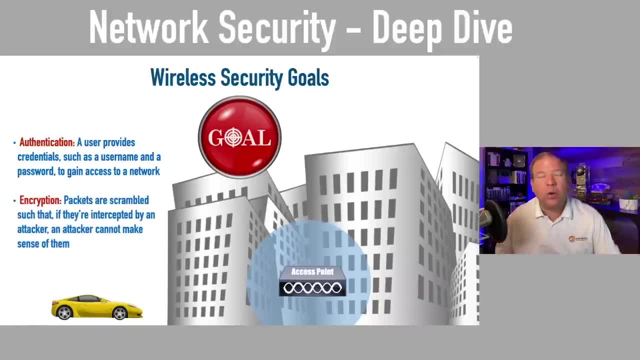 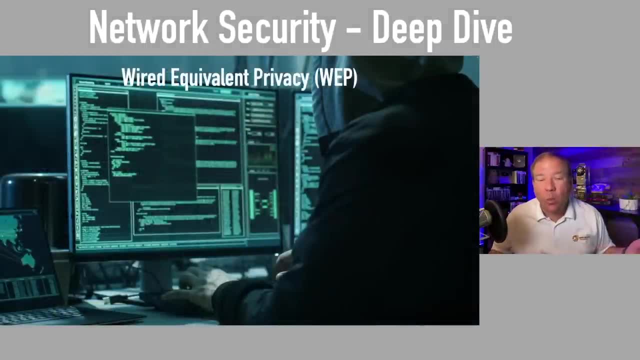 the network More than just having access to the signal. And once we're transmitting data on the network, if somebody were to eavesdrop in and capture that data, we don't want them to be able to do anything with that, So we want to encrypt it much like we talked about earlier. 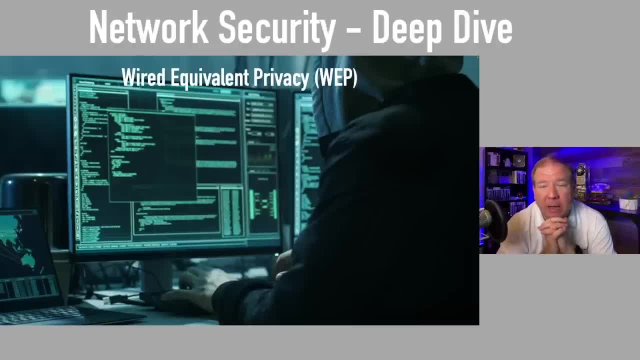 And there are several different wireless security standards out there. Let's go back to the original one. The original security standard for wireless networks back in the original 802.11 specification was something called WEP. That stands for Wired Equivalent Privacy. Now the name is a bit misleading, I think. 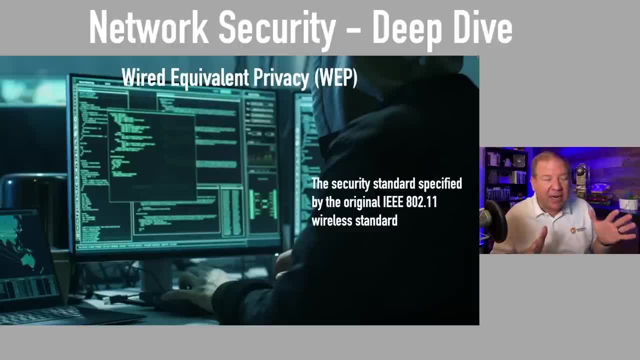 Wired Equivalent Privacy to me sounds like we're saying this is equivalent to being on a wired network. That's the level of privacy you get, Poppycock. It is not anywhere near the level of privacy you get on a wired network, In fact. 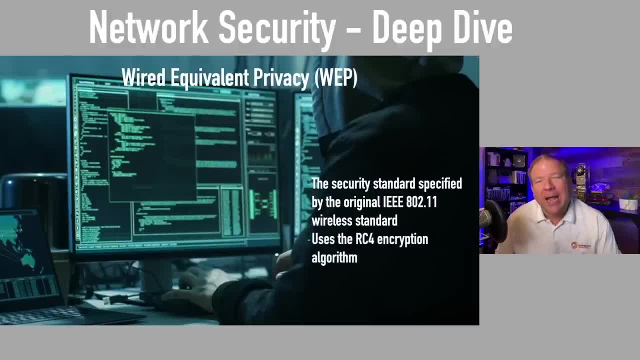 this is a very, very weak security standard. It uses the RC4 encryption algorithm, and that stands for Ron's Code 4.. And The issue isn't with Ron's Code 4, it's the issue with how it's implemented. 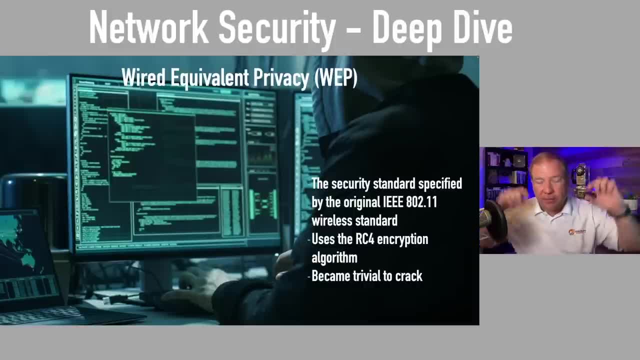 You see, RC4 is going to take the string of data that we're trying to secure. it's going to take our pre-shared key and it's going to take something called an initialization vector, an IV, and it's going to mathematically mush all that stuff together. 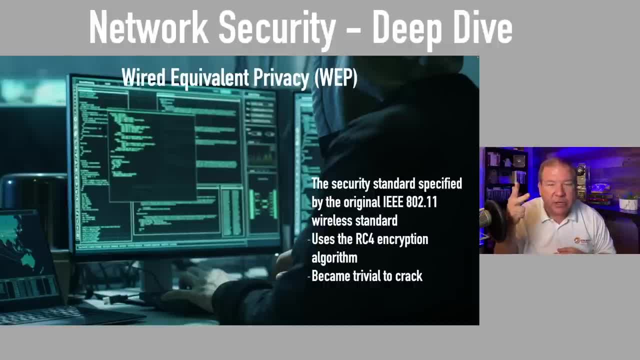 Again the string we're trying to encrypt, the pre-shared key and the initialization vector. And the problem with RC4 is it uses a very short initialization vector. It's only 24 bits and it's not long And that might sound like a lot, but you can in an environment with a decent. 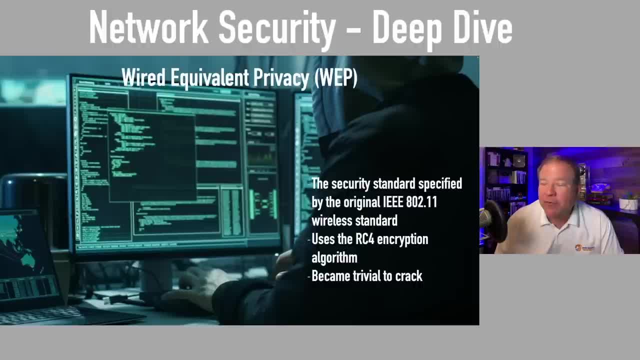 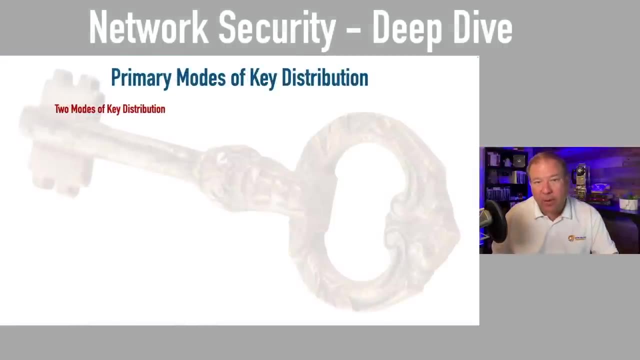 amount of traffic on a web network. if you capture traffic for about 8 minutes, there are utilities out on the internet that can take those captured packets and determine what the pre-shared key is in about 8 minutes. That just blows my mind. Now that was with a pre-shared key, Remember. 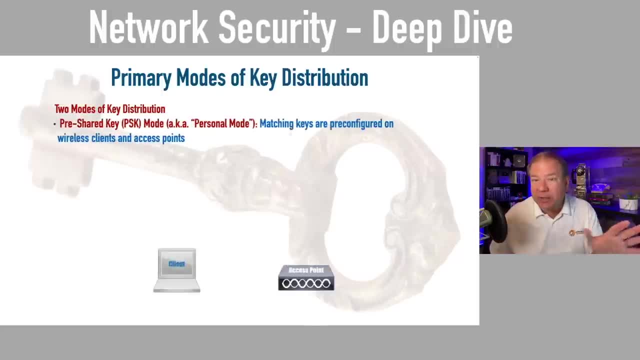 earlier we talked about having a symmetric key. That's kind of what a pre-shared key is. We go to the client, we go to the access point and we give them both the same key. So if you want to add a new device to your wireless network, somebody gets a new phone. you put in the pre-shared. 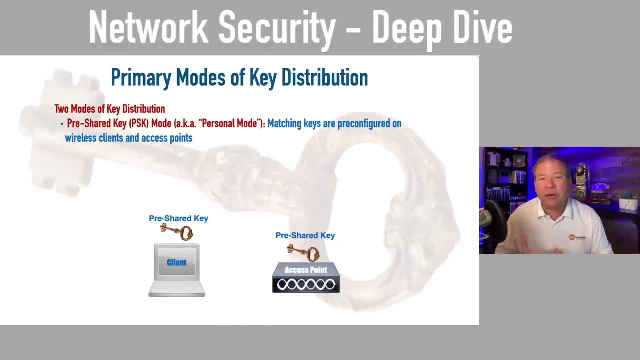 key that everybody uses and that pre-shared key is going to be used with whatever encryption algorithm we use to encrypt the data. Again, this is not going to scale very well If we had an enterprise environment with hundreds or maybe thousands of users. we don't want to give everybody. 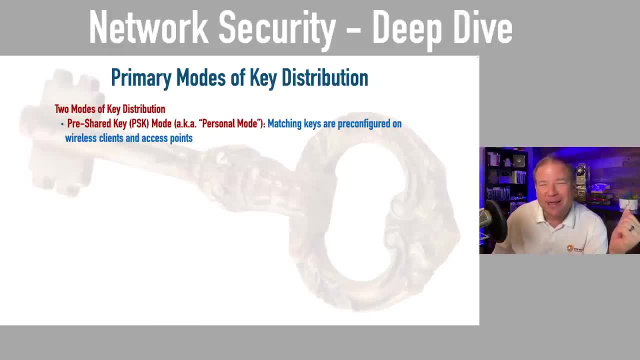 the pre-shared key. That could get lost or somebody might get lost, So we're going to give that away. That's not a good thing. So in a large environment we want to use not the pre-shared key or personal mode. We want to use something called enterprise mode. Here we have 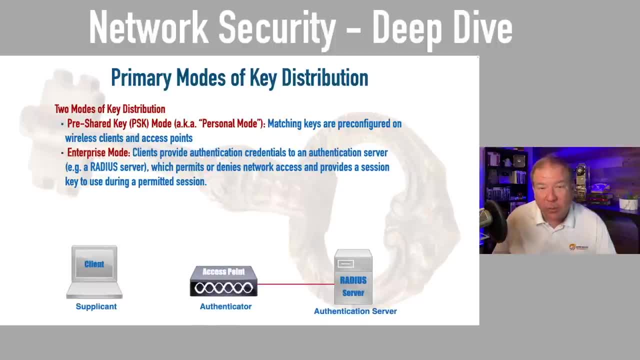 an authentication server like, typically, a radius server. We talked about radius earlier And this is really 802.1X that we mentioned, 802.1X, which we could use with a switch or we could use with an access point. it's got really three roles that are played here. One role is that of the device. 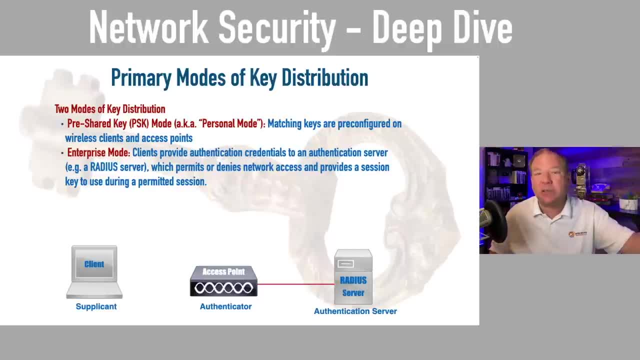 network. That's called a supplicant. To supplicate is to ask for something, So the supplicant is asking permission to get on the network. The authenticator- and I think that name is a little bit misleading as well- That's the switch or, in this case, the access point. The authenticator is: 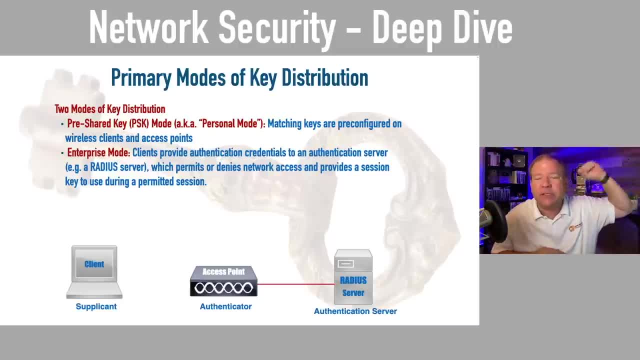 just sort of the relay that's taking these messages coming from the supplicant and it relays them over to our radius server And the radius server that's our authentication server. So the supplicant tells the authenticator: I'd really like to join the network. 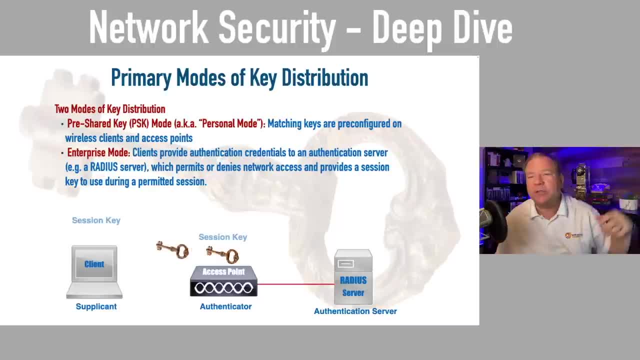 The authenticator sends that over to the radius server and the radius server, if we've provided the appropriate credentials, the radius server is going to create a key just for me and just for that session, And it's going to give a copy of that key to the authenticator. the access point. 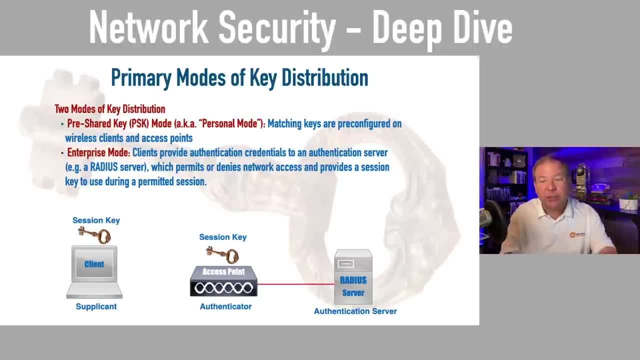 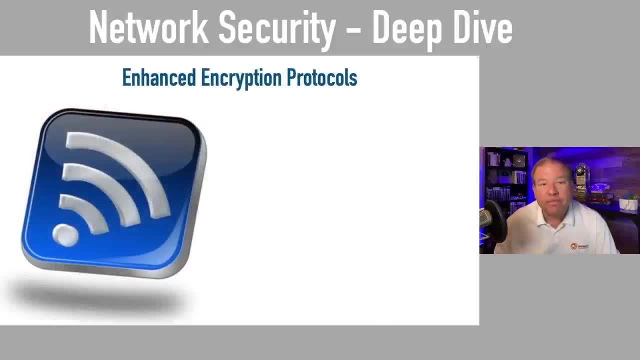 and to me the client And for the duration of that session, the client and the access point. they're going to be using that symmetric key pair to encrypt their data. But again, we don't want to use RC4 with 24-bit initialization vectors. That's going to. 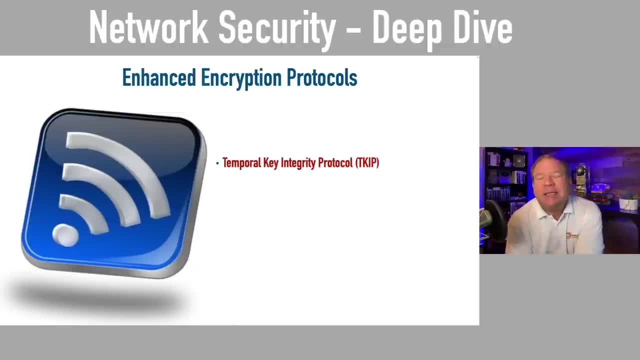 be very weak. Well, an improvement to that is TKIP. That stands for Temporal Key Integrity Protocol. This got popular after WEP was determined to be just so incredibly weak. With TKIP, we're still using RC4, but don't be discouraged: We're using a better version of RC4, making it. 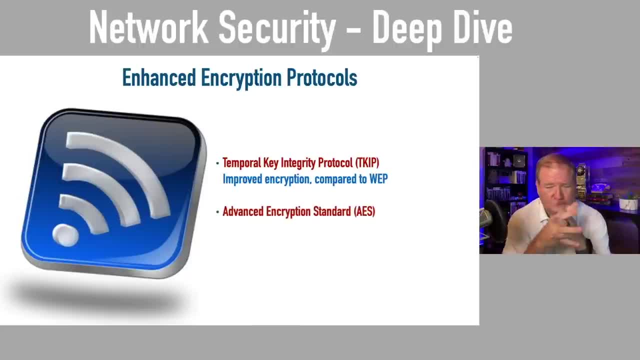 much more secure than WEP. Specifically, we're using a 48-bit initialization vector. Now you might say: well, Woo, we're using a 48-bit initialization vector. Well, we're using a 48-bit initialization vector. We went from 24 to 48.. Does that mean we're twice as secure? now It's. 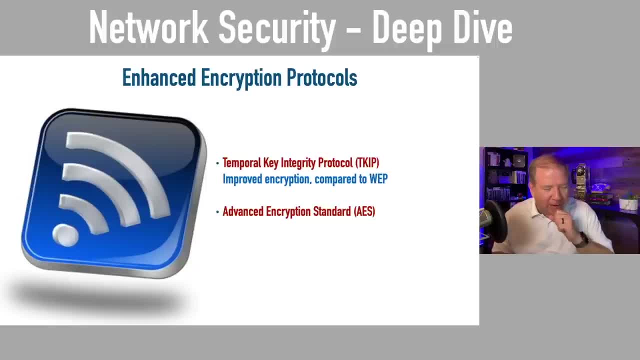 going to take 16 minutes instead of eight to break into the network? Not at all. You see, when we go from 24 bits to 25 bits, that doubles the security. We go to 26 bits, that doubles it again. So if we go from 24 to 48 bits, we are orders of magnitude more secure than we were. 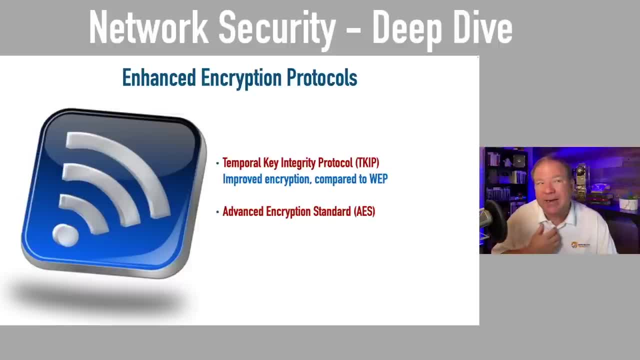 before And TKIP does not require a great deal of processing on the part of the wireless network card. So it was a great compromise For older devices that didn't have a lot of horsepower on their wireless interface card, while still giving us better security than WEP. But remember, we mentioned AES earlier. I said 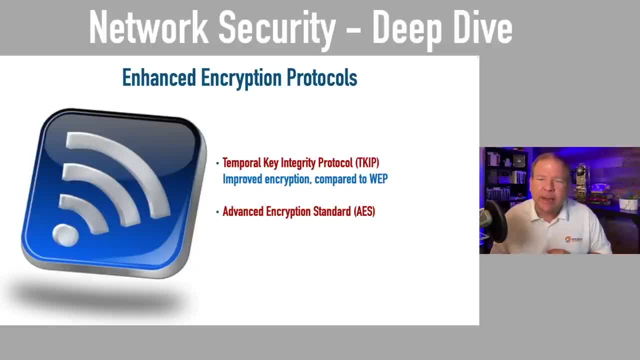 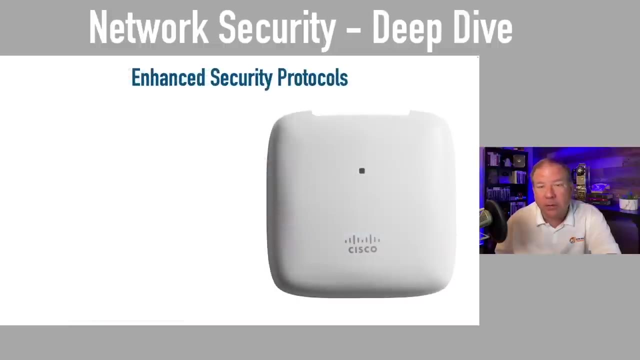 that's really the flagship encryption algorithm that we want to be using today. Yeah, it's better if we use AES. That's going to be better than TKIP and just insanely better than WEP was. But AES does take some extra horsepower. It takes some extra processor cycles for the clients or the access. 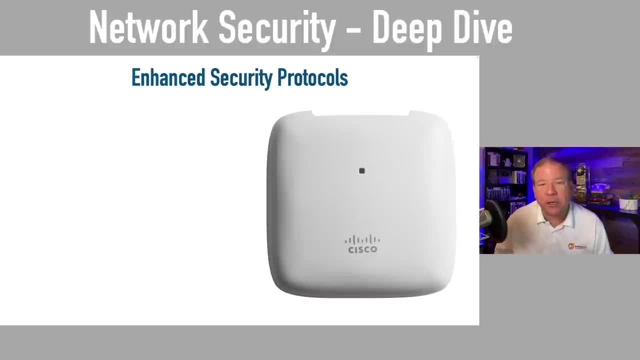 points or any wireless device to process. So it's going to be a great compromise To process that encryption. So when you're setting up your access point, you may be presented with a set of security standards: WPA, WPA2 and WPA3.. Now WPA: that stands for Wi-Fi Protected Access. 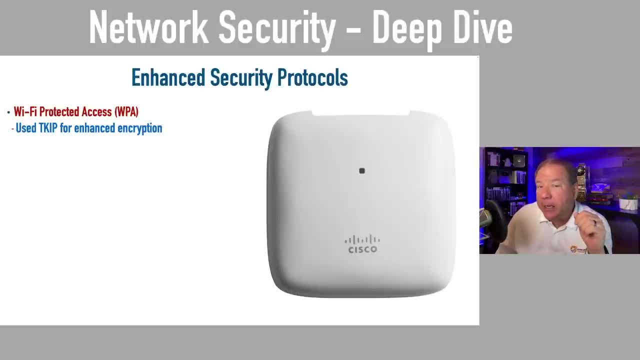 And the original WPA. it did use TKIP. That was good in that it supported some older devices that didn't have a lot of processing power, but it was better than WEP. So we got to preserve our investment in existing hardware. So we got to preserve our investment in existing hardware. 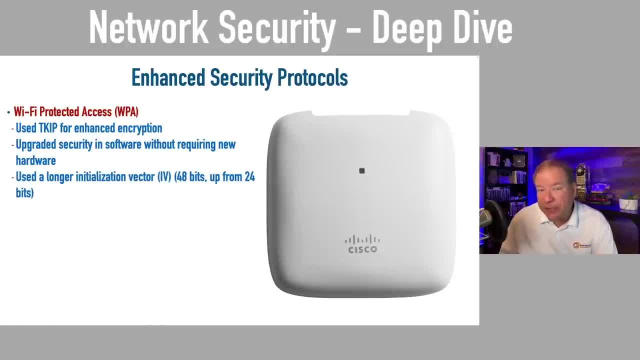 And remember, TKIP uses that better initialization vector: 48 bits as opposed to 24 bits, But still it's TKIP. It's still weaker, far weaker than AES. So Wi-Fi or Wi-Fi Protected Access or WPA2 came. 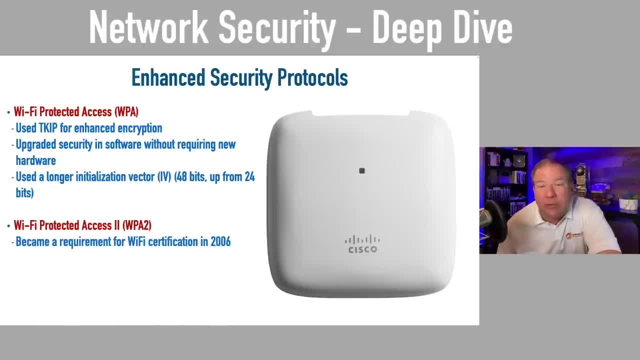 out And for over for about a decade or so, that was the end-all be-all of wireless security standards. You're setting up an access point. you better use WPA2.. In fact, the Wi-Fi Alliance that allows vendors to put their devices on WPA2, that's the end-all be-all of wireless security standards. 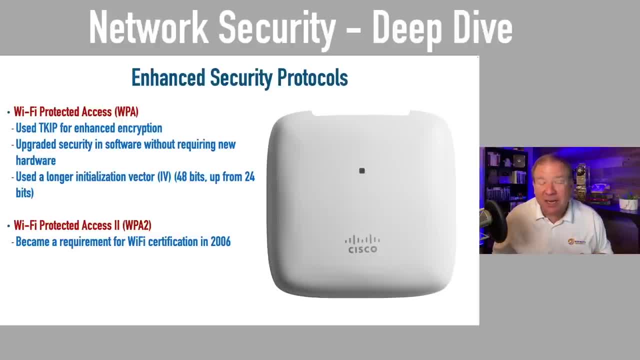 They put the Wi-Fi sticker on their device In 2006,. they said it's a requirement If you're going to, if you're going to be certified with the Wi-Fi Alliance, your WPA2 must or your device. 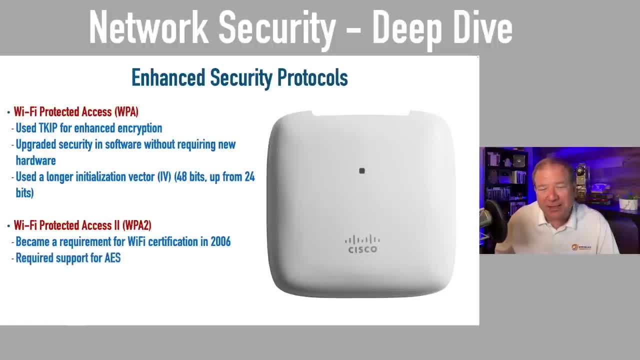 must support WPA2.. So they're pretty serious about this, And a requirement for WPA2 was that it had to support AES, that Better Encryption Standard. But notice the wording here. It had to support AES. It didn't necessarily mean we had to run AES. 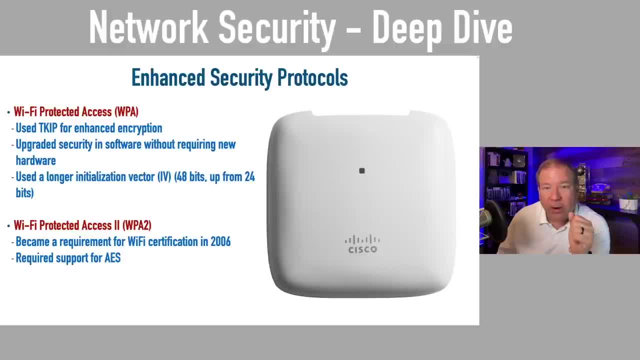 And this could vary depending on our hardware, the vendor. But in some cases you could be running WPA2, but you said: I've got all these old devices, I don't want to have to have to run AES My devices. 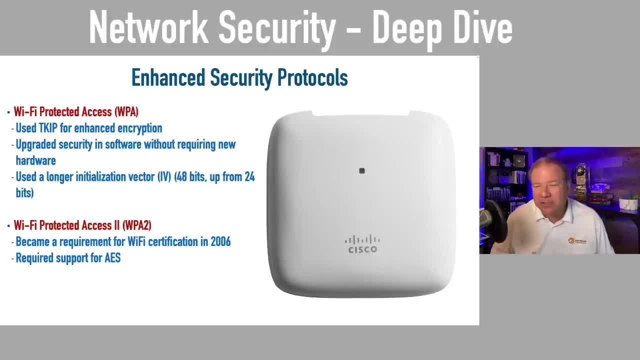 cannot handle it Well on some systems. you could tell WPA2 not to use AES, even though it could support it, and use TKIP instead. Or you could say just use AES, Or you could say: use either one, Let the client decide which one we're going to be using. But AES, it does require more. 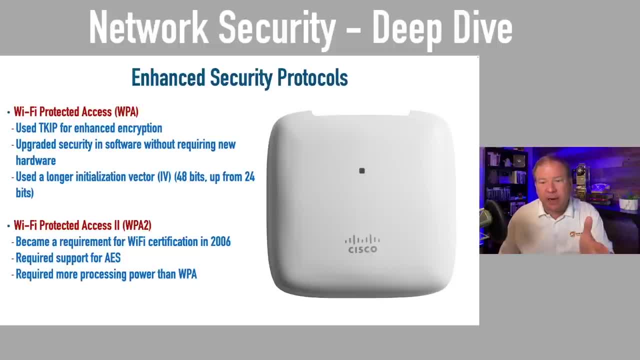 processing power than WPA. But over the years- I mean this has been out for a while- Over the years, more people will get more and more modern hardware with better processing And for, like I said, a decade, this was the go-to wireless security standard out there until 2016 happened. 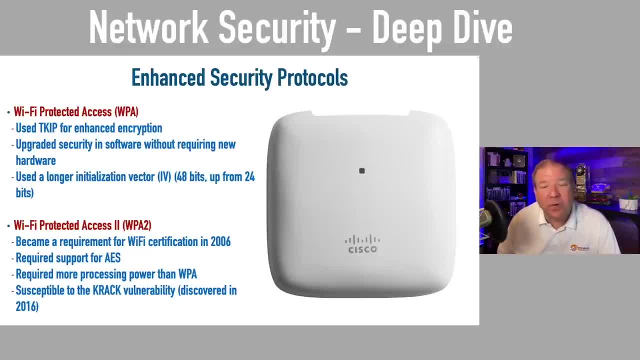 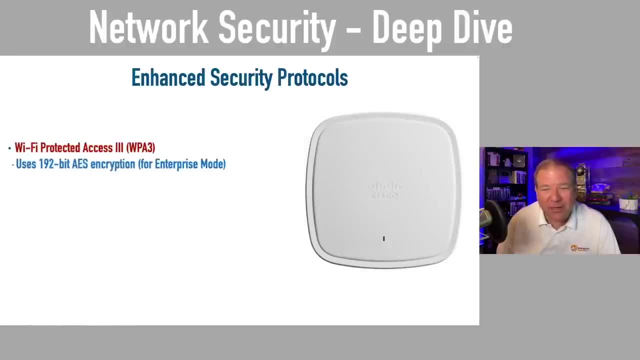 In 2016,, there was a vulnerability discovered with WPA2.. It was called the crack vulnerability. So, yeah, now we have WPA3.. It's what is going to be preferred. This is WPA2.. We're going to use just AES, no TKIP, And if we're in personal mode, we're using 128-bit AES keys. 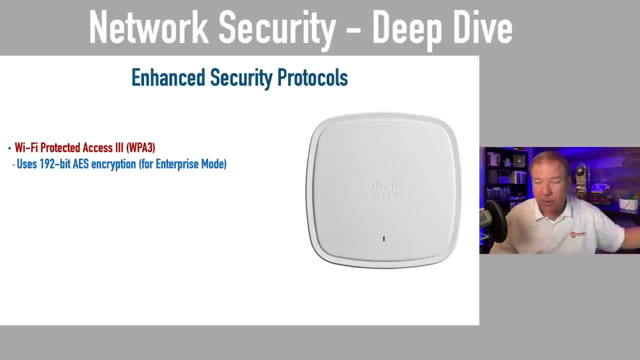 But if we're in enterprise mode with the radius server and .1x, we have 192-bit keys. So we get even more secure with AES. And remember we talked about those deauthentication frames that we might send or an attacker might send to knock somebody off of an access point. We're protected against. 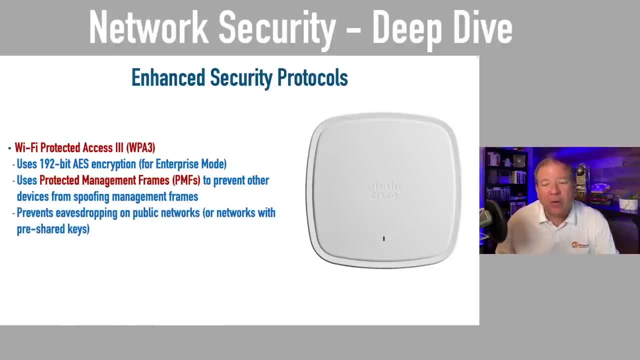 that with WPA3. And we also are going to use WPA2.. And we're going to use WPA3. And we're going to be more secure on publicly available networks, like you go to the airport or a coffee shop. 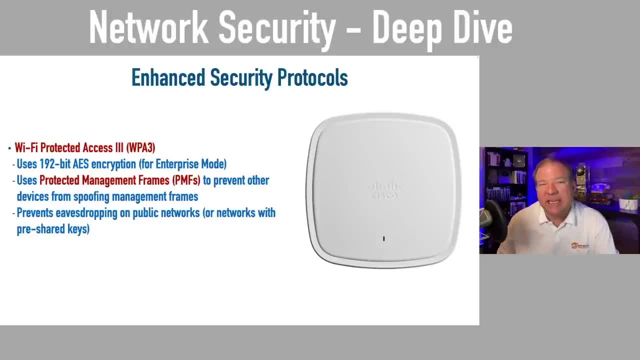 and you're on a public Wi-Fi. Yeah, instead of somebody just eavesdropping in, you're going to be better protected with WPA3.. And also, there used to be a button on the back of a lot of these home wireless access points that you might get from your big box store. It was labeled WPS. 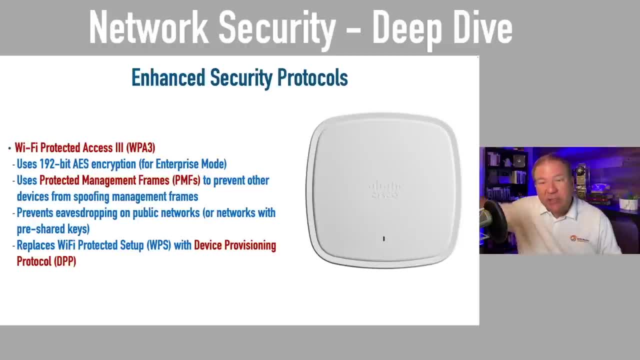 You would press that WPS button, And that was a way to easily go add another device to the network without having to key in a bunch of password information. Well, there was a weakness in that as well, So that I don't want to say, I want to say automated setup, but an assisted setup, I guess. 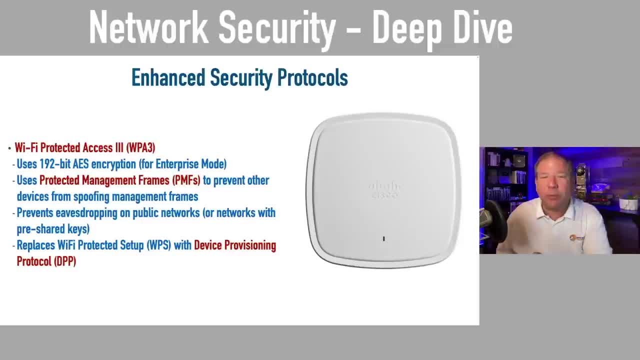 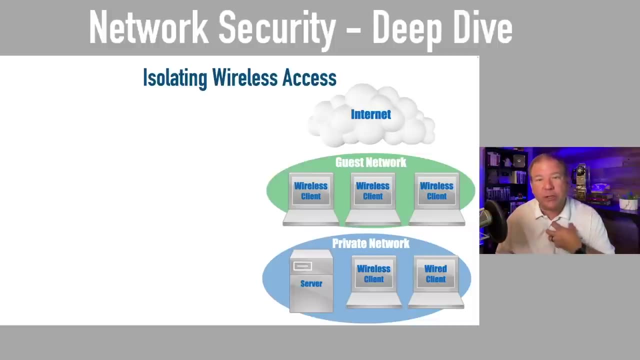 that's a better way of saying it. There was a different assisted setup process that was introduced with WPA3. that replaced WPS And it's called DPP device provisioning protocol. Something else we could do is have a separate guest network for people that come into our organization And they 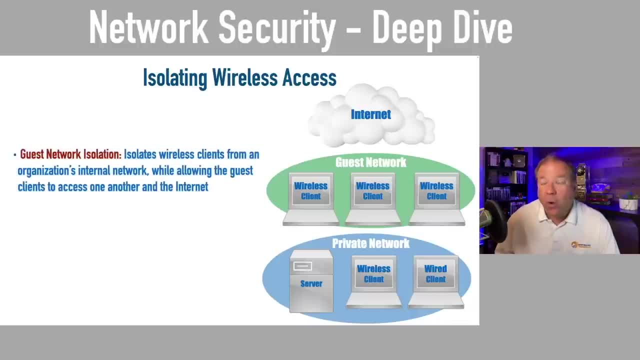 were isolating them to their own guest network, Or we might not want one guest to see what another guest is doing. So we can even give some additional protection for those guests by isolating individual wireless clients in that guest network So one guest client cannot eavesdrop. 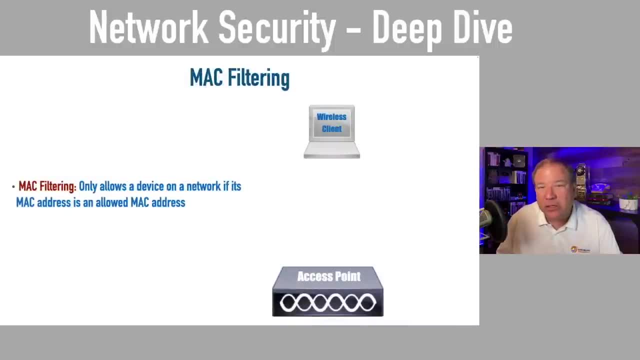 in on another guest client. We might also do MAC address filtering. Now, this is not super strong, but it's a layer. Remember the blankets on the cold winters. It's a layer of security. We might have a MAC address filter that says: in order for a wireless. 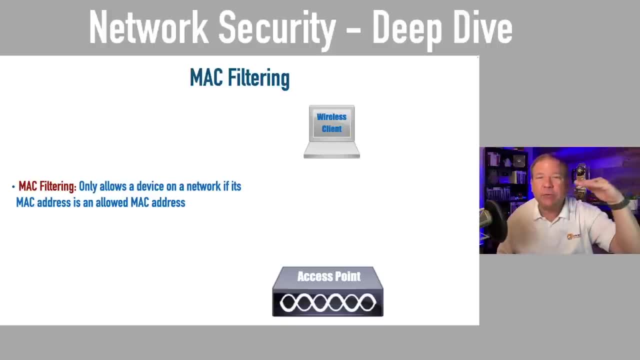 device to attach to this access point. it has to match one of the MAC addresses in this list And if it doesn't hold up a big stop sign and say, no, thou shall not pass And we're going to drop that traffic Again. it's not super secure because we can fairly easily falsify what MAC. 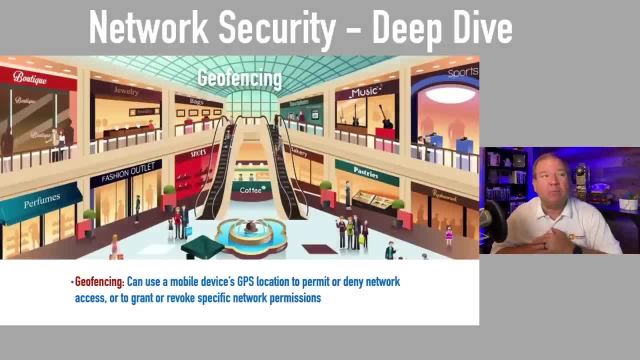 address that we're using. We also talked about being authenticated based on where we're are. We mentioned the term geofencing. That's what we could do, maybe in an environment that has a bunch of different vendors, like in a shopping mall. We've got all these different. 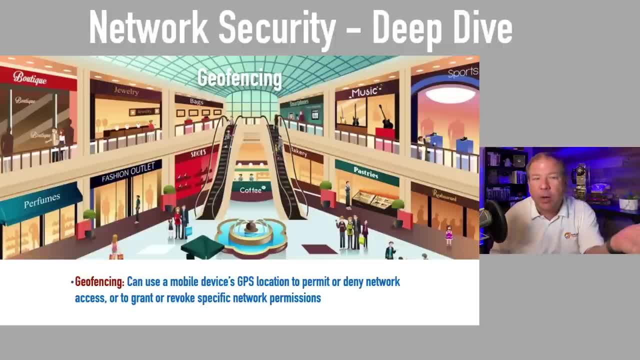 stores And maybe you're going to be given a coupon based on your proximity to a store. This has happened to me. I've been in a big shopping area and I'll get a pop-up message saying that some sort of discount coupon on this store that I happen to be standing in front of. 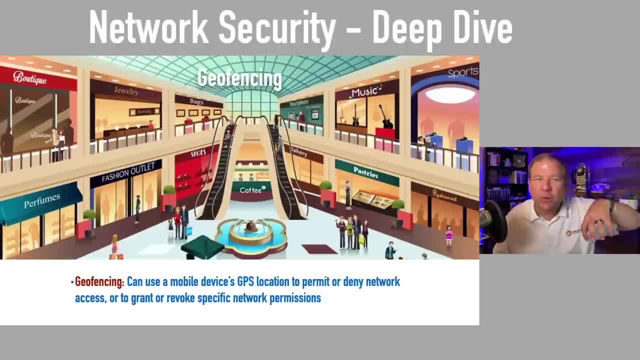 right then. So maybe based on our geographical location, we can or cannot get access to certain things, Or before we can. I think I mentioned the example of checking in on a cruise ship. I had to be in close proximity with that cruise ship. 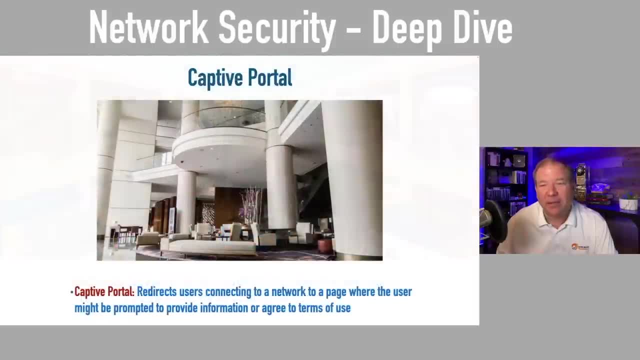 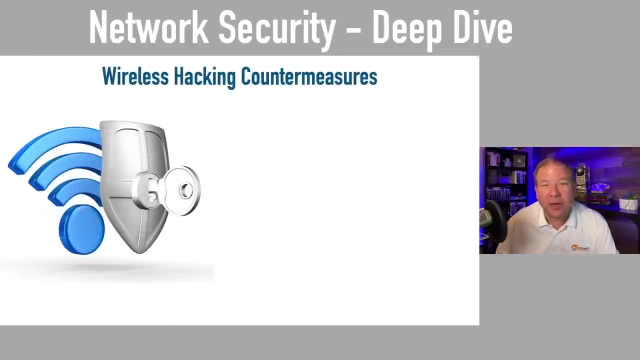 in order to be able to get on their network. We also talked about a captive portal. You might see that I gave the example on Delta Airlines and getting on their Wi-Fi Or in a hotel, you might be asked to give your account name, your actual name, and your password or your room. 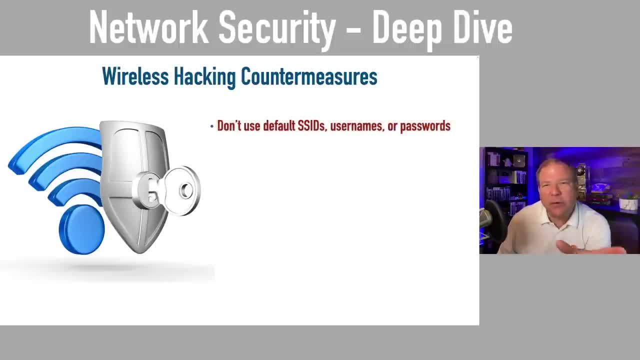 number as an example. Now something else, just another collection of best practices that we can use to better protect ourselves. Let's not use the default wireless network names that come with our access points, such as Linksys used to be the one. I think they've changed it since then, But you? 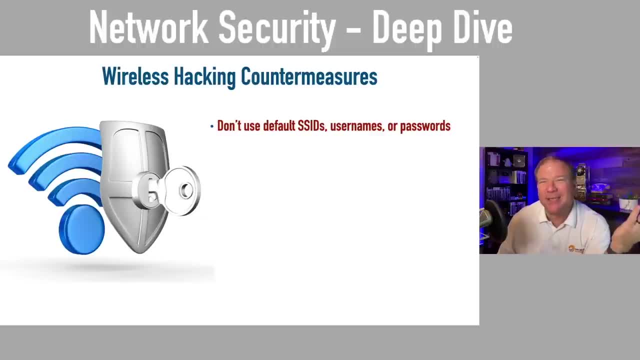 would go down and you'd buy a router from a big box store and it was Linksys And the password was Linksys or admin, admin or manager, manager or something like that, And those were well known, So it was very easy for people to get into equipment. 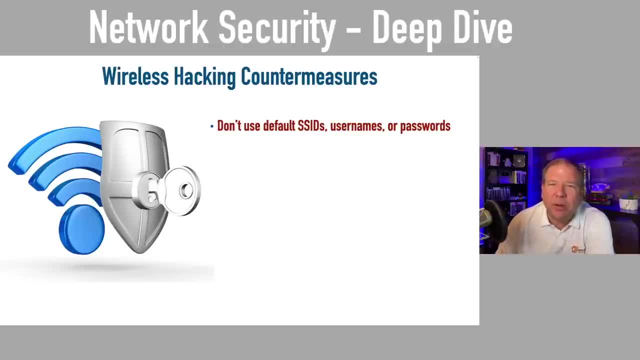 So let's change up the default wireless network names, the SSIDs, Let's change up the default username and passwords. In fact, again, this is not a high level of security, but it's a layer We might disable our SSID broadcasts. We might not even announce that this network is available. 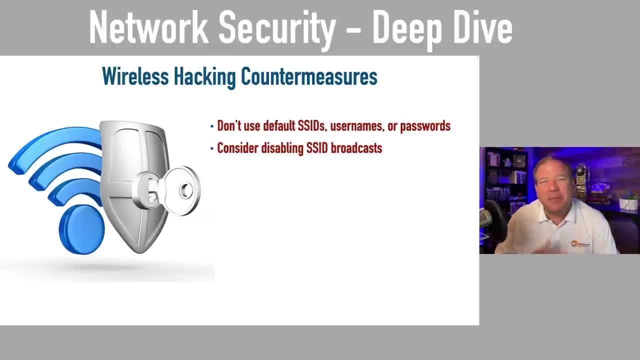 Now say it's not a super high level of security because somebody, an attacker, that's knowledgeable, they will be able to sniff the airwaves and they would still be able to see that SSID even if it was not being broadcast. And we talked about earlier how an attacker might introduce a rogue access point into the network. 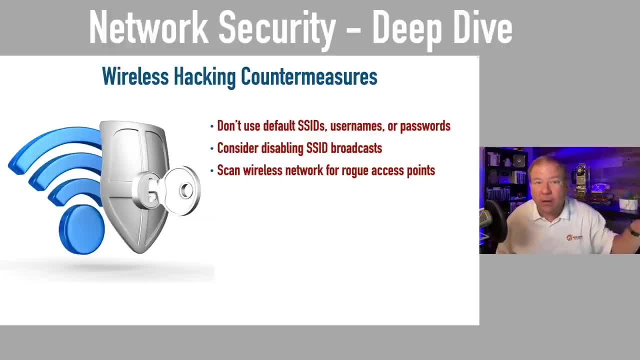 Well, there are scanners that a lot of the major enterprise level wireless enterprise level vendors have that will scan the network- Cisco does this- that can detect rogue wireless access points so you can locate and disable those And you might want to as part of that, you might want. 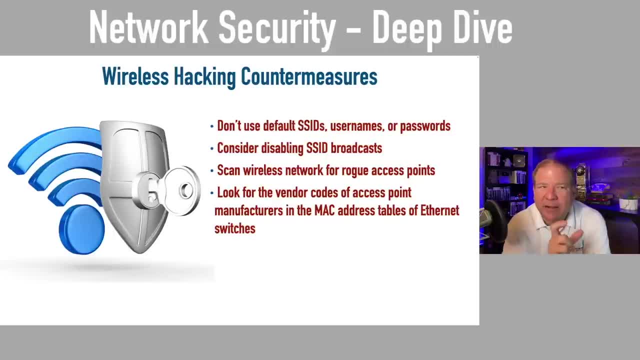 to make sure that you don't have to do that. You might want to make sure that you don't have to have any access points that have a vendor code that's different than the vendor you're using. If somebody inserts vendor X's access point into the network, that might be one way that we're 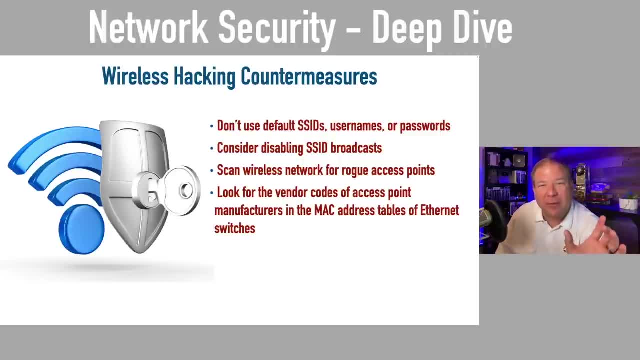 scanning for rogue access points. We're scanning the first half of the MAC address, the vendor code, to make sure we don't have some strange vendors access point in our network. And let's use strong encryption, strong authentication, at least WPA2, preferably WPA3, if we can. Other things we can do. 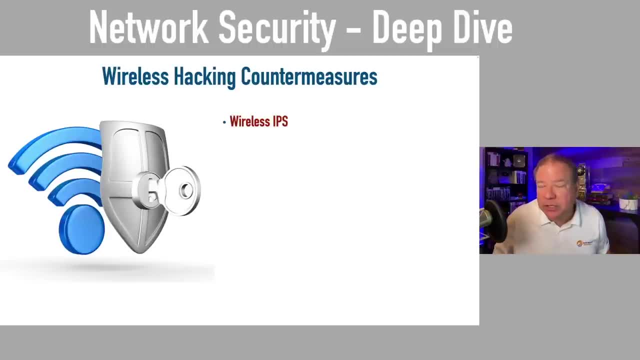 we can use wireless Intrusion prevention system sensors. That's right. What this might do is it could detect those evil twins where somebody is advertising the same network as the corporate network. It's going to try to detect somebody doing a wireless denial of service or a main in the middle or an on-path. 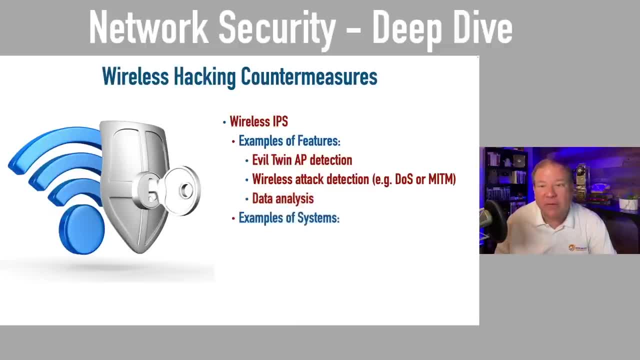 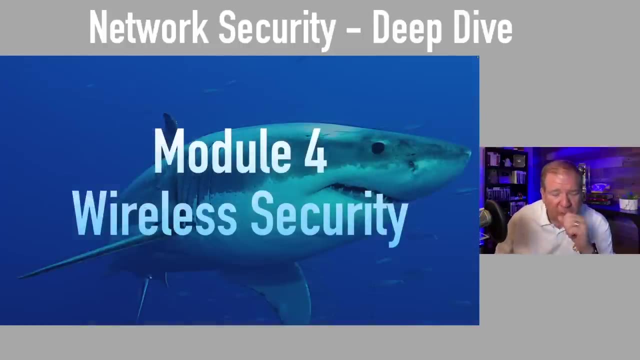 attack. It can collect and analyze data, give us a lot of analytics. Some examples of wireless IPS systems include Aruba's RF Protect Wireless IPS And Cisco has one called the Cisco Adaptive Wireless IPS. And that's a high level overview of some things we can do to better. 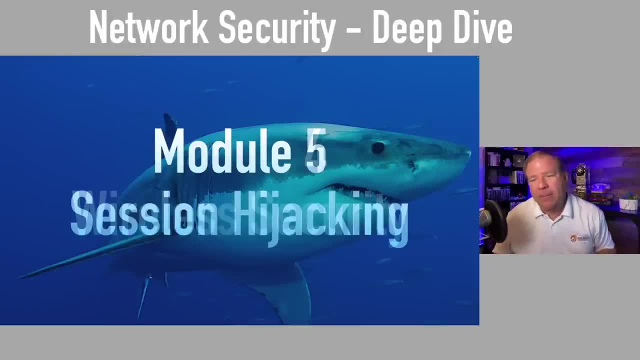 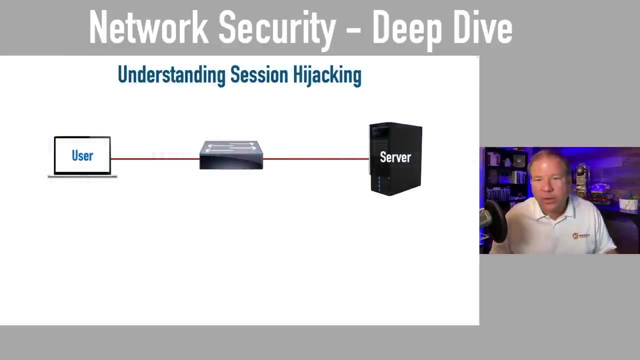 secure our wireless networks Now up. next, I want to talk about session hijacking, And I've hinted at this a couple of times already. With session hijacking, the attacker is letting the user go ahead and authenticate with whatever the target system is. So once they've, so once we've. 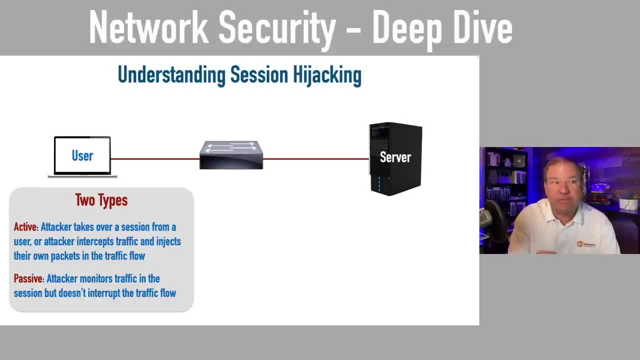 bypassed that authentication stage. the attacker just takes over that existing session. They don't have to authenticate because the user already did that And we just hijacked their session. Now that's an. that's an active attack, where we're going to take over a session from a user. 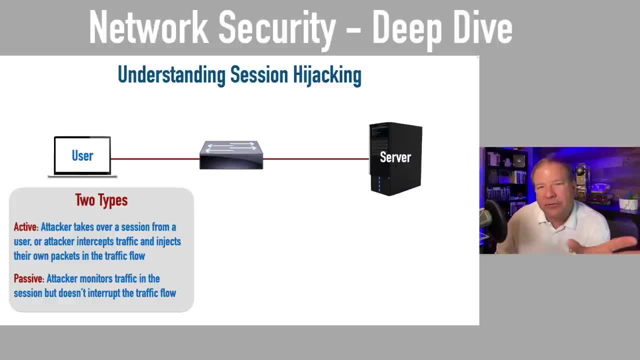 or we might do a passive attack Here. we're monitoring traffic in a session but we're not really interrupting the flow, but we've still hijacked the session. We're we're making the session flow through us as the attacker and we're monitoring it even. 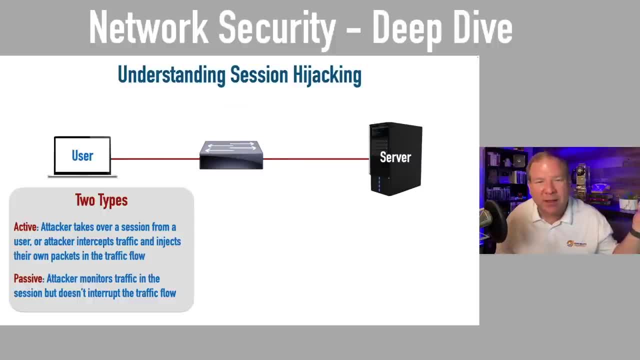 though we're not raising any red flags, we're not disturbing anything, So active and passive. So after the session is established, there is oftentimes a session ID that identifies the session And in some cases it depends on the implementation. But in some cases, if the attacker 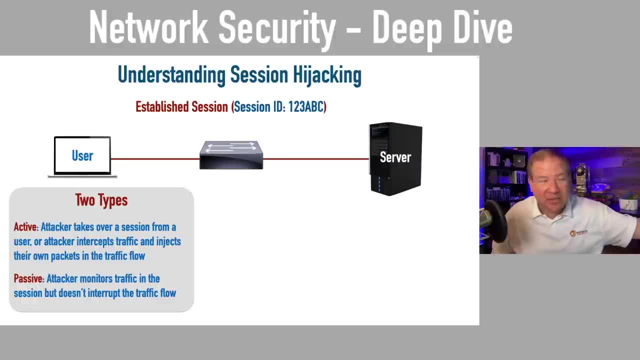 knows the session ID, they can join that session. They say: here's my session ID, let me in. And they get to be part of that session because they have, they've they've learned that session ID. So after the authentication happens, the attacker joins the network. they figure out the session ID. 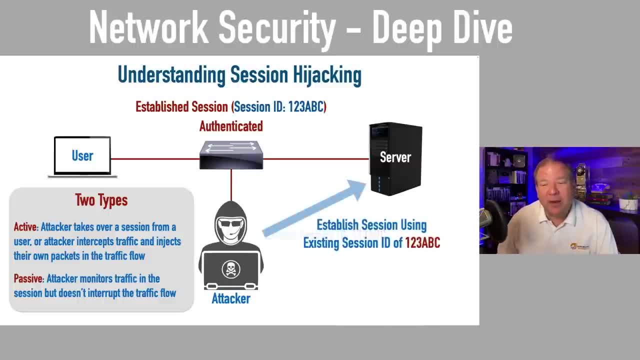 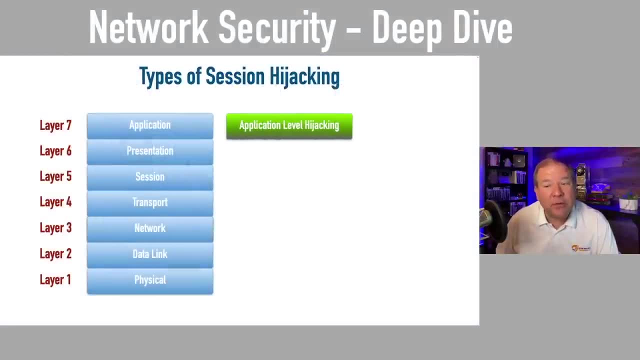 and we'll talk about ways of figuring out the session ID, And then they can be part of the session and they can establish a new session using that session ID. There is application level session hijacking And at the application level, this is often web attacks using HTTP or HTTPS, And this is. 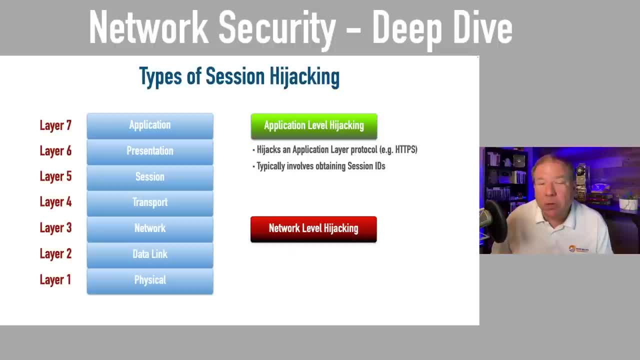 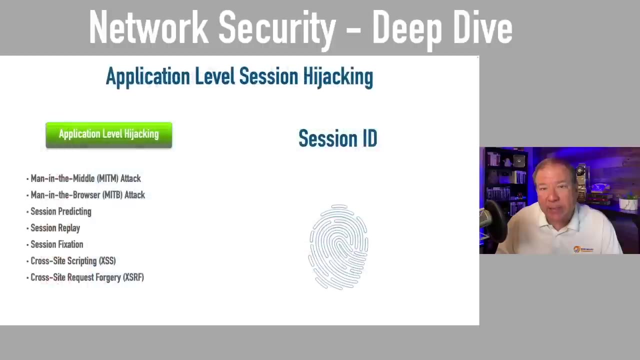 typically going to use those session IDs we talked about. There's also network level hijacking Here. we're more concerned with TCP and UDP things down at the at the transport and network levels, And this is usually going to involve intercepting packets, not just finding out a session ID. 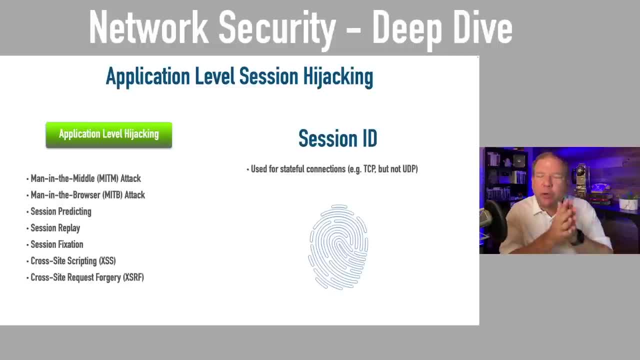 Now, when I say session ID, I'm talking about something that's going to uniquely identify a session. So it's going to be used for TCP, because that's a connection oriented protocol. It's not going to be used for UDP, which is connectionless, And it's usually going to be. 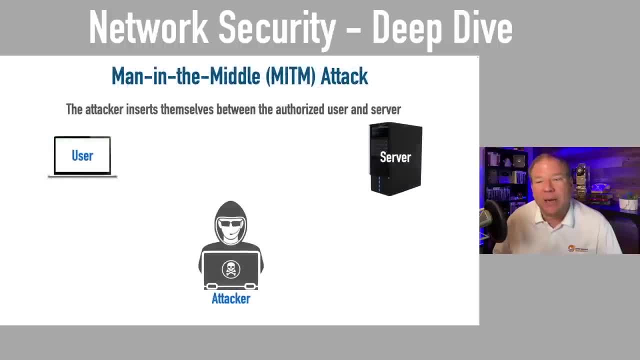 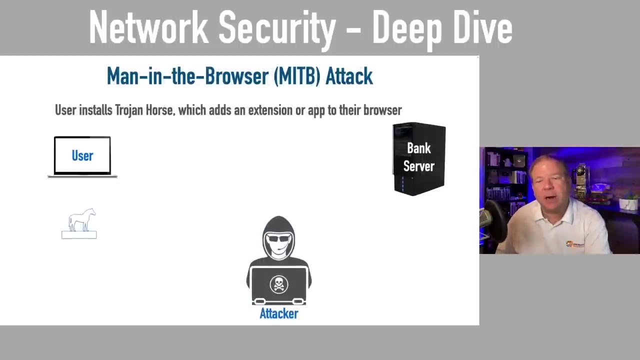 this big long string of seemingly random alphanumeric characters. So let's think about: how does the attacker get a session ID and inject themselves in that session So they can launch something like a man in the middle attack where the traffic starts flowing through the attacker? 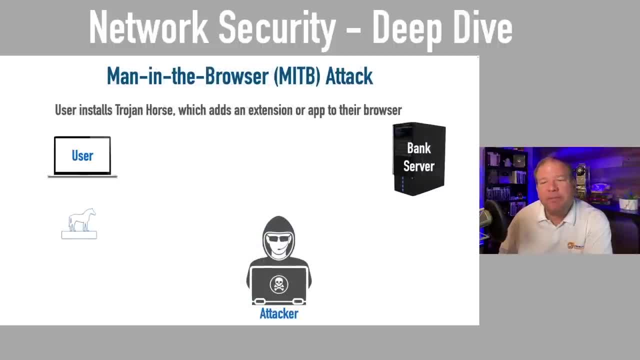 on the way from the user to the server. Well, one thing is they could use a man in the browser attack. A man in the browser attack is where there's some sort of a Trojan horse that's added to the browser software on the user's system And then when they try to, let's say, use that browser and 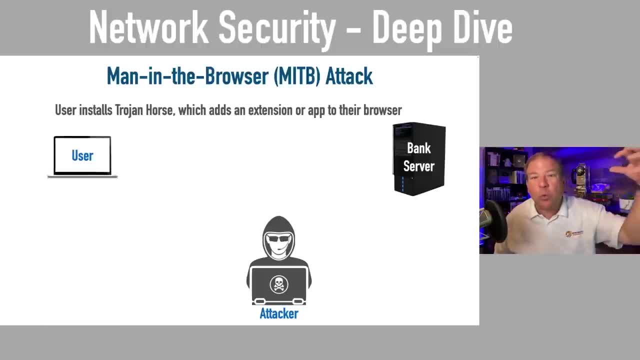 go to their bank. that Trojan horse software is going to redirect that down to the attacker. They go to that website and maybe they want to transfer a thousand dollars from their checking account to their savings account. But that Trojan horse in the browser software forces the traffic. 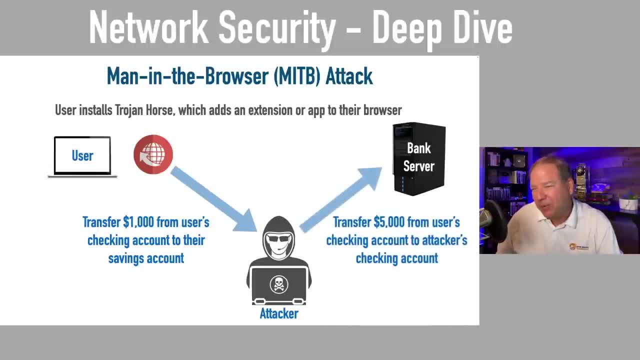 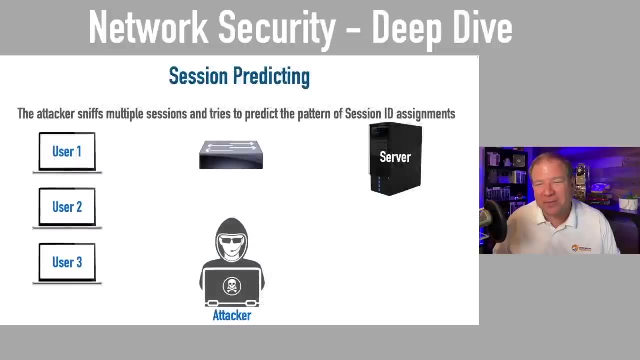 through the attacker's machine And the attacker says: let me change that up a little bit. Let's transfer $5,000. From your account to my account And then they can send the confirmation back to the user saying everything's good and dandy, When in reality they just lost $5,000. and it's been transferred to the. 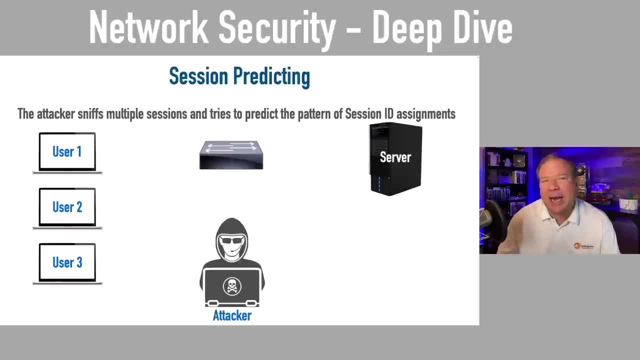 attacker. Sometimes session IDs are handed out in a somewhat predictable manner And an attacker might be able to guess what session ID that you're going to be using. If they sniff multiple sessions, they might be able to run some algorithms to determine or to estimate. 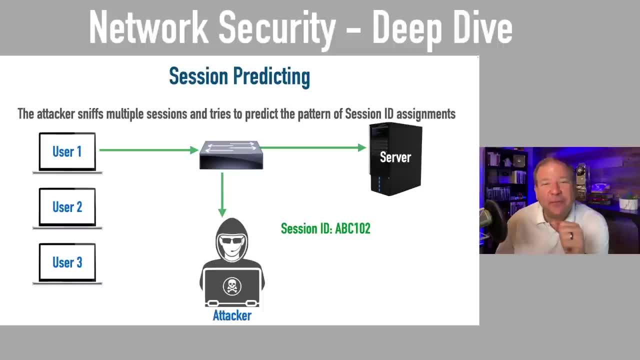 what you think the next one's going to be. Let's see how you do on this one. Let's say the first session ID is ABC102.. The next session ID is ABC104.. And the next session ID is ABC108.. Given that, 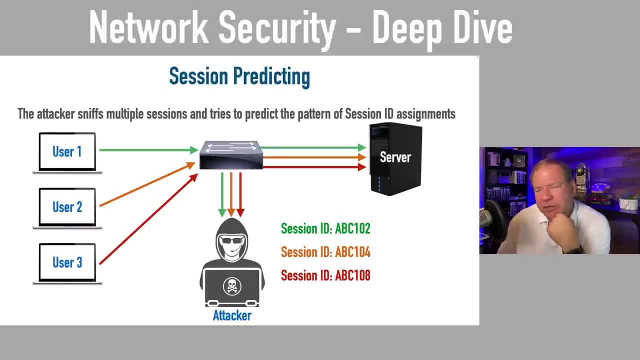 information. would you be able to guess the next session ID? Go ahead and chat it in. What do you think it might be? Obviously, I'm not being terribly secure here. This is just a simple example. Yeah, a lot of people saying ABC116.. I agree, Because you'll notice that rightmost number. 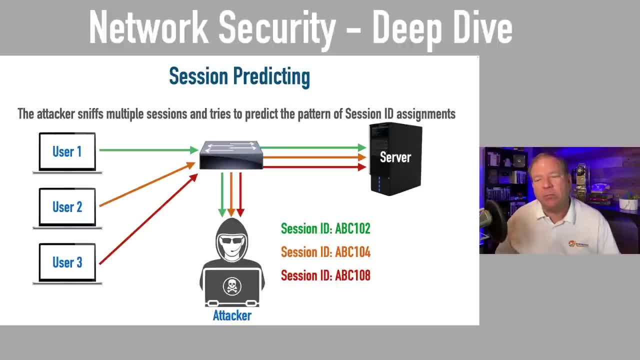 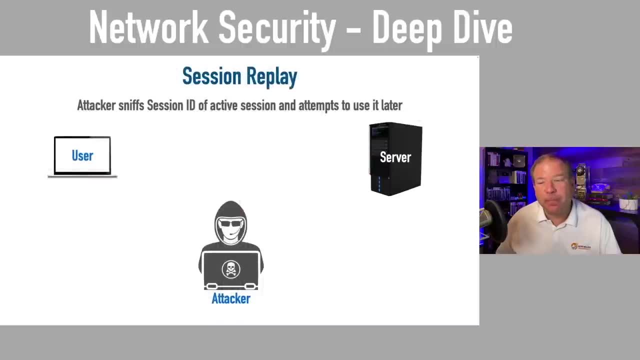 it's getting doubled each time. So two doubled is four, Four doubled is eight. Eight doubled- yeah, that's going to be 16.. That might be the next session key. The attacker might also sniff the packets in a session that gets established. that has all the right information in it. 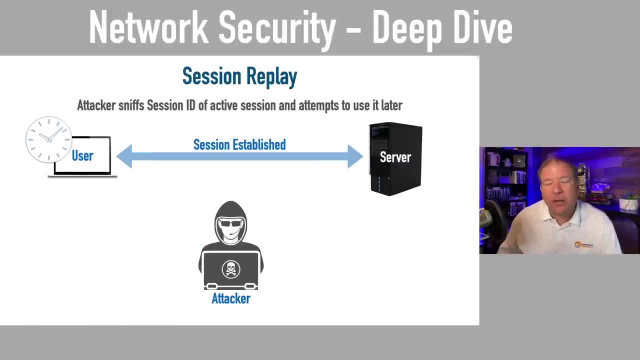 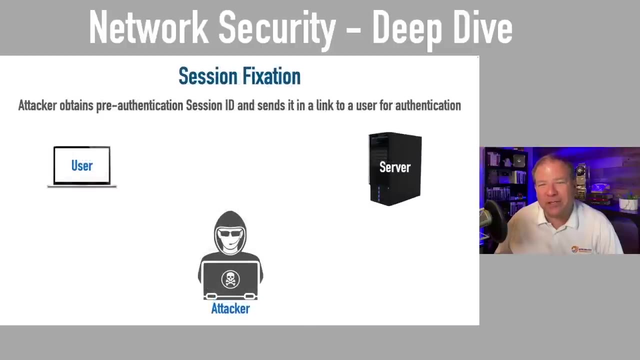 And then they come back later and use the session ID found in those capture packets. They're able to use that same session key as if the session were still going on. Assuming the user has walked away from their computer, we still got their session ID. The session is still active from the perspective of the server, The attacker. 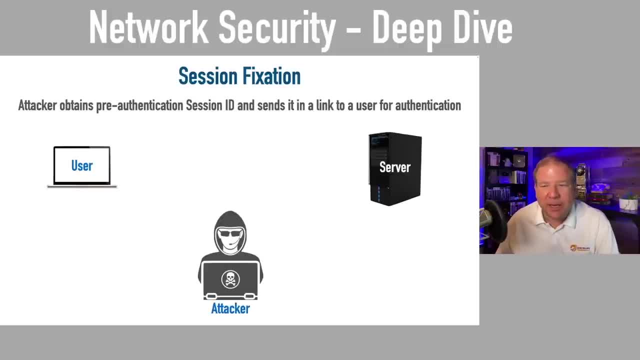 just kind of takes it over. Now, session fixation: Here the attacker is going to initiate the connection with the server. They say I'd like to set up a secure session And the server says, all right, here's the session ID that we're going to be using, but not so fast, You're still going to 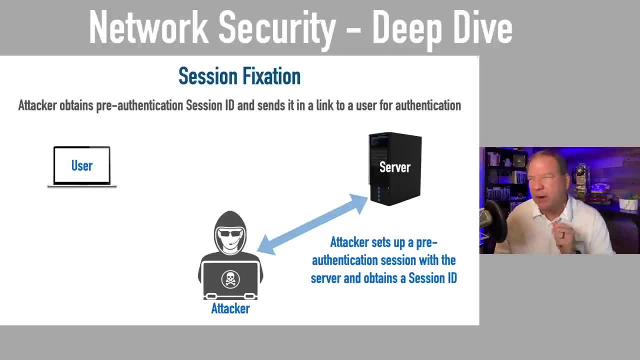 have to authenticate yourself. So the attacker says, okay, I'll get back with you, And the attacker takes the session ID that it just got from the server And then it's going to send a link- maybe in an email, maybe a text or something- to the user saying you need to reset your. 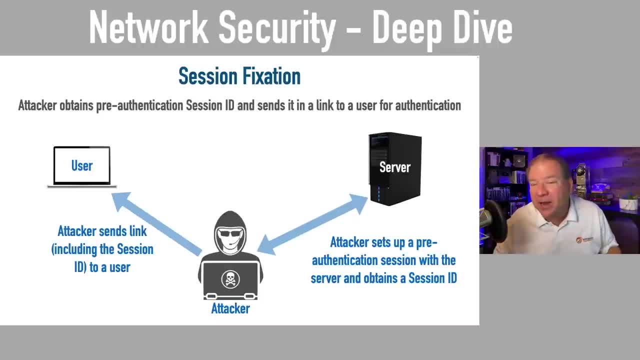 password, Go to this link, And that link connects the user with the server using the session ID provided by the attacker. So once the user authenticates with the server using that session ID- you guessed it- the attacker is now authenticated with the server. 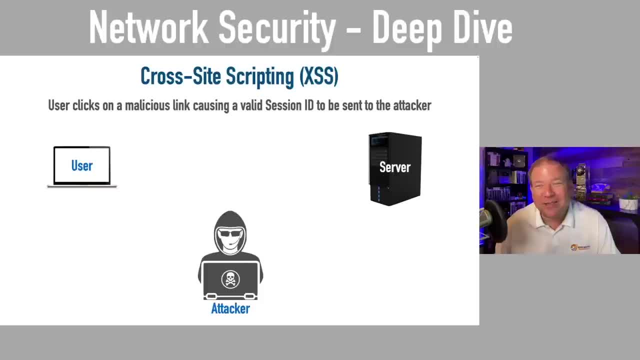 because they already. they had the session ID initially, So they get access to the server. Cross-site scripting you may have heard of This is where a user is going to have a link that they click on that maybe comes in an email And this is going to be a malicious link that causes a valid 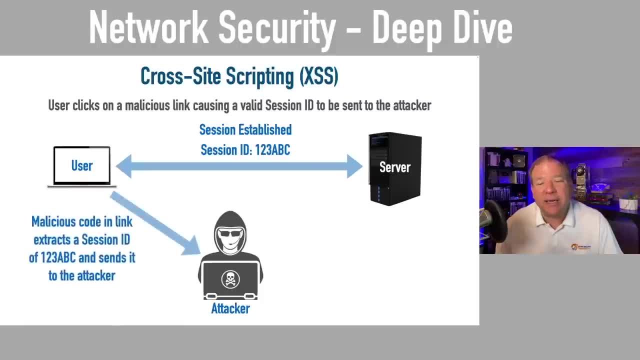 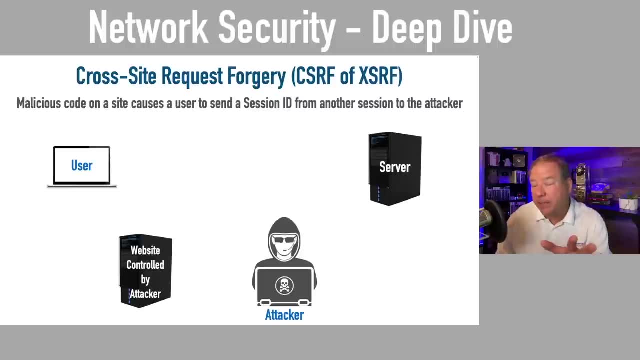 session ID that the user is using. It's going to send that session ID down to the attacker And the attacker again can use that session ID to talk to the server. That's similar to cross-site request forgery Here, instead of getting an email with some sort of malicious code in it, 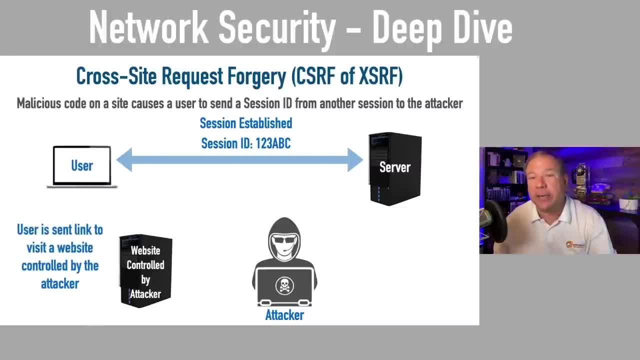 there's going to be some malicious code installed on a site that the user connects to And when they click on a link on the site, similar to the cross-site scripting, it's going to cause the user to send that session key to a website. 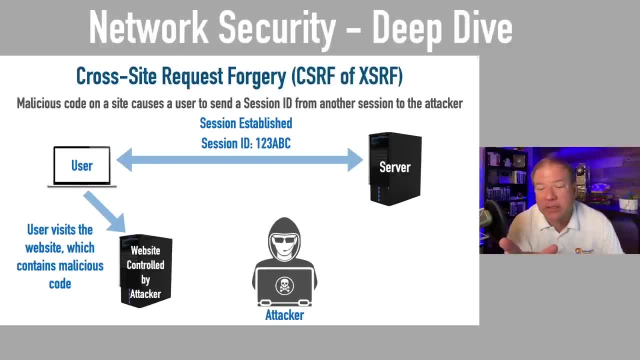 that's controlled by the attacker. Actually, I said that backwards, I got ahead of myself, Excuse me. We get the user to visit the attacker's website and the malicious code on that website- That's what extracts a session ID. I said that backwards, Pardon me, And that's going to be. 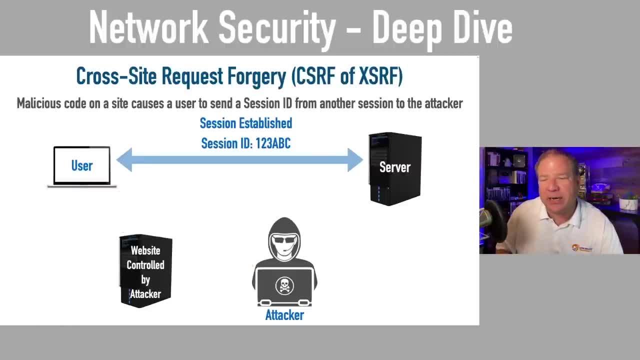 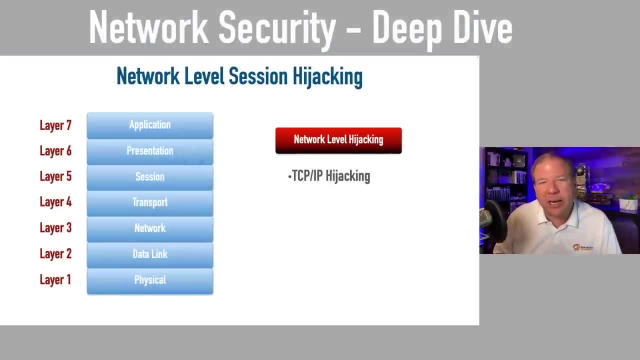 given to the attacker then, And then the attacker can use that session ID to communicate with the server. Next, let's consider network level hijacking. Network level hijacking is hijacking TCP and IP sessions. We can do a reset. We can be dealing with encrypted traffic. that we cannot. 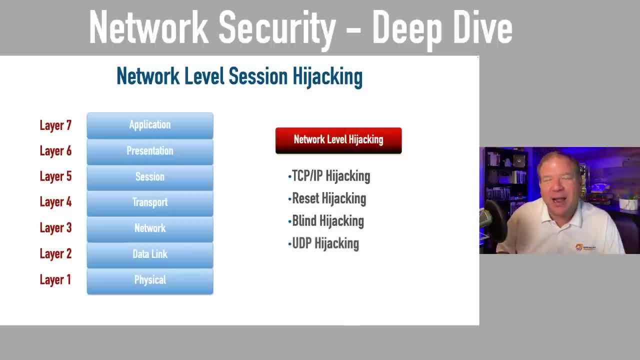 even interpret, but we can hijack it anyway. It's called blind hijacking And UDP hijacking is almost a misnomer because UDP is connectionless. We're not really setting up a session, but we can still do something called UDP hijacking And UDP hijacking is almost a misnomer because UDP is. 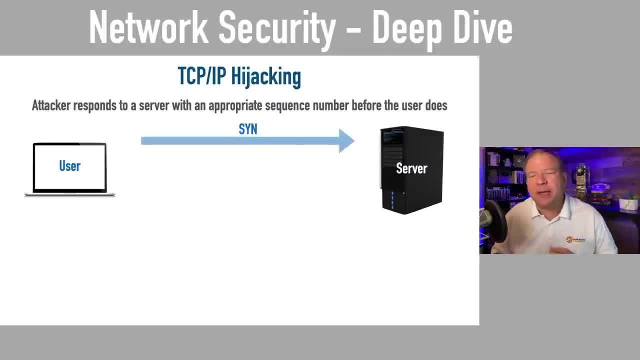 UDP hijacking- We'll talk about it in just a moment. But here with TCP hijacking, you remember the whole back and forth. the SYN, the SYNAC and the ACK is the three-way handshake. Well, in addition to that, there's an initial sequence number that's given an ISN and that's sent back. 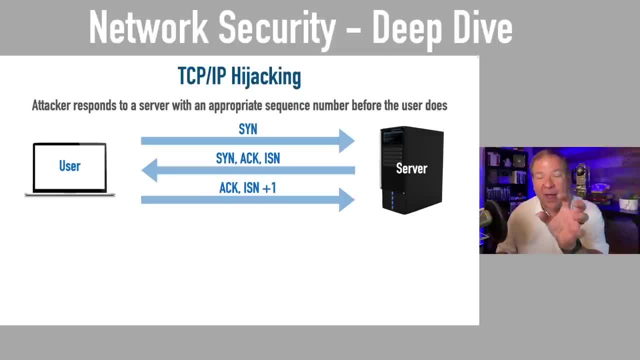 with the SYNAC And the user responds with that number plus one. Well, if the attacker is monitoring that traffic going back and forth, then the attacker is monitoring that traffic going back and forth When it gets that ISN sent from the server. if they're quick on their feet, the attacker is. 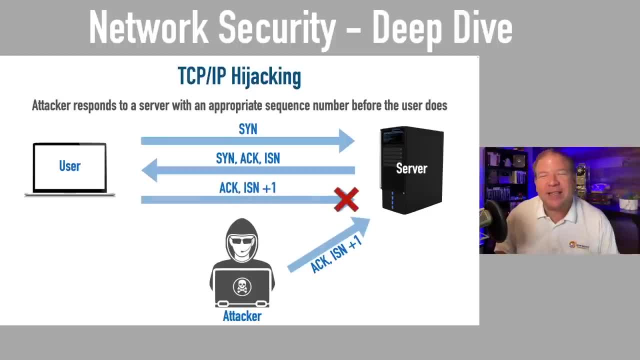 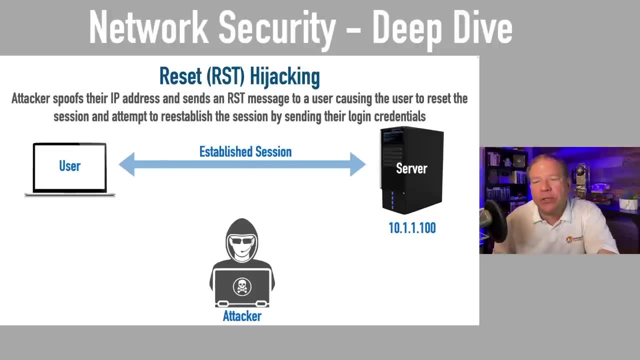 going to be able to respond to the server before the user does And they're going to get that session set up rather than the legitimate user. A reset is where the user is going to force the user to send a reset command telling the user they need to re-authenticate And when they 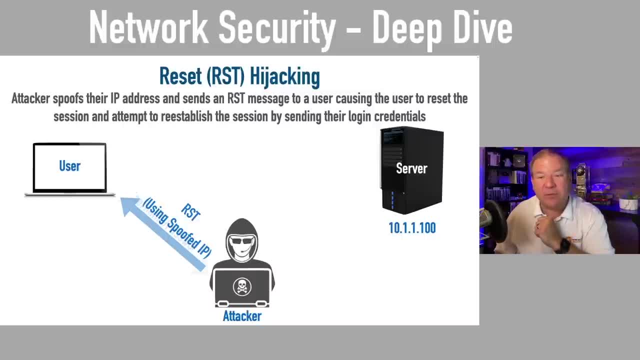 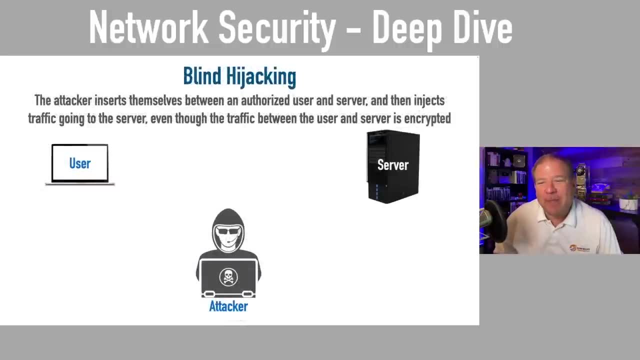 re-authenticate. the attacker is using the spoofed ID of the server. So the user is sending that username-password combination And when the attacker is sending that username-password combination to the attacker, which then uses it to get on the server, Blind hijacking is where we're able to. 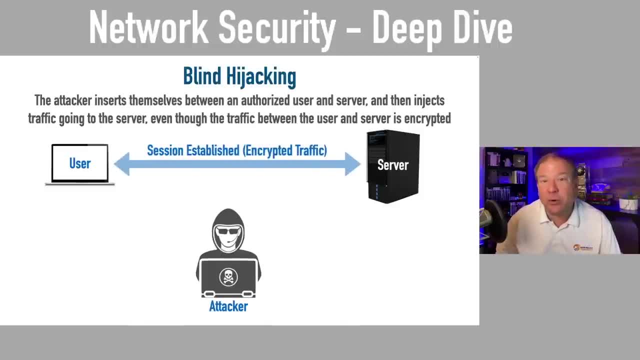 inject traffic going between a user and a server that's encrypted. It's called blind because it's encrypted. We cannot read it, but we can still mess with it. We can still, or the attacker can still, alter the data by injecting traffic going to the server. We also mentioned UDP hijacking. 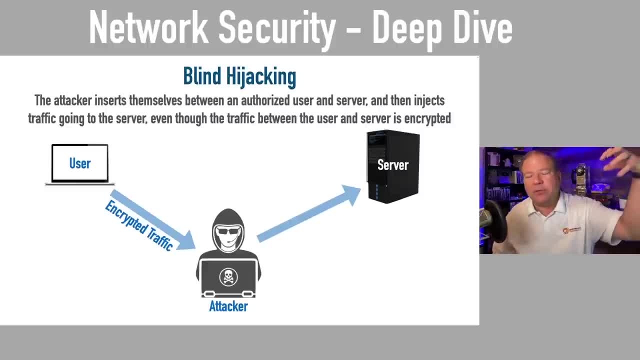 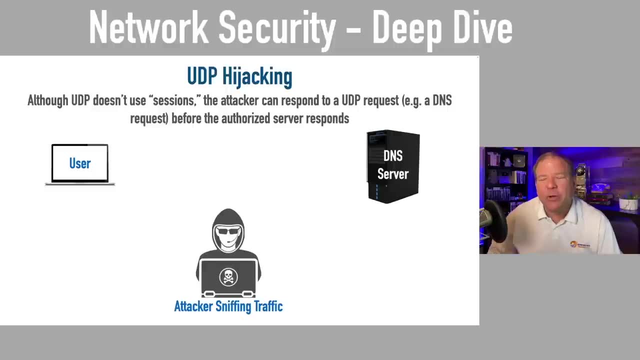 Oh yeah, I've got an animation here showing that the encrypted traffic could still flow through the attacker, Even though the attacker's not reading it. they could mess with it and they could add some additional traffic. Now, UDP hijacking- that term bothers me a little bit. We're not really. 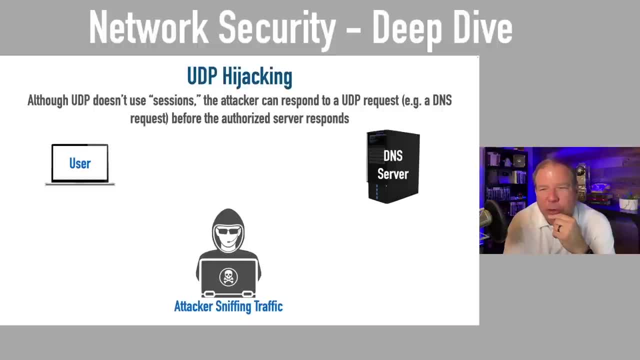 hijacking a session, because there is no such thing as a UDP session. However, we've got protocols that use UDP, like DNS. UDP hijacking means that we're going to respond to something using UDP faster than the legitimate user does. So let's say that the or faster than the server does. 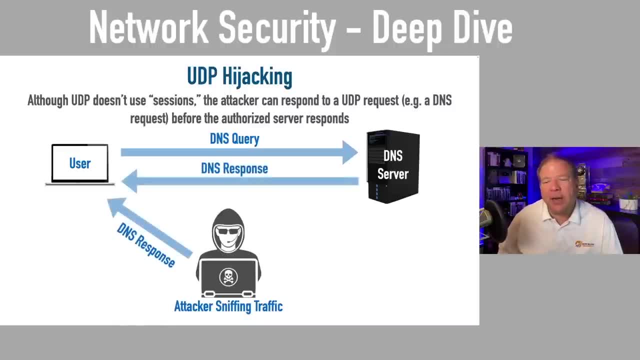 Let's say that the user does a DNS query and the attacker sees that query, looking up a certain website, and it responds with a false IP address for that fully qualified domain name. It responds with the DNS IP address faster than the DNS server does. That's a way that the attacker can redirect. 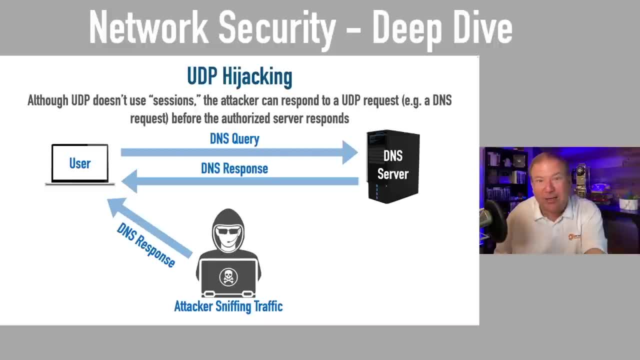 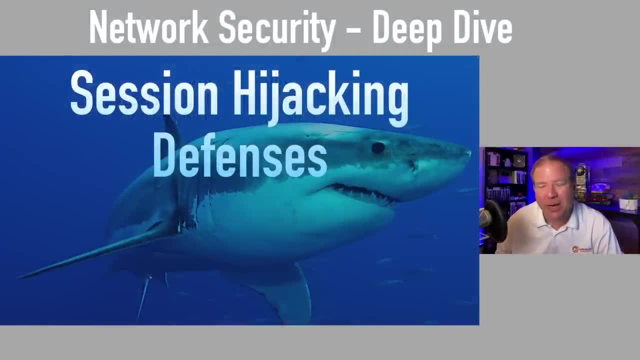 the user to their own malicious server that looks like the bank's server, but really we have one set up to copycat the bank's server. So that's a way that the user can redirect the user to their own. so we can capture username password combination. How do we protect against this? This sounds pretty. 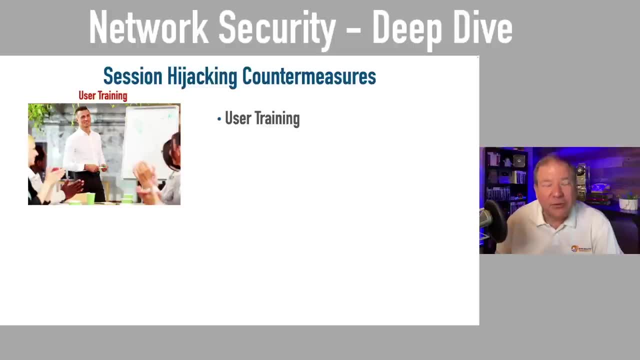 serious. Well, one big thing is user training. training your users. Do not click on anything in an email from unknown sources, And sometimes even from known sources. if it's your bank, don't click on the link in the email, open up a browser and go directly to your bank's website. 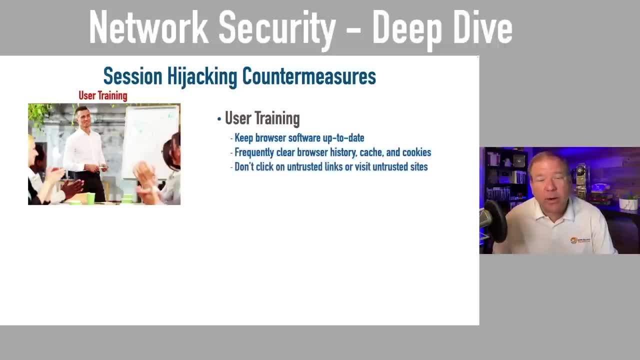 You want to keep your software up to date, all of your security software You want to clear out periodically and don't visit untrusted websites. Certainly don't click on links that come in texts or emails. We also might want to use secure session IDs, where an attacker cannot look at a bunch of 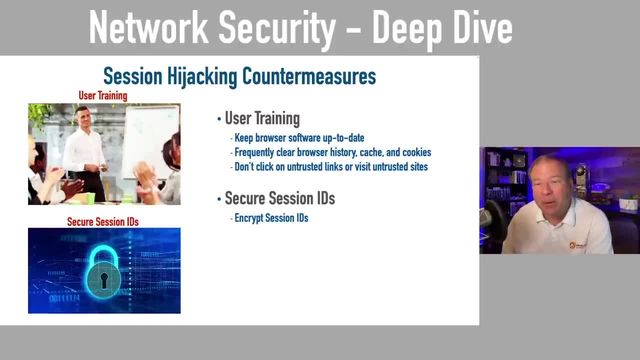 session IDs and then say, well, the next one's probably going to be this times two. No, let's use encrypted session IDs. Let's use session IDs that are not valid for the entire session, Depending on your system. sometimes you can use session keys that expire after a certain amount. 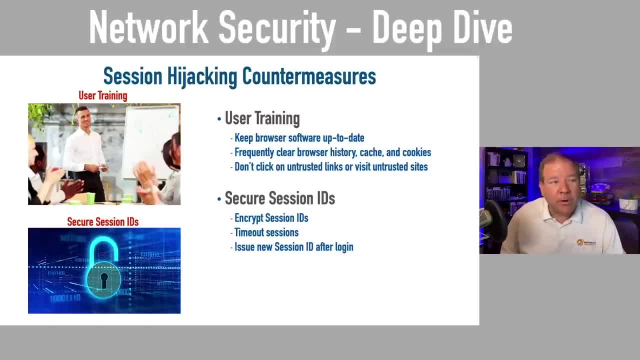 of time or you might have- uh, you might require periodic re-logins, like things time out. I go to my doctor's office, for example, and they log in, they check my records. We sit there and talk for a moment. They go to make an. 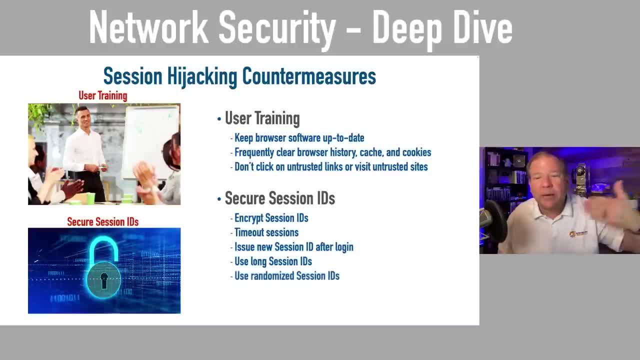 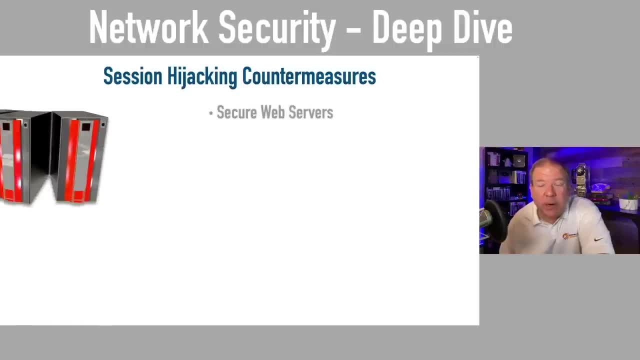 update on my records. They're logged out. Yeah, You might require repeated logins after a certain amount of time, And we want our session IDs to be randomized as much as possible, So they're going to be- they're going to be harder to predict. Other things we can do is to use secure web. 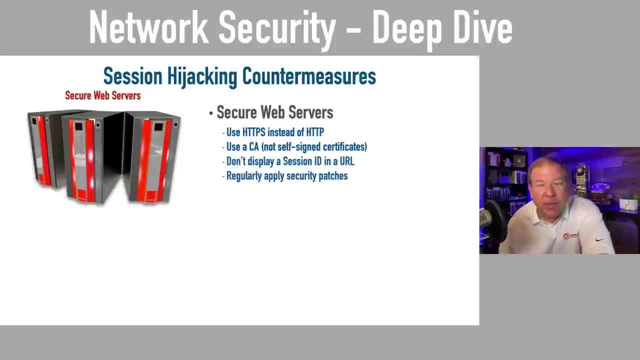 servers like HTTPS. instead of HTTP, It might be best to use a certificate of authority, a trusted authority, rather than a self-assigned certificate. Sometimes you'll look at a URL. you'll do a copy paste of a URL into notepad or something and you'll see this big long string And you'll think: 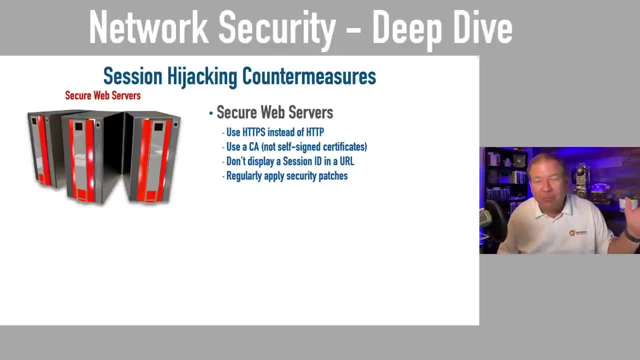 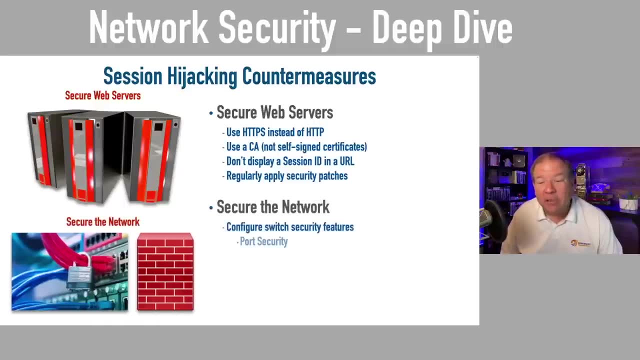 what is all this gibberish? It's a session ID. Let's not use session IDs that show up in the URL. That could be really bad. Let's keep our security patches up to date And let's just do basic network security, Like we talked about earlier. I showed you how to set all these up. 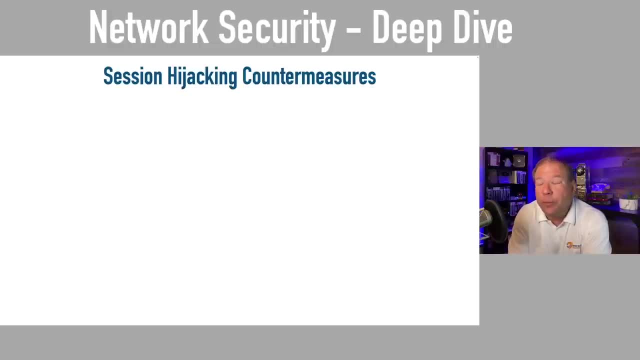 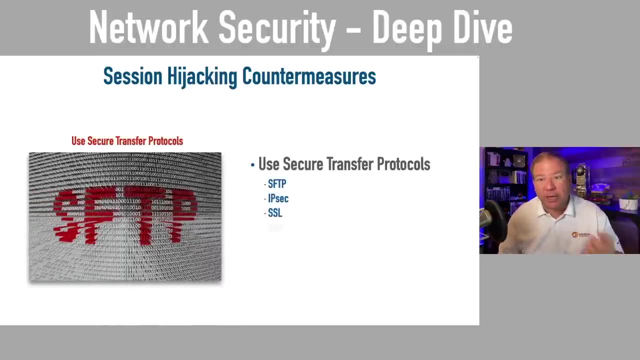 the port security, the DHCP, um snooping and, uh, the IP ARP inspection. What else can we do? Well, as already mentioned, let's use secure protocols like HTTP instead of HTTPS. Let's use a secure FTP or FTP. secure, Oh and uh. let's use um. let's do that instead of. 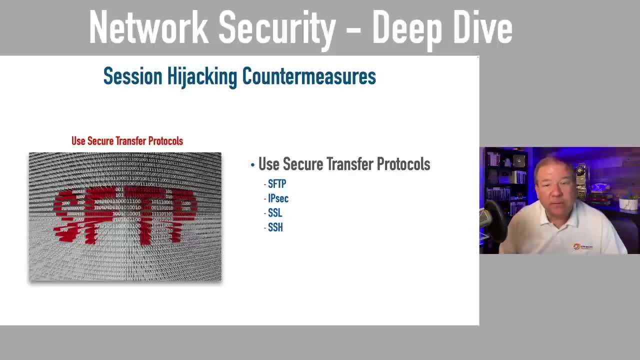 FTP. Let's use SSH instead of Telnet. Uh, let's use IPSec instead of GRE as a couple of examples. And we might want to use an IPSec VPN tunnel. So if I'm going across an untrusted network like the internet, if anybody 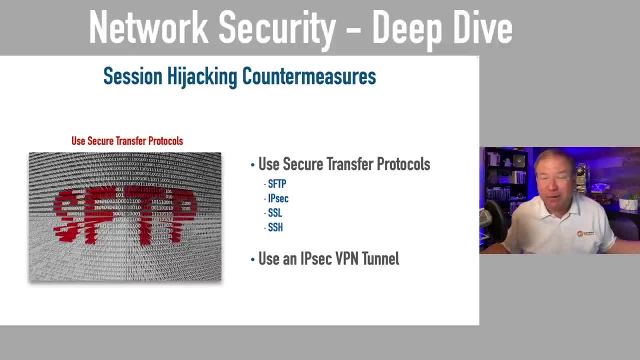 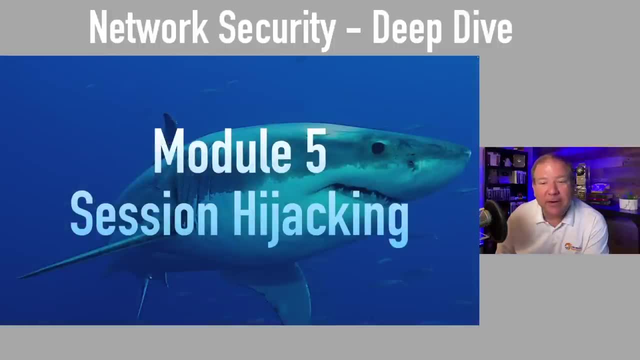 on the big untrusted internet captures my packets. they're not going to be able to do anything with them because it's all scrambled up thanks to IPSec, And we'll be talking about IPSec and VPNs at the very end of today's session, by the way, but that's a look at session hijacking. 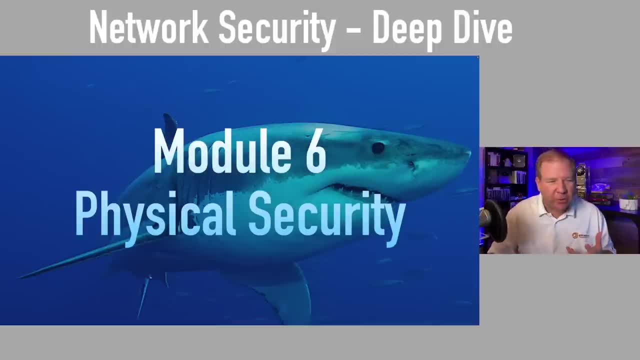 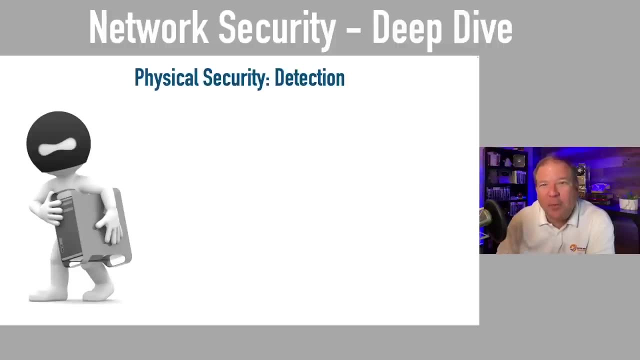 And now we're going to get into module six, And we hinted at this earlier. We're talking about physically securing our network gear so that somebody doesn't walk off with it or alter it or somehow compromise it or break into it. And one of the things we're concerned with is detecting. 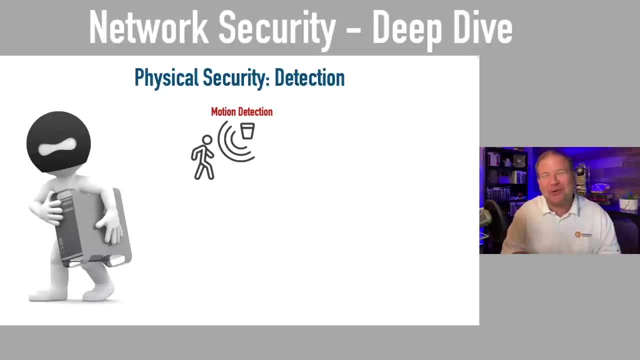 an intruder, Like the old video game intruder alert, intruder alert. And one thing we can do- pretty basic these days, we even have it in our homes a lot of times. we can have motion detection system sensors to detect any motion. We can have our passive RFID tags put on as inventory. 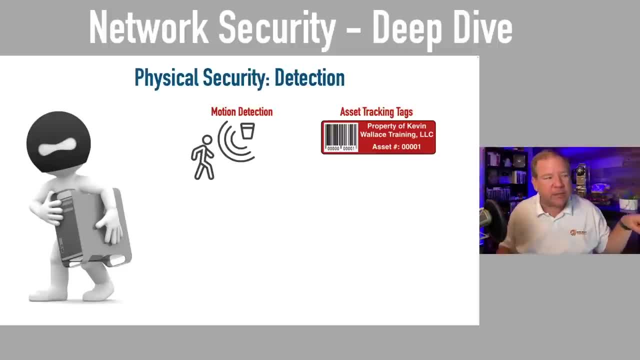 tags on our equipment and we can have portals around doorways. So if somebody carries a piece of equipment with one of these inventory tags on it, it sets off an alert or gives a notification. We can have video surveillance In the old movies where people are breaking into a casino or 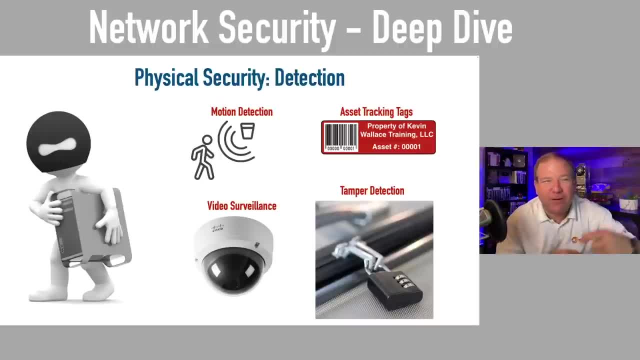 something or a bank. they might have a video that they loop and they play on replay. Not as easy to do that with IP cameras. So if we have IP-based video surveillance that's going to go a long way towards physically securing our equipment. We can also have something that's going to give. 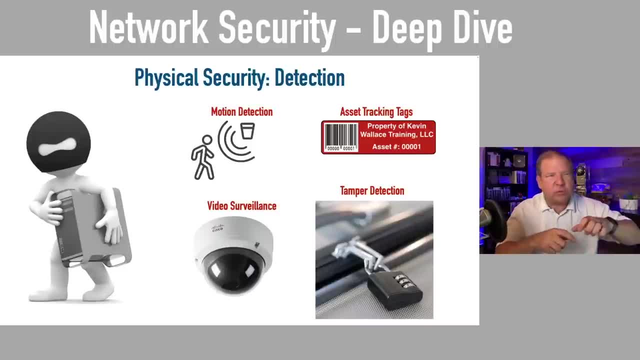 evidence of any tampering. You can get these sort of metallic stickers or even wire ties that you can close a computer chassis together with, maybe in a server farm or data center, And if somebody were to open it up, to try to insert something in it or take out a drive. 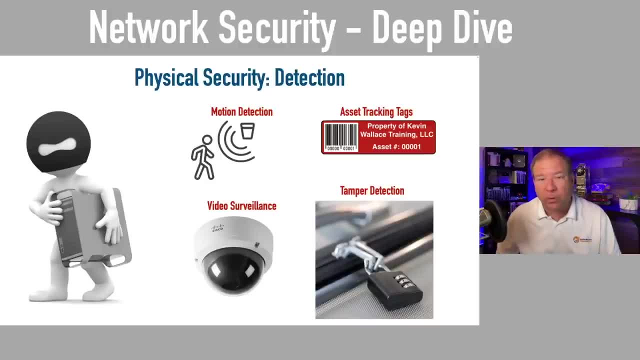 or something it's going to be evident. there's going to be evidence that they tampered with it, because that seal is going to be broken or it'll look stretched or it'll give some evidence of it, Or that maybe that wire tie is broken as an example. 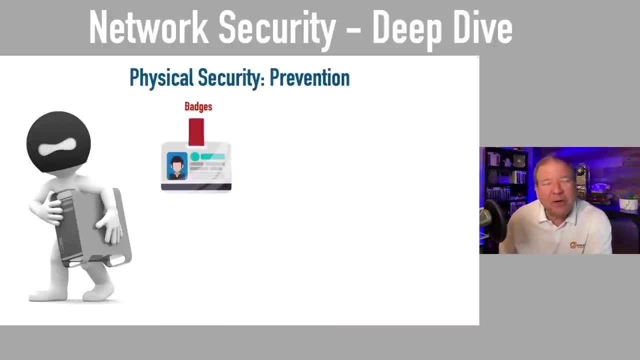 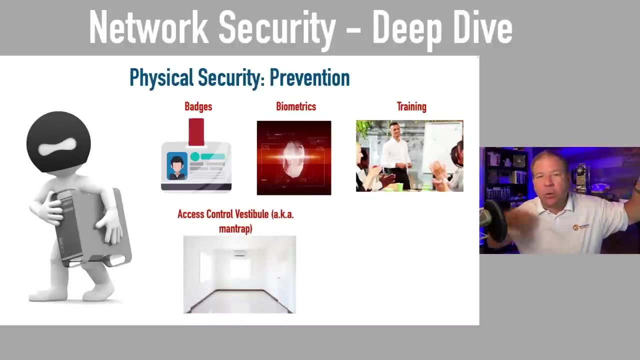 To prevent people from accessing these areas. I think it's a great idea to have people badge in to areas, areas maybe use something like a fingerprint scanner, a retinal scanner, and make sure your users are trained on what to watch out for if, maybe, in front of a data center you don't want. 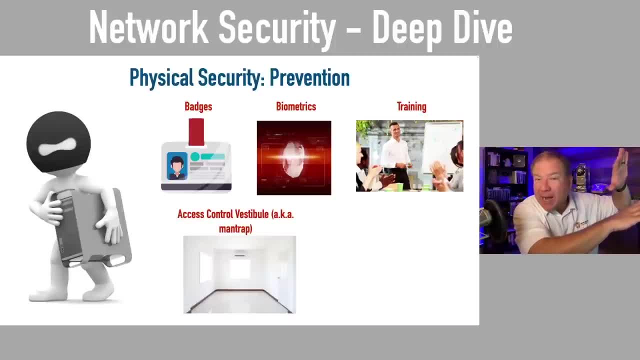 somebody to wander through and get into a data center by piggybacking on somebody else. remember before we said: i'm carrying this box, can you hold the door for me while i go through the door and somebody might let you in the door? well, there's something called an access control vestibule, or 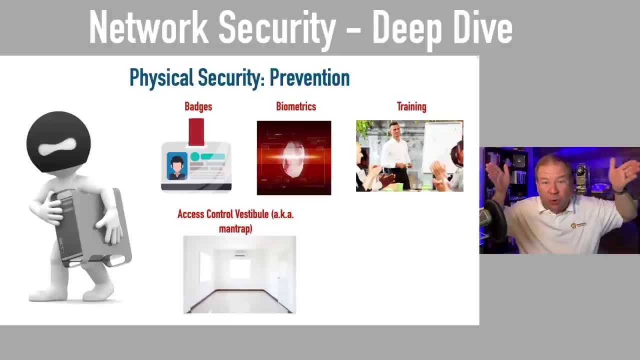 man trap, sometimes it's called. this is a room that has two doors and it's set up such that for one door to, if one door is open, the other door has to be closed. so there's no way for somebody just to sort of watch you go through into the data center and they just kind of follow right. 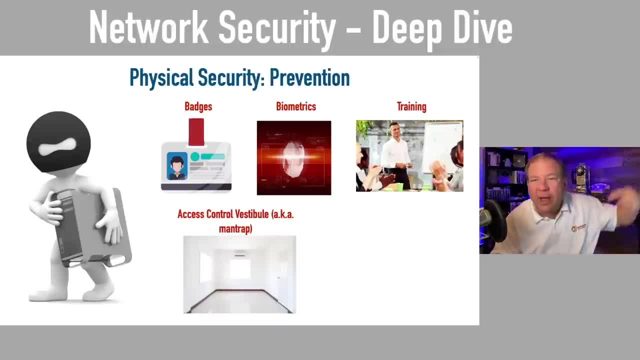 behind you because before you open that door going into the data center in the, you're in this vestibule- the attacker. if you're going into the data center, the door that the attacker would go through to get into the vestibule is closed. the only way for them to do it is to be in the vestibule with you at the same time. 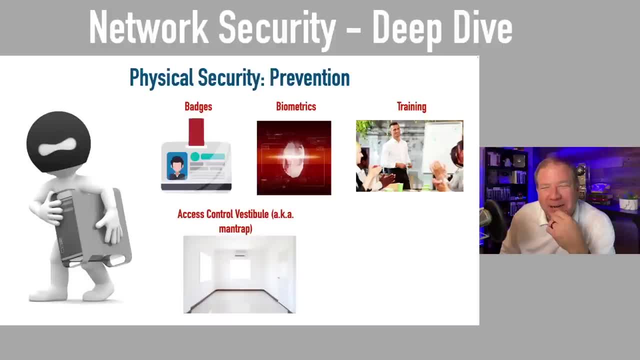 and they're gonna, and you're gonna like, who are you? so that's uh. and sometimes there's a security guard in there and you have to show credentials to them before you can just wander in to a data center and, at the very least, let's lock our stuff up. personal confession time. i'm a big, uh, i'm a. 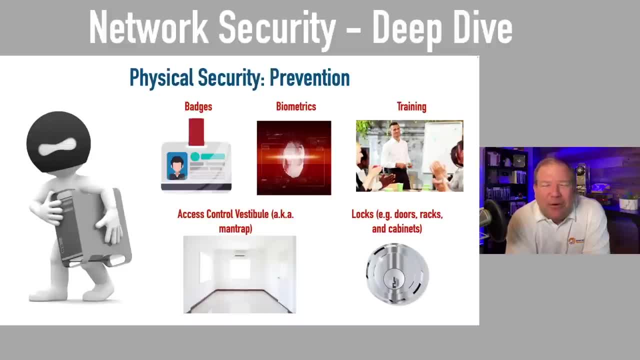 big fan of of physical security after an incident that i went through when i was working at a university. we used to, back in those days, we had a lot of atm equipment, asynchronous transfer mode equipment along with ethernet, and we had a bunch of extra gear like maybe like a hundred thousand dollars worth of extra atm gear, uh, in a server farm now. 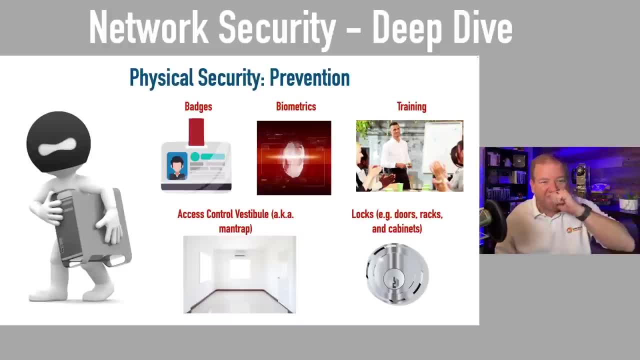 to get to the server farm you had to walk through this, uh, this computer training room that we had set up, and to get into that computer training room you had to go down a hallway and through a door, and there was another door to get into that hallway, so you had to go through one hallway. 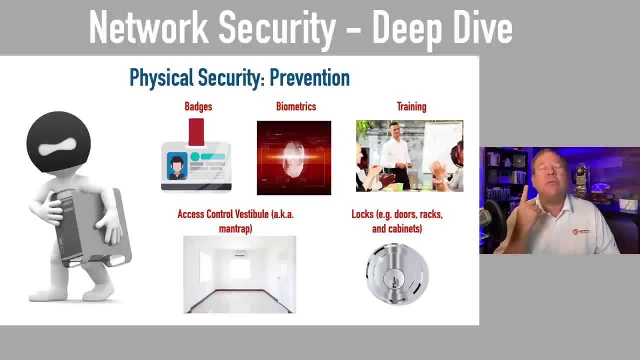 to get into the door another, another door, or have to go through another door to get into the door. one door to get to the hallway, then you go through a door to get to the training room, then you have to get through another door to get to the server farm. so i thought nobody's going to wander all the. 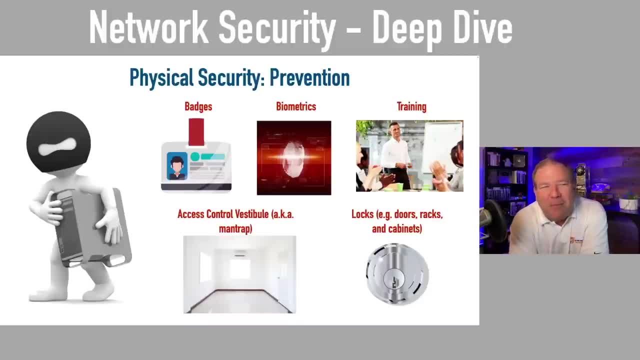 way back there. our stuff is secure in the server farm. no need to lock it up because who's going to go through three doors and wander around to get that somebody did because my- i mean my- fault. i'll take responsibility, because i was a network manager. i will. i did not have all the doors. 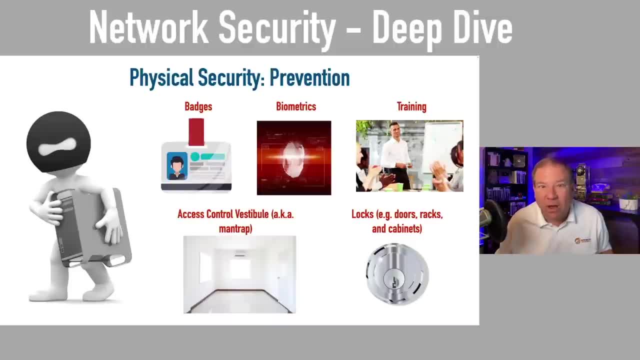 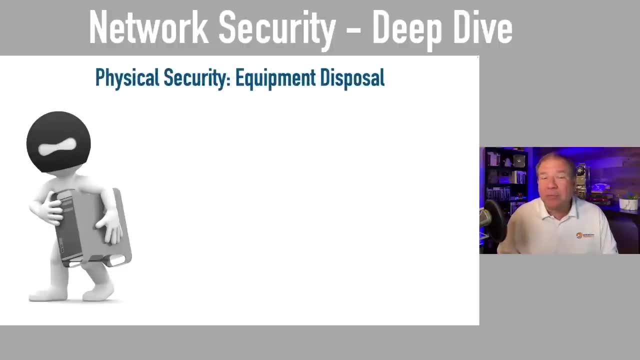 secured and somebody walked out with a lot of atm equipment and i had to go through a door to get equipment. so yikes, that one, that one's done. i don't want you to be in that position, and when it's time to get rid of equipment, you don't want to just say: all right, i did a format on my c drive. 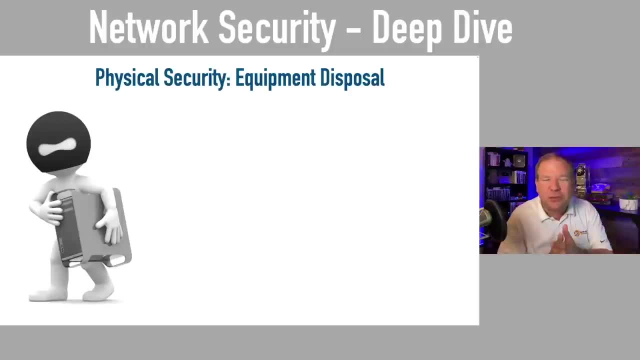 it's good to go and you give it somewhere. no, just because you like do a format on your c drive, that does not mean you've erased all the data. you've erased the- uh, you've erased the index, basically, of the files on that hard drive. so you want to wipe out any configuration that you have, if you. 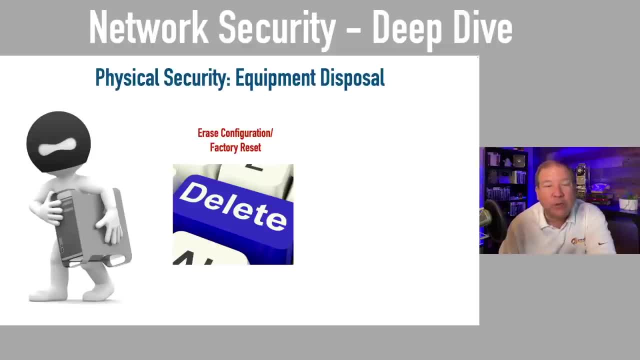 have a device where you can do a factory default reset, you should do that. you should sanitize the device. now, if i'm getting rid of a computer and nobody else is going to use it, i'm just disposing of it. i've done this so many times. i'll find a nice concrete floor and i'll find a big hammer and i'll put the hard drive on. 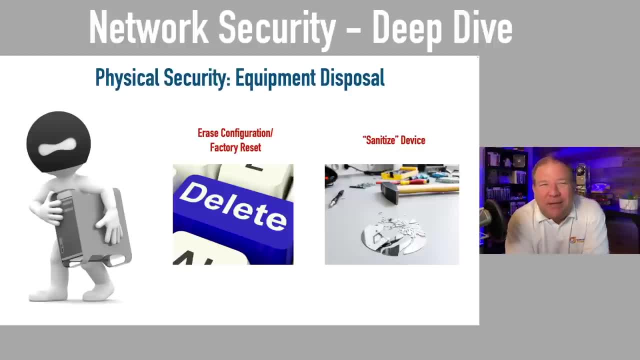 the floor and i will just. i'll just beat it until it rattles, and that's one way of making sure nobody's ever going to read that data. but let's say you are wanting to transfer a system to somebody else and you do want them to be able to use that hard drive. you don't want to take a hammer. 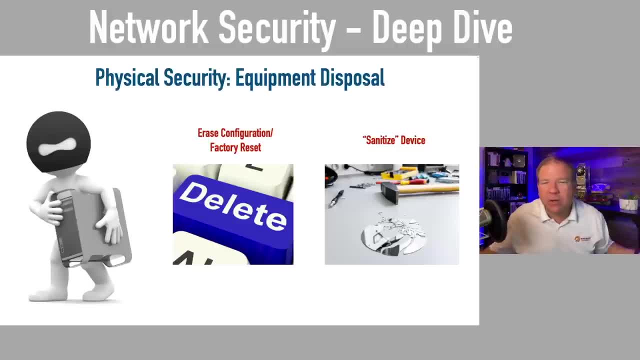 to it. what can you do? again, just formatting it? that's not what. that doesn't do it. i like to use something called dbn, it's called derrick's boot and nuke, and you can boot up on this, this usb key or a dvd or cd. you can boot up on this and it's going to not just erase your hard drive. you can. 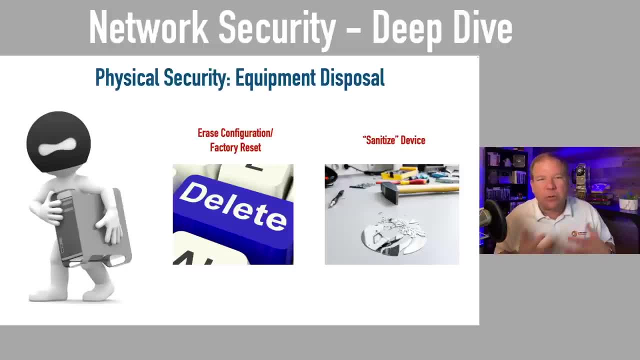 do several, several passes over that hard drive. and you can do several, several passes over that hard drive where it's just going to write some like random ones and zeros to it. so it's not just like formatting, where we're erasing the index of what's on there, no, it actually overwrites everything on. 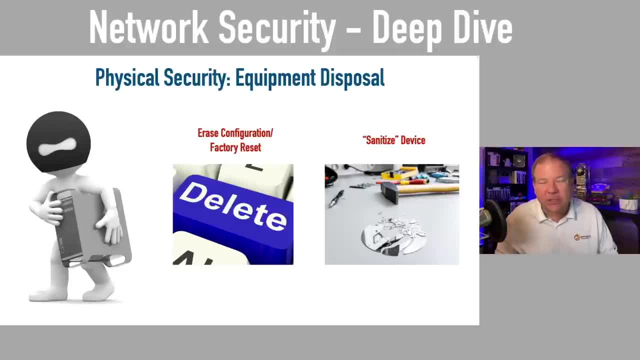 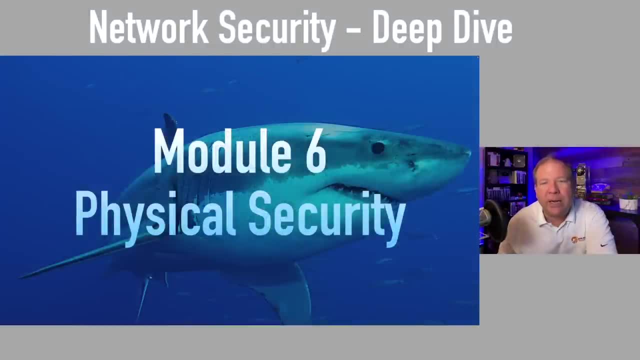 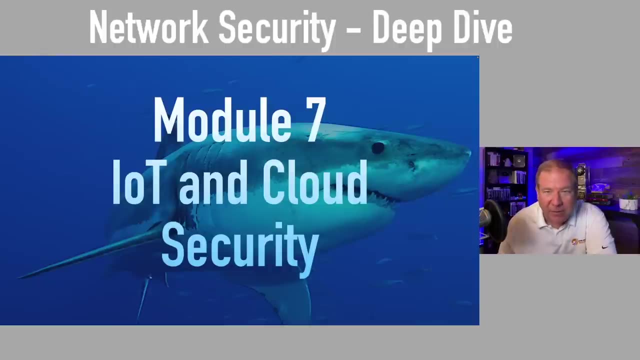 there and it can override it multiple times. and uh, yeah, that's, if i'm reusing a system, i'm going to transfer it to somebody else. i'll frequently use dbn derrick's boot and nuke. so that's a look at physical security. next up is the internet of things and cloud security- things that we didn't. 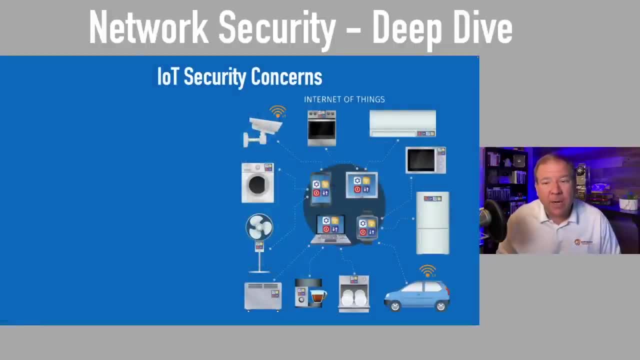 use 10 years ago as much, but we have to today. you see iot, internet of things devices. think about the ones that you have in your home. you might want to chat it in. what sort of iot devices do you have? i'll give you a sampling in my home. we've got doorbells. we've got video cameras. i've got a tv. 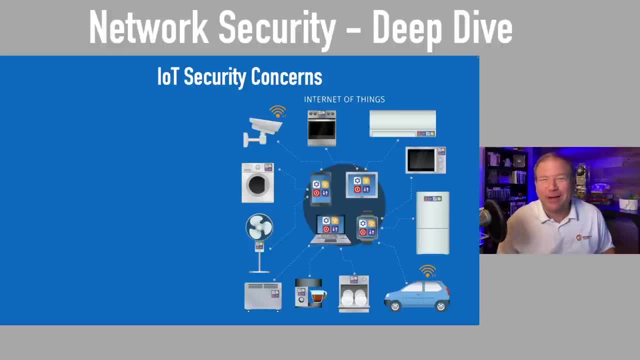 my refrigerator can tell me if, uh it, i finally turned it off. it was annoying. if somebody leaves the refrigerator door open too long, it would pop up a message on my phone and i'm my television, uh, the range, um, just all kinds of things. i've got a dyson fan. it just goes on and on. 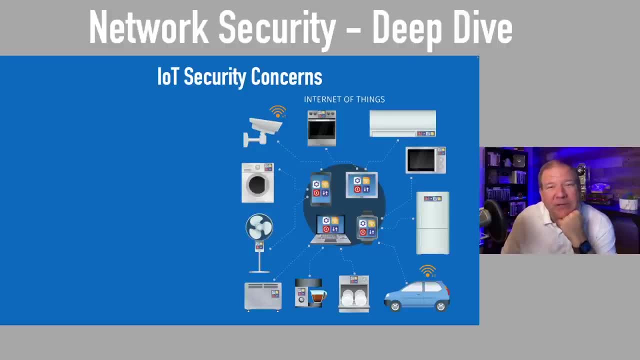 light bulbs that we have that are internet of things devices. it's super convenient. i love that we can set schedules on how the lights come on and i can see the. i can see all around the house if i'm away from the house. but you know what all those devices do? you know a lot about them have? 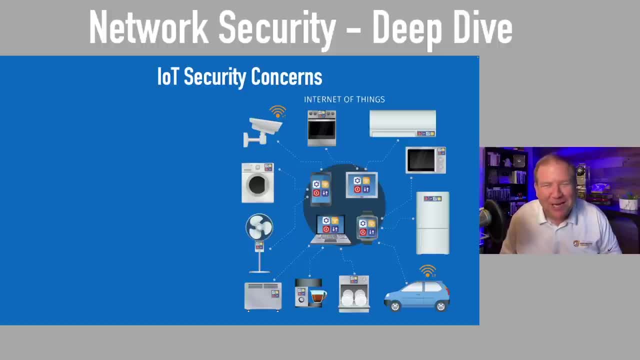 you ever done a firmware update on your iot light bulb, for example? there can be a lot of security holes when we introduce. we're poking holes when we introduce these iot devices because a lot of these devices, their security was not foremost on the designer's. 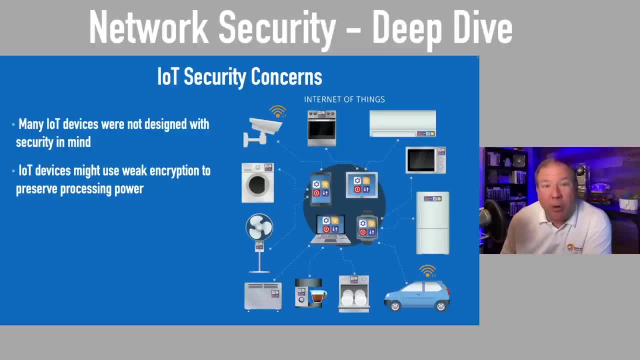 mind when they made those devices and we talked about processing power and versus encryption strength. yeah, a lot of those devices, if they are encrypting at all, they use a weak encryption algorithm, just so they don't don't have to put a more powerful processor in that device and drive. 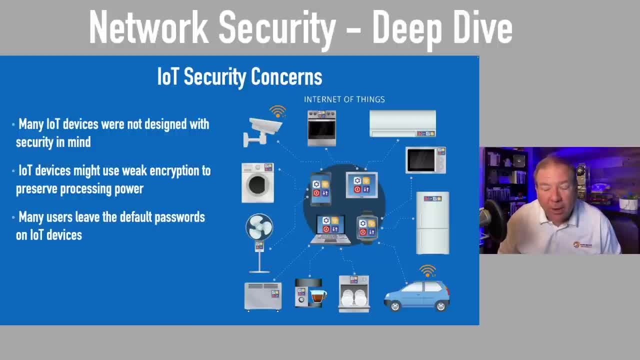 all stuff and a lot of those devices have default passwords, like your, your video cameras or your, even your wireless routers, and sometimes people don't do software updates. they might not be automatically deployed. and do you really think to go update your light bulbs? very often i don't. 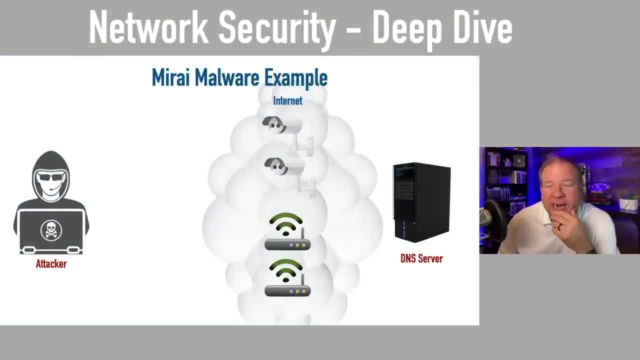 think of that. one of the most famous examples of somebody taking advantage of an iot uh. security vulnerability was a distributed denial of security, and that's what we're going to talk about today. security vulnerability was a distributed denial of security, and that's what we're going to talk about today. 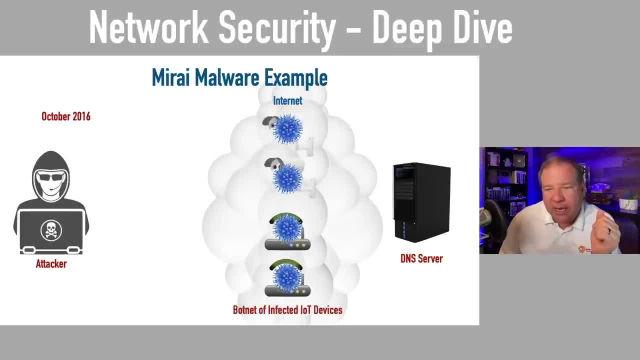 attack. this happened back in october of 2016, and remember where we talked about how an attacker could uh, using malware, infect a bunch of computers and they became bots or zombies. well, in this case, the attacker sort of scoured the internet looking for video- ip-based video cameras like home. 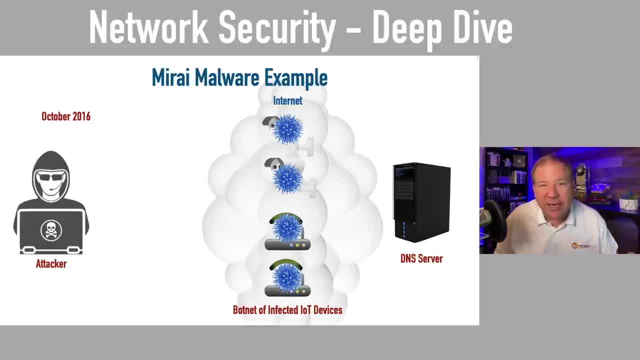 surveillance cameras and wireless routers that were set to their default credentials. so many people just unbox them. they're not going to be able to access them, they're not going to be able to plug them in. they left them at their default credentials, so the attacker just trying all these. 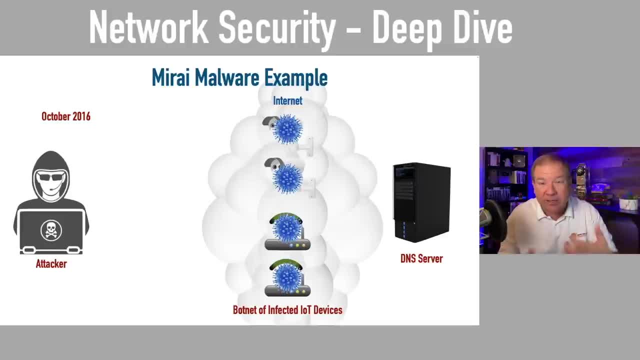 video cameras and all these wireless routers and, attempting to log in with default credentials, was able to log into a lot of them. so, at their at their beck and call. this attacker had all these cameras and all these wireless routers around the world and the attacker had them simultaneously attack. 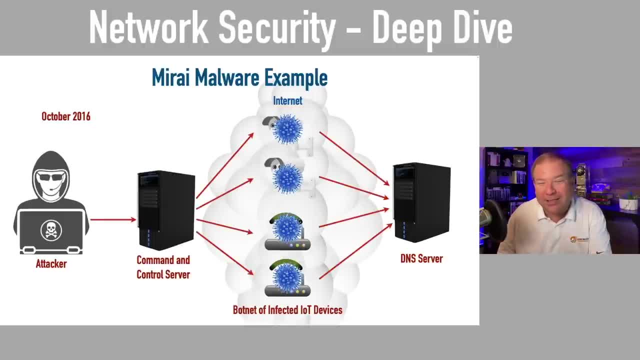 this dns server, which one one of the dns- uh one of the sites at that dns server was servicing was twitter. it actually brought twitter down for a large portion of the world in october of 2016 because somebody just logged into all these iot devices using default. 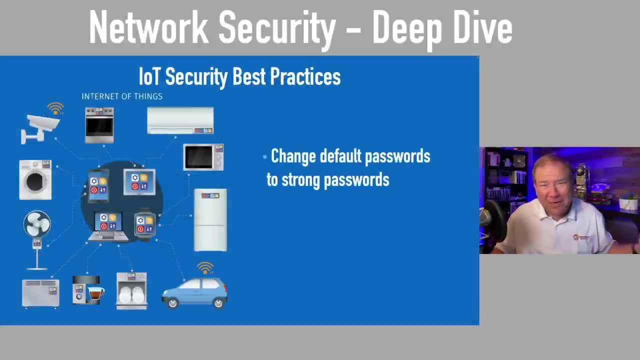 credentials. so what should we do? definitely don't leave things at their default passwords, and when you change the password, make it a strong password, and something that i recommend is putting your iot devices in their own vlan. so here's the thing: even if i have a firewall set up and the firewall is, 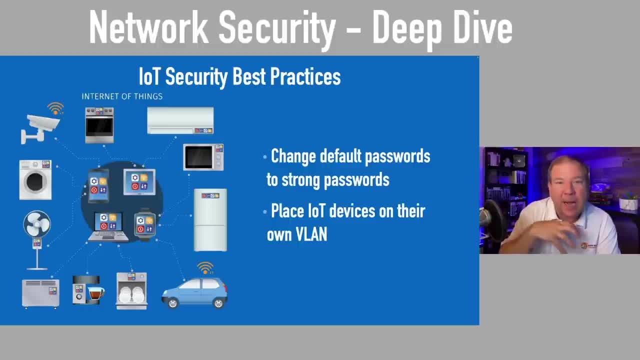 not going to allow any of the devices to be able to access the dns server. it's not going to allow any of the devices to be able to access the dns server- anyone on the internet to come into my network if the session initiates out on the internet. 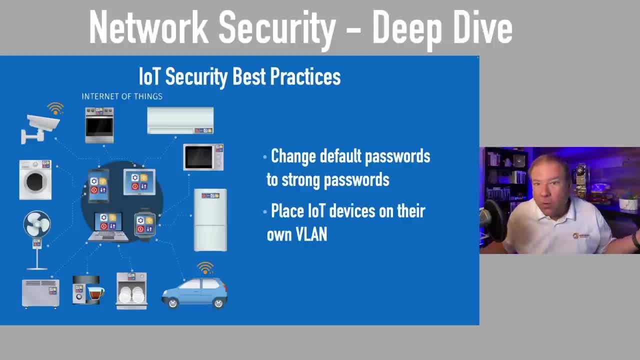 i've got all these iot devices. i don't know about these manufacturers. i didn't buy my light bulb from cisco, i bought it from some other, some vendor i've never heard of. who knows. could that vendor create malware inside of that bulb? or could somebody maliciously have have pre-injected? 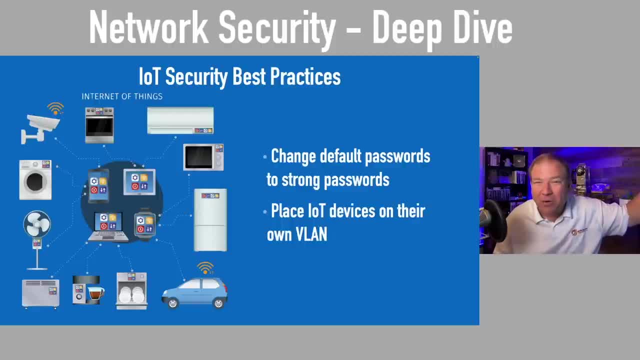 malware inside that light bulb that's now hanging outside my network and i don't know, garage, if they did, it's on the inside of my network and it could go out to the internet and start reporting information and start trying to scour the rest of my network. it's on the inside. 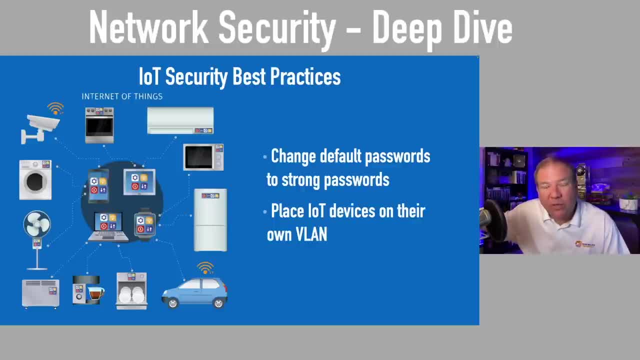 so it does have permission to have bi-directional communication with the internet. my light bulb could. i don't want my light bulb scanning around and trying to to get into my linux file systems. so what do we do? we put them on their own vlan. it's almost like having a guest wireless land, just for. 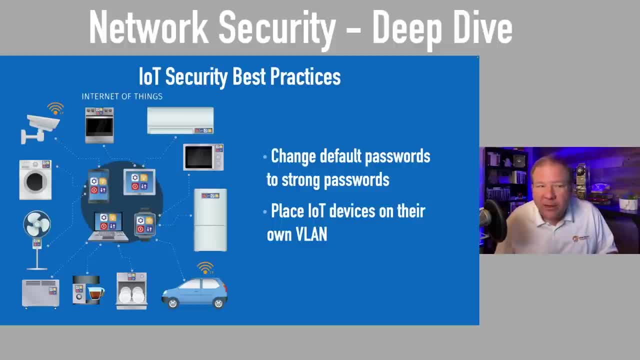 iot devices. this is something that i've never heard of, so i'm going to show you how to do that. i'll frequently do when i'm setting up wi-fi: let's put them on their own wi-fi network. don't not just a different name, actually a different subnet, so you can have. you can have this. 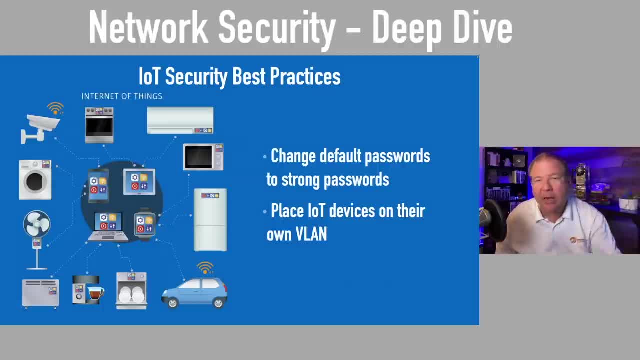 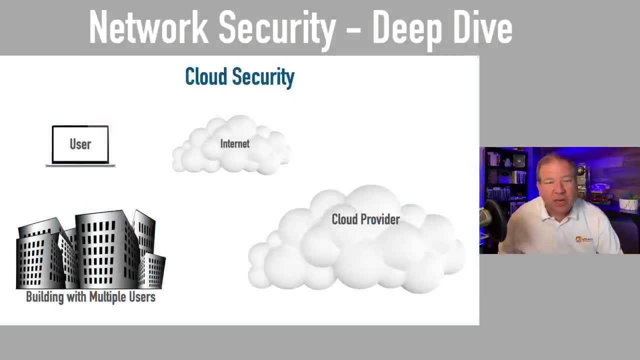 demarcation point between your iot devices and the rest of your network devices. cloud security: that's a big concern these days that i didn't used to think about because i- the networks that i grew up in- had server farms or data centers. data was stored locally. 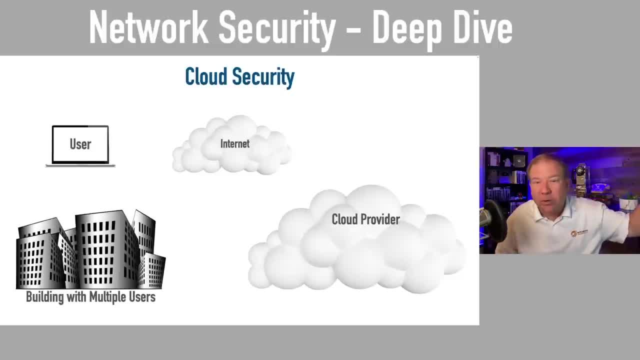 but over the past, really the past decade or so, there's the been this mass exodus of data going from our on-site data centers out to the cloud. after all, we move our data to servers in the cloud. those can be virtual machines. we can spin up servers as we need them. we don't have to buy. 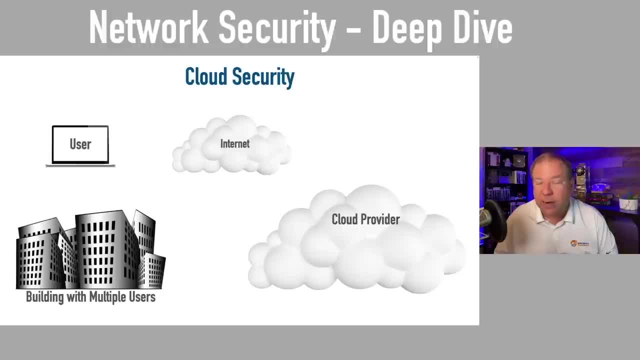 the hardware. we don't have to maintain the hardware. we don't have to provide redundant power to the hardware. we just pay for the, the power or the processing power and the storage resources that we need at any given moment, and we don't have to buy the hardware. we don't have to. 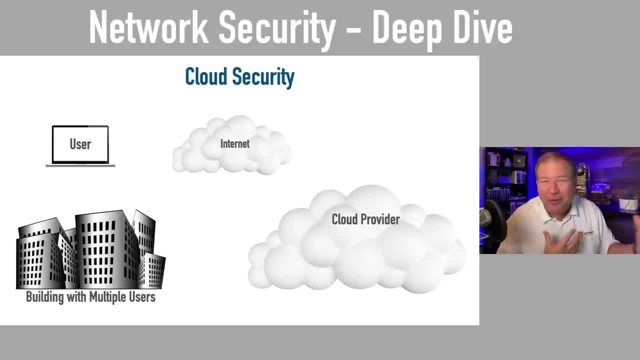 it's. it's great, except we've got all of our data flowing back and forth between our site and the cloud and we want to make sure that that data is secure. if i'm going over the internet, maybe using a web browser, we want to do that securely, and one way to do that, with one security feature that we 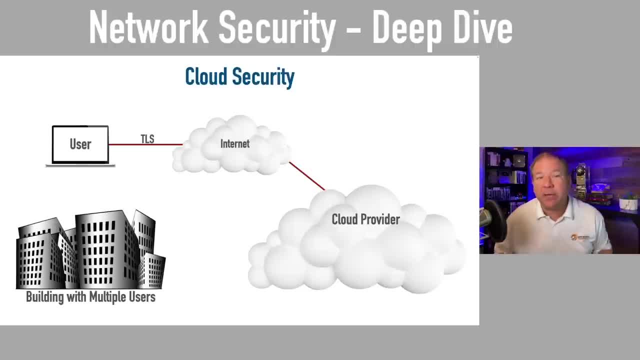 can have in our web browser is tls- transport layer security that's going to encrypt the data being sent between our browser and whoever our cloud provider is. maybe- and we'll be talking about vpns here in just a moment- maybe we want to set up a virtual private network between our site and our cloud provider, so, as we 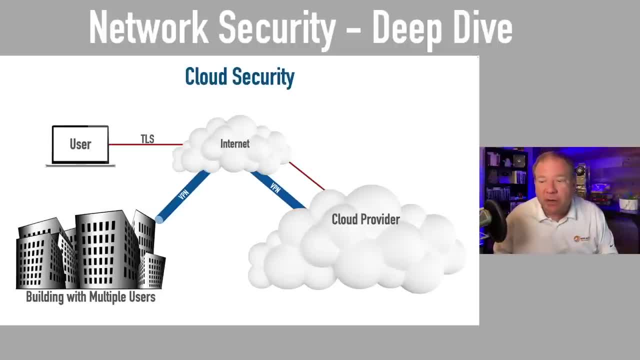 go through the internet. if anybody were to intercept our traffic, they wouldn't be able to make any sense of it because it's all scrambled up inside of that vpn. maybe we've got a private win cloud where we're using something like metro ethernet or maybe mpls, but we've got this private. 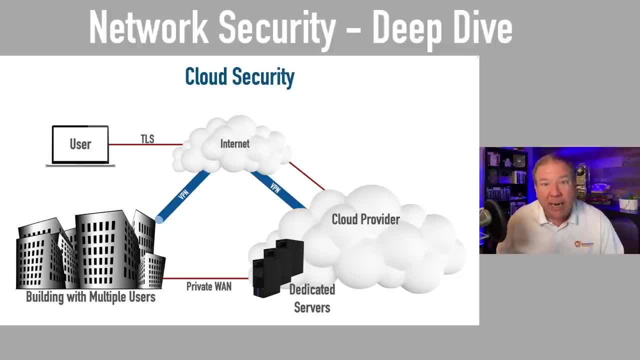 connection that does not use the internet, and maybe we've got some dedicated servers in the cloud where we're not sharing resources on a physical. we don't have a vm on the internet. we don't have a vm on the internet. we don't have a vm on the internet. 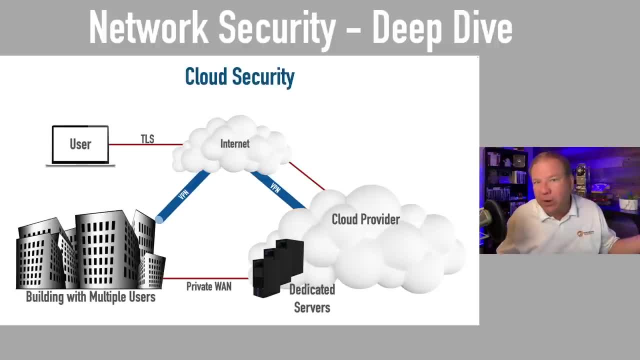 the same physical server that somebody else has their vm on. i mean, theoretically they're going to be isolated, but we might want to have some just for extra security, some dedicated servers, physical servers that nobody else is using. something else we can do is use a feature or a this function we 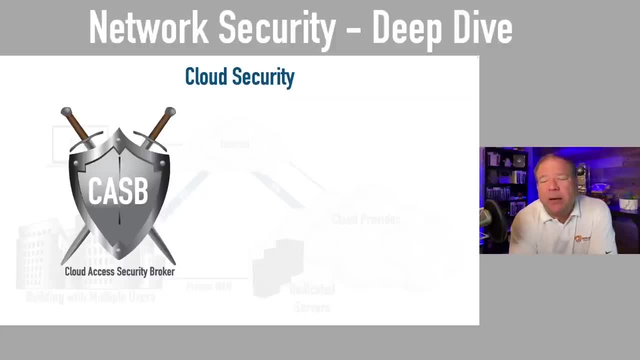 can get from different providers called casby. casby stands for cloud access, a security broker. it's sort of going to be the agent that stands in the middle between the users at the corporate site and the resources in the cloud, and it can monitor traffic going back and forth between the enterprise and the cloud provider to make sure. 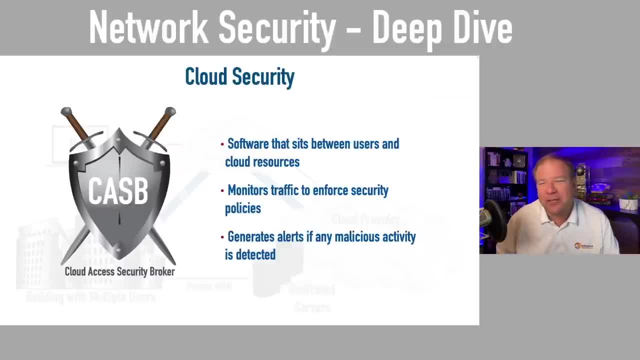 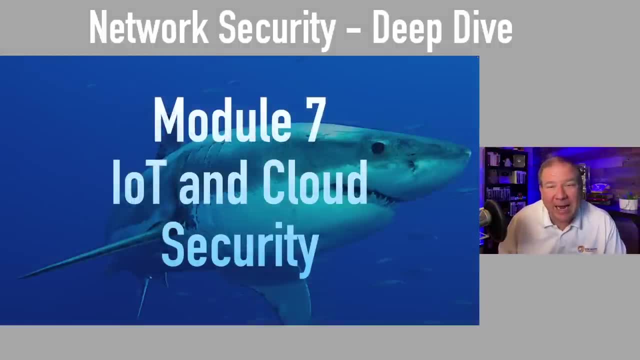 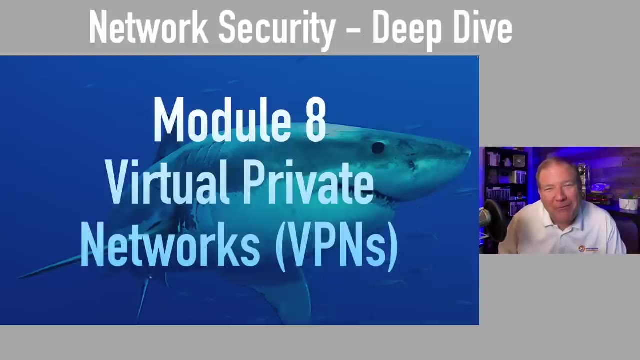 everything looks good, nobody's doing anything uh fishy, and if there is malicious activity, it can report that to us. so that's a look at better securing the internet and our the internet of things devices we have and our cloud. and in our final module- that's right- we finally reached the 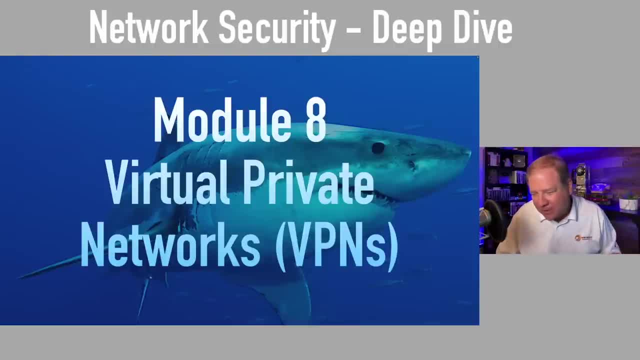 final module. let's see. i was estimating we'd go about five hours today. i'm just doing a projection here. we're going to be maybe just a hair over four hours. it looks like between four and five hours. looks like where we're going to land today. but let's take a look at our final module at vpn's. 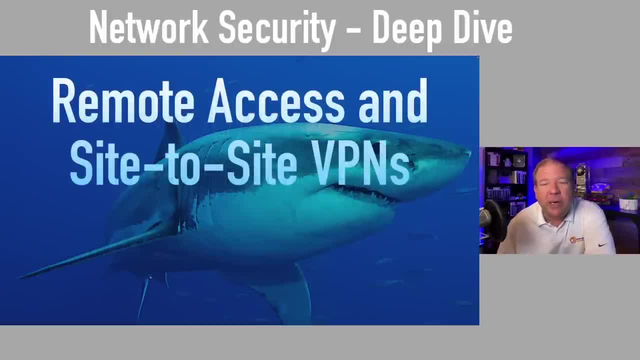 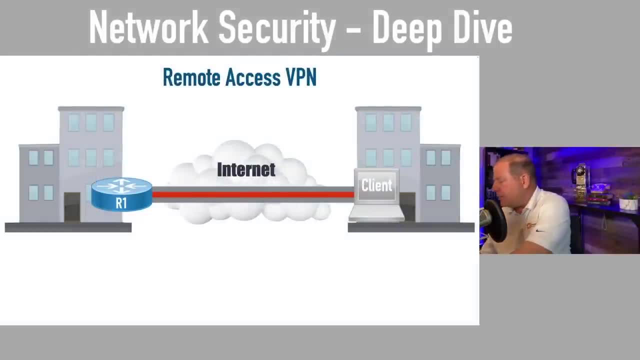 virtual private networks. first, let's distinguish between remote access and site-to-site vpns. a remote access vpn is where we've got. let's see. here's my laptop. i've got my laptop. this is one of the the new macbook airs and this color. they say it has bad fingerprint problems. i don't know if you. 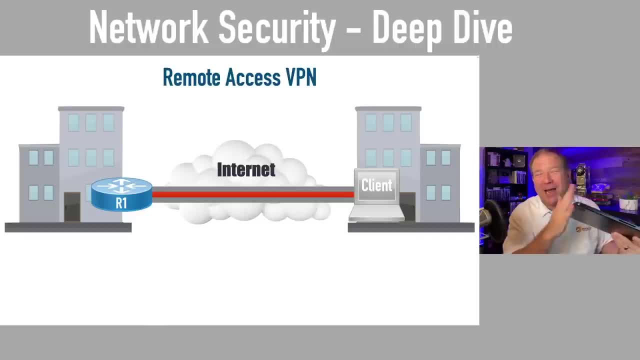 can see it, but, uh, they're not going to be able to see it, but they're going to be able to see it. but i love my laptop and if i'm on the road and i want to communicate securely back with another system, i've got vpn software on here i can set up a vpn. uh, the um, the appliance in my home has a vpn. 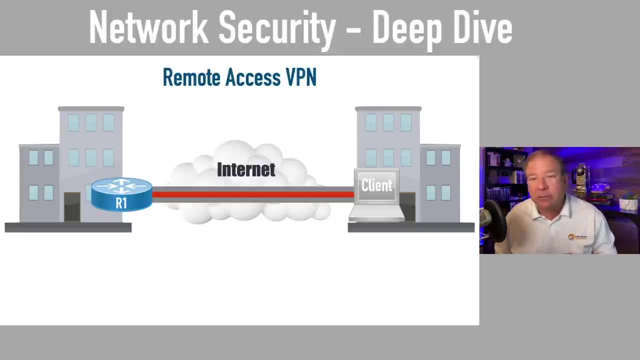 server built into it so i can set up a secure connection between whatever hotel room i'm in and the security appliance in my home. and uh yeah, it's all encrypted through the internet, but i've got to have software on my laptop to do that. so i'm going to set up a vpn and i'm going to 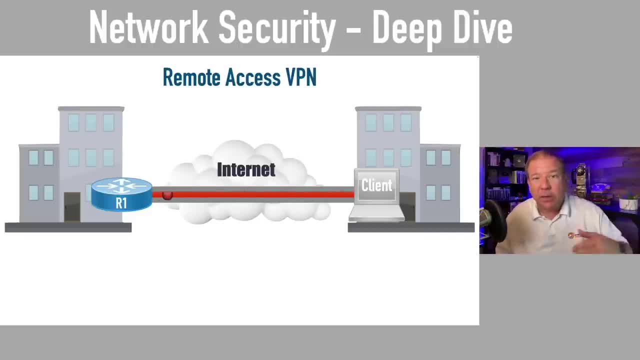 do that, but if i do, i mean it's a great solution. i'm not bound by physical location and i can be encrypted. i can have encrypted traffic sent over the internet and it doesn't even have to be necessarily software that i install. i could use clientless ssl where you go to a portal. 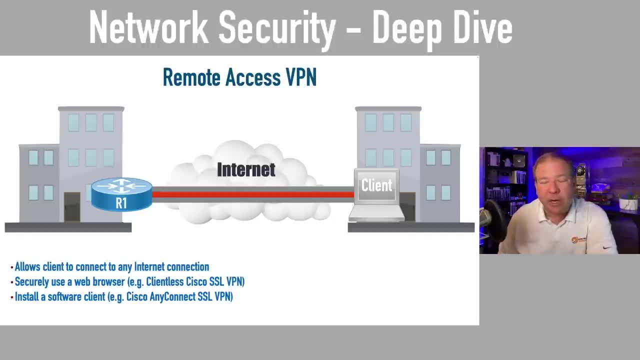 and you get through a web interface. you get secure access to selected resources at a site. but normally we're installing a software vpn on a system and that's a little extra work. so what we might do if we just want to connect two offices together, we've got a branch office. 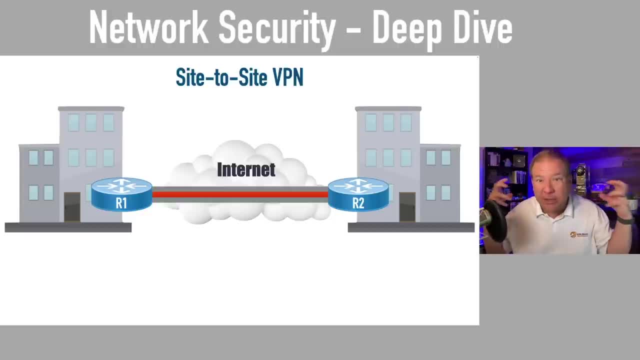 in the main office, the headquarters. what we could do is have the routers at those sites act as the endpoints in this vpn tunnel. so all the devices at the different sites- this is transparent to them- they don't have to install. they don't have to install vpn software, they just talk normally to. 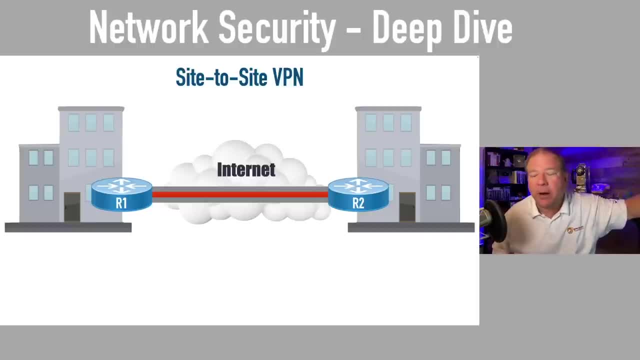 their router. they want to go back to the headquarters, no problem, the router is going to get them there. but there's configuration in the routers that are going that's going to encrypt the data going back and forth between those sites. that is a site-to-site vpn, and i remember used to uh back in the 90s when i would work with 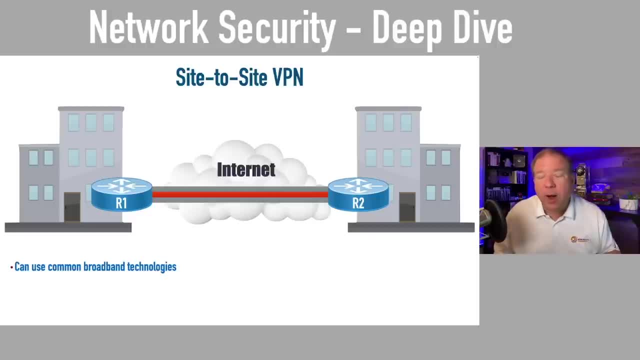 a client that wanted to connect sites together. you're probably looking at something like getting a vpn- not a vpn but a frame relay connection. i've worked on more of those than i than i care to think about a frame relay connection or maybe an atm connection if you're really bougie back in. 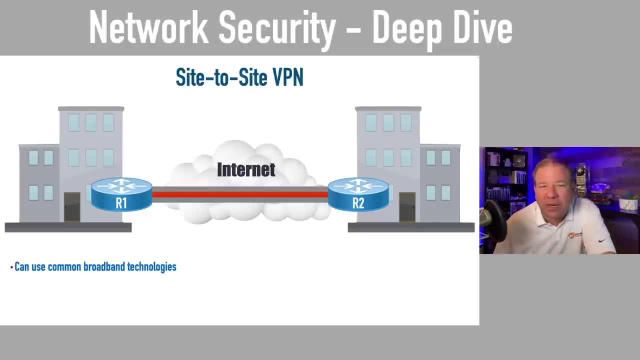 the day, or maybe a direct t1 link between a couple of sites. all those options were really expensive. i mean, i think i pay a hundred dollars a month in my home for at&t fiber and it's a gig. it's a gig up and down that's unheard of. back when i was hooking up these, uh, these businesses back in the 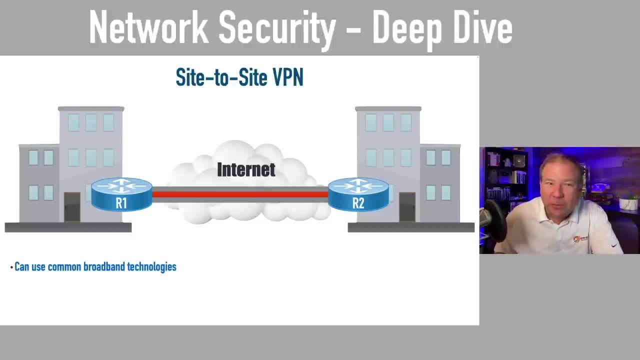 day, yeah, yeah, it's really inexpensive and really fast for a lot of locations to get to the internet. let's use that, but let's do it securely with a vpn, and that's what we can do with the site-to-site vpn and, again, this is going to be transparent to our end devices. now what i want to do now. 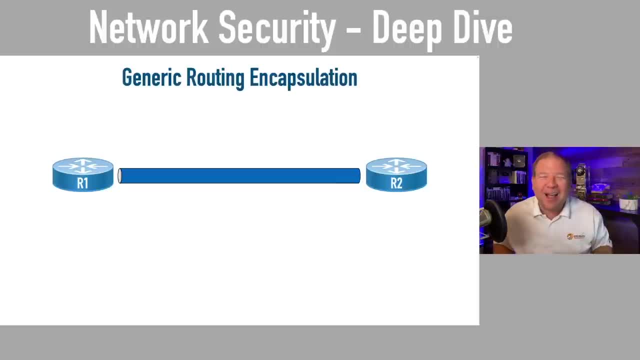 and you might want to take some notes about the vpn, and what i want to do now is i'm going to. you do want to take some notes on this. i'll just tell you i want to talk about two different vpn protocols: gre- generic routing encapsulation- and ipsec, short for ip security. first let's consider 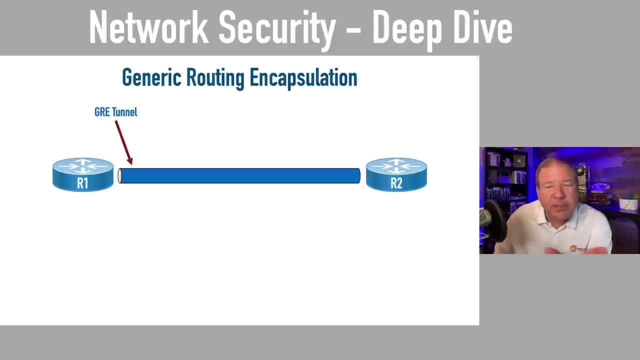 the protocol of gre, a gre tunnel. a gre tunnel is super flexible in that just about any kind of any kind of packet we can put uh send out of a router interface, we can put that in a gre tunnel. there's going to be a gre packet that wraps it up. 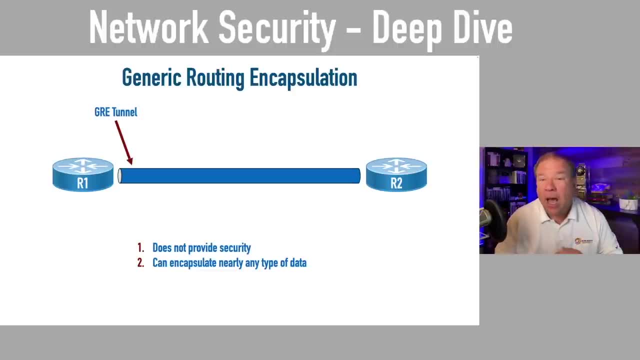 i don't care if it's unicast broadcast multicast, i don't care if it's, i don't care if it's the old novell ipx or apple talk, it doesn't matter. if you can send it out of a router interface, you're going. 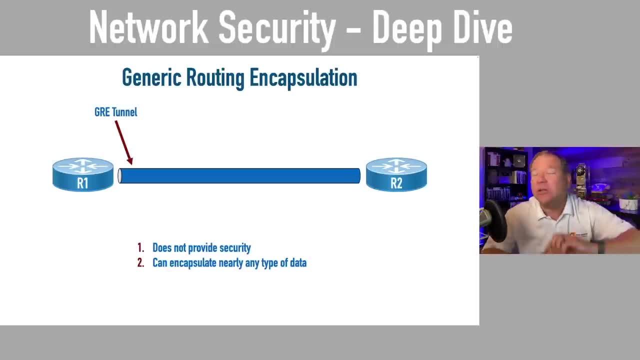 to be able to encapsulate that inside of a gre packet. it is super flexible, awesome. bad news: it's not secure at all there. there is no encryption with gre. it's not at all secure. so, oh, that kind of kills our whole, whole idea of being secure across the internet, doesn't it? 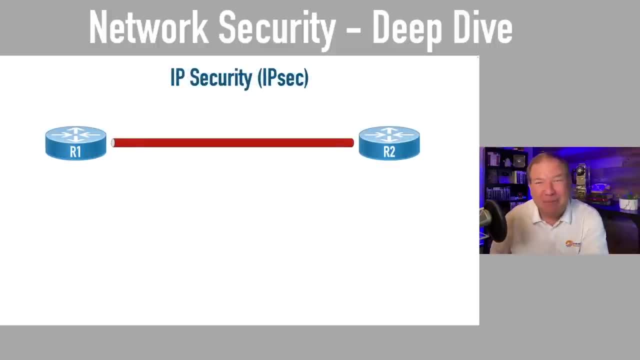 another one. here's a protocol that is very secure. it's in the name. it's ip security or ipsec. this is a super secure protocol. it's going to give us confidentiality in the form of encryption, like aes it can use. it'll give us hashing, maybe shaw. it can do authentication with pre-shared. 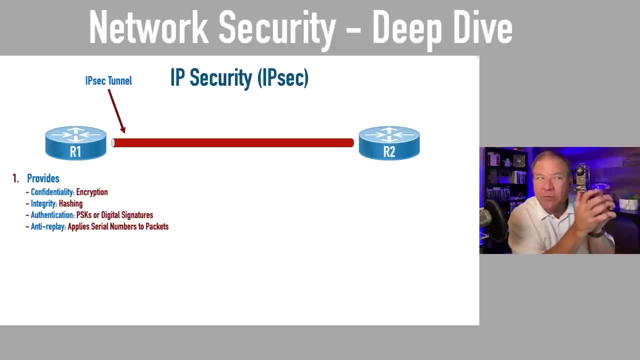 keys or digital signatures and if somebody tries to tries to capture packets as part of a valid login sequence and play those back later to get logged in, it's not going to work because ipsec is giving almost like sequential numbers to packets as they're sent across. so if i come back later and 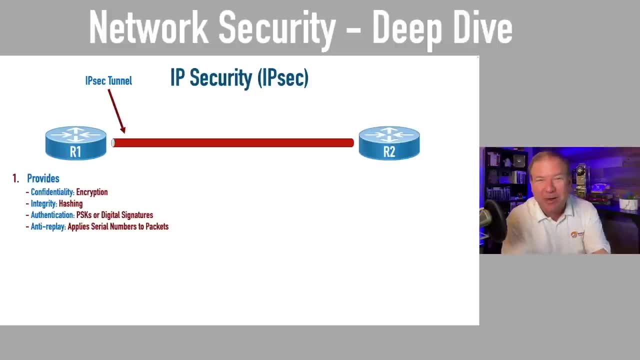 try to play back valid packets earlier. the sequence numbers are going to be all out of and it's not going to be believed. so it's very secure, awesome bad news. and the bad news is it's not flexible. whereas gre could do unicast, broadcast, multicast, whatever we wanted, ipsec is limited to. 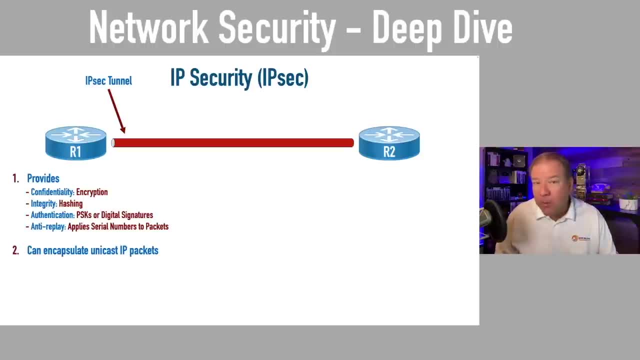 unicast ip packets only. is that a problem? you bet it's a problem because most of our routing are going to use multicast. if i'm trying to do ospf then i want to be sending traffic to the multicast addresses of 224.0.0.5 and 224.0.0.6 with uh, with rip version 2, 224.0.0.9, eigrp, 224.0.0.10. 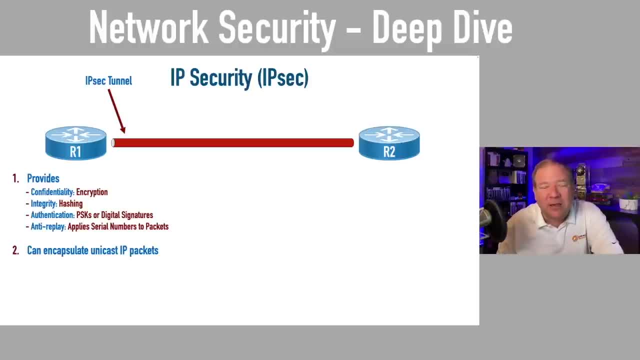 i just killed all that. if i try to send it over an ipsec tunnel, okay, well, we'll get back to that problem. but there's so many cool things about ipsec. let me give you some more features, and first i want you to understand that there are two different modes of communication. 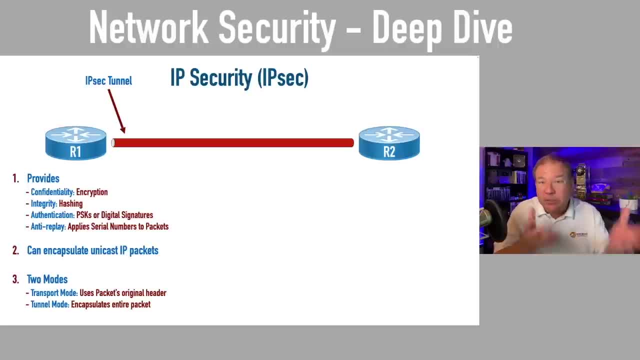 there's transport mode and there's tunnel mode. now this is a trade-off. you can have a little bit more security but you get more overhead, or you can have a little bit less security and less overhead, so it's a balancing act. what's more important to you, transport mode is going to 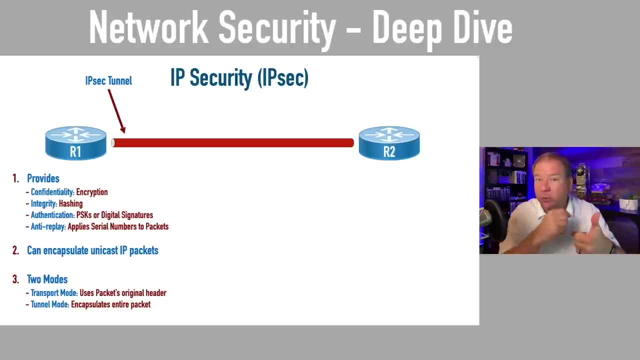 keep the original packets header intact, so the original source and ip, destination, ip addresses. they're still going to be there, they're going to be seen. however, with tunnel mode we're encapsulating the entire packet, including the original source and destination ip addresses. that means that if somebody were to capture that packet and they were to look at the source and 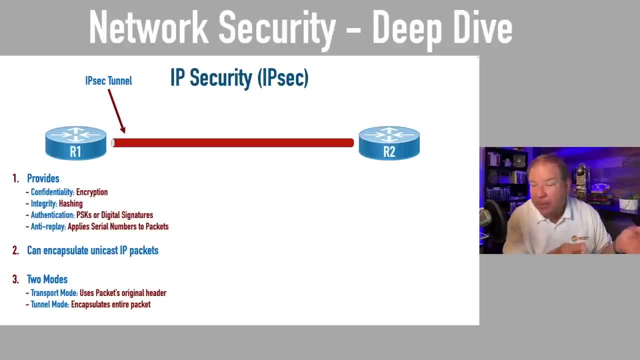 destination ips. they wouldn't see the actual ips of the actual systems involved in the conversation. they would see the ip addresses of the of the end points of the vpn tunnel, like the routers as an example. um, yeah, we're adding header information so there's more overhead, but a 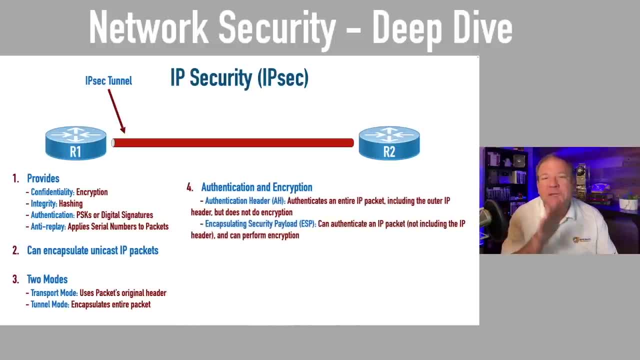 little bit better security, we can ultimately make the installation a better one. if we have a also use authentication or authentication and encryption, And we've got a couple of options here, We can do something called authentication header. It does not do encryption, but it does. 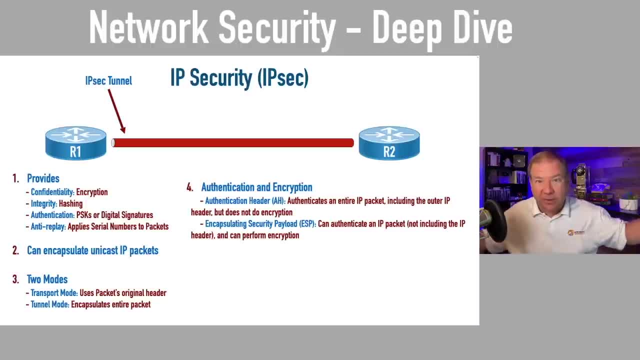 authenticate the entire IP packet, including the outer header. As compared to encapsulating security payload, it does perform encryption, but it's not going to authenticate the header. It's just going to authenticate the packet. So what's more important to you? Typically, 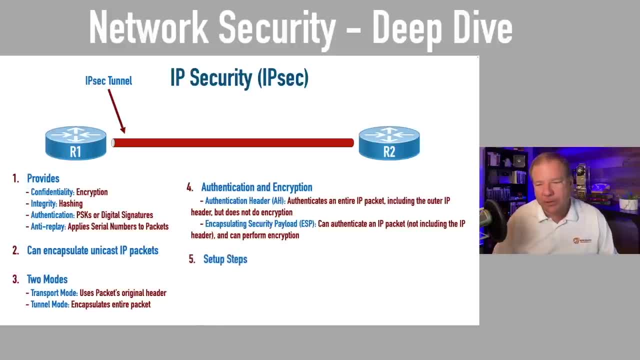 I'm going to go with ESP. That's what I. that's my normal go-to. Now. when we set up an IPsec tunnel, there are two steps involved. There's Ike phase one and Ike phase two. Now Ike, that stands. 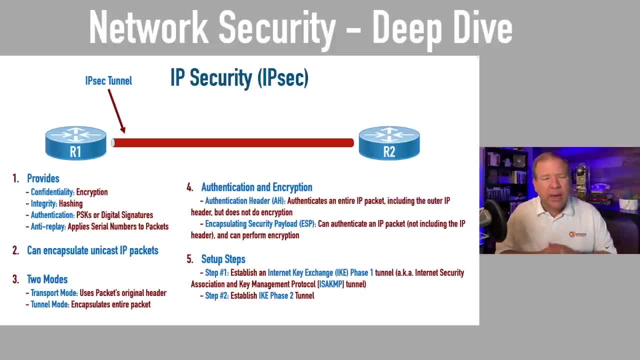 for internet key exchange And in Ike phase one is a metaphor. Did you ever watch the old TV show? or now it's a few years ago it came out as a movie with Steve Carell: Get Smart. Have you seen that one? I was a big fan of Get Smart on TV back in the back in the old days. 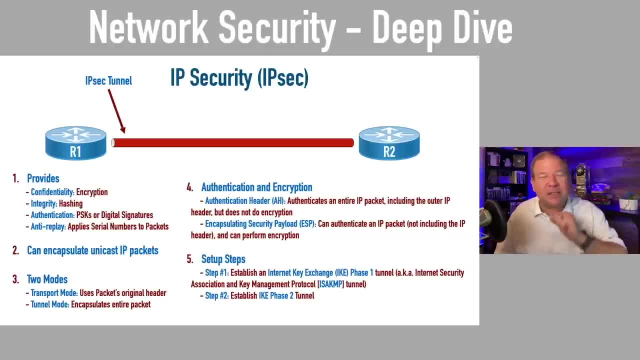 And I love the movie If you've not seen Get Smart with Steve Carell, it is hilarious, It is, it is fantastic. And whether you watch the movie or the TV shows, there's usually a scene where Max Maxwell Smart. he wants to talk to the chief and of control And he wants to talk to the chief. 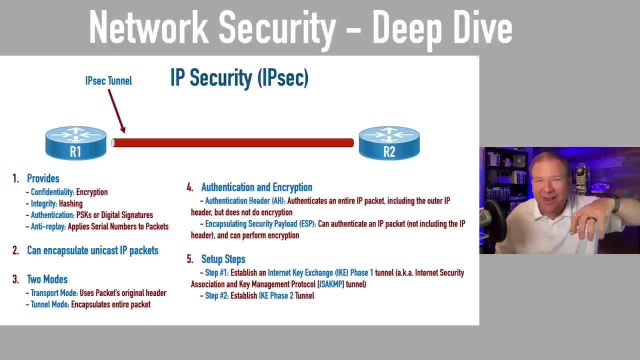 using something called the, the cone of silence, And then the old TV show was like this big plastic thing that came over them, over their heads, And it's like this sort of virtual bubble in the movie. But in the cone of silence the idea is the two parties are going to be able. 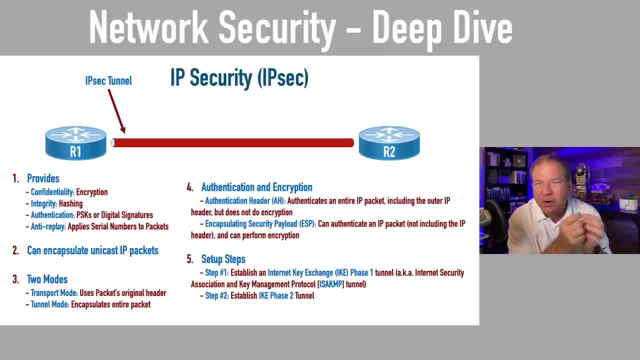 to talk to one another and nobody else is going to be able to listen in. They're not going to be able to eavesdrop in on that conversation because they're under the cone of silence Now in the movies and the TV show. for you know, for the comedy aspect it never works right. 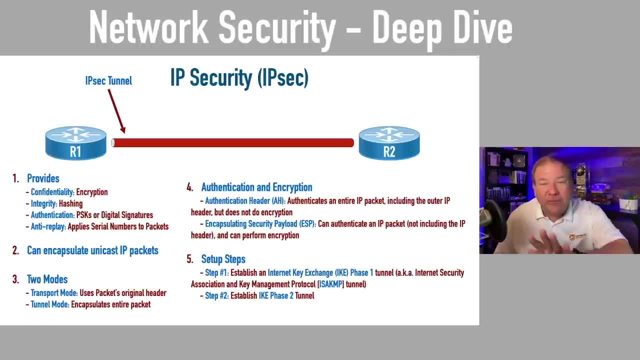 But that's kind of what's going on here with IBSEC Ike. phase one, also known as the ISECEMP phase, is we're metaphorically lowering the cone of silence over these two endpoints And that's going to give them a private communication channel. Now what's going? 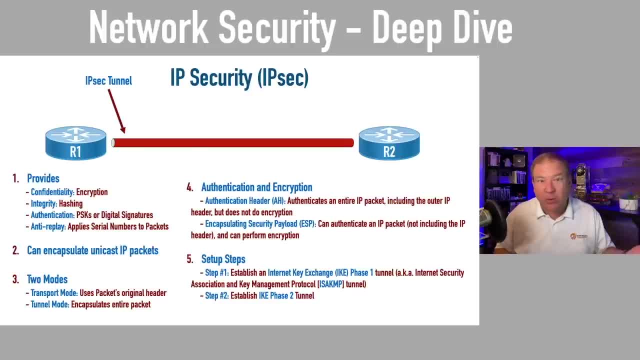 to be communicated over that private communication channel. Is it the data that we want to send? Not yet We're going to use the security of that cone of silence, the Ike phase one tunnel, to negotiate the parameters of the Ike phase two tunnel, which is the actual IBSEC tunnel. 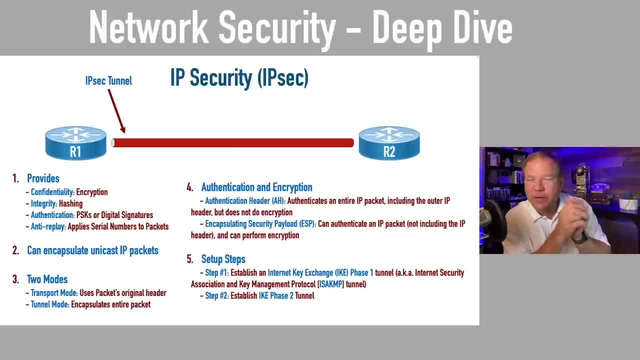 So we can say, all right, I support, I support this set of features, this transform set, And I support this, this encapsulation, or I support this encryption protocol, I support this authentication protocol, or all the things you support. Diffie-Hellman group one, two, whatever. All the parameters are going to be. 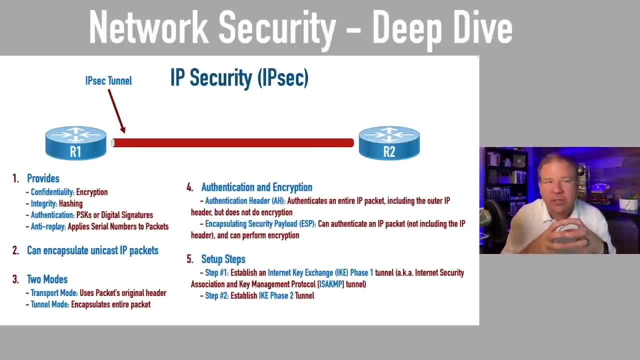 negotiated within the protection of Ike phase one tunnels And then, once the two parties agree on what they're going to be using for encryption and for integrity, they're going to set up the Ike phase two tunnel, That's the IBSEC tunnel, where the actual data is going to be sent. 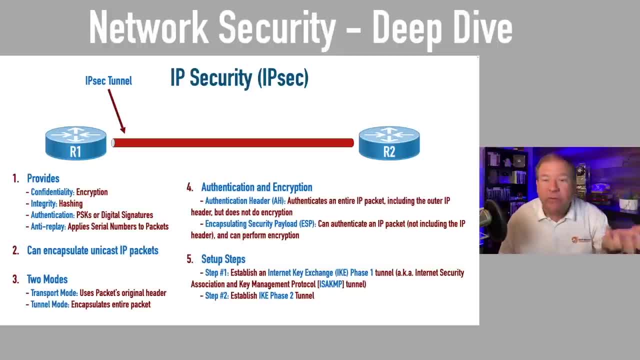 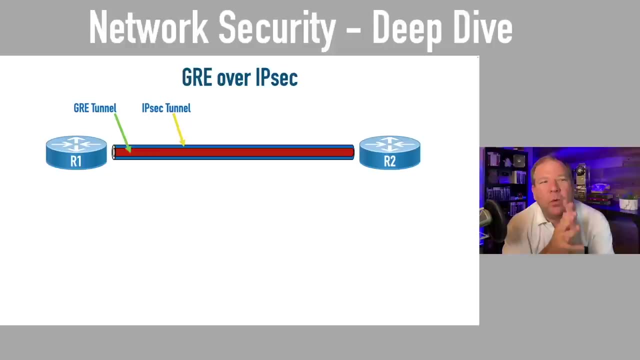 But getting back to the big paradox we have: on the one hand we've got GRE- super flexible, not secure. On the other hand, we've got IBSEC- super secure, not flexible. It only supports Unicast IP traffic. So what do we do? What if we do both? What if we do? 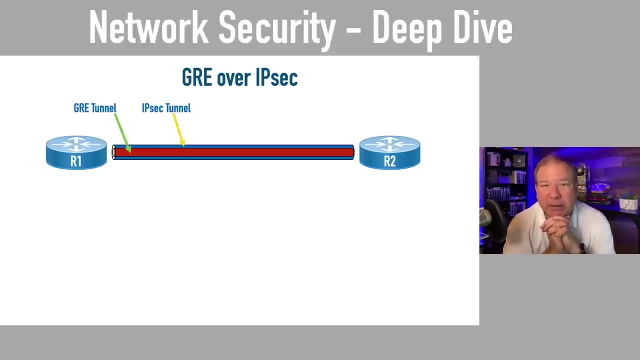 GRE and IBSEC. Here's what I mean. We can take our original packet. I don't care if it's multicast, Unicast, broadcast, whatever. We're going to take that original packet and encapsulate it inside of a GRE. 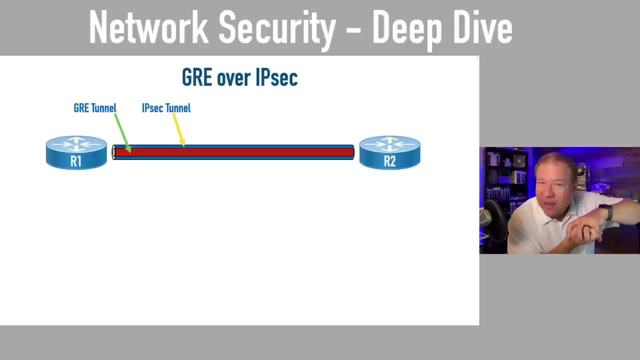 Packet. What is a GRE packet? It's a Unicast IP packet. Do you see where I'm going with this? I'm going to take that Unicast IP packet and then protect it with the security of an IBSEC tunnel. So we take whatever, wrap it up in a Unicast IP packet, a GRE packet, which can then be put inside. 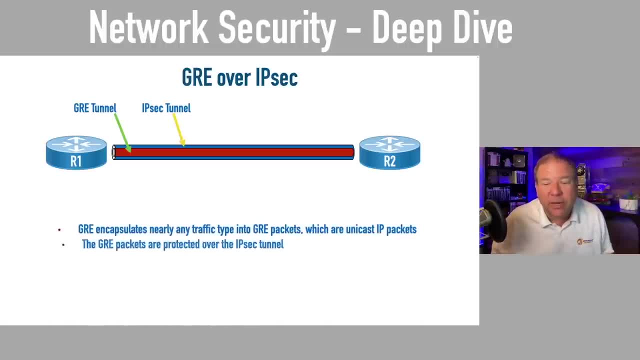 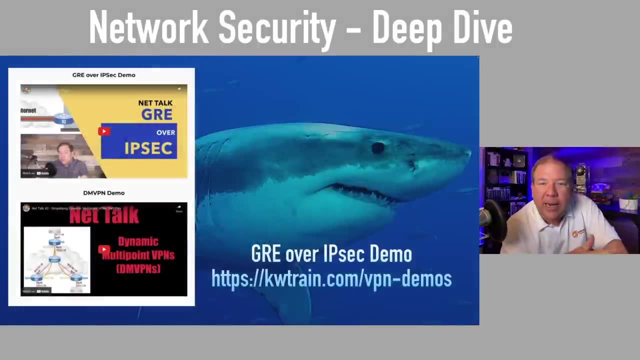 of the IBSEC tunnel. So we're going to use both. We're going to use the best of both worlds here, And that's called GRE- GRE over IBSEC- And I was originally planning to demonstrate creating a GRE over IBSEC tunnel. 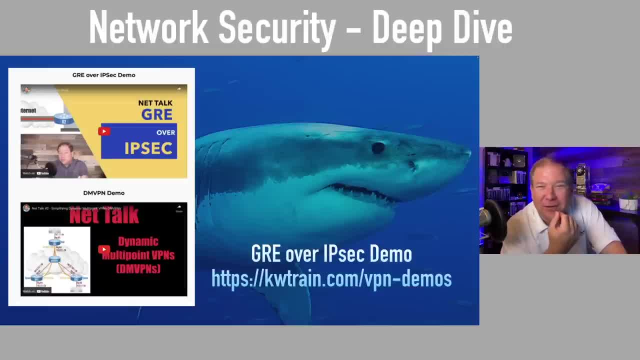 with you today. And then I realized that our session is going to be getting close to five hours And, if I added a couple of extra demos, we're looking at another hour. And then I remembered you know what? I've got a YouTube video where I'm setting this up, So I created 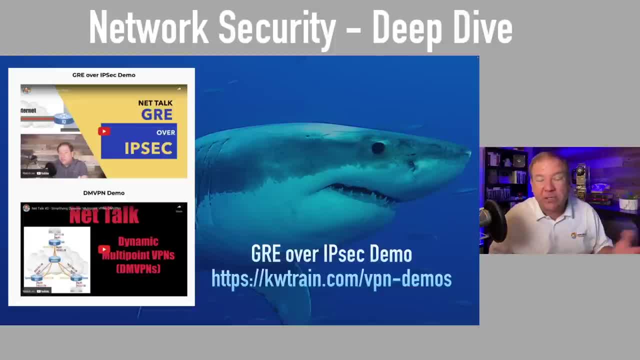 a little link for you that'll take you to a page with a couple of demos that I just didn't want to spend class time on today. But if you go to kwtraincom slash VPN hyphen demos, the first video on that page is going to be GRE over IBSEC, And I'll show you step by step how to. 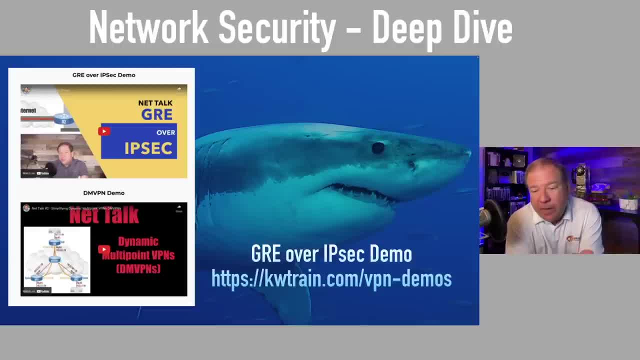 set up what we just talked about in theory when we test it out. The other video is going to be on the last topic we have coming up in just a moment, And that's dynamic multipoint VPNs. I set that up from scratch and talk about how we verify that type of VPN connection that's dynamically brought. 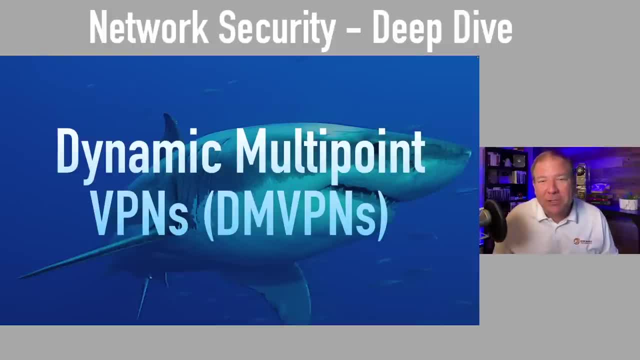 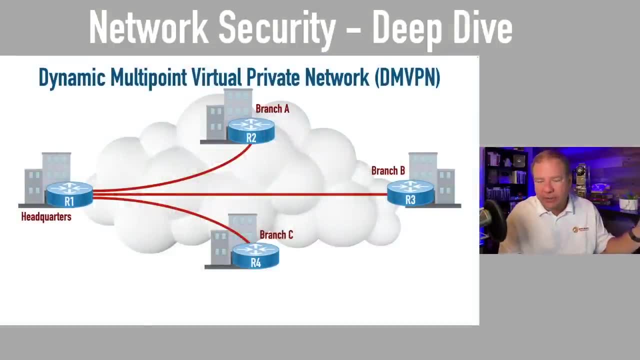 up. In fact, let's talk about that. Our final topic of the day is dynamic multipoint VPNs, or DMVPNs. The idea is this: if I have a point to multipoint topology like this, maybe I have all these direct connections, Maybe they're, I don't know if they're. 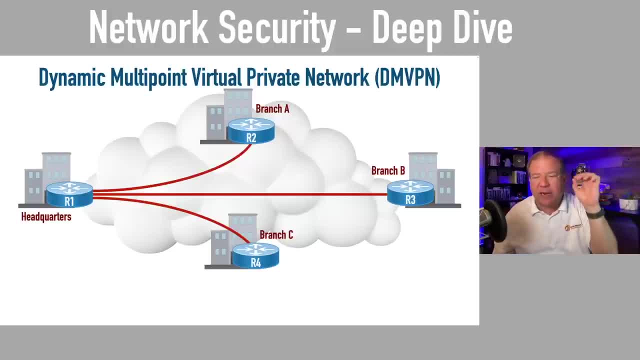 Metro Ethernet connections, maybe MPLS connections, but virtually I've got a connection from the headquarters to branch A, I've got a connection from the headquarters to branch B and a connection from the headquarters to branch C. Well, from time to time, even though most of the communication 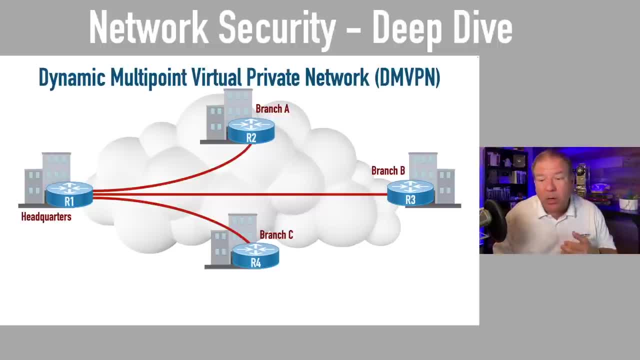 goes between the branch office and the headquarters. there might be times when I want to go from C directly to branch B And right now it's going to be hairpin. It's going to go back to the headquarters and then it's got to go to branch B. It'd be great if I could do that over the 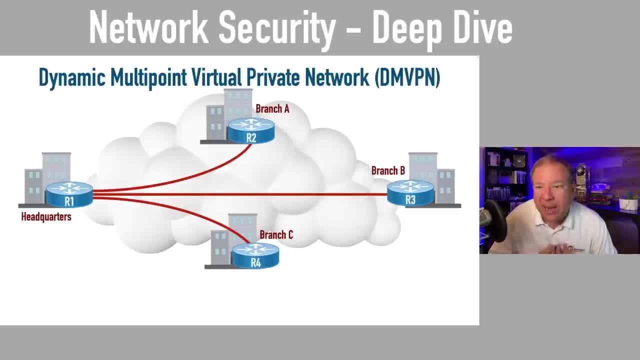 internet directly with branch B, wouldn't it? But I don't want to pay to have a permanent virtual circuit set up all the time between our two sites, But when I need it, I'd sure like to bring up a dynamic multipoint VPN over the internet. Let's dynamically bring it up when. 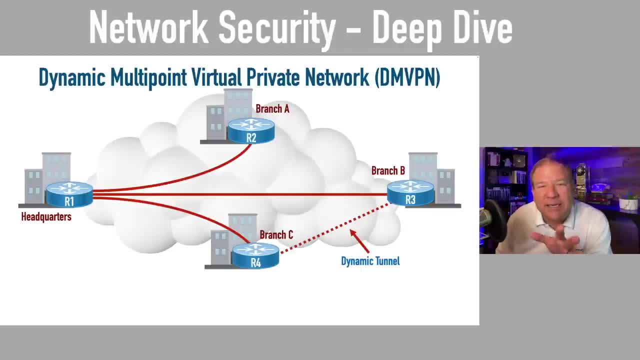 we need it, And when we don't need it, let's tear it back down. That's what DMVPNs let us do. They allow us to, on the fly, dynamically bring up a tunnel between these two sites, And it's going to use something called multipoint GRE. Again that video, and I'll give you that. 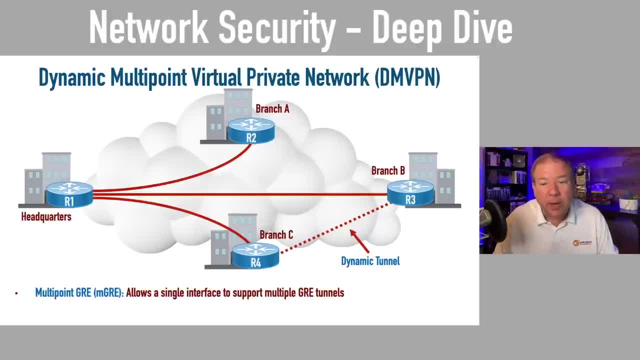 link again here in a moment. but that video walks you through how we set up a multipoint GRE interface, And the idea is this: We're going to use the Nextop resolution protocol to figure out the publicly available IP address with which we should set up this dynamic tunnel. You see, 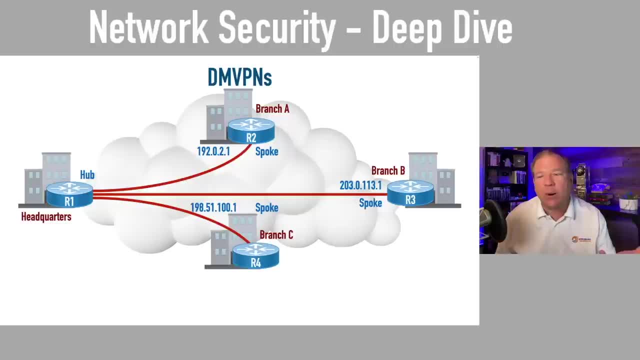 I've got. within branch A, I've got a private network. Maybe it's the 10-dot address space. In branch B, I've got maybe it's the 172.16 address space In branch C. maybe I've got the. 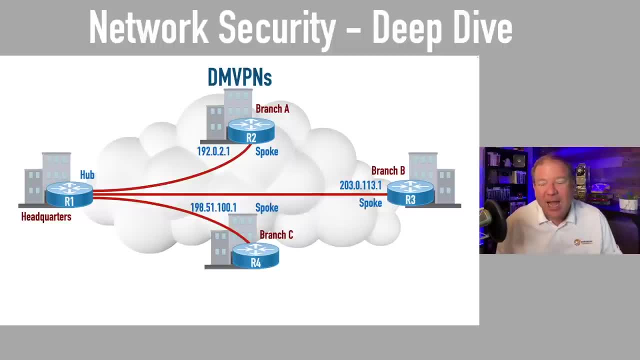 192.168.1.0-24 address space. I've got private IP addresses within my sites And if I'm advertising, maybe like OSPF or EIGRP, I'm advertising out to the hub. here are the networks I have, And then 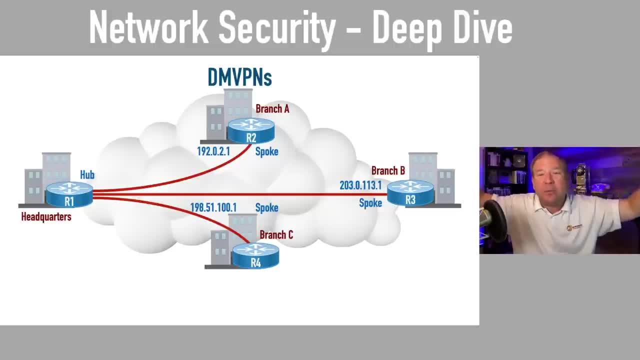 the hub relays that to the other remote sites and say here are the networks that branch C has. Branch B might say: wow, I'd really like to talk to that network over at branch C, but it's a private IP address And I have to get to it over the public internet. 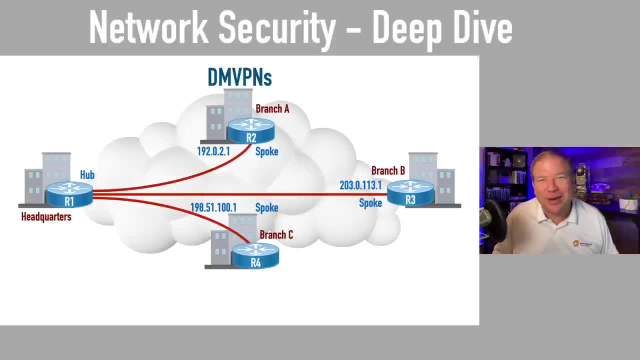 How's that going to work? I cannot route to the 192.168.1.0-24 network over the internet. It's private. It's RFC 1918 private IP addressing. That's not going to work. It cannot be routed. 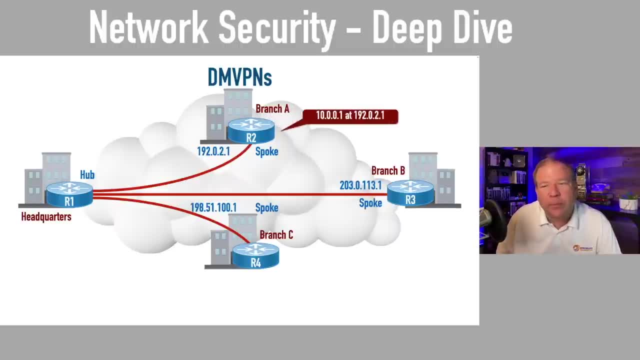 over the public internet. So what we do is use the Nextop resolution protocol- and here I'm actually used a different set of private IP addresses in this example. But what we're going to do is we're going to tell this database back at the headquarters. 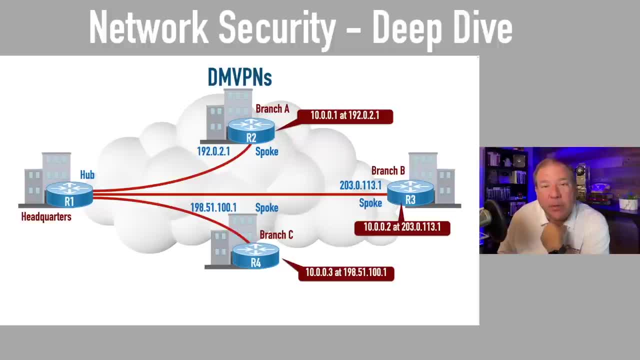 hey, if anybody wants to set up a tunnel with me, here's my publicly routable IP address. on the outside of my router that goes out to the internet. Here's my publicly routable IP address If they would like to set up a tunnel with that IP address. yeah, I'm game, Let's dynamically set. 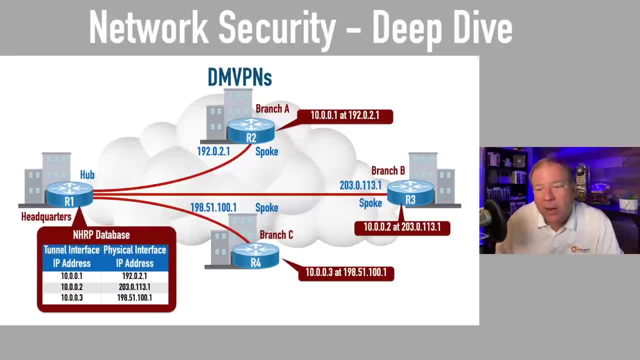 up a tunnel. Let's set up a tunnel with that IP address. Let's set up a tunnel with that IP address And then they can get to the private IP addresses within my network. So here's the database on that hub router. We see the IP address that's going to be on the other end of the tunnel. 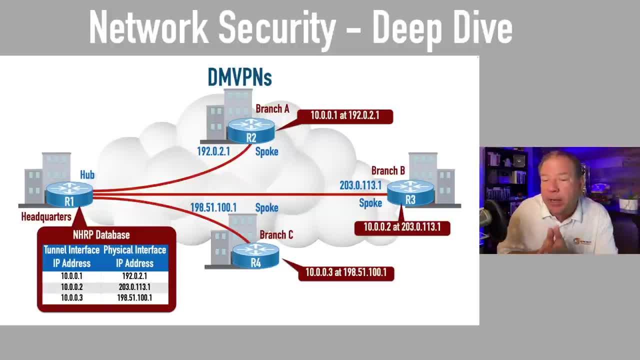 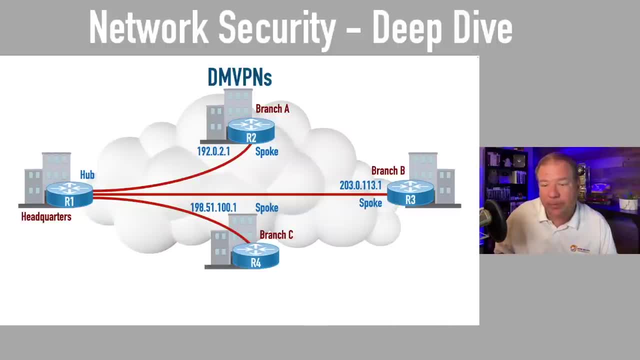 the private IP address and we see the physically publicly routable IP address that we'll use to set up that tunnel. Let's go through an example. Let's say that R4 at break C, it wants to set up a tunnel. Let's say that R4 at break C, it wants to set up a tunnel. 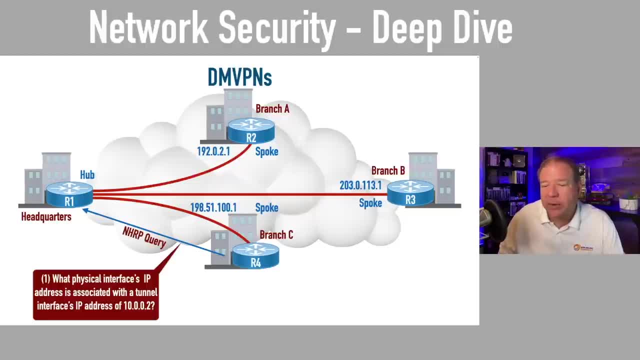 It wants to talk to this network of 10, or it wants to talk to the IP address of 10.0.0.2, which I believe was the branch B router. It wants to set up a tunnel with that, However. 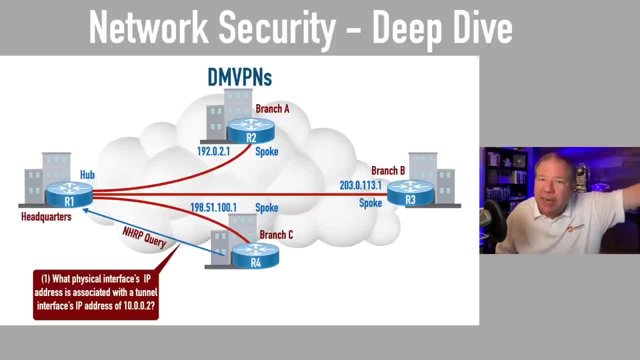 it doesn't know the publicly routable IP address to use. So it sends up a next top resolution protocol in HRP query saying: hey, what's the public IP address I can use to get to 10.0.0.2?. 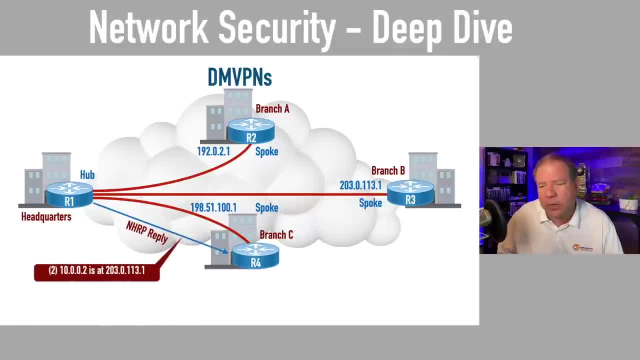 And the hub says: oh, you want to go talk over to 203.0.113.1, R3.. That is a public IP address. So dynamically, R4 is going to set up this link with R3.. It's going to dynamically. 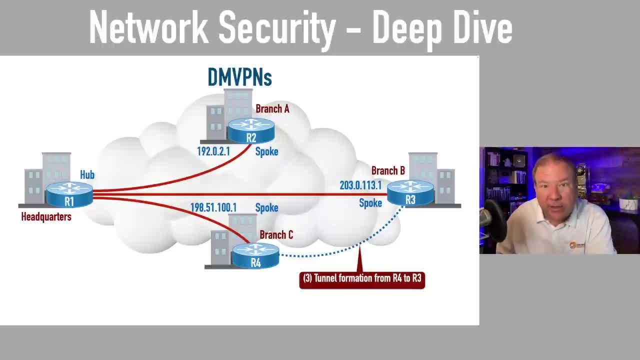 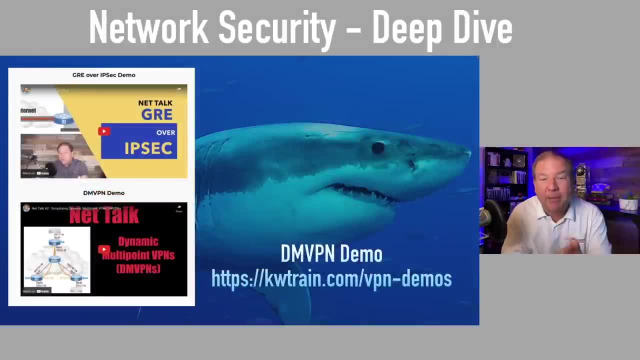 form that tunnel which is then going to allow users at branch C to get to the private IP address space inside of branch B over that dynamic tunnel. Again, if you want to see step-by-step how all that is set up, just go to kwtraincom slash VPN, hyphen demos And I've got those two VPN. 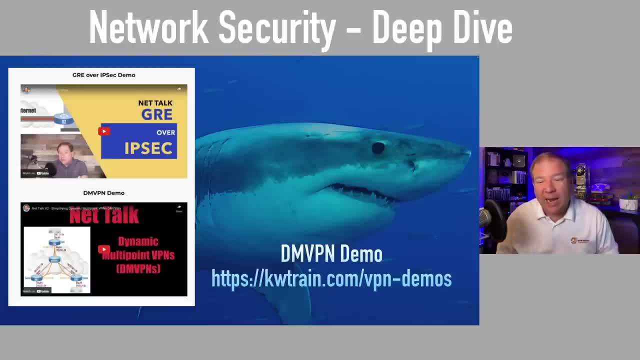 demos on there for you: The first one, GRE, over IPsec, and there's one on setting up IP address Dynamic multi-point VPNs. It would have added probably more than an hour to have done all that live for you today, So we're already getting long, So we will go ahead and let you watch those.